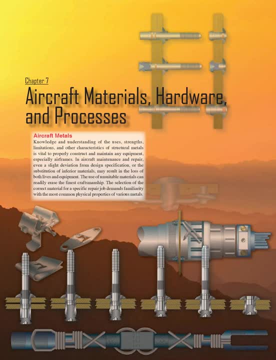 specification or the substitution of inferior materials may result in the loss of both lives and equipment. The use of unsuitable materials can readily erase the finest craftsmanship. The selection of the correct material for a specific repair job demands familiarity with the most common physical properties of various metals. Properties of metals of primary concern. 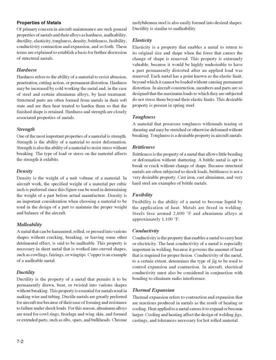 in aircraft maintenance are such general properties of metals and their alloys as hardness, malleability, ductility, elasticity, toughness, density, brittleness, fusibility, conductivity, contraction and expansion, and so forth. These terms are explained to establish. 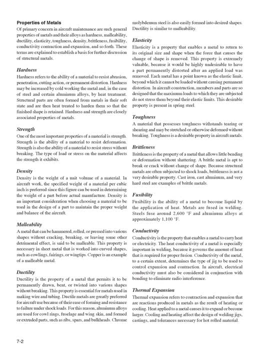 a basis for further discussion of structural metals Hardness. Hardness refers to the ability of a material to resist abrasion, penetration, cutting action or permanent distortion. Hardness may be increased by cold working the metal and, in the case of steel and certain aluminum alloys, by heat treatment. Structural parts are often 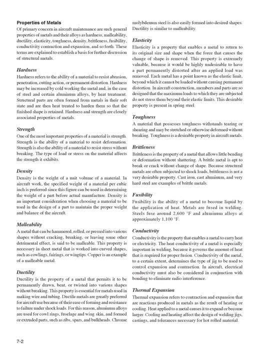 formed from metals in their soft state and are then heat treated to harden them so that the finished shape is retained. Hardness and strength are closely associated properties of metals. Strength- One of the most important properties of a material- is strength. Strength is the 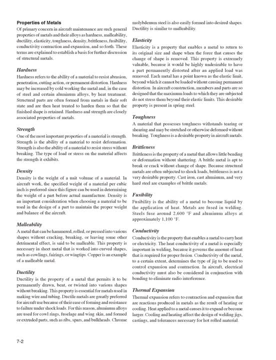 ability of a material to resist deformation. Strength is also the ability of a material to resist stress without breaking. The type of load or stress on the material affects the strength it exhibits. Density: Density is the weight of a unit volume of a material In aircraft work. the specified weight: 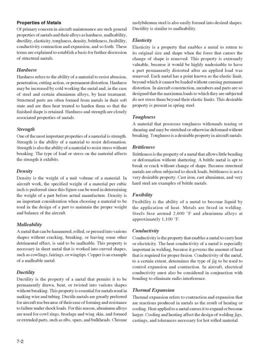 of a material per inch 3 is preferred, since this figure can be used in determining the weight of a part before actual manufacture. Density is an important consideration when choosing a material to be used in the design of a part to maintain the proper weight of a part. The weight of a part is: 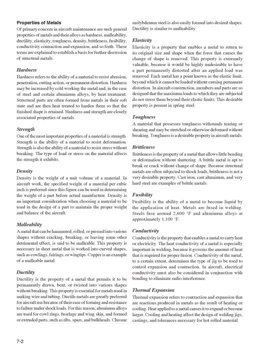 achieved when the part of the part is held in the right place from the left place. Strength- Yes, this is the part of a material to be used. Strength- Yes, this is the part of a material to be used. Strength- It is the part of a material to be used to control the weight and balance of the aircraft. 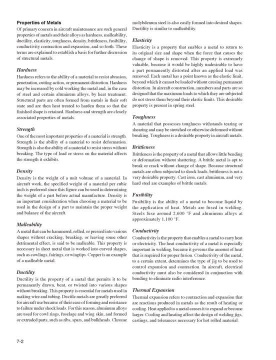 Strength, Malleability- A metal that can be hammered, rolled or pressed into various shapes without cracking, breaking or leaving some other detrimental effect is said to be malleable. This property is necessary in sheet metal that has worked into curved shapes such as cowlings, fairings or wingtips. Copper is an 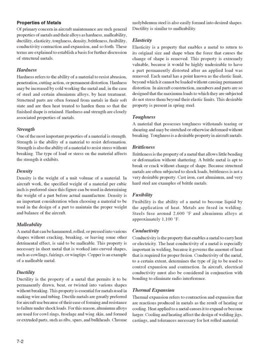 example of a malleable metal: Ductility. Ductility is the property of a metal that permits it to be permanently drawn, bent or twisted into various shapes without breaking Strength. Strength- Strength, Strength- essential for metals used in making wire and tubing, Ductile metals are greatly preferred. 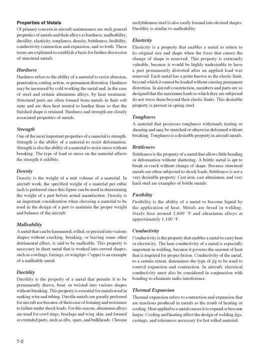 for aircraft use because of their ease of forming and resistance to failure under shock loads. For this reason, aluminum alloys are used for cowl rings, fuselage and wing skin and formed or extruded parts such as ribs, spars and bulkheads. Chromolybdenum steel is 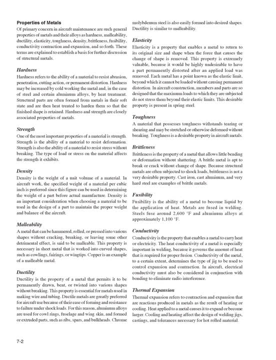 also easily formed into desired shapes. Ductility is similar to malleability- Elasticity. Elasticity is a property that enables a metal to return to its original size and shape when the force that causes the change of shape is removed. This property is 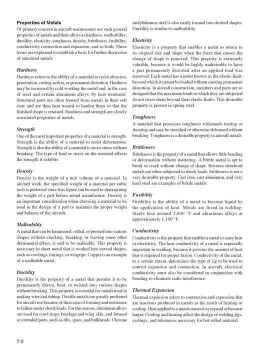 extremely valuable because it would be highly undesirable to have a part permanently distorted after an applied load was removed. Each metal has a point, known as the elastic limit, beyond which it cannot be loaded without causing permanent distortion. In aircraft construction members and parts are so designed that the maximum loads to which they are subjected do not stress them. 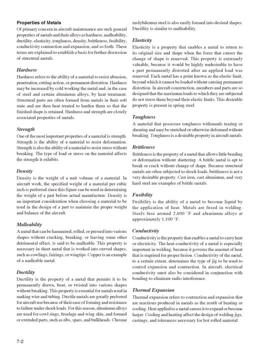 beyond the elastic limit. This desirable property is present in spring steel Toughness, A material that possesses toughness, withstands tearing or shearing and may be stretched or otherwise deformed without breaking Toughness, is a desirable property in aircraft metals Brittleness. Brittleness is the property of a metal that 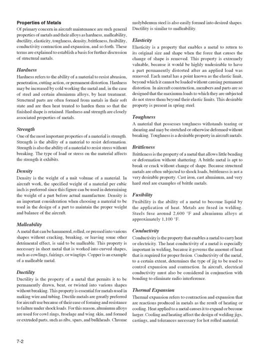 allows little bending or deformation without shattering. A brittle metal is apt to break or crack without change of shape. Because structural metals are often subjected to shock loads, brittleness is not a very desirable property. Cast iron, cast aluminum and very hard steel are examples of brittle metals. 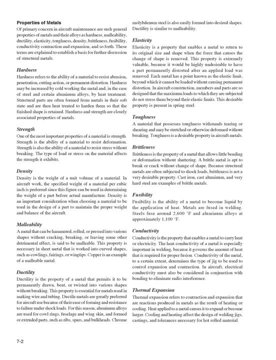 Fusibility: Fusibility is the ability of a metal to become liquid by the application of heat. Metals are fused in. welding. Steels fuse around 2,600 degree Fahrenheit and aluminum alloys at approximately 1,100 degrees Fahrenheit. Conductivity: Conductivity is the property that enables a metal. 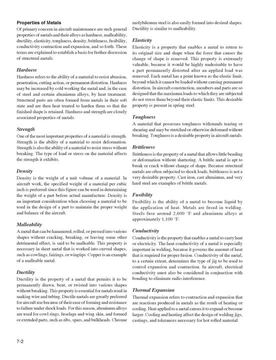 to carry heat or electricity. The heat conductivity of a metal is especially important in welding because it governs the heat of the metal. The heat conductivity of a metal is especially important in welding because it governs the heat of the metal. The heat conductivity of a metal is especially important in welding because it governs the amount of heat that is required for proper fusion. 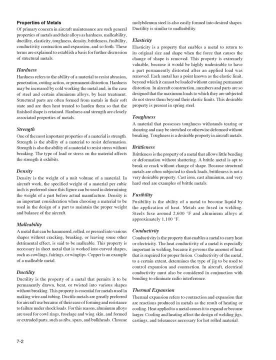 Conductivity of the metal to a certain extent determines the type of jig to be used to control expansion and contraction In aircraft. electrical conductivity must also be considered in conjunction with bonding to eliminate radio interference. Thermal expansion: Thermal expansion refers to contraction and expansion that are reactions produced in metals as the result of heating. 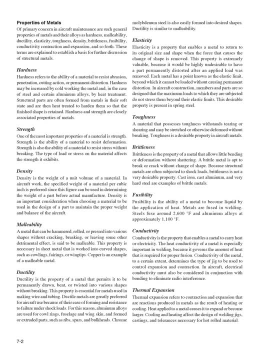 or cooling. Heat applied to a metal causes it to expand or become larger. Cooling and heating effect that design a metal is the property of a metal. The heat conductivity of a metal is especially important in welding because it governs the heat of the metal. 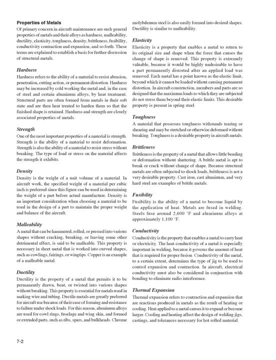 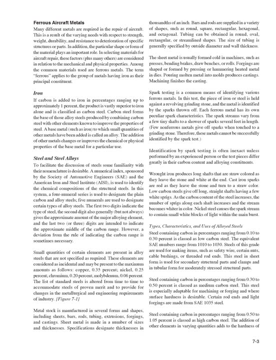 rices necessary for hot rolled material. Ferrous aircraft metals. Many different metals are required in the repair of aircraft. This is a result of the varying needs with respect to strength, weight, durability and resistance to deterioration of specific structures or parts. In addition, 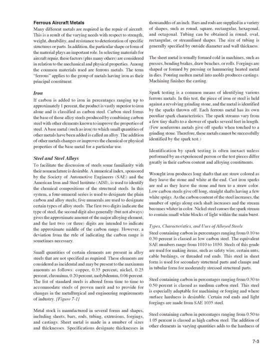 the particular shape or form of the material plays an important role In selecting materials for aircraft repair. these factors, plus many others, are considered in relation to the mechanical and physical properties in landscape Cavaliers. are considered in relation to the mechanical and physical properties in landscape Cavaliers. 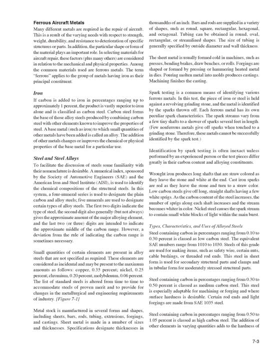 properties. Among the common materials used are ferrous metals. The term ferrous applies to the group of metals having iron as their principal constituent, Iron. if carbon is added to iron in percentages ranging up to approximately 1%, The product is vastly superior to iron alone and is 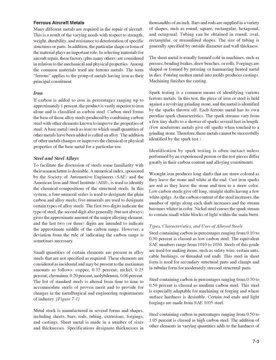 classified as carbon steel. Carbon steel forms the base of those alloy steels produced by combining carbon steel with other elements known to improve the properties of steel. A base metal, such as iron, to which small quantities of other metals have been added, is called an alloy. The addition. 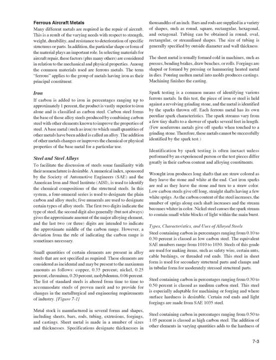 of other metals changes or improves the chemical or physical properties of the base metal for a particular use. Steel and steel alloys. to facilitate the discussion of steels, some familiarity with their nomenclature is desirable- A numerical index sponsored by the Society of Automotive. 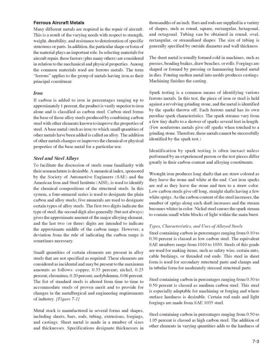 Engineers, SAE and the American Iron and Steel Institute. AISI is used to identify the chemical compositions of the structural steels. In this system, a four-numeral series is used to designate the plain carbon and alloy steels. five numerals are used to designate certain types of alloy steels. The first two digits indicate the. 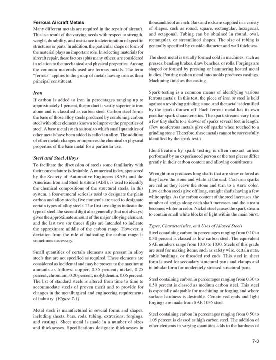 type of steel. the second digit also generally, but not always, gives the approximate amount of the major alloying element, and the last two or three digits are intended to indicate the approximate middle of the carbon range. However, a deviation from the rule of indicating the carbon 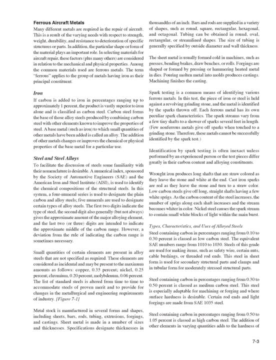 range is sometimes necessary. These elements are considered as incidental and may be present to the maximum amounts as follows: copper: 0.35%. nickel: 0.25%. chromium 0.20%. molybdenum: 0.06%. 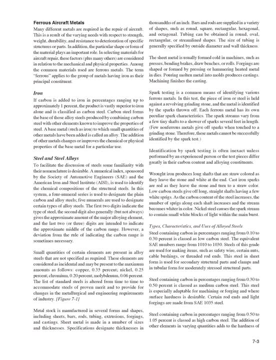 The list of standard steels is altered from time to time to accommodate steels of proven merit and to provide for changes in the metallurgical and engineering requirements of industry. Figure 7-1.. Metal stock is manufactured in several forms and shapes, including sheets, bars, rods, tubing. 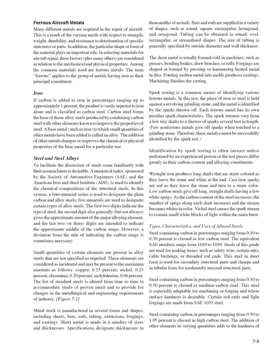 extrusions, forgings and castings. Sheet metal is made in a number of sizes and thicknesses. Specifications designate thicknesses in thousandths of an inch. Bars and rods are supplied in a variety of shapes, such as round, square, rectangular, hexagonal and octagonal. 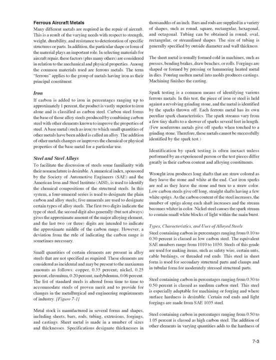 Tubing can be obtained in round, oval, rectangular or streamlined shapes. The size of tubing is generally specified by outside diameter and wall thickness. The sheet metal is usually formed cold. in machines such as presses, bending brakes, draw benches or rolls, Forgings are shaped or formed by pressing. 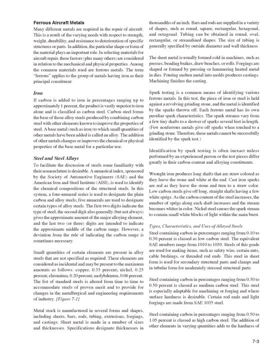 or hammering heated metal in dies. Pouring molten metal into molds produces castings. Machining finishes the casting. Spark testing is a common means of identifying various ferrous metals. In this test, the piece of iron or steel is held against a revolving grinding stone. 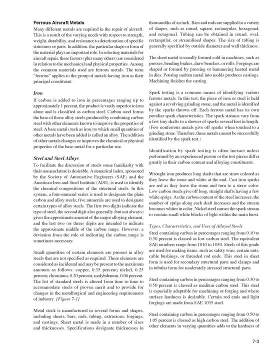 and the metal is identified by the source. The metal is then casted into the mold. The metal is thrown off. Each ferrous metal has its own peculiar spark characteristics. The spark streams vary from a few tiny shafts to a shower of sparks several feet in length. Few non-ferrous metals. 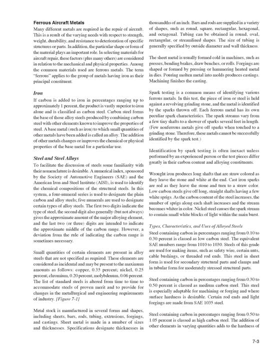 give off sparks when touched to a grinding stone. Therefore, these metals cannot be successfully identified by the spark test. Identification by spark testing is often inexact, unless performed by an experienced person, or the test pieces differ greatly in their carbon content and alloying constituents. 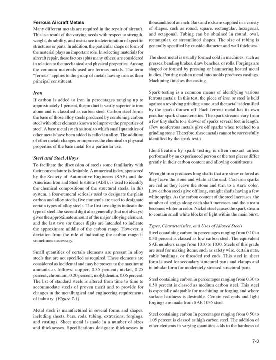 The carbon content of the steel increases as the number of sprigs along each shaft increases and the stream becomes whiter in color. Nickel steel causes the spark stream to contain small white blocks of light within the main burst. Types, characteristics and uses of alloyed steel steel. 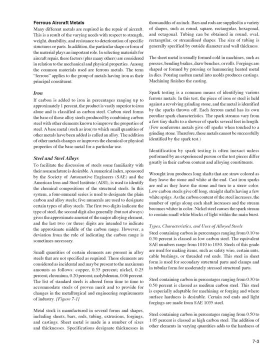 containing carbon and percent ranging from 0.10 to 0.30% is classed as low carbon steel. The equivalent say numbers range from 1010 to 1030.. Steels of this grade are used for making items such as safety wire. 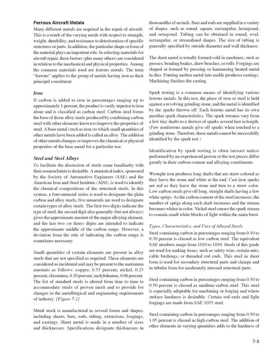 certain nuts, cable bushings or threaded rod ends. This steel in sheet form is used for secondary structural parts and clamps, and in tubular form for moderately stressed structural parts. Steel containing carbon in percentages ranging from 0.30 to 0.50% is classed as medium. 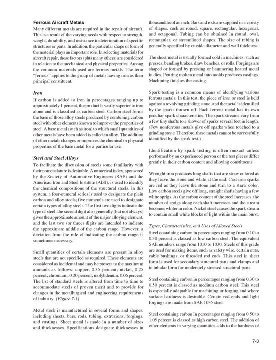 carbon steel. This steel is especially adaptable for machining or forging and where surface hardness is desirable. Certain rod ends and light forgings are made from, say, 1035 steel. Steel containing carbon in percentages ranging from 0.50 to 1.05% is classed as high carbon steel. 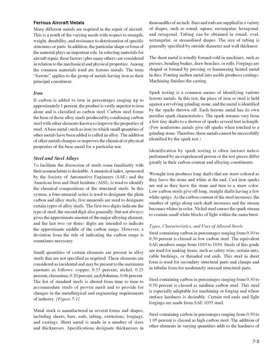 The addition of other elements in varying quantities adds to the high carbon steel. Steel containing carbon in percentages ranging from 0.50 to 1.05% is classed as hardness of This steel. in the fully heat treated condition it is very hard. withstands high shear. 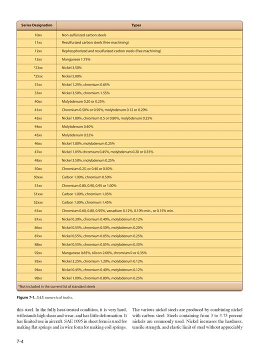 and wear and has little deformation. It has limited use in aircraft. Say 1095 in sheet form is used for making flat springs and in wire form for making coil springs. The various nickel steels are produced by combining nickel with carbon steel Steels containing from 3 to 3.75% nickels. 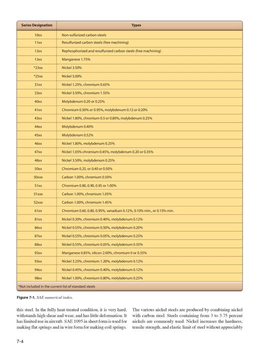 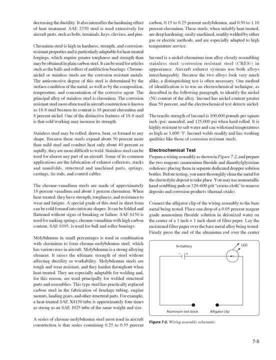 are commonly used. Nickel increases the hardness, tensile strength and elastic limit of steel without appreciably decreasing the ductility. It also intensifies the hardening effect of heat treatment. Say 2330. steel is used extensively for aircraft parts such as bolts, terminals. 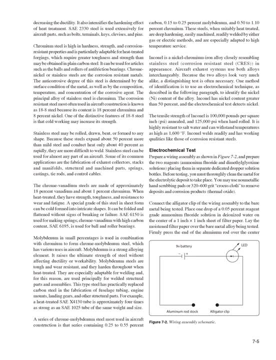 keys, cleavises and fins. Chromium steel is high in hardness, strength and corrosion resistant properties and is particularly adaptable for heat treated forgings, which require greater toughness and strength than may be obtained in plain carbon steel. It can be used for articles such as the: 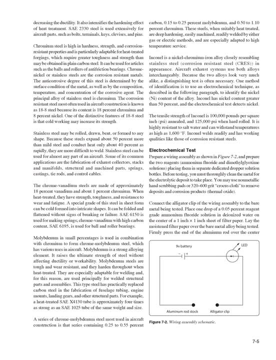 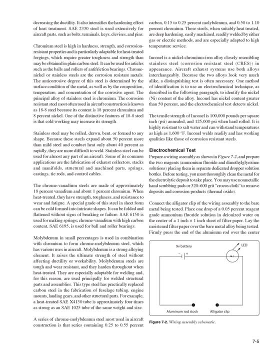 of the metal, as well as by the composition, temperature and concentration of the corrosive agent. The principal alloy of stainless steel is chromium. The corrosion resistant steel most often used in aircraft construction is known as 18 to 8 steel because its content is 18%. 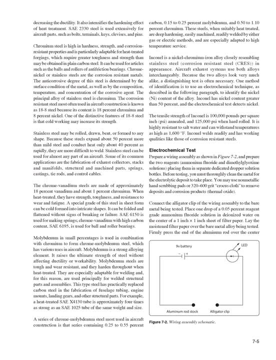 chromium and 8% nickel. One of the distinctive features of 18 to 8 steel is that cold working may increase its strength. Stainless steel may be rolled, drawn, bent or formed to any shape, Because these steels expand about 50% more than mild steel and conduct heat only about 40%. 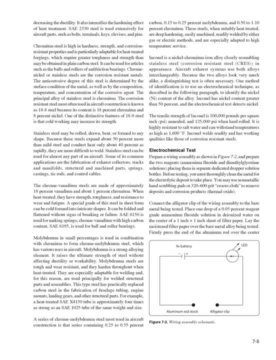 as rapidly, they are more difficult to weld. Stainless steel can be used for almost any part of an aircraft. Some of its common applications are the fabrication of exhaust collectors, stacks and manifolds, structural and machined parts, springs, castings, tie rods and control. 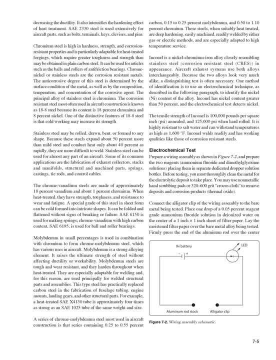 cables. The chrome vanadium steel is the most common application of stainless steel. The chrome vanadium steel is the most common application of stainless steel. are made of approximately 18% vanadium and about 1% chromium. When heat treated they have strength. 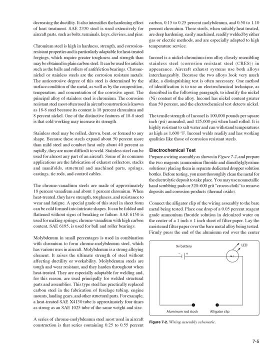 toughness and resistance to wear and fatigue. A special grade of this steel in sheet form can be cold formed into intricate shapes. It can be folded and flattened without signs of breaking or failure. Say 6150 is used for making springs. chrome vanadium with high carbon content. 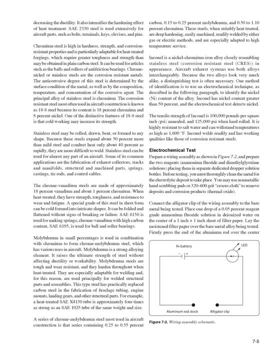 say 6195, is used for ball and roller bearings. Molybdenum, in small percentages, is used in combination with chromium to form chrome molybdenum steel, which has various uses in aircraft. Molybdenum is a strong alloying element. It raises the ultimate strength of steel without 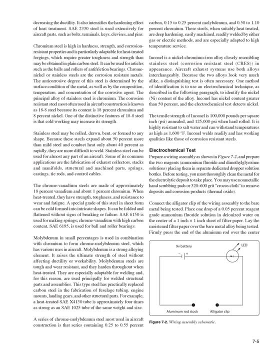 affecting ductility or workability. Molybdenum steels are tough and wear resistant, and they harden throughout when heat treated. They are especially adaptable for welding and for this reason are used principally for welded structural parts and assemblies. This type steel has 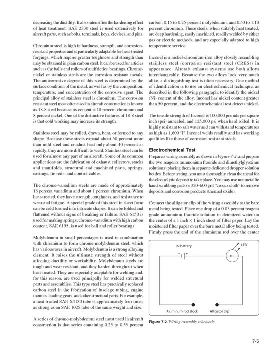 practically replaced carbon steel in the fabrication of fuselage tubing, engine mounts, lending gears and other structural parts. For example, a heat-treated say X4130 tube is approximately four times as strong as an say 1025 tube of the same weight and size. 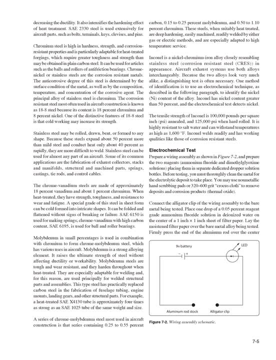 A series of chrome molybdenum steel most used in aircraft construction is that series containing 0.25 to 0.55 percent carbon, 0.15 to 0.25 percent molybdenum and 0.50 to 1.10 percent chromium. 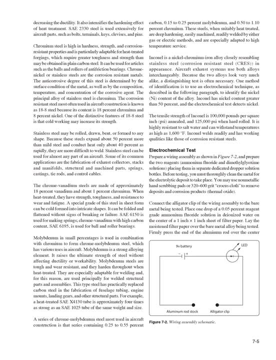 These steels, when sealed, are used for welding and assembly. They are suitably heat-treated, are deep-hardening, easily machined, readily welded by either gas or electric methods and are especially adapted to high-temperature service. Inconel is a nickel-chromium. 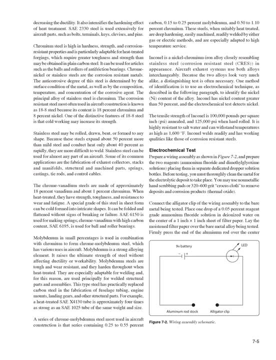 iron alloy closely resembling stainless steel, corrosion-resistant steel, CREs- in appearance. Aircraft exhaust systems use both alloys interchangeably. Because the two alloys look very much alike, a distinguishing test is often necessary. One method of identification is to use an electrochemical technique, as described in the article. The two alloys are used to. 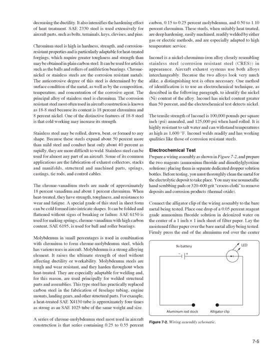 identify the nickel content of the alloy. Inconel has nickel content greater than 50 percent and the electrochemical test detects nickel. The tensile strength of Inconel is 100,000 pounds per square inch psi annealed and 125,000 pounds per square inch when hard-rolled. 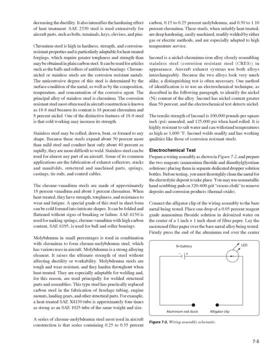 It is highly resistant to salt water and can withstand temperatures as high as 1,600 degrees Fahrenheit. Inconel welds readily and has working qualities like those of corrosion-resistant steel. Electrochemical test. prepare a wiring assembly as shown in figure 7-2,. 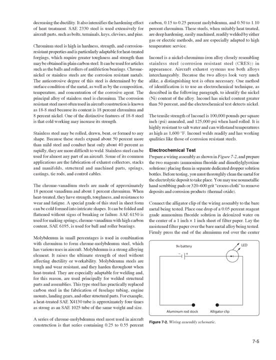 and prepare the two reagents, ammonium fluoride and dimethylglyoxime solutions, placing them in separate, dedicated dropper solution bottles. Before testing, you must thoroughly clean the metal. for the electrolytic deposit to take place, You may use non-metallic. 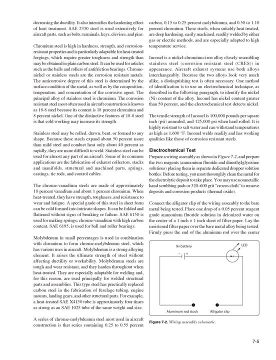 hand scrubbing pads or 320-600 grit crocus cloth to remove deposits and corrosion products. thermal oxide: Connect the alligator clip of the wiring assembly to the bare metal being tested. Place one drop of a 0.05% reagent-grade ammonium fluoride solution in 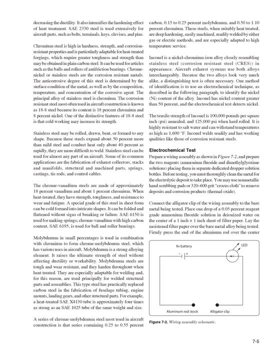 deionized water on the center of a 1-inch x 1-inch sheet of filter paper. Lay the moistened filter paper over the bare metal alloy being tested Firmly. press the end of the aluminum rod over the center of the moist paper. Maintain connection for 10 seconds while rocking the aluminum rod on. 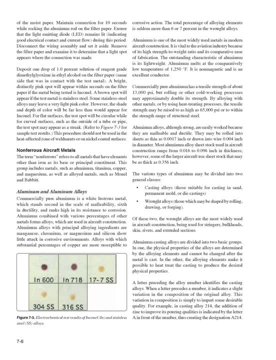 the filter paper. Ensure that the light-emitting diode LED remains lit, indicating good electrical contact and current flow. during this period, Disconnect the wiring assembly and set it aside. Remove the filter paper and examine it to determine that a light spot appears where. 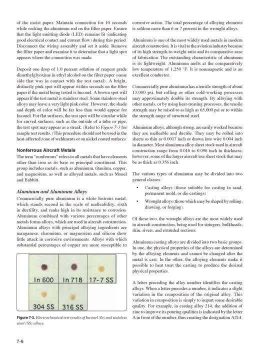 the connection was made. Deposit one drop of 1.0% solution of reagent-grade dimethylglyoxime and ethyl alcohol on the filter paper- same side that was in contact with the test metal. A bright, distinctly pink spot will appear within seconds on the filter paper. if the 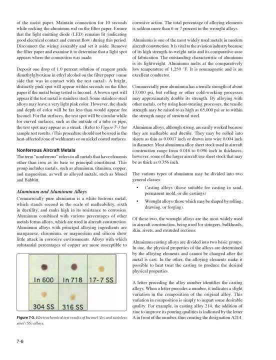 metal being tested is inconal, A brown spot will appear. if the test metal is stainless steel, Some stainless steel alloys may leave a very light pink color. However, the shade and depth of color will be far less than would appear for inconal. For flat surfaces, the test spot will 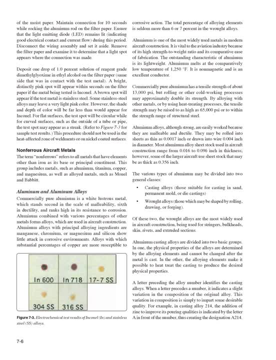 be circular, while for curved surfaces, such as the outside of a tube or pipe, the test spot may appear as a streak. Refer to figure 7-3 for sample test results. This procedure should not be used in the heat-affected zone of weldments or on nickel-coated surfaces. Non-ferrous aircraft metals. 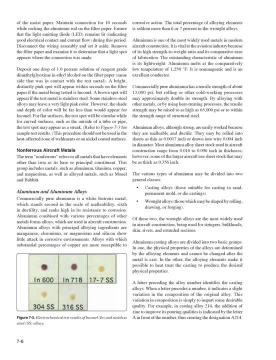 the term non-ferrous refers to all metal-based metal. Non-ferrous metals are made of non-ferrous metals that have elements other than iron as its base or principal constituent. This group includes metals such as aluminum, titanium, copper and magnesium, as well as alloyed metals such as: 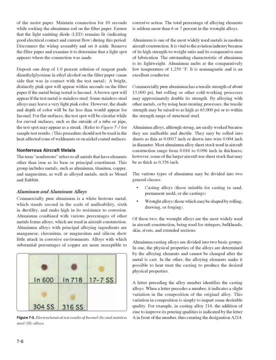 monol and babbitt, Aluminum and aluminum alloys. Commercially pure aluminum is a white, lustrous metal which stands second in the scale of malleability, sixth in ductility and ranks high in its resistance to corrosion. Aluminum combined with various percentages of other 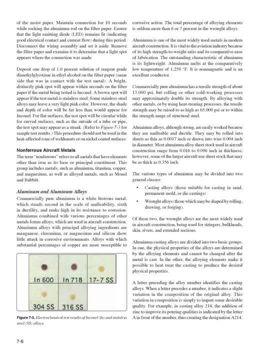 metals forms alloys which are used in aircraft. construction. alloys with principal alloying ingredients are manganese, chromium or magnesium and silicon show little attack in corrosive environments. Alloys with which substantial percentages of copper are more susceptible to corrosive action. The total percentage of alloying elements is 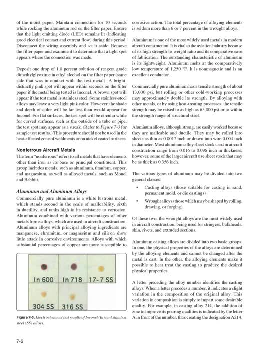 seldom more than 6 or 7% in the wrought alloys. Aluminum is one of the most widely used metals in modern aircraft construction. It is vital to the aviation industry because of its high strength-to-weight ratio and its comparative ease of fabrication. The outstanding characteristic of 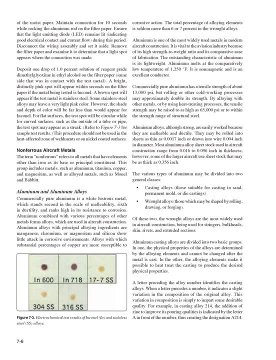 aluminum is its lightweight. Aluminum melts at the comparatively low temperature of 1250 degree Fahrenheit. It is non-magnetic and is an excellent conductor. Commercially pure aluminum has a tensile strength of about 13,000 psi, but rolling or other cold working processes may. 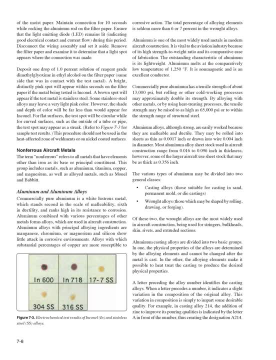 approximately double its strength. By alloying with other metals or by using heat-treating processes, the tensile strength may be raised. Aluminum alloys, although strong, are easily worked because they are malleable and ductile. They may be rolled into sheets as thin as 0.0017 inch or drawn into wire 0.004 inch in diameter. 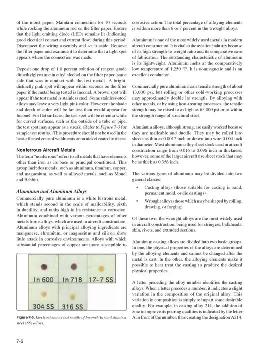 Most aluminum alloy sheet stock used in aircraft construction range from 0.016 to 0.096 inch in thickness. However, some of the larger aircraft use sheet stock that may be as thick as 0.356 inch. The various types of aluminum may be divided into two general classes. 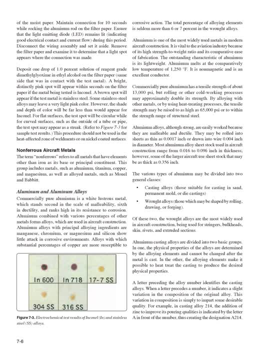 Casting alloys: those suitable for casting in sand, permanent mold or die castings. wrought alloys: those which may be shaped by rolling, drawing or forging. Of these two, the wrought alloys are the most widely used in aircraft construction, being used for stringers. 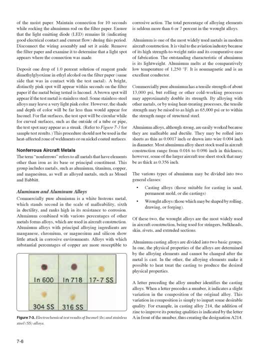 bulkheads, skin rivets and extruded sections. Aluminum casting alloys are divided into two basic groups. In one, the physical properties of the alloys are determined by the alloying elements and cannot be changed after the metal is cast. In the other, the alloying elements make it possible to heat. 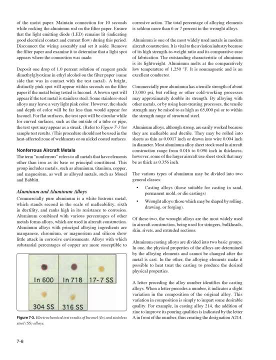 treat the casting to produce the desired physical properties. A letter preceding the alloy number identifies the casting alloys. When a letter precedes a number, it indicates a slight variation in the composition of the original alloy. This variation in composition is simply to impart some desirable quality, For example, in casting alloy 214,. 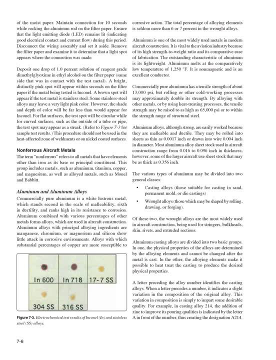 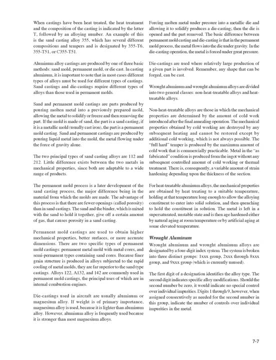 the addition of zinc to improve its pouring qualities is indicated by the letter A in front of the number, thus creating the designation A214.. When castings have been heat treated, the heat treatment and the composition of the casting is indicated by the letter T. 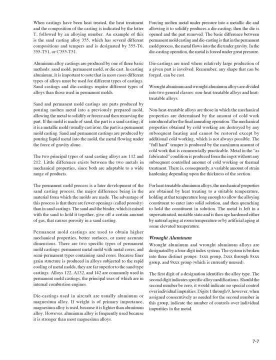 followed by an alloying number. An example of this is the sand casting alloy 355,, which has several different compositions and tempers and is designated by 355T6,, 355T51, or C355T51.. Aluminum alloy castings are produced by one of three basic methods: sand mold, permanent mold. 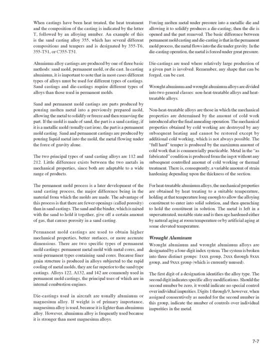 or die cast In casting aluminum. it is important to note that in most cases, different types of alloys must be used for different types of castings. Sand castings and die castings require different types of alloys than those used in permanent molds, Sand and permanent mold castings. 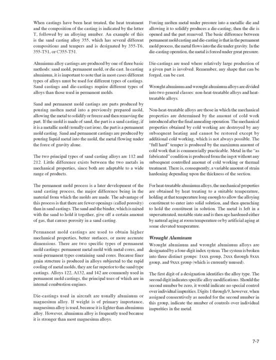 are parts produced by pouring molten metal into a previously prepared mold, allowing the metal to solidify or freeze and then removing the part. If the mold is made of sand, the castings are: the part is a sand casting. if it is a metallic mold, usually cast iron, the part is a permanent. 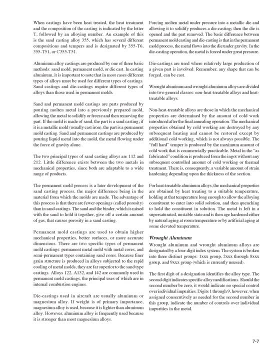 mold casting. Sand and permanent castings are produced by pouring liquid metal into the mold, the metal flowing under the force of gravity alone. The two principal types of sand casting alloys are 112 and 212.. Little difference exists between the two metals in mechanical properties. 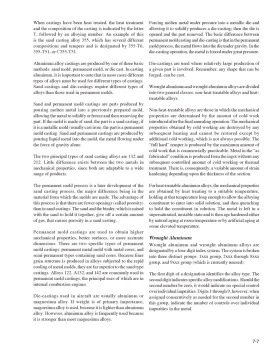 since both are adaptable to a wide range of products. The permanent mold process is a later development of the sand casting process. The advantage of this process is that there are fewer openings, called porosity, than in sand castings. The sand in the binder, which is mixed with the sand to hold it together, give off a 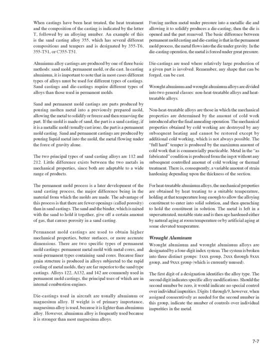 certain amount of gas that causes porosity in a sand casting. Permanent mold castings are used to obtain higher mechanical properties, better surfaces or more accurate dimensions. There are two specific types of permanent mold castings: permanent metal mold with metal cores and. 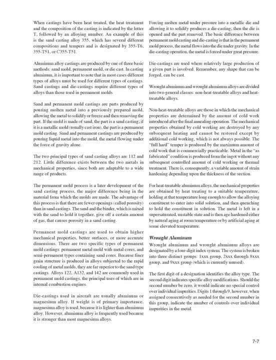 semi-permanent types containing sand cores. Because finer grain structure is produced in alloy subjected to the rapid cooling of metal molds, they are far superior to the sand type castings. Alloys 122,, A132, and 142 are commonly used in permanent mold castings, the principal 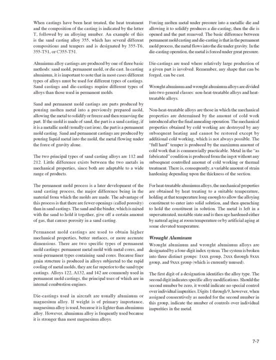 uses of which are in internal combustion engines. Die castings used in aircraft are usually aluminum or magnesium alloy. If weight is of primary importance, magnesium alloy is used because it is lighter than aluminum. However, aluminum alloy is frequently used because it is stronger than most magnesium alloys. 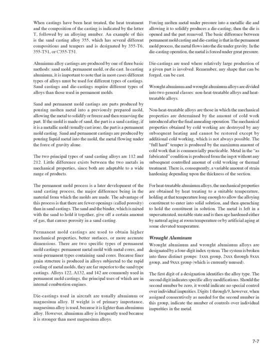 Forcing molten metal under pressure into a metallic die and allowing it to solidify produces a die casting. then the die is opened and the part removed. The basic difference between permanent mold casting and die casting is that in the permanent mold process the metal flows. 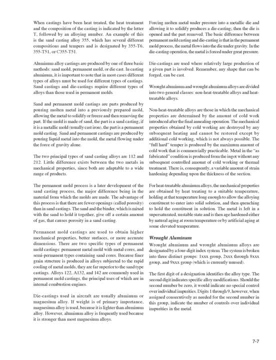 into the die under gravity. In the die casting operation, the metal is forced under great pressure. Die castings are used where relatively large production is needed. Remember, any shape that can be forged can be cast. Rot aluminum and rot aluminum alloys are divided into two general classes: non-heat treatable. 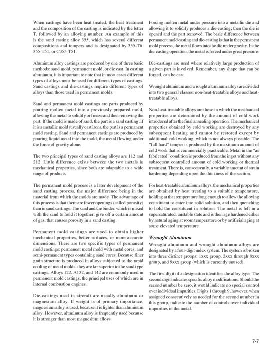 alloys and heat treatable alloys. Non-heat treatable alloys are those in which the mechanical properties are determined by the amount of cold work introduced after the final annealing operation. The mechanical properties obtained by cold working are destroyed by any subsequent heating and cannot be restored except by additional cold working, which is not always possible. 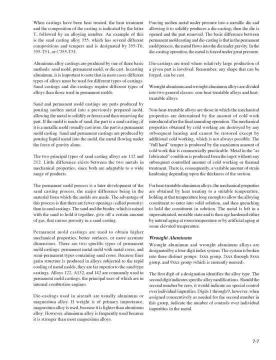 The full hard temper is produced by the maximum amount of cold work that is commercially practicable. Metal in the as-fabricated condition is produced from the ingot without any subsequent controlled amount of cold working or thermal treatment. There is consequently a variable. 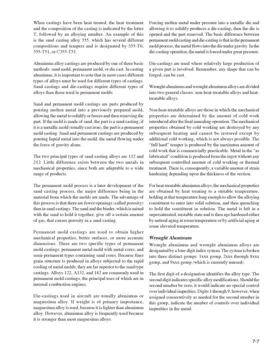 amount of strain hardening, depending upon the thickness of the section. For heat treatable aluminum alloys, the mechanical properties are obtained by heat treating to a suitable temperature, holding at that temperature long enough to allow the alloying constituent to enter into solid solution. 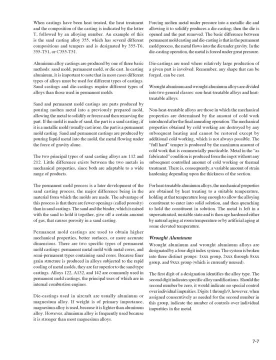 Quenching to hold the constituent in solution. The metal is left in a supersaturated, unstable state and is then age-hardened either by natural aging at room temperature or by artificial aging at some elevated temperature. Rot aluminum: rot aluminum and rot aluminum alloys are designated by a four-digit index. 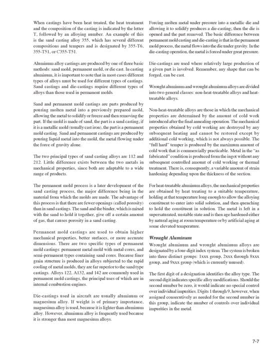 system. The system is broken into three distinct groups: one triple-X group, two triple-X through a triple-X group and nine triple-X group which is currently unused. The first digit of a designation identifies the alloy type. The second digit indicates specific alloy modifications, Should the second number be zero. 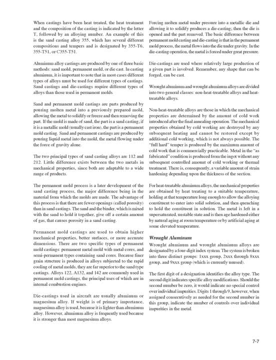 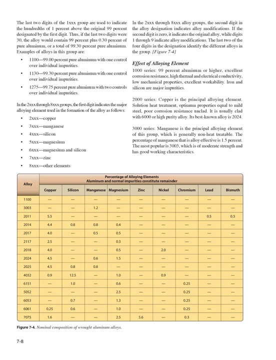 it would indicate no special control over individual impurities. Digits one through nine, however, when assigned consecutively as needed for the second number in this group, indicate the number of controls over individual impurities in the metal. The last two digits of the one triple-X group are used to indicate the hundreds of one percent. 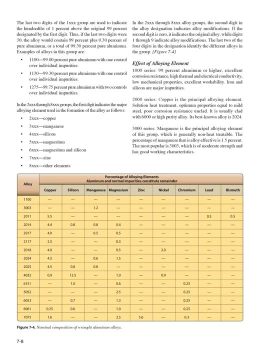 above the original 99 percent designated by the first digit. Thus, if the last two digits were 30,, the alloy would contain 99% plus 0.30% of pure aluminum, or a total of 99.30% pure aluminum. 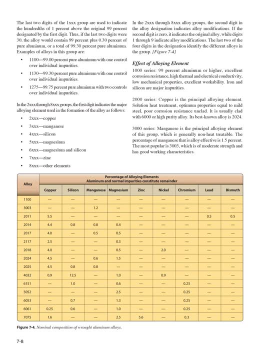 Examples of alloys in this group are: 1,100, 99.00% pure aluminum with one control over individual impurities. 1,130, 99.30% pure aluminum with one control over individual impurities. 1,275, 99.75% pure aluminum with two controls. 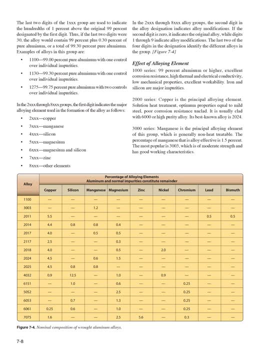 over individual impurities In the 2XXX through 8XXX groups. the first digit indicates the major alloying element used in the formation of the alloy, as follows: 2XXX copper, 3XXX manganese, 4XXX silicon, 5XXX magnesium, 6XXX magnesium and silicon, 7XXX zinc. 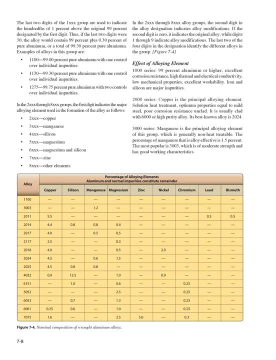 8XXX and zinc In the 2XXX through 8XXX alloy groups. the second digit in the alloy designation indicates alloy modifications. If the second digit is 0, it indicates the original alloy, while digits 1 through 9 indicate alloy modifications. The last two of the four digits in the designation identify: 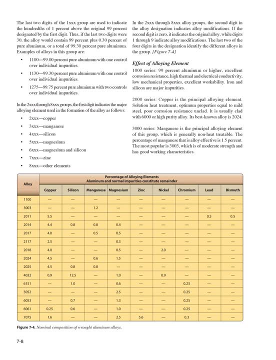 the different alloys in the group. Figure 7-4, effect of alloying element 1000 series, 99% aluminum or higher. excellent corrosion resistance. high thermal and electrical conduct resistance. high thermal and electrical conduct resistance. and high thermal and electrical 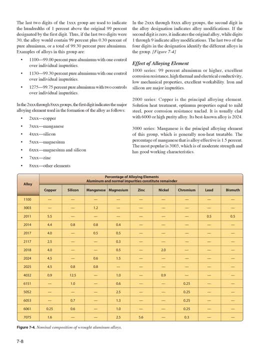 conductivity. low mechanical properties, excellent workability. Iron and silicon are major impurities 2000 series. copper is the principal alloying element: Solution: heat treatment, optimum properties equal to mild steel, poor corrosion resistance. unclad It is usually 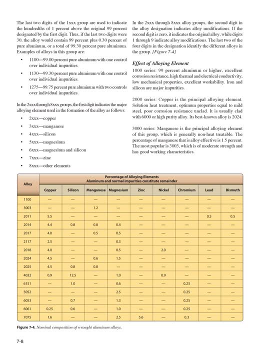 clad with 6000 or high purity alloy. Its best known alloy is 2024.. 3000 series manganese is the principal alloying element of this group, which is generally non-heat treatable. The percentage of manganese that is alloy effective is 1.5%. The most popular is 3003, which is of 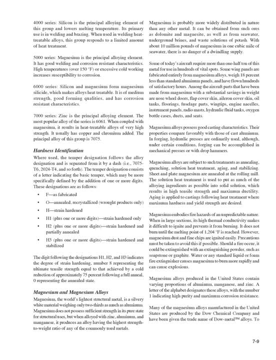 moderate strength and has good working characteristics. 4000 series silicon is the principal alloying element of this group and lowers melting temperature. Its primary use is in welding and brazing. When used in welding heat treatable alloys, this group responds to a limited amount. 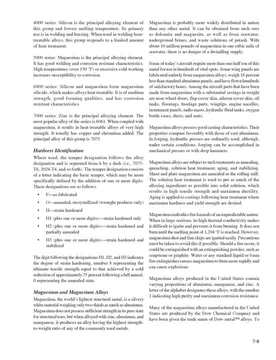 of heat treatment. 5000 series: magnesium is the principal alloying element. It has good welding and corrosion resistant characteristics. High temperatures over 150 degrees Fahrenheit or excessive cold working increases susceptibility to corrosion. 6000 series: silicon and magnesium. 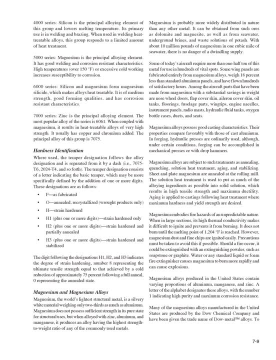 form magnesium silicide, which makes alloys heat treatable. It is of medium strength, good forming qualities and has corrosion resistant characteristics. 7000 series zinc is the principal alloying element. The most popular alloy of the series is 6061.. 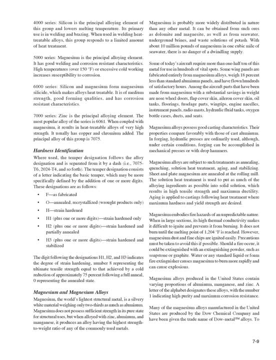 When coupled with magnesium, it results in heat treatable alloys of very high strength. It usually has copper and chromium added. The principal alloy of this group is 7075.. Hardness identification: where used. the temper designation follows the alloy designation and is separated from it by a dash. ie 7075, T6,, 2024, T4, and so forth. The temper designation. 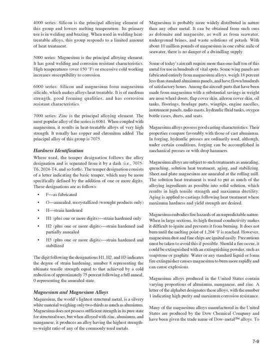 consists of a letter indicating the basic temper, which may be more specifically defined by the addition of one or more digits. These designations are as follows: F as fabricated. O. annealed recrystallized raw products only H- strain hardened H1,. 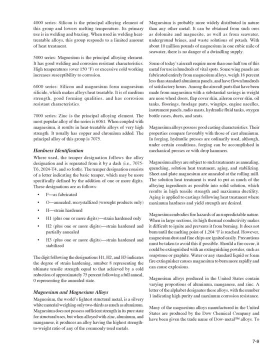 plus one or more digits strain hardened only. H2, plus one or more digits strain hardened and partially annealed: H3, plus one or more digits strain hardened and stabilize the digit following the designations H1,, H2, and H3 indicates the degree of strain hardening. 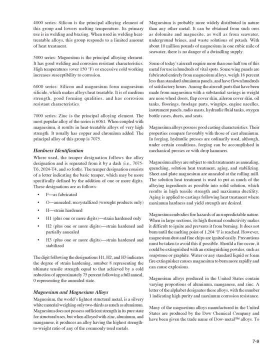 Number 8, representing the ultimate tensile strength equal to that achieved by a cold reduction of approximately 75% following a full. anneal 0, representing the annealed state. Magnesium and magnesium alloys. Magnesium, the world's lightest structural metal. 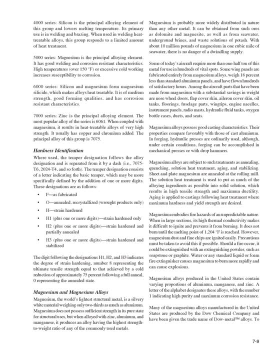 is a silvery-white material weighing only two-thirds as much as aluminum. Magnesium does not possess sufficient strength in its pure state for structural uses, but when alloyed with zinc, aluminum and manganese, it produces an alloy having the highest strength-to-weight ratio of any of the commonly used materials. 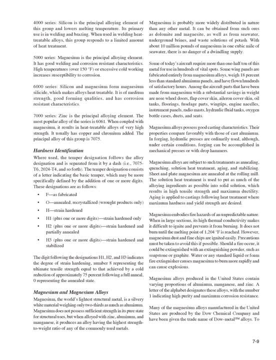 Magnesium is probably more widely distributed in nature than any other metal. It can be obtained from such ores as dolomite and magnesite, as well as from seawater, underground brines and waste solutions of potash, With about 10 million pounds of magnesium in one. 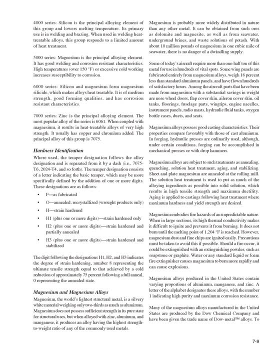 cubic mile of seawater. there is no danger of a dwindling supply. Some of today's aircraft require more than one-half ton of this metal for use in hundreds of vital spots. Some wing panels are fabricated entirely from magnesium alloys- 18% less than standard aluminum panels, and have flown hundreds of satisfactory hours. 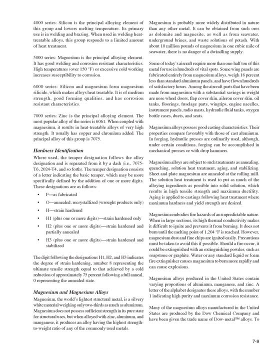 Among the aircraft parts that have been made from magnesium, with a substantial savings in weight, are nose-wheel doors, flap-cover skin, aileron-cover skin, oil tanks, floorings, fuselage parts, wingtips, engine nacelles, instrument panels, radio masts, hydraulic. 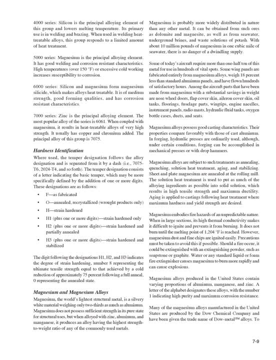 fluid tanks, oxygen bottle cases, ducts and seats. Magnesium alloys possess good casting characteristics. Their properties compare favorably to those of other metals, but are not as good as those of cast aluminum. In forging, hydraulic presses are ordinarily used, although under 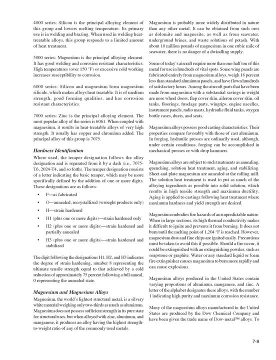 certain conditions, forging can be accomplished in mechanical presses or with drop hammers. Magnesium alloys are subject to such treatments as annealing, quenching solution, heat treatment, aging and stabilizing. Sheet and plate magnesium are annealed at the rolling mill. 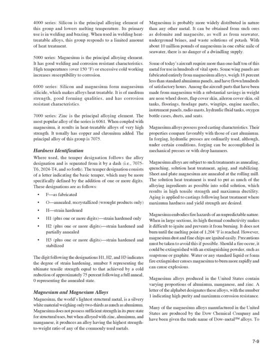 The solution. heat treatment is used to put as much of the alloying ingredients as possible into solid solution, which results in high tensile strength and maximum strength. Aging is applied to castings following heat treatment where maximum hardness and yield strength are desired. Magnesium embodies fire hazards of an unpredictable nature. 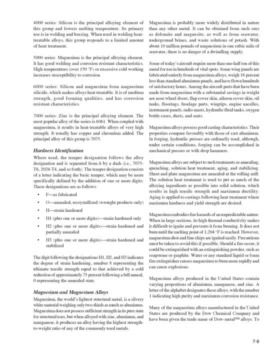 When, in large sections, its high thermal conductivity makes it difficult to ignite and prevents it from burning. It does not burn until the melting point of 1204 degrees Fahrenheit is reached. However, magnesium dust and fine chips are ignited easily. Precautions must be. 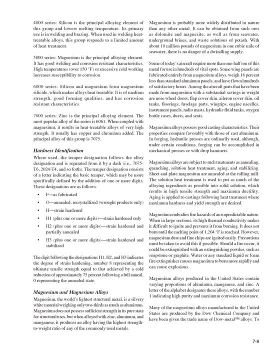 taken to avoid this if possible. Should a fire occur, it could be extinguished with an extinguishing powder such as soapstone or graphite, Water or any standard liquid or foam. fire extinguisher causes magnesium to burn more rapidly and can cause explosions. Magnesium alloys produced in the United States contain 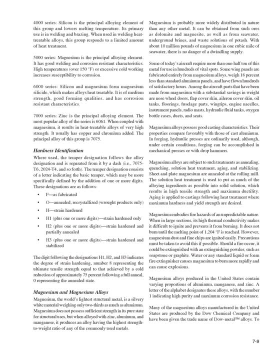 varying proportions of aluminum, manganese and zinc. A letter of the alphabet designates these alloys, with the number one indicating high purity and maximum corrosion resistance. Many of the magnesium alloys manufactured in the United States are produced by the Dow Chemical Company and have been given the trade name of Dow Metal Alloys. 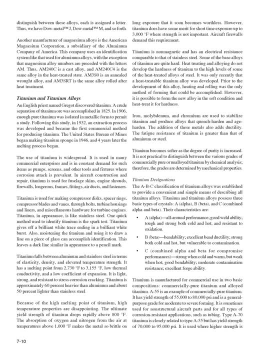 2. Distinguished. between these alloys, each is assigned a letter. Thus we have Dow Metal J, Dow Metal M, and so forth. Another manufacturer of magnesium alloys is the American Magnesium Corporation, a subsidiary of the Aluminum Company of America. This company uses an 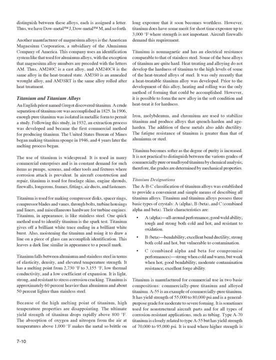 identification system like that used for aluminum alloys, with the exception that magnesium alloy numbers are preceded with the letter J 2.. Distinguished between these alloys, each is assigned a letter. Thus we have Dow Metal J, Dow Metal M and so forth. Another manufacturer of magnesium alloys, whichenza, features a. 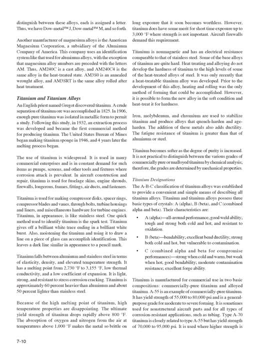 letterimi is assigned a letter J. Thus, AM240C is a cast alloy and AM240C4 is the same alloy in the heat-treated state. AM3S0 is an annealed raw alloy and a mesert is the same alloy rolled after heat treatment. 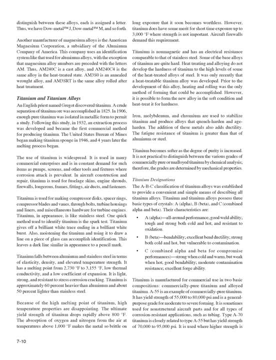 Titanium and titanium alloys. an English priest named Griggett discovered titanium. A crude separation of titanium ore was accomplished in 1825. In 1906, enough pure titanium was isolated in metallic form to permit a study Following its creation. there was a study in the University of Chicago where a study was conducted to check the titanium alloy was 버ntable met혔ic. 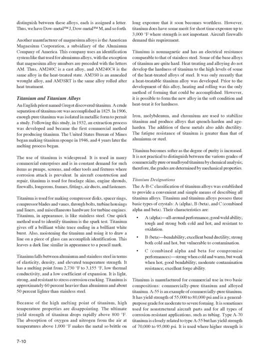 Following this study, in 1932, an extraction process was developed and became the first commercial method for producing titanium. The United States Bureau of Mines began making titanium sponge in 1946, and four years later the melting process began. The use of titanium is widespread. 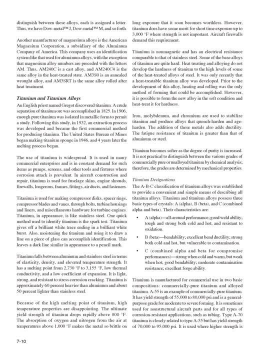 It is used in many commercial enterprises and is in constant demand for such items as pumps, screens and other tools and fixtures where corrosion attack is prevalent. In aircraft construction and repair. titanium is used for fuselage skins, engine shrouds, firewalls, long-arons, frames, fittings, air ducts and fasteners. 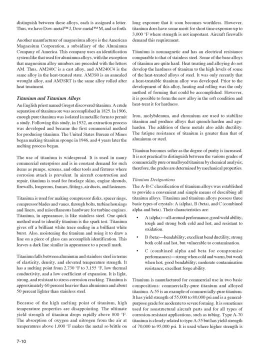 Titanium is used for making compressor discs, spacer rings, compressor blades and vanes through bolts, turbine housings and liners and miscellaneous hardware for turbine engines. Titanium in appearance is like stainless steel. One quick method used to identify titanium is the spark test. 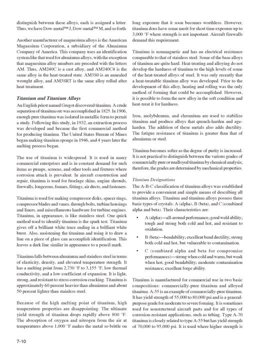 Titanium gives off a brilliant white trace, The trace ending in a brilliant white burst. Also, moistening the titanium and using it to draw a line on a piece of glass can accomplish identification. This leaves a dark line similar in appearance to a pencil mark. Titanium falls between aluminum and stainless steel in terms of elasticity, density and elevated temperature strength. It has a melting point from 2,730 degrees Fahrenheit to 3,155 degrees Fahrenheit, low thermal conductivity and a low coefficient of expansion. It is light, strong and resistant to stress, corrosion, cracking. 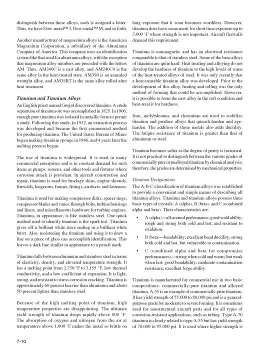 Titanium is approximately 60 percent heavier than aluminum and about 50 percent lighter than stainless steel. Because of the high melting point of titanium, high temperature properties are disappointing. The ultimate yield strength of titanium drops rapidly above 800 degree Fahrenheit. The absorption of oxygen and nitrogen from the air at temperatures above 1,000 degrees. 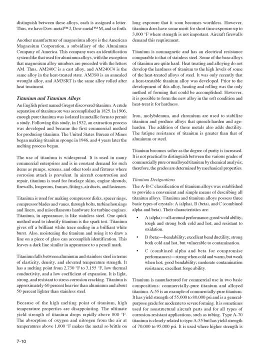 Fahrenheit makes the metal so brittle on long exposure that it soon becomes worthless. However, titanium is a very strong material. Titanium does have some merit for short-time exposure up to 3,000 degrees Fahrenheit, where strength is not important. Aircraft firewalls demand this requirement. 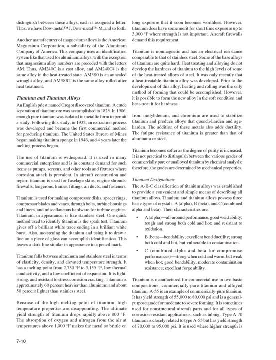 Titanium is non-magnetic and has an electrical resistance comparable to that of stainless steel. Some of the base alloys of titanium are quite hard. Heat treating and alloying do not develop the hardness of titanium to the high levels of some of the heat-treated alloys of steel. It was only recently that a heat-treatable titanium alloy was developed. Prior to the development of this alloy, heating and rolling was the only method of forming that could be accomplished. However, it is possible to form the new alloy in the soft condition and heat treat it for. 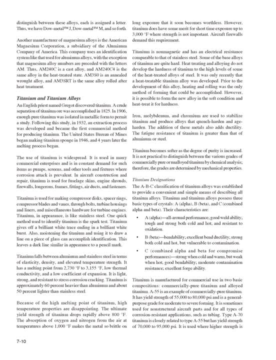 hardness. Iron, molybdenum and chromium are used to stabilize titanium and produce alloys that quench harden and age harden. The addition of these metals also adds ductility. The fatigue resistance of titanium is greater than that of aluminum or steel. 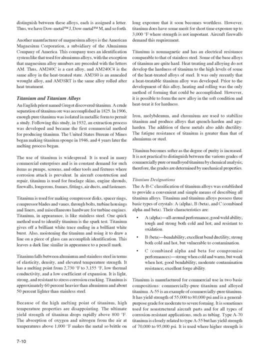 Titanium becomes softer as the degree of purity is increased. It is not practical to distinguish between the various grades of commercially pure or unalloyed titanium by chemical analysis. therefore, the grades are determined by mechanical properties. Titanium designations- The ABC classification of titanium alloys was established to provide a convenient and 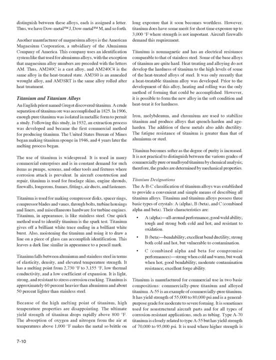 simple means of describing all titanium alloys. Titanium and titanium alloys possess three basic types of crystals: A-alpha, B-beta and C combined alpha and beta. Their characteristics are A-alpha, all-round performance, good weldability, tough and strong, both cold and 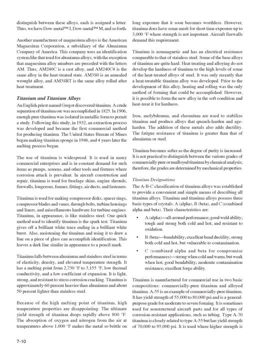 hot and resistant to oxidation. B-beta bendability. excellent bend ductility. strong both cold and hot, but vulnerable to contamination. C combined alpha and beta for compromise performances: strong when cold and warm, but weak when hot. good bendability. 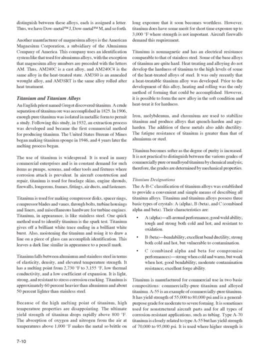 moderate contamination resistance. excellent forgeability. Titanium is manufactured for commercial use in two bases. A-55 is an example of commercially pure titanium. It has yield strength of 55,000 to 80,000 pounds per square inch and is a general purpose grade for moderate to severe forming. It is sometimes 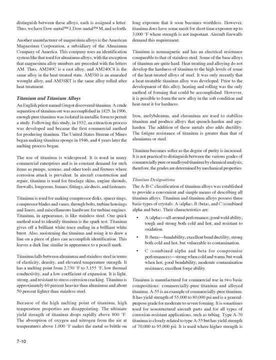 used for non-structural aircraft parts and for all types of corrosion-resistant applications such as tubing. Type A-70 titanium is closely related to type A-55, but has yield strength of 70,000 to 95,000 pounds per square inch. Titanium is used for non-structural aircraft parts and for 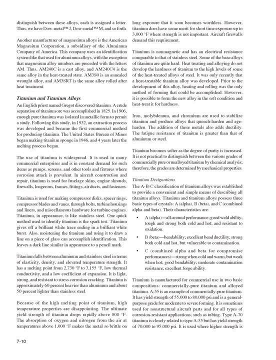 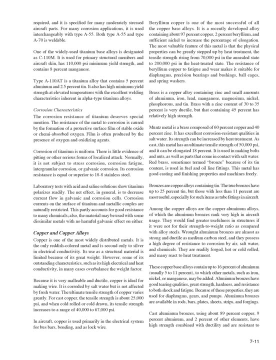 it is used where higher strength is required and it is specified for many moderately stressed aircraft parts. For many corrosion applications it is used interchangeably with type A-55.. Both type A-55 and type A-70 is weldable. One of the widely used titanium base alloys is designated. 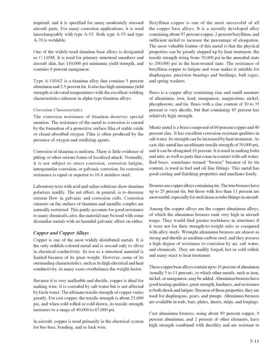 as C-110M. It is used for primary structural members and aircraft skin, has 110,000 pounds per square inch minimum yield strength and contains 8% maximum yield strength. Type A-110It is a titanium alloy that contains 5% aluminum and 2.5% tin. It also has high minimum. 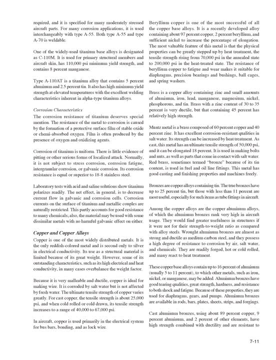 yield strength at elevated temperatures with the excellent welding characteristics inherent in alpha-type titanium alloys. Corrosion characteristicsThe corrosion resistance of titanium deserves special mention. The resistance of the metal to corrosion is caused by the formation of a protective surface film of stable oxide or chemi-absorbed oxygen Film is often 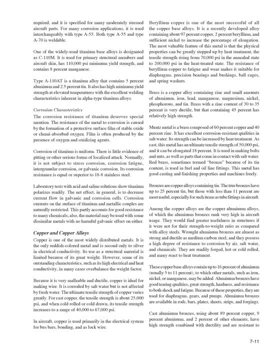 produced by the presence of oxygen and oxygen gas. The corrosion resistance of the metal is caused by oxidizing agents. Corrosion of titanium is uniform. There is little evidence of pitting or other serious forms of localized attack. Normally it is not subject to stress corrosion- corrosion. 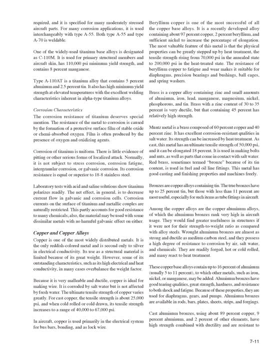 fatigue, intergranular corrosion or galvanic corrosion. Its corrosion resistance is equal or superior to 18-to-8 stainless steel. Laboratory tests with acid and saline solutions show titanium polarizes readily. The net effect in general is to decrease current flow in galvanic and 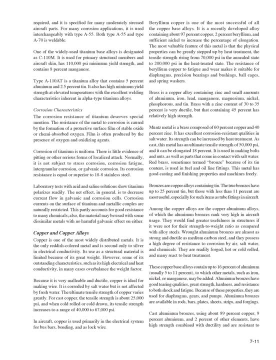 corrosion systems. Corrosion currents on the surface of titanium and metallic couples are naturally restricted. This partly accounts for good resistance to many chemicals. Also, the material may be used with some dissimilar metals with no harmful galvanic effect on either Copper and copper alloys. 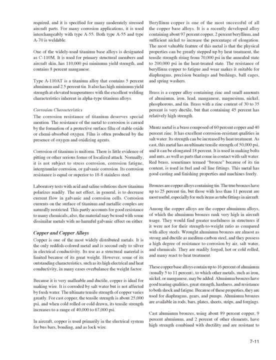 Copper is one of the most widely distributed metals. It is the only reddish-colored metal and it's second only to silver and electrical conductivity. Its use as a structural material is limited because of its great weight. However, some of its outside effects are not so great. 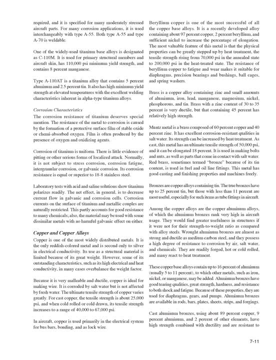 Copper has outstanding characteristics such as its high electrical and heat conductivity. in many cases overbalance the weight factor. Because it is very malleable and ductile, copper is ideal for making wire. It is corroded by salt water but is not affected by fresh water. 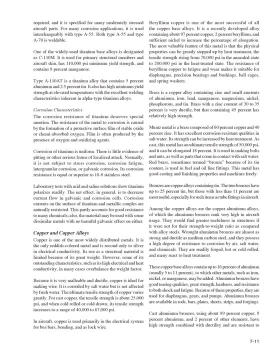 The ultimate tensile strength of copper varies greatly. For cast copper, the tensile strength is about 25,000 pounds per square inch, and when cold rolled or cold drawn its tensile strength increases to a range of 40,000 to 67,000 pounds per inch. Copper is a very strong metal. Copper is 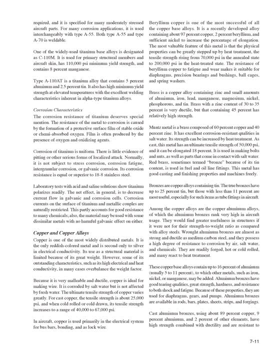 used primarily in the electrical system, for bus bars, bonding and as lock wire. Beryllium copper is one of the most successful of all the copper base alloys. It is a recently developed alloy containing about 97% copper, 2% beryllium and sufficient nickel to increase the percentage. 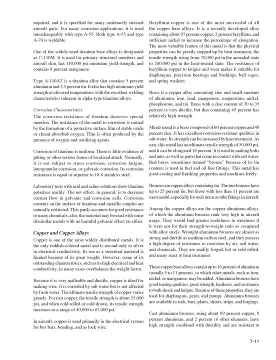 of elongation. The most valuable feature of this metal is that the physical properties can be greatly stepped up by heat treatment, the tensile strength rising from 70,000 pounds per square inch in the annealing process. Copper is used primarily in the electrical system for bus bars, bonding. 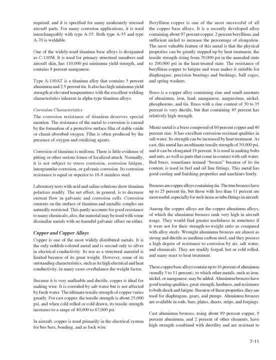 shield state to 200,000 psi in the heat treated state. The resistance of beryllium copper to fatigue and wear makes it suitable for diaphragms, precision bearings and bushings, ball cages and spring washers. Brass is a copper alloy containing zinc and small amounts of aluminum. 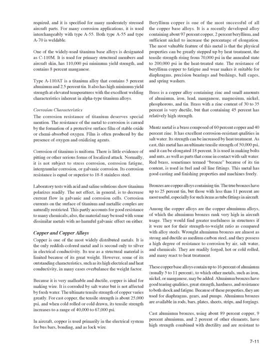 iron, lead, manganese, magnesium, nickel, phosphorus and tin. Brass with a zinc content of 30 to 35% is very ductile, but that containing 45% has relatively high strength. Muntz metal is a brass composed of 60%. 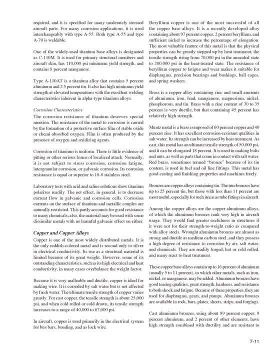 copper and 40% zinc. It has excellent corrosion-resistant qualities in salt water. Its strength can be increased by heat treatment. As cast, this metal has an ultimate tensile strength of 50,000 pounds per square inch and it can be elongated 18%. It is used in making 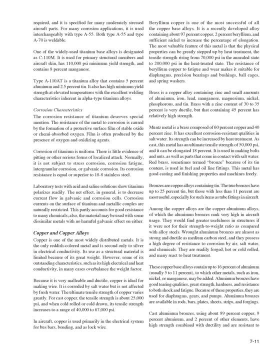 bolts and nuts, as well as parts that come in contact with salt water. Red brass, sometimes termed bronze because of its tin content, is used in fuel and oil line fittings. This metal has good casting and finishing performance. It is used in making bolts and nuts, as well as parts that come 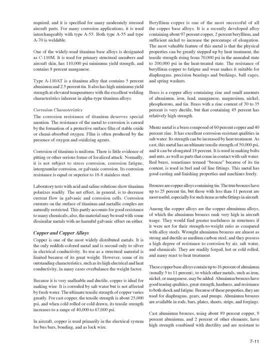 in contact with salt water. It has excellent corrosion-resistant properties and machines freely. Bronzes are copper alloys containing tin. The true bronzes have up to 25% tin, but those with less than 11% are most useful, especially for such items as tube fittings in. 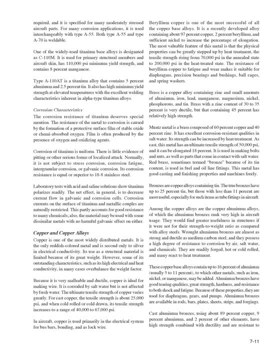 aircraft. Among the copper alloys are the copper-aluminum alloys, of which the aluminum bronzes rank very high in aircraft usage. They would find greater usefulness in structures if it were not for their strength-to-weight ratio as compared with alloy steels. 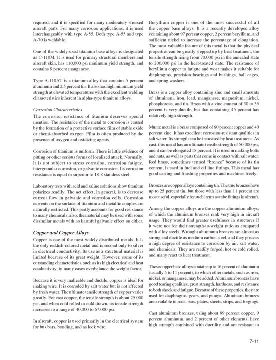 Rod aluminum bronzes are almost as strong and ductile as medium-carbon steel and they possess a high degree of resistance to corrosion by air, salt water and chemicals. They are readily forged, hot or cold-rolled and many react to. 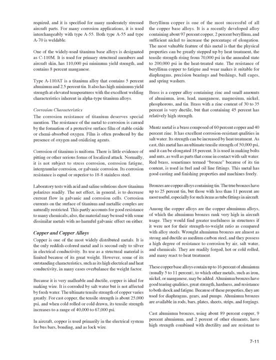 heat treatment. These copper-base alloys contain up to 16% of aluminum, usually 5-11%, to which other metals such as iron, nickel or manganese may be added. Aluminum bronzes have good tearing qualities, great strength, hardness and resistance to both shock and fatigue. Because of these, 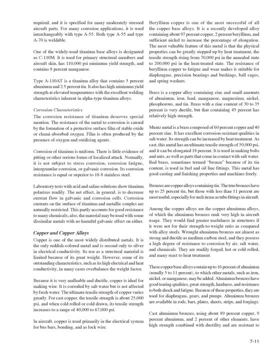 properties. they are used in making bolts and nuts, as well as for such items as tube fittings. in the air They are used for diaphragms, gears and pumps. Aluminum bronzes are available in rods, bars, plates, sheets, strips and forgings. Cast aluminum bronzes using about 89% copper. 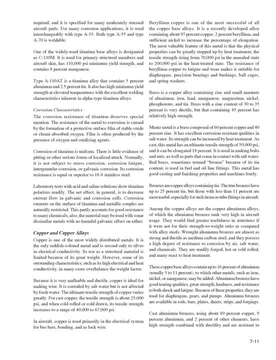 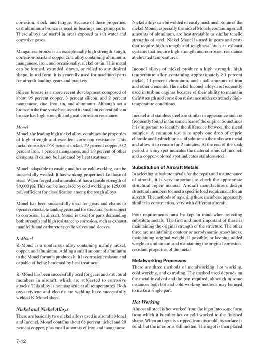 9% aluminum and 2% of other elements. have high strength combined with ductility, and are resistant to corrosion, shock and fatigue. Because of these properties, cast aluminum bronze is used in bearings and pump parts. These alloys are useful in areas exposed to salt water. 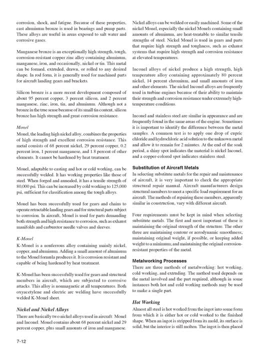 and corrosive gas. They are used in making bolts and nuts, as well as for such items as tube fittings and brasses. Manganese bronze is an exceptionally high-strength, tough, corrosion-resistant copper, zinc alloy containing aluminum, manganese, iron and, occasionally, nickel or tin. This metal can 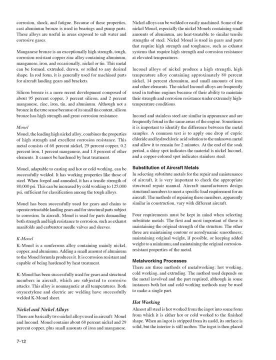 be formed, extruded, drawn or rolled to any desired shape In rod form. it is generally used for machined parts for aircraft, landing gears and brackets. Silicon bronze is a more recent development, composed of about 95% copper, 3% silicon and 2% manganese, zinc, iron, tin and 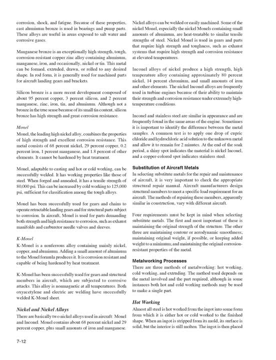 aluminum. Although not a bronze in the true sense because of its small tin content, silicon bronze has high strength and great corrosion resistance. Monol- monol, the leading high nickel alloy, combines the properties of high strength and excellent corrosion resistance. This metal 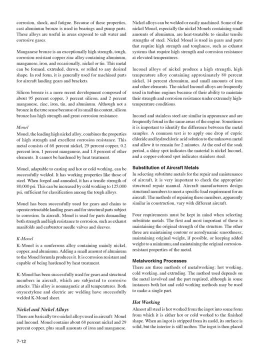 consists of 68% nickel, 29% copper, 0.2% iron, 1% manganese and 1.8% of other elements. It cannot be hardened by heat treatment. Monol adaptable to casting in hot or 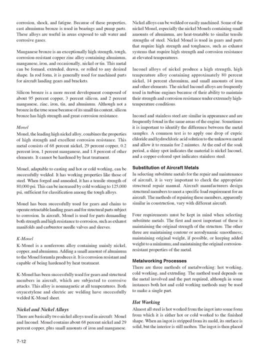 cold working can be successfully welded. It has working properties like those of steel. When forged and annealed it has a tensile strength of 80,000 pounds per square inch. This can be increased by cold working to 125,000 psi, sufficient for classification among the tough. 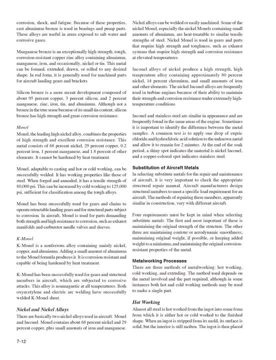 alloys. Monol has been successfully used for gears and chains to operate retractable landing gears and for structural parts subject to corrosion. In aircraft, monol is used for parts demanding both strength and high resistance to corrosion, such as exhaust manifolds and carburetor needle valves and sleeves. 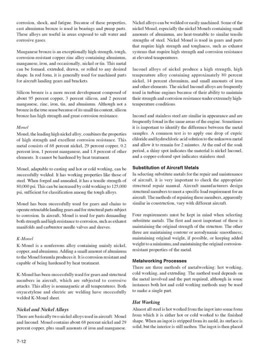 K-Model. K-Model is a non-ferrous alloy containing mainly nickel, copper and aluminum. Adding a small amount of aluminum to the monol formula produces it. It is corrosion resistant and capable of being hardened by heat treatment. K-Model has been successfully used for gears and structural members in aircraft. 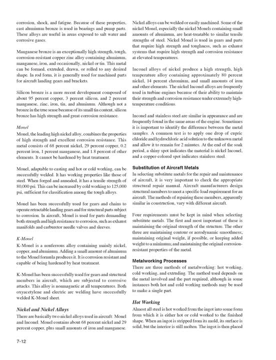 which are subjected to corrosive attacks. This alloy is non-magnetic at all temperatures. Both oxyacetylene and electric arc welding have successfully welded K-Model sheet Nickel and nickel alloys. There are basically two nickel alloys used in aircraft: monol and inconol. Monol contains about 68% nickel and 29% copper. plus small amounts of iron and manganese. Nickel alloys can be welded or easily machined. Some of the nickel monol, especially the nickel monols containing small amounts of aluminum, are heat treatable to similar tensile strengths of steel. Nickel monol is used in gears and parts that require high strength and toughness. 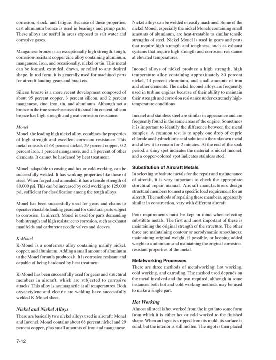 such as exhaust systems that require high strength and corrosion resistance at elevated temperatures. Inconol alloys of nickel produce a high-strength, high-temperature alloy containing approximately 80% nickel, 14% chromium and small amounts of iron and other elements. 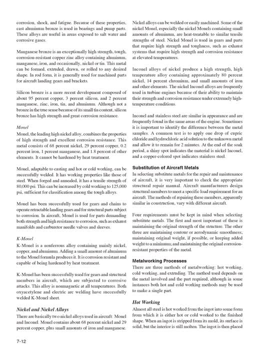 The nickel-inconol alloys are frequently used in turbine engines because of their ability to maintain their strength and corrosion resistance under extremely high temperature conditions. Inconol and stainless steel are similar in appearance and are frequently found in the same areas of the engine. Sometimes it is important to identify the difference between the metal. 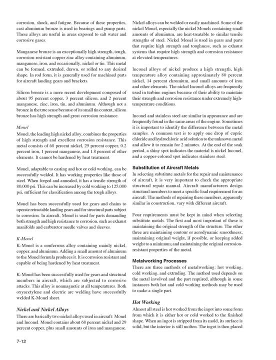 samples. A common test is to apply one drop of cupric chloride and hydrochloric acid solution to the unknown metal and allow it to remain for two minutes. At the end of the soak period, a shiny spot indicates the material is nickel-inconol, and a copper-colored spot. 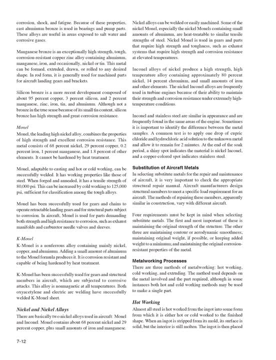 indicates stainless steel Substitution of aircraft metals. in selecting substitute metals for the repair and maintenance of aircraft, it is very important to check the appropriate structural repair manual. Aircraft manufacturers design structural members to meet a specific load requirement for an aircraft. The methods of repairing these members apparently similar. in construction vary with different aircraft. Four requirements must be kept in mind when selecting substitute metals. The first and most important of these is maintaining the original strength of the structure. The other three are maintaining contour or aerodynamic smoothness, maintaining original weight if possible, or keeping added weight to a minimum. 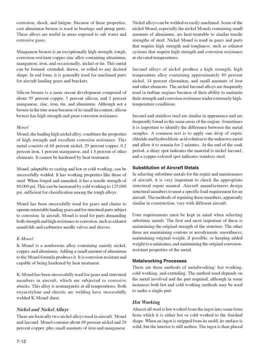 and maintaining the original corrosion-resistant properties of the metal Metalworking processes. There are three methods of metalworking: hotworking, coldworking and extruding. The method used depends on the metal involved and the part required, although in some instances both hot and coldworking methods may be used. 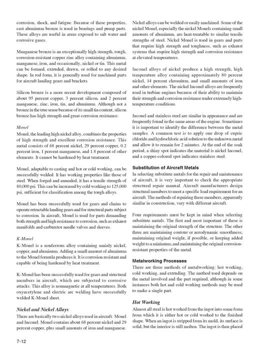 to make a single part: Hotworking. Almost all steel is hotworked from the ingot into some form, from which it is either hot or coldworked to the finished shape. The ingot is stripped from its mold, its surface is solid, but the interior is still molten. 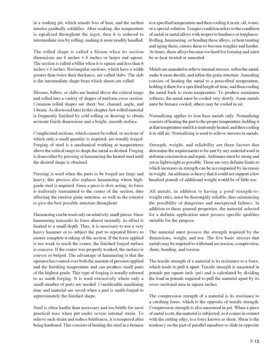 The ingot is then placed in a soaking pit, which retards loss of heat and the molten interior gradually solidifies. After soaking, the temperature is equalized throughout the ingot. then it is reduced to intermediate size by rolling, making it more. 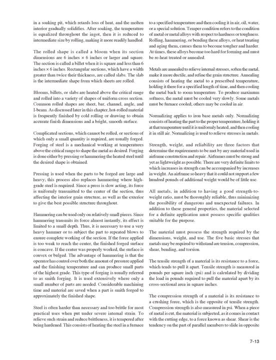 readily handled. The rolled shape is called a bloom when its section dimensions are 6 inches times 6 inches or larger, and square. The section is called a billet when it is square and less than 6 inches or larger. The section is called a billet when it is square and less than 6 inches or larger. 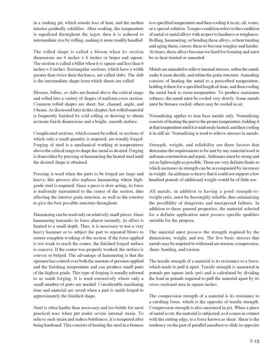 6 inches times 6 inches. Rectangular sections which have a width greater than twice their thickness are called slabs. The slab is the intermediate shape from which sheets are rolled. Blooms, billets or slabs are heated above the critical range and rolled into a variety of. 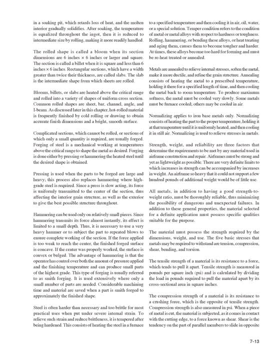 shapes of uniform cross-section. Common rolled shapes are sheet, bar, channel angle and I-beam, As discussed later in this chapter. hot-rolled material is frequently finished by cold rolling or drawing to obtain accurate finish dimensions and a bright. 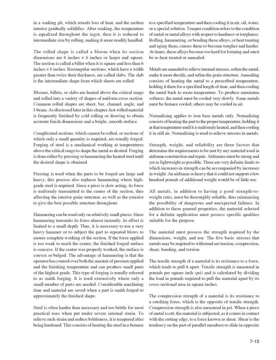 smooth surface. Complicated sections which cannot be rolled or sections of which only a small quantity is required are usually forged. Forging of steel is a mechanical working at temperatures above the critical range to shape the metal as desired. Forging is done either by: 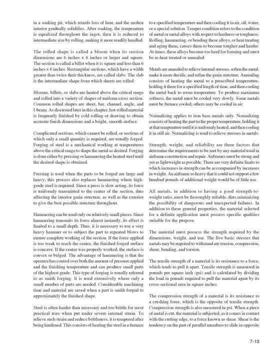 pressing or hammering the heated steel until the desired shape is obtained. Pressing is used when the parts to be forged are large and heavy. This process also replaces hammering, where high-grade steel is required. Since a press is slow-acting, it's forced to be forged when the parts are 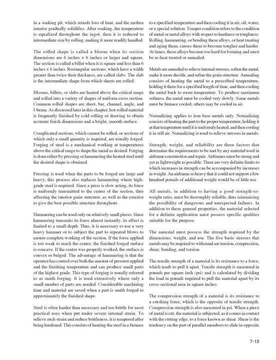 hammered, The force is uniformly transmitted to the center of the section, thus affecting the interior grain structure as well as the exterior. to give the best possible structure throughout, Hammering can be used only on relatively small pieces, Since hammering transmits its force. 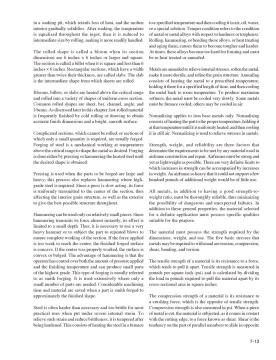 almost instantly. its effect is limited to a small depth. Thus, it is necessary to use a very heavy hammer or to subject the part to repeated blows to ensure complete working of the section. If the force applied is too weak to reach the center, the finished forged surface is concave. 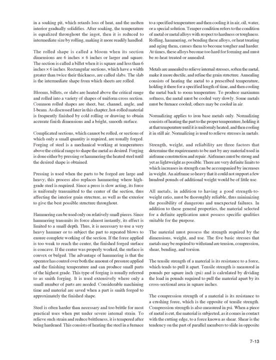 If the center was properly worked, the surface is convex or bulged. The advantage of hammering is that the operator has control over both the amount of pressure applied and the finishing temperature and can produce small parts of the highest grade. This type of forging is usually referred to as 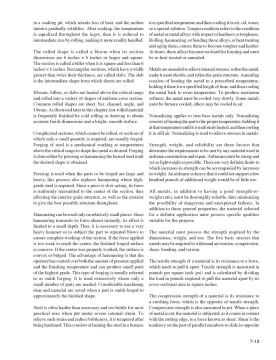 Smith forging. It is used extensively where only a small number of parts are needed. Considerable machining time and material are saved when a part is Smith forged to approximately the finished shape. Steel is often harder than necessary and too brittle for most of the practical uses when put under severe internal strain. To relieve such strain and reduce 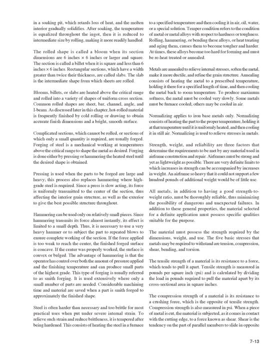 brittleness. it is tempered after being hardened. This consists of heating the steel in a furnace to a specified temperature and then cooling it in air, oil, water or a special solution. Temper condition refers to the condition of metal or metal alloys with respect to hardness or 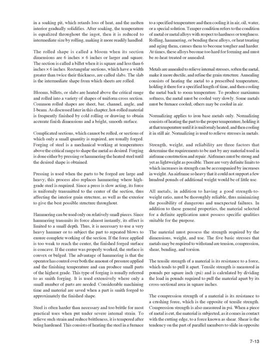 toughness. Rolling, hammering or bending these alloys or heat treating and aging them causes them to become tougher and harder. At times, alloys become too hard for forming and must be reheat treated or annealed. Metals are annealed to relieve internal stresses, soften the metal, make it more ductile. 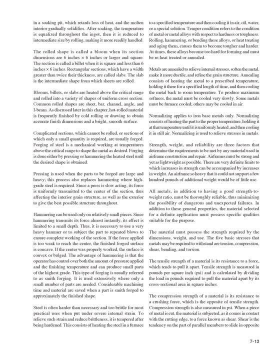 and refine the grain structure. Annealing consists of heating the metal to a prescribed temperature, holding it there for a specified length of time and then cooling the metal back to room temperature. To produce maximum softness, the metal must be cooled very slowly. 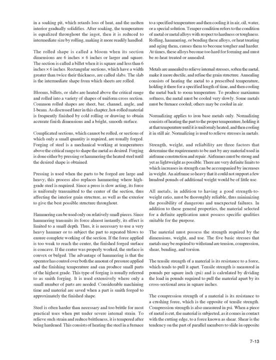 Some metals must be furnace cooled. others may be cooled in air. Normalizing applies to iron-based metals only. Normalizing consists of heating the part to the proper temperature, holding it at that temperature until it is uniformly heated, and then cooling it in still air. 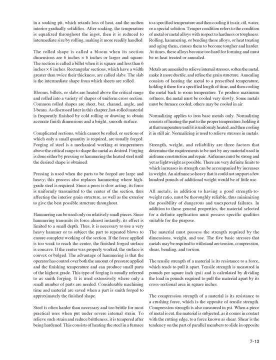 Normalizing is used to relieve stresses in metals. Strength, weight and reliability are three factors that determine the requirements to be met by any material used in airframe construction and repair. Airframes must be strong and yet as lightweight as possible. There are very definite limits to which increases in strength can be accompanied by increases in. 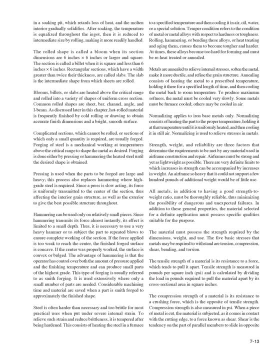 weight. If a metal is too heavy that it could not support a few hundred pounds of additional weight would be of little use. All metals, in addition to having a good strength-to-weight ratio, must be thoroughly reliable, thus minimizing the possibility of dangerous and unexpected failures. 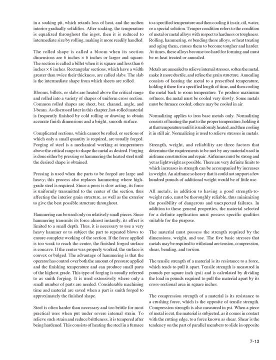 In addition to these general properties, the material selected for a definite application must possess specific quality suitable for the purpose. The material must possess the strength required by the dimensions, weight and use. The five basic stresses that metals may be required to withstand are tension. 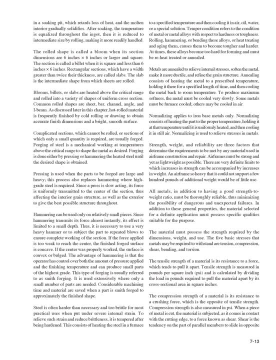 compression, shear, bending and torsion. The tensile strength of a material is its resistance to a force which tends to pull it apart. Tensile strength is measured in pounds per inch to psi and is calculated by dividing the load in pounds required to pull the material apart by. 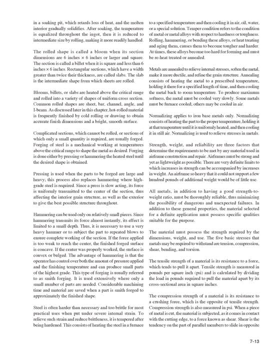 its cross-sectional area in square inches. The compression strength of a material is its resistance to a crushing force, which is the opposite of tensile strength. Compression strength is also measured in psi. When a piece of metal is cut, the material is subjected, as it comes in contact with a cutting edge, to a force known as shear. 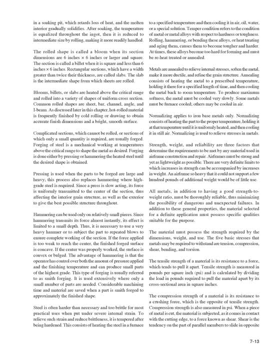 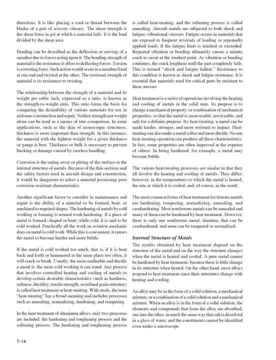 Shear is the tendency on the part of parallel members to slide in opposite directions. It is like placing a cord or thread between the blades of a pair of scissors. shears- The shear strength- is the shear force in psi at which a material fails. 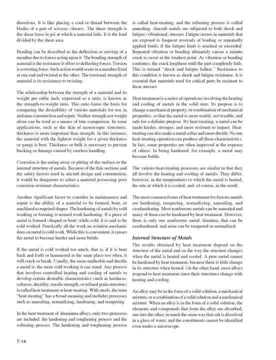 It is the load divided by the shear area. Bending can be described as the deflection or curving of a member due to forces acting upon it. The bending strength of material is the resistance it offers to deflecting forces. Torsion is a twisting force. Such action would occur in a member fixed at one. 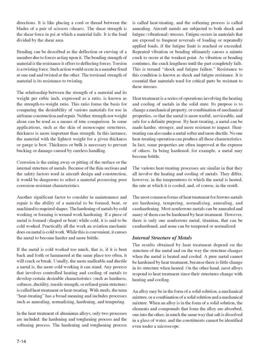 end and twisted at the other. The torsional strength of material is its resistance to twisting. The relationship between the strength of a material and its weight per cubic inch, expressed as a ratio, is known as the strength-to-weight ratio. This ratio forms the basis for comparing the desirability of various materials for use in 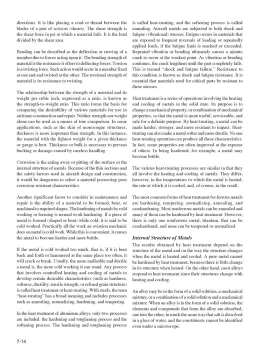 airframe construction and repair. Neither strength nor weight alone can be used as a means of true comparison. In some applications, such as the skin of monocoque structures, thickness is more important than strength. In this instance, the material with the lightest weight for a given 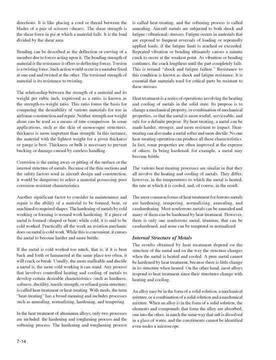 thickness or gauge is best. Thickness or bulk is necessary to prevent bucking or damage caused by careless handling. Corrosion is the eating away or pitting of the surface or the internal structure of metals Because of the thin sections and the safety factors used in aircraft design. 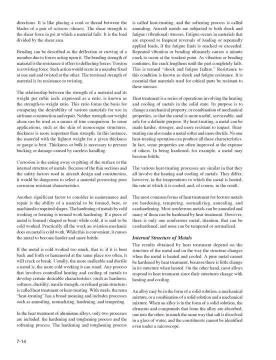 and construction, it would be dangerous to select a material possessing poor corrosion. In this case, the material with the lightest weight is the one with the least strength. Another significant factor to consider in maintenance and repair is the ability of a material to be formed, bent or machined to required shapes. The hardening of metals by 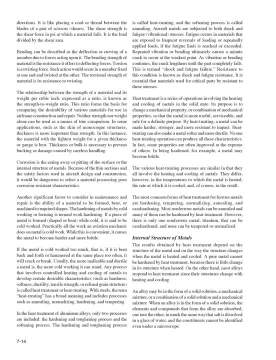 cold working or forming is termed work hardening. If a piece of metal is formed, shaped or bent while cold, it is said to be cold worked. Practically all the work an aviation mechanic does on metal is cold work. While this is convenient, it causes the metal to become 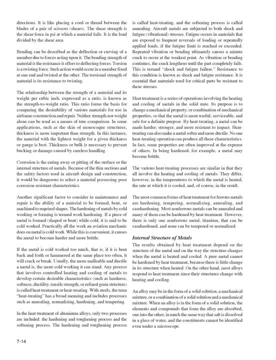 harder and more brittle. If the metal is cold worked too much, that is, if it is bent back and forth or hammered at the same place too often, it will crack or break. Usually, the more malleable and ductile a metal is. 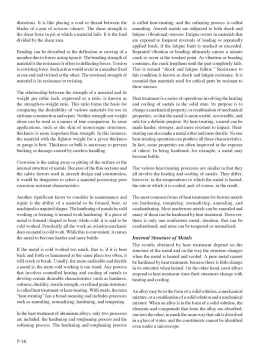 the more cold working it can stand. Any process that involves controlled heating and cooling of metals to develop certain desirable characteristics, such as hardness, softness, ductility, tensile strength or refined grain structure, is called heat treatment or heat treating. 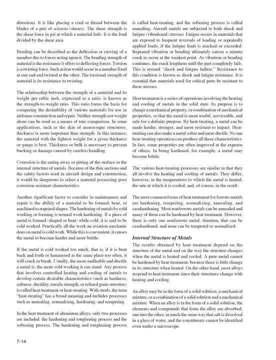 With steels. the term heat treating has a broad meaning and includes processes such as annealing, normalizing, hardening and tempering. In the heat treatment of aluminum alloys, only two processes are included: the hardening and toughening process and the softening process. 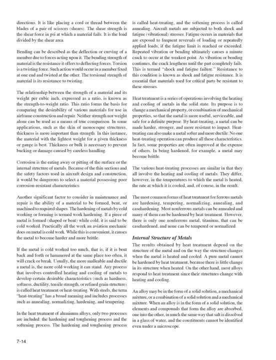 The hardening and toughening process is called heat treating and the softening process is called annealing. Aircraft metals are subjected to both shock and fatigue stresses. Fatigue occurs in materials that are exposed to frequent reversals of loading or repeatedly applied loads if the fatigue limit is reached or exceeded. Repeated vibration or bending ultimately causes a minute crack to occur at the weakest point. As vibration or bending continues, the crack lengthens until the part completely fails. This is termed shock and fatigue failure. Resistance to this condition is known as shock and fatigue resistance. It is essential that materials used for critical parts be resistant. 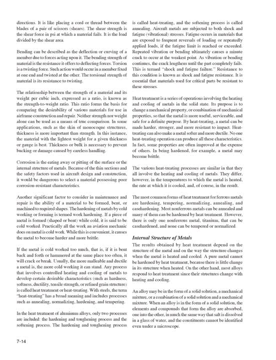 to these stresses. Heat treatment is a series of operations involving the heating and cooling of metals in the solid state. Its purpose is to change a mechanical property. A metal can be made hard or stronger and more resistant to impact. Heat treating can also make 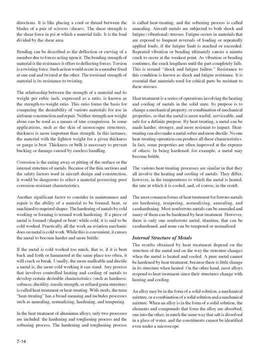 a metal softer and more ductile. No one heat treating operation can produce all these characteristics. In fact, some properties are often improved at the expense of others. In being hardened, for example, a metal may become brittle. The various heat treating processes are similar in the heat treatment of metal. The heat treatment of metal can be: 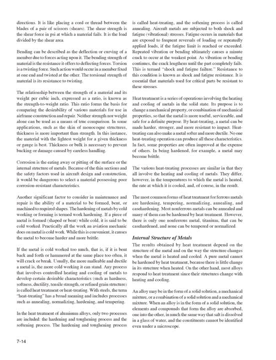 similar to the whole process In the heat treatment of metal- heat treatment can be hardened or tightened and the metal can become brittle or stronger- are similar in that they all involve the heating and cooling of metals. They differ, however, in the temperatures to which the metal is heated, the rate at which it is cooled and, of course, 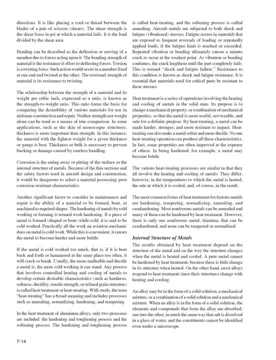 in the result. The most common forms of heat treatment for ferrous metals are hardening, tempering, normalizing, annealing and case hardening. Most non-ferrous metals can be annealed and many of them can be hardened by heat treatment. However, there is only one non-ferrous metal. 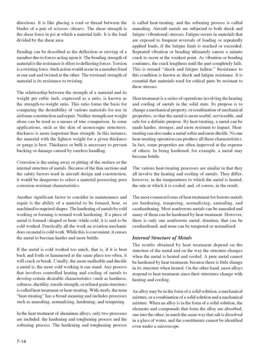 titanium, that can be case hardened and none can be tempered or normalized. Internal structure of metals. The results obtained by heat treatment depend on the structure of the metal and on the way the structure changes when the metal is heated and cooled. A pure metal cannot be hardened by heat treatment because there is little change in its 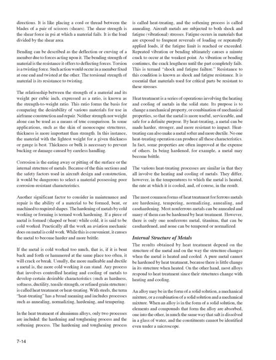 structure when heated. On the other hand, most alloys respond to heat treatment, since their structures change with heating and cooling. An alloy may be in the form of a solid solution, a mechanical mixture or a combination of a solid solution and a mechanical mixture. 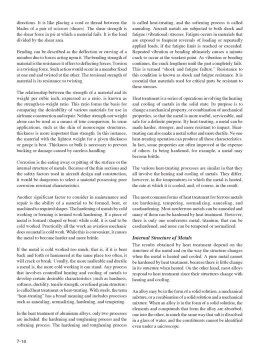 When an alloy is in the form of a solid solution, the elements and compounds that form the alloy are absorbed one into the other in much the same way that salt is dissolved in a glass of water, and the constituents cannot be identified even under a microscope. When two or more elements or compounds are mixed, but can be: 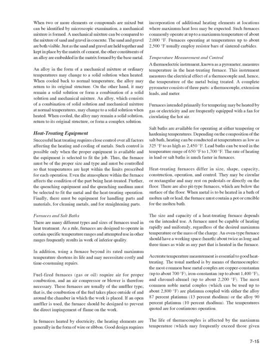 identified by microscopic examination, a mechanical mixture is formed. A mechanical mixture can be compared to the mixture of sand and gravel in concrete. The sand and gravel are both visible. Just as the sand and gravel are held together and kept in place by the matrix of cement, the other constituents of an alloy are embedded in the matrix formed by the. 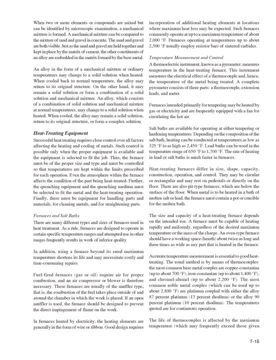 base metal, An alloy in the form of a mechanical mixture at ordinary temperatures may change to a solid solution when heated. When cooled back to normal temperature, the alloy may return to its original structure. On the other hand, it may remain a solid solution or form a combination. 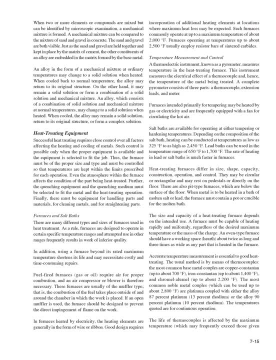 of a solid solution and mechanical mixture. An alloy which consists of a combination of solid solution and mechanical mixture at normal temperatures may change to a solid solution at regular temperatures. When cooled, the alloy may remain a solid solution. return to its original. 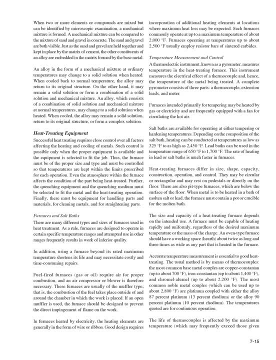 structure or form a complex solution. Heat treating equipment. Successful heat treating requires close control over all factors affecting the heating and cooling of metals. Such control is possible only when the proper equipment is available and the equipment is selected to fit the job. Thus, the furnace must be of the proper size and type and must be 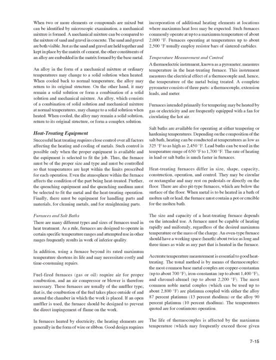 controlled so that temperatures are kept within the limits prescribed for each operation. Even the atmosphere within the furnace affects the condition of the part being heat treated. Further, the quenching equipment and the quenching medium must be selected to fit the metal and the 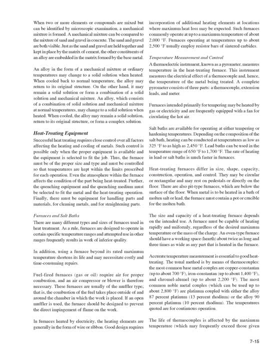 heat treating operation. Finally, there must be equipment for handling parts and materials, for cleaning metals and for straightening parts, Furnaces and salt baths. There are many different types and sizes of furnaces used in heat treatment. As a rule, furnaces are designed to operate in. 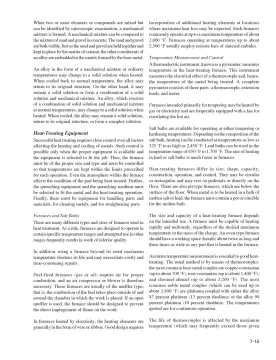 certain specific temperature ranges, and attempted use in other ranges frequently results in work of inferior quality. In addition, using a furnace beyond its rated maximum temperature shortens its life and may necessitate costly and time-consuming repairs. Fuel-fired furnaces, gas or oil require air for proper combustion, and an air compressor or blower is therefore. 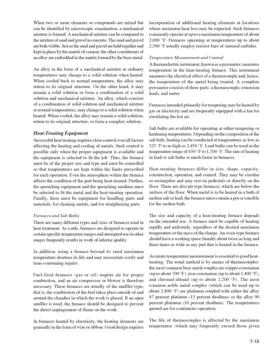 necessary. These furnaces are usually of the muffler type, that is, the combustion of the takes place outside of and around the chamber in which the work is placed. If an open muffler is used, the furnace should be designed to prevent the direct impingement. 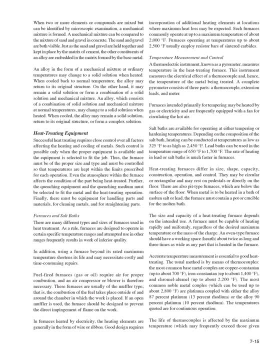 of flame on the work. In furnaces heated by electricity, the heating elements are generally in the form of wire or ribbon. Good design requires incorporation of additional heating elements at locations where maximum heat loss may be expected. Such furnaces commonly operate at up. 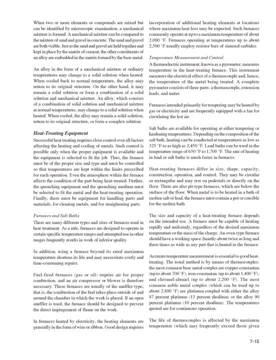 to a maximum temperature of about 2000°F. Furnaces operating at temperatures up to about 2500°F usually employ resistor bars of sintered carbides. Temperature measurement and control: a thermoelectric instrument are usually used to measure temperature and control a thermoelectric instrument. 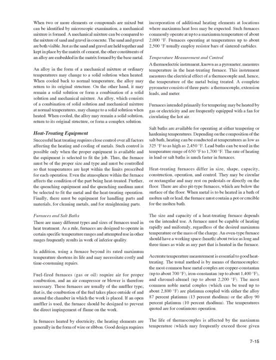 A thermoelectric instrument known as a pyrometer measures temperature in the heat-treating furnace. This instrument measures the electrical effect of a thermocouple and hence the temperature of the metal being treated. A complete pyrometer consists of three parts. 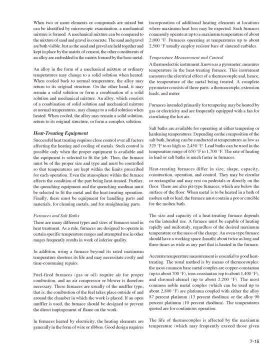 a thermocouple, extension leads and meter. Furnaces intended primarily for tempering may be heated by gas or electricity and are frequently equipped with a fan for circulating the hot air. Salt baths are available for operating at either tempering or hardening temperatures. 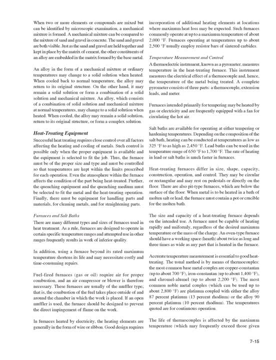 Depending on the condition of the furnace, the temperature of the furnace may be set to the temperature of the furnace For the composition of the salt bath. heating can be conducted at temperatures as low as 325°F to as high as 2450°F. Lead baths can be used in the temperature range 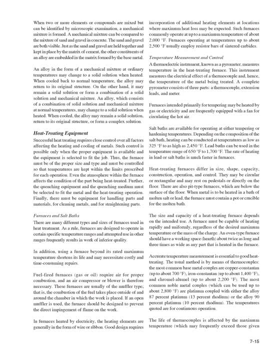 of 650°F to 1700°F. The rate of heating in lead or salt baths is much faster in furnaces. Heat-treating furnaces differ in size, shape, capacity, construction, operation and control. They may be circular or rectangular and may rest on pedestals. 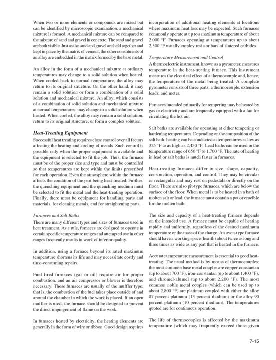 or directly on the floor. There are also pit-type furnaces which are below the surface of the floor. When metal is to be heated in a bath of molten salt or lead, the furnace must contain a pot or crucible for the molten bath. The size and capacity of a heat-treating furnace depends. 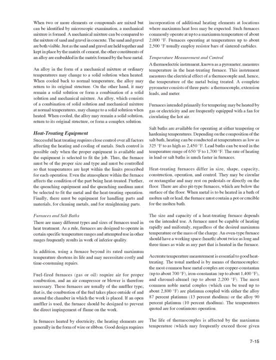 on the intended use. A furnace must be capable of heating rapidly and uniformly, regardless of the desired maximum temperature or the mass of the charge. An oven-type furnace should have a working space hearth about twice as long and three times as wide as any furnace. The furnace 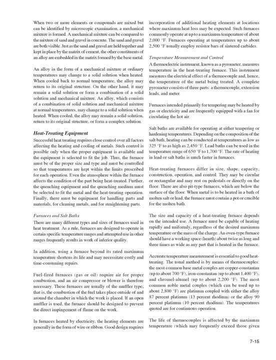 must be heat-treated in the furnace. Accurate temperature measurement is essential to good heat-treating. The usual method is by means of thermocouples. The most common base metal couples are: copper constantan up to about 700°F. iron constantan up to about 1400°F. 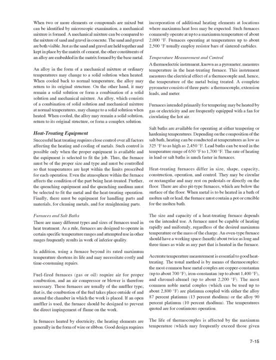 and chromal alumal up to about 2200°F. The most common noble metal couples which can be used up to about 2800°F are platinum coupled with either the alloy 87% platinum- 13% rhodium or the alloy 90% platinum 10% rhodium. The temperatures quoted are for 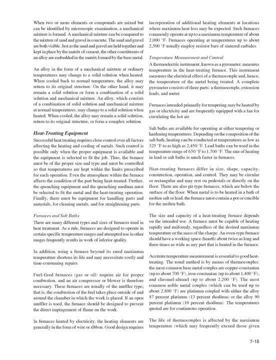 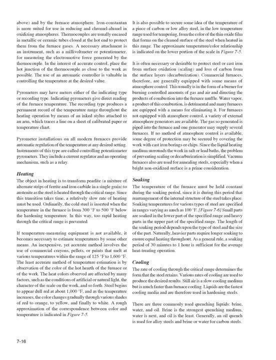 continuous operation. The life of thermocouples is affected by the maximum temperature, which may frequently exceed those given above, and by the furnace atmosphere. Iron constantan is more suited for use in reducing and chromal alumal in oxidizing atmospheres. Thermocouples are usually: 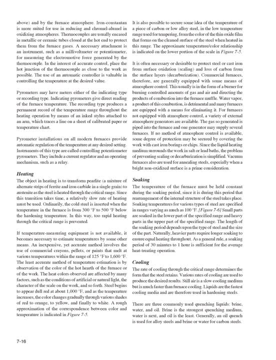 encased in metallic or ceramic tubes, closed at the hot end to protect them from the furnace gases. A necessary attachment is an instrument such as a millivolt meter or potentiometer for measuring the electromotive force generated by the thermocouple. In the interest of accurate 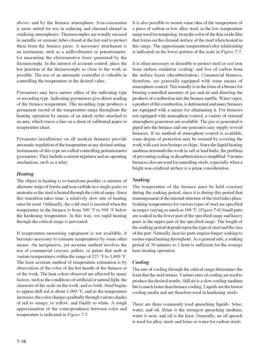 control place the hot junction of the thermocouple as close to the work as possible. The use of an automatic controller is valuable in controlling the temperature at the desired value. Pyrometers may have meters either of the indicating type or recording type. 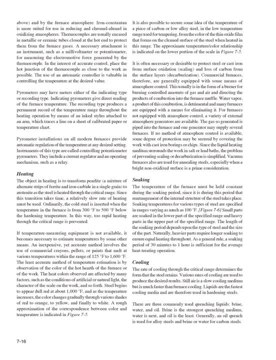 Indicating pyrometers give direct reading of the furnace temperature. The recording type produces a permanent accurate of the temperature range throughout the heating operation by means of an inked stylus attached to an arm which traces a line on a sheet of calibrated paper or temperature chart. 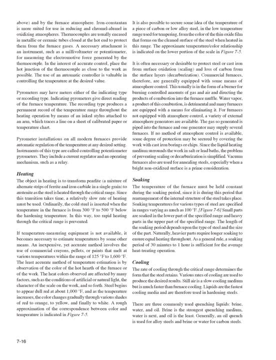 Pyrometer installations on all modern furnaces provide automatic regulation of the temperature at any desired setting. Instruments of this type are called controlling potentiometer pyrometers. They include a current regulator and an operating mechanism such as a relay Heating. the object in heating is to transform perlite. a mixture of alternate strips of. 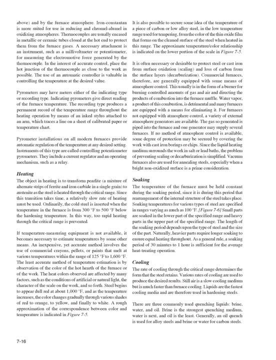 ferrite and iron carbide. in a system, The temperature of the furnace is determined by single grain to austenite as the steel is heated through the critical range. Since this transition takes time, a relatively slow rate of heating must be used. 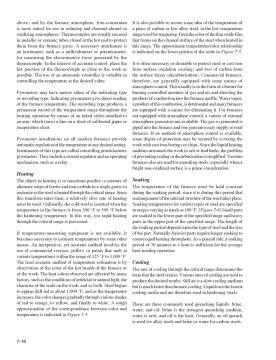 Ordinarily, the cold steel is inserted when the temperature in the furnace is from 300 degrees Fahrenheit to 500 degrees Fahrenheit below the hardening temperature. In this way, too, rapid heating through the critical range is prevented. If temperature measuring equipment is not available, it becomes necessary to estimate temperatures by some other means. 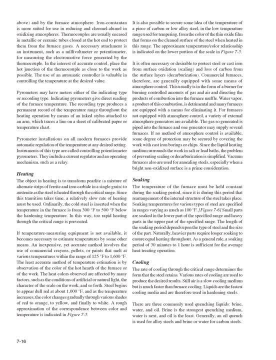 An inexpensive yet accurate method involves the use of commercial crayons, pellets or paints that melt at various temperatures within the range of 125 degrees Fahrenheit to 1600 degrees Fahrenheit. The least accurate method of temperature estimation is by observation of the color. 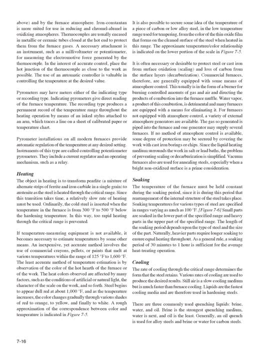 of the hot hearth of the furnace or of the work. The heat colors observed are affected by many factors, such as the conditions of artificial or natural light, the character of the scale on the work and so forth. Steel begins to appear dull red at about 1000 degrees Fahrenheit. 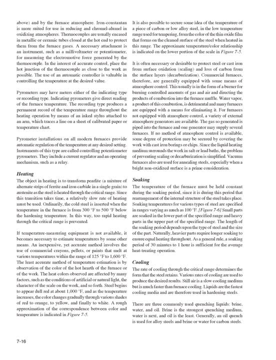 and as the temperature increases, the color changes gradually through various shades of red to orange, to yellow and finally to white. A rough approximation of the correspondence between color and temperature is indicated in Figure 7-5.. It is also possible to secure some idea of the 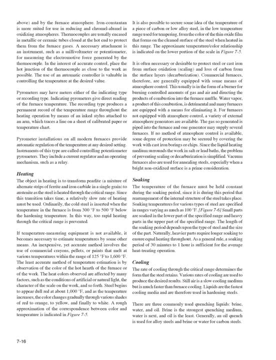 temperature of a piece of carbon or low-alloy steel in the low-temperature range used for tempering from the color of the thin oxide film that forms on the clean surface of the steel when heated. in this range, The approximate temperature-slash-color relationship is indicated on the lower-bottom. 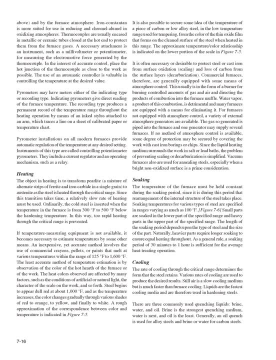 portion of the scale in Figure 7-5.. It is often necessary or desirable to protect steel or cast iron from surface oxidation, scaling and loss of carbon from the surface layers. decarburization Commercial furnaces, therefore, are generally equipped with some means of atmosphere control. 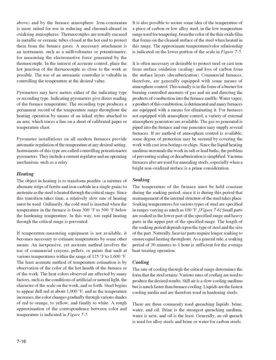 This usually is in the form of a burner for burning controlled amounts of gas and air and directing the products of combustion into the furnace muffle- Water vapor. a product of this combustion is detrimental and many furnaces are equipped with a means for a limited amount of 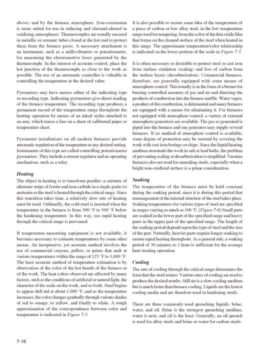 heat. The furnace is not equipped with atmosphere control. a variety of external atmosphere generators are available. The gas so generated is piped into the furnace, and one generator may supply several furnaces. If no method of atmosphere control is available, some degree of protection may. 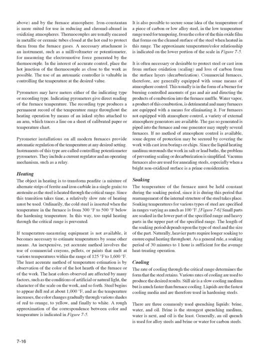 be secured by covering the work with cast iron borings or chips. Since the liquid heating medium surrounds the work in salt or lead baths, the problem of preventing scaling or decarburization is simplified. Vacuum furnaces also are used to protect the furnace from the heat of the furnace. 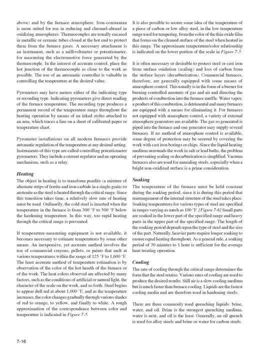 Soaking. the temperature of the furnace must be held constant during the soaking period, since it is during this period that rearrangement of the internal structure of the steel takes place. Soaking temperatures for various types of steel are specified in ranges varying as much as 100. 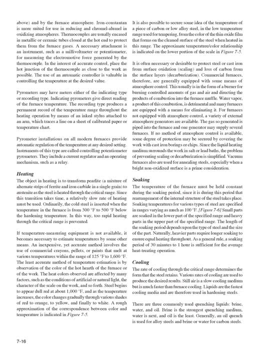 degrees Fahrenheit. Figure 7-6,. small parts are soaked in the lower part of the specified range and heavy parts in the upper part of the specified range. The length of the soaking period depends on the temperature of the furnace. The temperature of the furnace must be held. 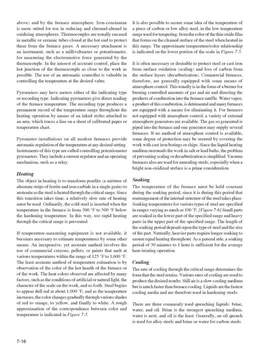 according to the type of steel and the size of the part. Naturally, heavier parts require longer soaking to ensure equal heating throughout. As a general rule, a soaking period of 30 minutes to 1 hour is sufficient for the average heat treating operation- Cooling the rate of cooling through the 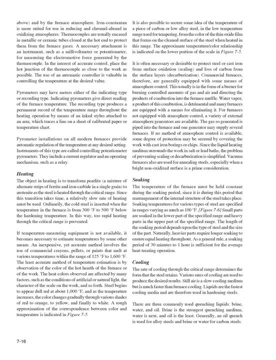 critical range determines the form that the steel retains. Various rates of cooling are used to produce the desired results. Still, air is a slow cooling medium but is much faster than furnace cooling. Liquids are the fastest cooling media and are therefore the fastest cooling media. 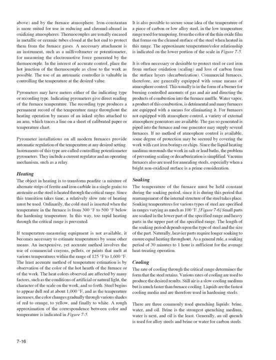 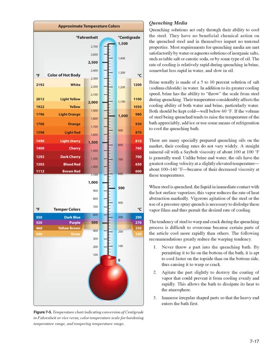 There are three commonly used quenching liquids: brine, water and oil. Brine is the strongest quenching medium, water is next and oil is the least. Generally, an oil quench is used for alloy steels and brine or water for carbon steels. Temperature range and tempering temperature. 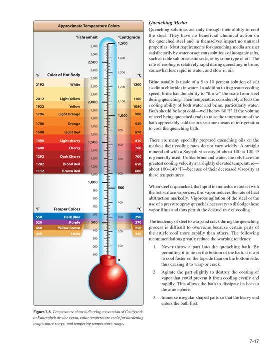 range Quenching media. quenching solutions act only through their ability to cool the steel. They have no beneficial chemical action on the quenched steel and in themselves impart no unusual properties. Most requirements for quenching media are met satisfactorily by water or aqueous solutions. 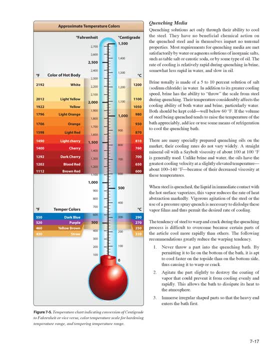 of inorganic salts such as table salt or caustic soda or by some type of oil. The rate of cooling is relatively rapid during quenching in brine, somewhat less rapid in water and slow in oil. Brine usually is made of a 5-10% solution of salt sodium chloride in water. In addition to its 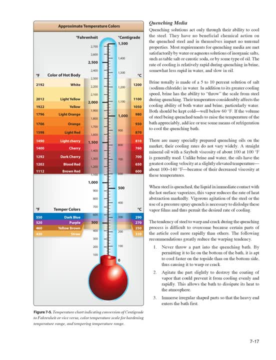 greater cooling speed. brine has the ability to throw the scale from steel during quenching. Their temperature considerably affects the cooling ability of both water and brine, particularly water. Both should be kept cold, well below 60 degrees Fahrenheit, If the volume of steel being quenched tends to raise the 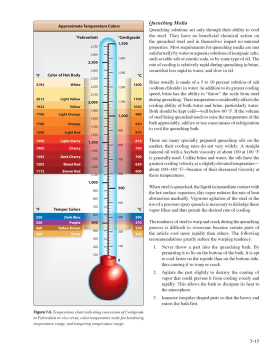 temperature of the bath appreciably. add ice or use some means of refrigeration to cool the quenching bath. There are many specially prepared quenching oils on the market. their cooling rates do not vary widely. A straight mineral oil with a sable viscosity. 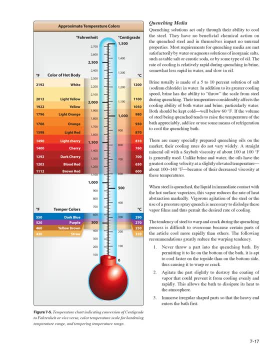 of about 100 at 100 degrees Fahrenheit is generally used. Unlike brine and water, the oils have the greatest cooling velocity at a slightly elevated temperature, about 100 to 140 degrees Fahrenheit, because of their decreased viscosity at these temperatures. When steel is quenched, the liquid in immediate contact with the hot surface vaporizes. 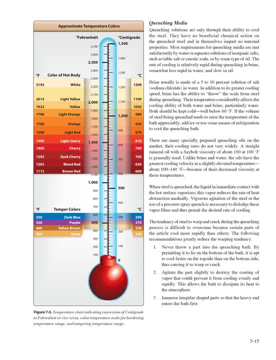 This vapor reduces the rate of heat abstraction markedly Vigorous agitation of the steel or the use of a pressure spray quench is necessary to dislodge these vapor films and thus permit the desired rate of cooling. The tendency of steel to warp and crack during the quenching process is 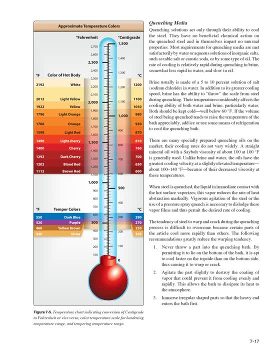 difficult to understand. The oil is often used to cool the hot surface. The oil is used to cool the hot surface. The oil is used to cool the hot surface. The oil is used to cool the hot surface To overcome because certain parts of the article cool more rapidly than others. 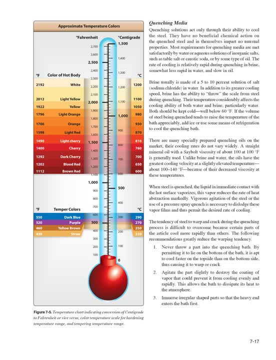 The following recommendations greatly reduce the warping tendency: 1. Never throw a part into the quenching bath By permitting it to lie on the bottom of the bath, it is apt to cool faster on the top side than on the bottom side, thus causing it to warp or crack. 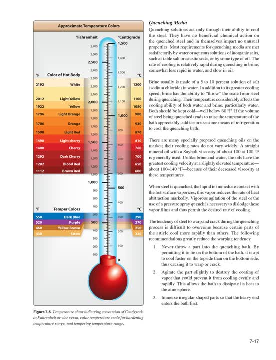 2. Agitate the part slightly to destroy the coating of vapor that could prevent it from cooling evenly and rapidly. This allows the bath to dissipate its heat to the atmosphere. 3. Immerse irregular-shaped parts so that the heavy end enters the bath first. 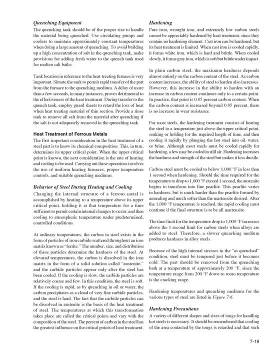 Quenching equipment. The quenching tank should be of the proper size to handle the material being quenched. Use circulating pumps and coolers to maintain approximately constant temperatures when doing a large amount of quenching To avoid building up a high. 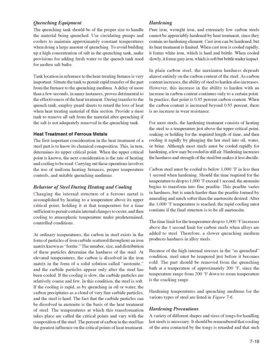 concentration of salt in the quenching tank. make provisions for adding fresh water to the quench tank used for molten salt baths. Tank location in reference to the heat-treating furnace is very important. Situate the tank to permit rapid transfer of the part from the furnace to the quenching medium. 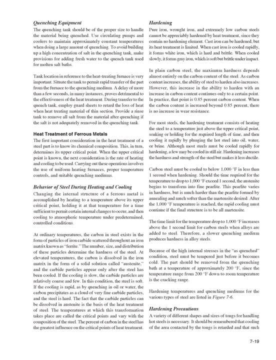 A delay of more than a few seconds in many instances proves detrimental to the effectiveness of the heat treatment. During transfer to the quenched tank, employ guard sheets to retard the loss of heat when heat-treating material of thin section. Provide a rinse tank to remove all salt. 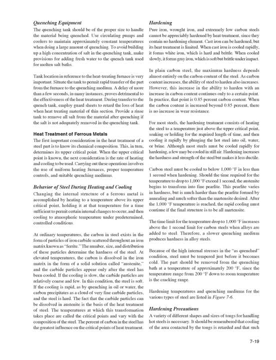 from the material after quenching if the salt is not adequately removed in the quenching tank. Heat treatment of ferrous metals. The first important consideration in the heat treatment of a steel part is to remove all salt from the material after quenching. If the salt is not. 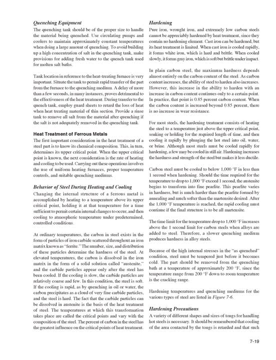 removed from the material after quenching. the heat treatment of a steel part is to know its chemical composition. This in turn determines its upper critical point. When the upper critical point is known, the next consideration is the rate of heating and cooling to be used. Carrying out 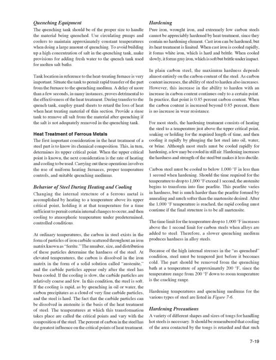 these operations involves the use of uniform heating furnaces, proper temperature controls and suitable quenching mediums. Behavior of steel during heating and cooling. Changing the internal structure of a ferrous metal is accomplished by heating to a temperature above its upper critical point, holding it at that temperature for a time sufficient to permit certain. 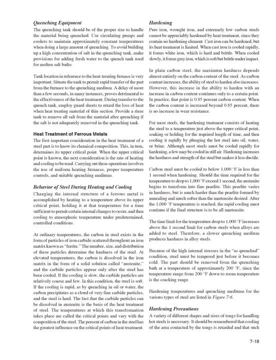 internal changes to occur and then cooling to atmospheric temperature under predetermined controlled conditions. At ordinary temperatures, the carbon in steel exists in the form of particles of iron carbide scattered throughout an iron matrix known as ferrite. The number, size and distribution of these particles determine the hardness of the steel. 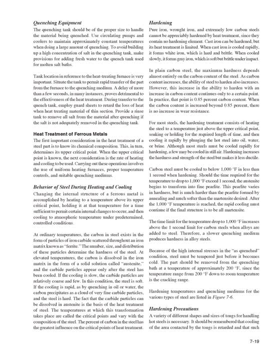 At elevated temperatures, the carbon is dissolved in the iron matrix in the form of a solid solution called austenite, and the carbide particles appear only after the steel has been cooled. If the cooling is slowed, the carbon is dissolved in the iron matrix in the form of a solid solution. 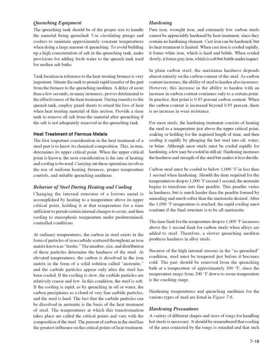 The carbide particles are relatively coarse and few. In this condition, the steel is soft. If the cooling is rapid, as by quenching in oil or water, the carbon precipitates as a cloud of very fine carbide particles and the steel is hard. The fact that the carbide particles 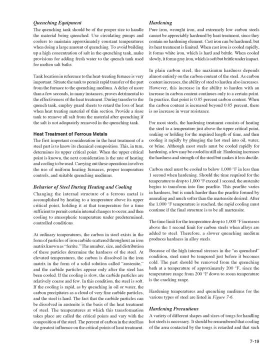 can be dissolved in austenite is the basis of the heat treatment of steel. The temperatures at which this transformation takes place are called the critical points and vary with the composition of the steel. The percent of carbon in the steel has the greatest influence on the 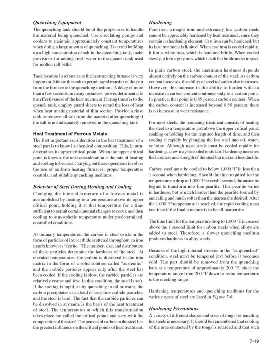 critical points of heat treatment. Hardening pure iron, wrought iron and extremely low carbon steels cannot be appreciably hardened by heat treatment since they contain no hardening element. Cast iron can be hardened, but its heat treatment is limited When cast iron is cooled. 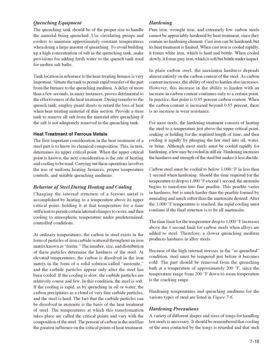 rapidly, it forms white iron, which is hard and brittle. When cooled slowly, it forms gray iron, which is soft but brittle under impact. In plain carbon steel, the maximum hardness depends almost entirely on the carbon content of the steel. As carbon content increases, the ability of steel to harden also increases. 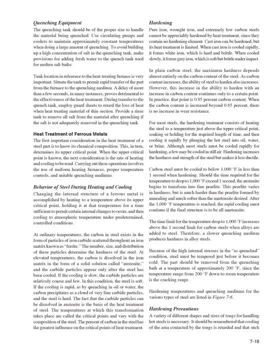 However, this increase in the ability to harden with an increase in carbon content continues only to a certain point In practice. that point is 0.85% carbon content. When the carbon content is increased beyond 0.85%, there is no increase in wear resistance For most steels. the hardening 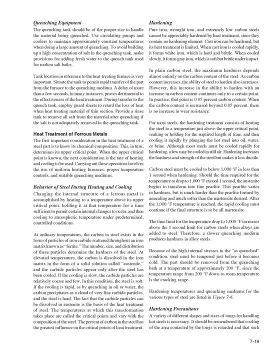 treatment consists of heating the steel to a temperature just above the upper critical point, soaking or holding for the required time, And then cooling it rapidly by plunging the hot steel into oil, water or brine. Although most steels must be cooled rapidly for hardening, a few may be cooled in still air. 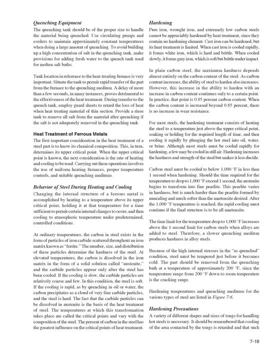 Hardening increases the hardness and strength of the steel, but makes it less ductile. Carbon steel must be cooled to below 1000 degrees Fahrenheit in less than one second. when hardening, Should the time required for the temperature to drop to 1000 degrees Fahrenheit exceed one second. 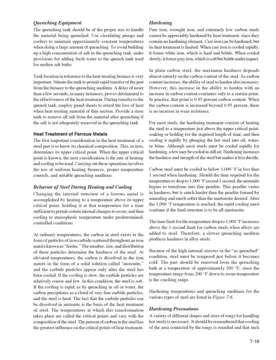 the austenite begins to transform into fine perlite. Perlite varies in hardness, but is much harder than the perlite formed by annealing and much softer than the martensite desired After the 1000 degrees Fahrenheit temperature is reached. 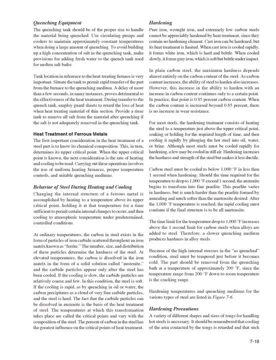 the rapid cooling must continue if the final structure is to be all martensite. The time limit for the temperature drop to 1000 degrees Fahrenheit increases above the one second limit for carbon steels when alloys are added to steel. Therefore a slower quenching. 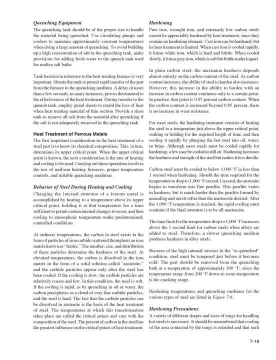 medium produces hardness in alloy steels Because of the high internal stresses. in the as-quenched condition the hardening process is more difficult. The hardening process is more difficult because the steel must be tempered just before it becomes cold. The part should be removed from the quenching bath. 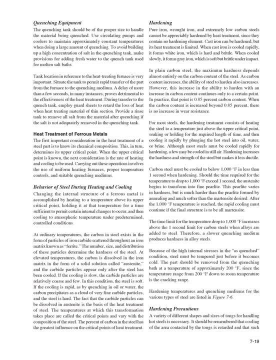 at a temperature of approximately 200 degrees Fahrenheit. since the temperature range from 200 degrees Fahrenheit down to room temperature is the cracking range, Hardening temperatures and quenching mediums for the various types of steel are listed in figure 7-6.. Hardening precautions. 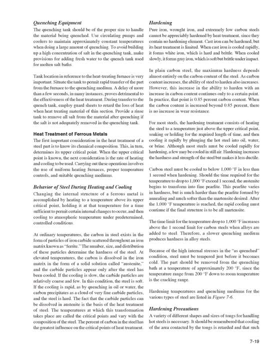 a variety of different shapes and sizes of tongs for handling hot steels is necessary. It should be remembered that cooling of the area contacted by the tongs is retarded and such Areas may not harden, particularly if the steel being treated is very shallow hardening. 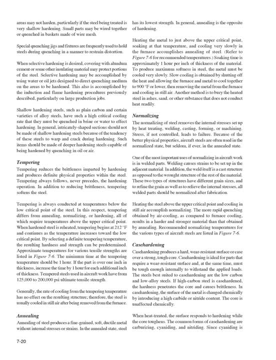 Small parts may be wired together or quenched in baskets made of wire mesh. Special quenching jigs and fixtures are frequently used to hold steels during quenching in a manner to restrain distortion. When selective hardening is desired, covering with a lundum, cement or some 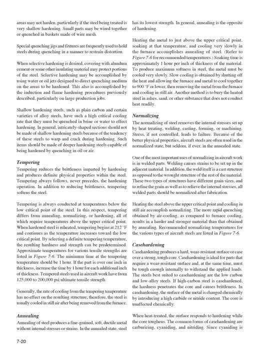 other insulating material may protect portions of the steel. Selective hardening may be accomplished by using water or oil jets designed to direct quenching medium on the area. This also is accomplished by the induction and flame hardening procedures previously described, particularly on large production jobs. Shallow hardening steels such as plain carbon and. 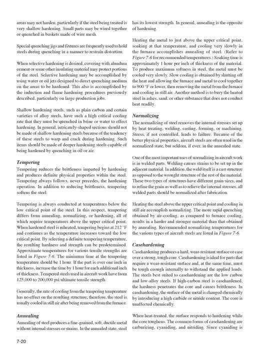 certain varieties of alloy steels have such a high critical cooling rate that they must be quenched in brine or water to affect hardening In general. intricately shaped sections should not be made of shallow hardening steels because of the tendency of these steels to warp and crack. 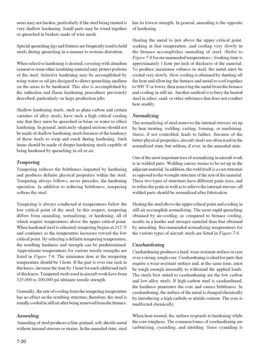 during hardening. Such items should be made of deeper hardening steels capable of being hardened by quenching in oil or air. Tempering Tempering reduces the brittleness imparted by hardening and produces definite physical properties within the steel. Tempering always follows, never precedes. 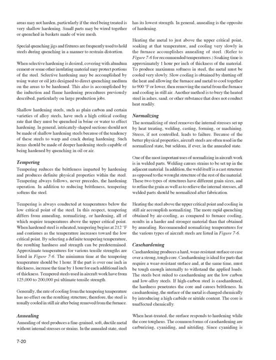 the hardening operation. In addition to reducing brittleness, tempering softens the steel. Tempering is always conducted at temperatures below the low critical point of the steel. In this respect, tempering differs from annealing, normalizing or hardening. 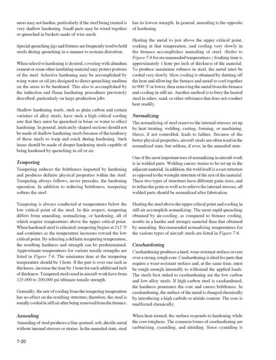 all of which require temperatures above the upper critical point. When hardened steel is reheated, tempering begins at 212 degrees Fahrenheit and continues as the temperature increases toward the low critical point. By selecting a definite tempering temperature, the resulting hardness and strength can be predetermined. Approximate temperatures for: 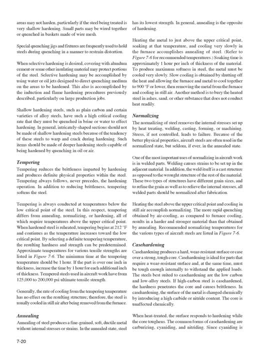 various tensile strengths are listed in figures 7 to 6.. The minimum time at the tempering temperature should be one hour. If the part is over one inch in thickness, increase the time by one hour for each additional inch of thickness. Tempered steels used in aircraft. 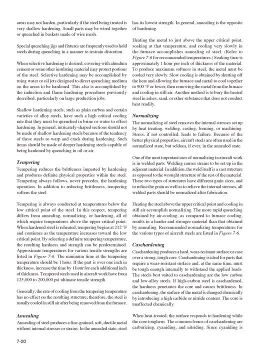 work have from 125,000 to 200,000 pounds per square inch ultimate tensile strength. Generally, the rate of cooling from the tempering temperature has no effect on the resulting structure. Therefore, the steel is usually cooled in still air after being removed from the furnace. 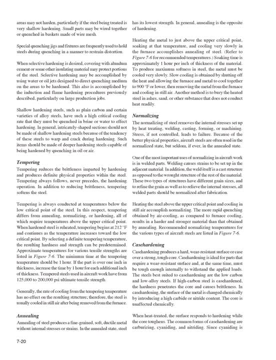 Annealing. Annealing of steel produces a fine-grained, soft, ductile metal without internal stresses or strains. In the annealed state, steel has its lowest strength. In general, annealing is the opposite of hardening, Heating the metal to just above. 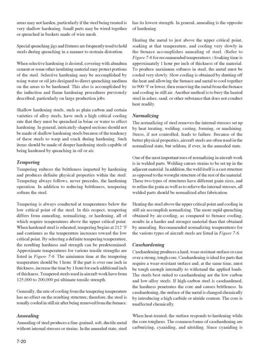 the upper critical point. soaking at that temperature and cooling very slowly in the furnace accomplishes annealing of steel. Refer to figure 7-6 for recommended temperatures. Soaking time is approximately one hour per inch of thickness of the material. To produce maximum softness in steel, the metal must be cooled very slowly. 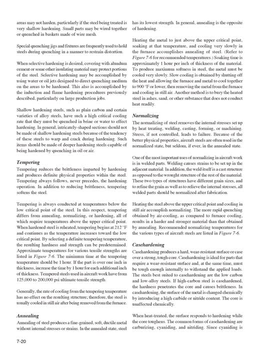 Slow cooling is obtained by shutting off the heat and allowing the furnace and metal to cool together to 900 degrees Fahrenheit or lower, then removing the metal from the furnace and cooling in still air. Another method is to bury the heated steel in ashes, sand or other substance that does. 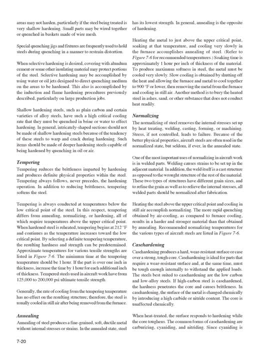 not conduct heat readily. Normalizing the normalizing of steel removes the internal stresses set up by heat treating, welding, casting forming or machining. Stress, if not controlled, leads to failure. Because of the better physical properties, aircraft steels are often used in the normalized state but seldom if ever in the annealed state. 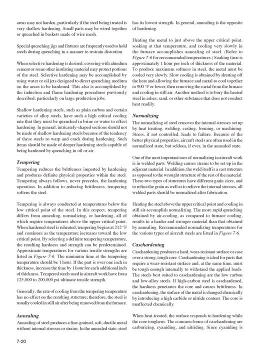 One of the most important uses of normalizing in aircraft work is in welded parts. Welding causes strains to be set up in the adjacent material. In addition, the weld itself is a cast structure as opposed to the wrought structure of the rest of the material. These two types of structures have different grain sizes and to refine the 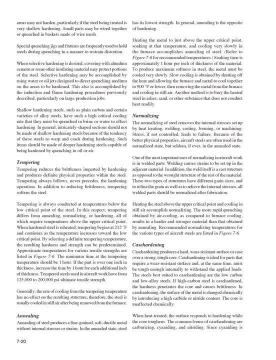 grain as well as to relieve the internal stresses. all welded parts should be normalized after fabrication. Heating the steel above the upper critical point and cooling in still air accomplish normalizing, The more rapid quenching obtained by air cooling as compared to furnace cooling. 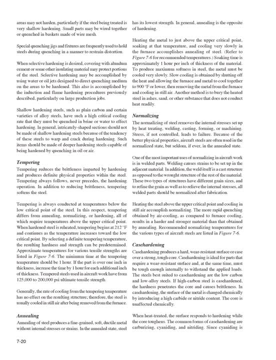 results in a harder and more stable structure. The more rapid quenching obtained by air cooling, the more stable structure and stronger material than that obtained by annealing. Recommended normalizing temperatures for the various types of aircraft steels are listed in figure 7-6.. Case hardening: Case hardening produces a hard. 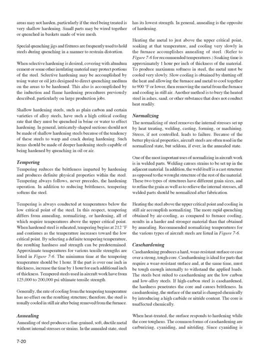 wear-resistant surface or case over a strong tough core. Case hardening is ideal for parts that require a wear-resistant surface and, at the same time, must be tough enough internally to withstand the applied loads. The steels best suited to case hardening are the low-carbon and. 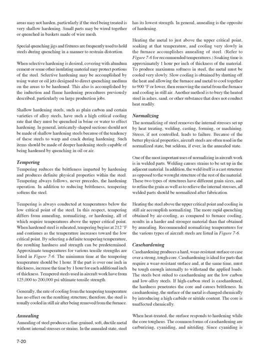 alloy steels. If high-carbon steel is case-hardened, the steel is best suited to case-hardening. The hardness penetrates the core and causes brittleness. In case hardening, the surface of the metal is changed chemically by introducing a high carbide or nitride content. The core is 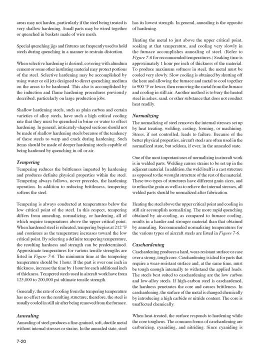 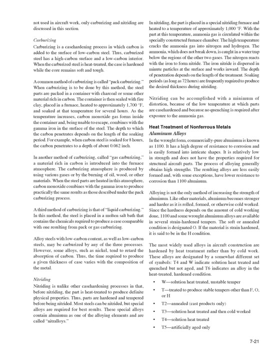 unaffected chemically. When heat-treated, the surface responds to hardening, while the core toughens. The common forms of case hardening are carburizing, cyaniding and nitriding. Since cyaniding is not used in aircraft work, only carburizing and nitriding are discussed in this. 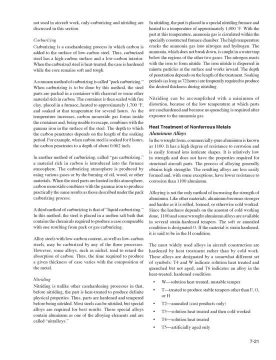 section. Carburizing is a case-hardening process in which carbon is added to the surface of low-carbon steel. Thus, carburized steel has a high-carbon surface and a low-carbon interior. When the carburized steel is heat-treated, the case is hardened while the core remains soft and tough. 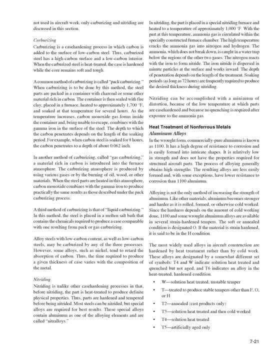 A common method of carburizing is called packed carburizing. When carburizing is to be done by this method, the steel parts are packed in a container with charcoal or some other material rich in carbon. The container is then sealed with fire clay. 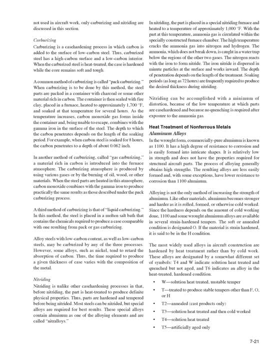 placed in a furnace heated to approximately 1,700 degrees Fahrenheit and soaked at that temperature for several hours. As the temperature increases, carbon monoxide gas forms inside the container and, being unable to escape, combines with the gamma iron in the surface of the steel. 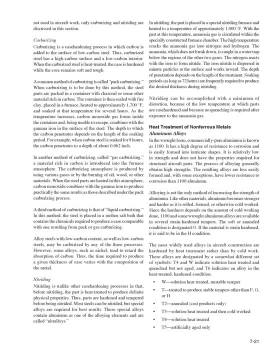 The depth to which the carbon penetrates depends on the length of the soaking period. For example, when carbon steel is soaked for 8 hours, the carbon penetrates to a depth of about 0.062 inch. Carburizing Called gas. carburizing a material rich in carbon is introduced into the furnace atmosphere. 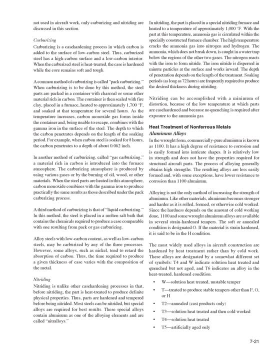 The carburizing atmosphere is produced by using various gases or by the burning of oil, wood or other materials. When the steel parts are heated in this atmosphere, carbon monoxide combines with the gamma iron to produce practically the same results as those described under the packed carburizing process. A third method of carburizing is that of liquid. 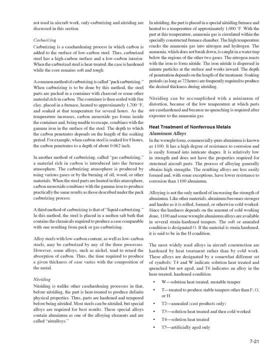 carburizing. In this method, the steel is placed in a molten salt bath that contains carbon monoxide. This means the chemicals required to produce a case comparable with one resulting from pack or gas carburizing. Alloy steels with low carbon content, as well as low carbon steels, may be carburized by 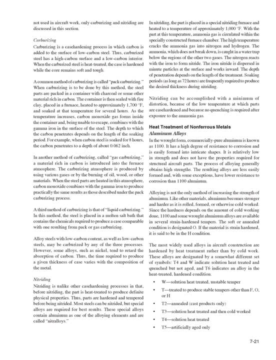 any of the three processes. However, some alloys, such as nickel, tend to retard the absorption of carbon. Thus the time required to produce a given thickness of case varies with the composition of the metal: Nitriding. Nitriding is unlike other case hardening processes in that before nitriding, 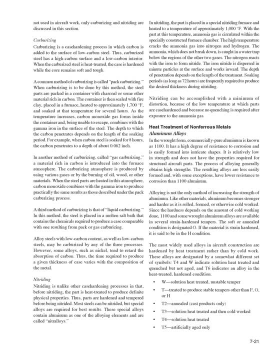 the part is heat-treated to produce definite physical properties. Thus parts are hardened and tempered before being nitrided. Most steels can be nitrided, but special alloys are required for best results. These special alloys contain aluminum as one of the alloying elements and are called nitraloys. 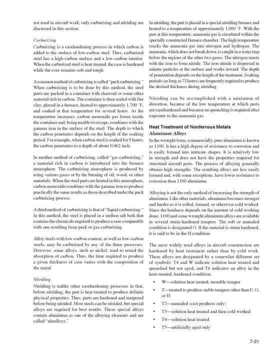 In nitriding. the part is placed in a special nitriding furnace and heated to a temperature of approximately 1000 degrees Fahrenheit. With a part at this temperature, ammonia gas is circulated within the specially constructed furnace chamber. The high temperature cracks the ammonia gas into nitrogen and hydrogen. The ammonia which does not break down is caught in a 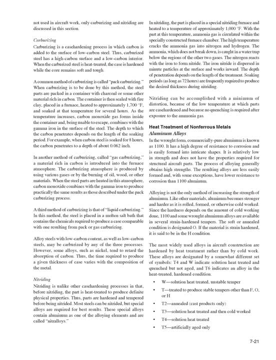 water trap below the regions of the other two gases. The nitrogen reacts with the iron to form nitride. The iron nitride is dispersed in minute particles at the surface and works inward. The depth of penetration depends on the length of the treatment: Soaking periods as long as 72 hours. 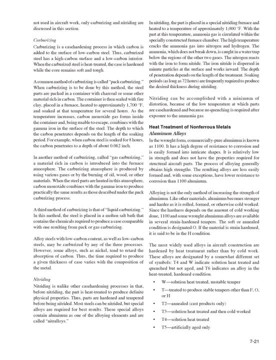 are frequently required to produce the desired thickness during nitriding. Nitriding can be accomplished with a minimum of distortion Because of the low temperature at which parts are case-hardened and because no quenching is required after exposure to the ammonia gas. Heat treatment of non-ferrous metals- aluminum. 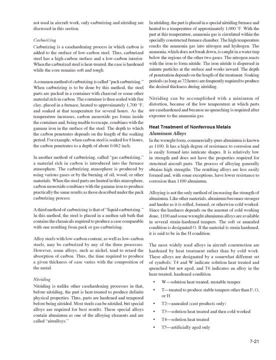 alloys in the wrought form. commercially pure aluminum is known as 1100. It has a high degree of resistance to corrosion and is easily formed into intricate shapes. It is relatively low in strength and does not have the properties required for structural aircraft parts. 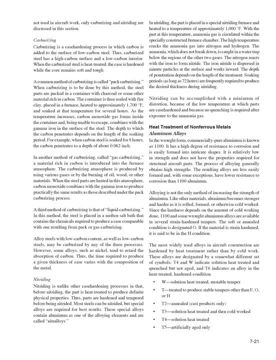 The process of alloying generally obtains high strengths. The resulting alloys are less efficient and more durable. The process of alloying generally obtains high strengths. Easily formed and, with some exceptions, have lower resistance to corrosion than 1100 aluminum. Alloying is not the only method of increasing the strength of aluminum. 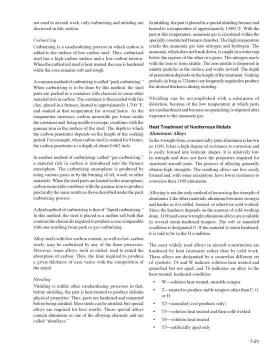 Like other materials, aluminum becomes stronger and harder as it is rolled, formed or otherwise cold-worked, Since the hardness depends on the amount of cold-working done. 1100 and some wrought aluminum alloys are available in several strain-hardened tempers. 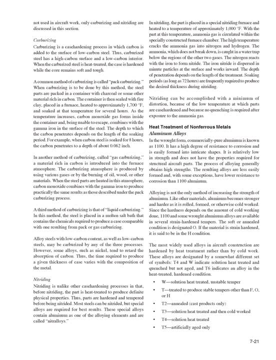 The soft or annealed condition is designated O. If the material is strain-hardened, it is said to be in the H condition. The most widely used alloys in aircraft construction are hardened by heat treatment rather than by cold work. These alloys are designated by a somewhat 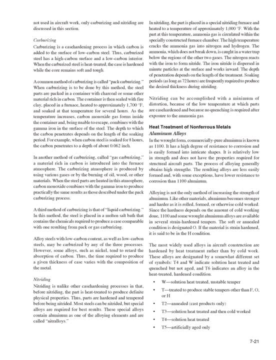 different set of symbols. T4 and W indicate solution heat-treated and quenched but not aged, and T6 indicates an alloy in the heat-treated hardened condition. W- solution- heat-treated, unstable temper. T- treated to produce stable tempers other than F. 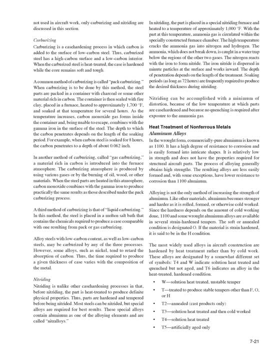 O or H- T2, annealed Cast products: only T3,. solution heat-treated and then cold-worked: D4, solution heat-treated- D5, artificially aged: only T6,. solution heat-treated and then artificially aged. T7, solution heat-treated and then stabilized. T8, solution heat-treated, cold-worked and then artificially aged. T9, solution heat-treated, artificially aged and then cold-worked. T10, artificially aged and then cold-worked. 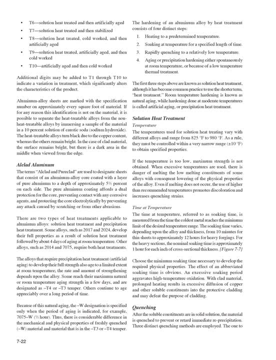 Additional digits may be added to T1 through T2.. tend to indicate a variation in treatment which significantly alters the characteristics of the product. Aluminum alloy sheets are marked with a specification number on approximately every square foot of material. If, for any reason, this identification is not on the material, 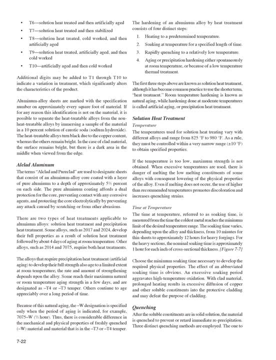 it is possible to separate the heat-treatable alloys from the non-heat-treatable alloys by immersing a sample of the material in a 10% solution of caustic soda sodium hydroxide. The heat-treatable alloys turn black due to the copper content, whereas the others remain bright. 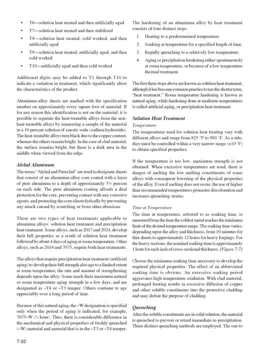 In the case of clad material, the surface remains bright, but there is a dark area in the middle when viewed from the edge. Alclad- aluminum. The terms alclad and pure clad are used to designate sheets that consist of an aluminum alloy core coated with a layer of 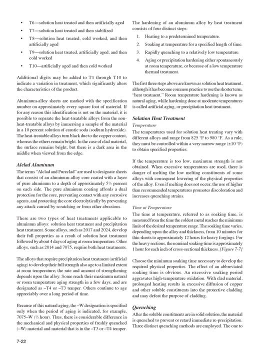 pure aluminum to a depth of approximately 51.5% on each side. The pure aluminum coating affords a dual protection for the core, preventing contact with any corrosive agents and protecting the core electrolytically by preventing any attack caused by scratching or from other abrasions. 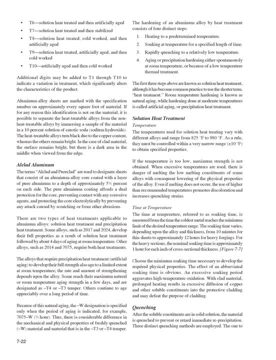 Alclad aluminum. There are two types of heat treatments applicable to aluminum alloys: solution heat treatment and precipitation heat treatment. Some alloys, such as 2017 and 2024, develop their full properties as a result of solution heat treatment, followed by about. four days of aging at room temperature. Other alloys, such as 2014 and 7075, require both heat treatments. The alloys that require precipitation heat treatment- artificial aging- to develop their full strength- also age to a limited extent at room temperature. The rate and amount of strengthening depends upon the alloy. 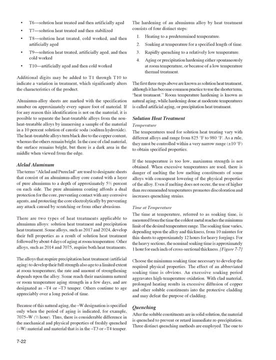 Some reach their maximum natural or room temperature aging strength in a few days and are designated as T4 or T3 temper. Others continue to age appreciably over a long period of time Because of this natural aging. the W designation is specified only when the period 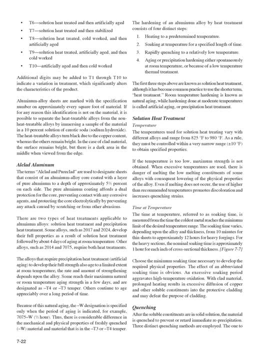 of aging is indicated, for example 7075 W half hour. Thus there is considerable difference in the mechanical and physical properties of freshly quenched aluminum. The alloys that are used to heat. heat treatment consist of four distinct steps: 1. Heating to a predetermined temperature. 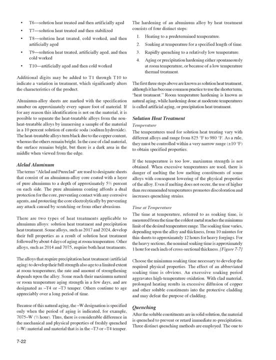 2. Soaking at temperature for a specified length of time. 3. Rapidly quenching to a relatively low temperature. 4. Aging or precipitation hardening, either spontaneously at room temperature or because of a low temperature thermal treatment. 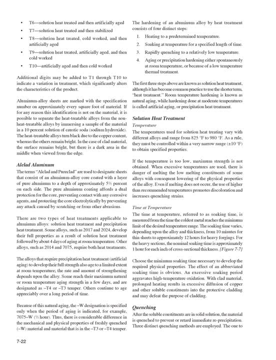 The first three steps are the following. The three steps above are known as solution heat treatment, although it has become common practice to use the shorter term heat treatment. Room temperature hardening is known as natural aging, while hardening done at moderate temperatures is called artificial aging. or precipitation heat treatment. Solution heat treatment temperature. The temperatures used for solution heat treating vary with different alloys and range from 825 degrees Fahrenheit to 980 degrees Fahrenheit. As a rule, they must be controlled within a very narrow range: plus or minus 10 degree Fahrenheit. The temperature used for heat treatment is used. 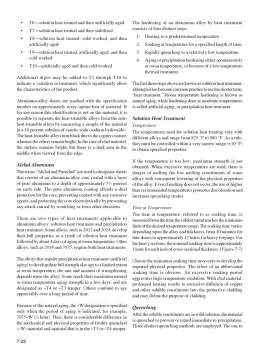 to obtain specified properties. If the temperature is too low, maximum strength is not obtained. When excessive temperatures are used, there is danger of melting the low melting constituents of some alloys, with consequent lowering of the physical properties of the alloy. Even if melting does not occur, the use of higher than recommended temperatures promotes 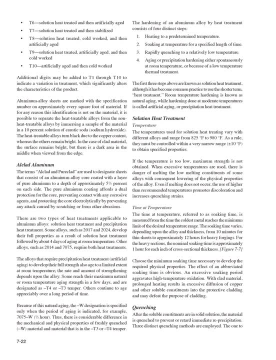 discoloration and increases quenching strains. Time at temperature. The time at temperature, referred to as soaking time, is measured from the time the coldest metal reaches the minimum limit of the temperature. The soaking time varies depending upon the alloy and thickness, from 10 minutes for thin sheets to 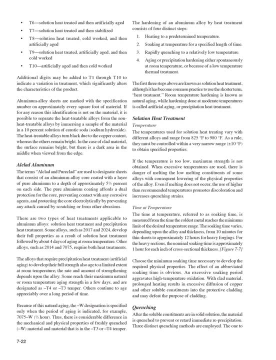 approximately 12 hours for heavy forgings. For the heavy sections, the nominal soaking time is approximately one hour for each inch of cross-sectional thickness. Figure 7-7, choose the minimum soaking time necessary to develop the required physical properties. The effect of an. 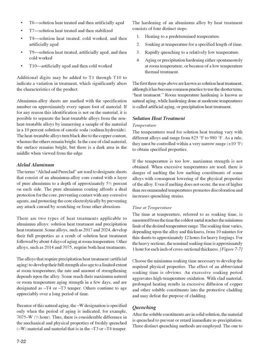 abbreviated soaking time is obvious. An excessive soaking period aggravates high temperature oxidation. The effect of an abbreviated soaking time is obvious. An excessive soaking period aggravates high temperature oxidation With the minimum soaking time required. the soaking time With clad material. prolonged heating results in excessive diffusion of copper and other. 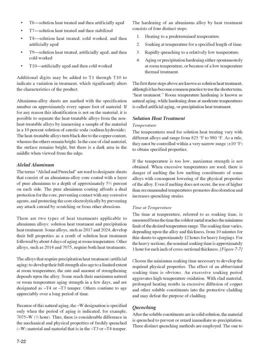 soluble constituents into the protective cladding and may defeat the purpose of cladding Quenching. after the soluble constituents are in solid solution, the material is quenched to prevent or retard immediate re-precipitation. Three distinct quenching methods are employed. 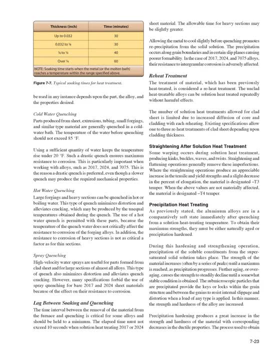 The one to be used in any instance depends upon the part, the alloy and the properties desired. Cold water quenching parts produced from sheet extrusions, tubing, small forgings and similar type material are generally quenched in a cold water bath. 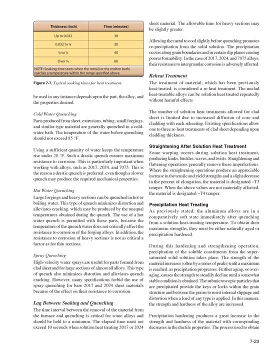 The temperature of the water before quenching should not exceed 85 degrees Fahrenheit. Using a sufficient quantity of water keeps the temperature rise under 20 degrees Fahrenheit. Such a drastic quench ensures maximum resistance to corrosion. This is particularly important when working with alloys such as 2017, 2024, and 7070. 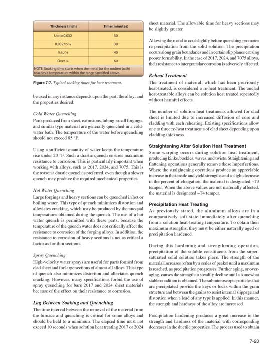 This is the reason a drastic quench is preferred, even though a slower quench may produce the required mechanical properties. Hot water quenching, large forgings and heavy sections can be quenched in hot or boiling water. This type of quench minimizes distortion and alleviates cracking which may be produced. 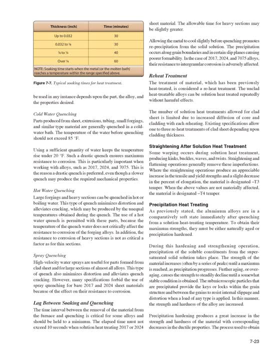 by the unequal temperatures obtained during the quench. The use of a hot water quench is permitted with these parts because the temperature of the quench water does not critically affect the resistance to corrosion of the forging alloys. In addition, the resistance to corrosion of heavy sections is not as critical a factor as for thin sections. 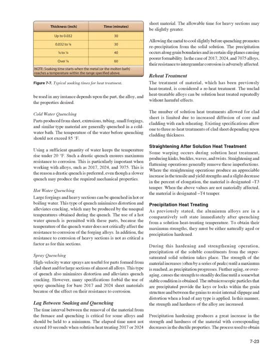 Spray quenching. high-velocity water sprays are useful for parts formed from clad sheet and for large sections of almost all alloys. This type of quench also minimizes distortion and alleviates quench cracking. However, many specifications forbid the use of spray quenching for bare 2017 and 2024. 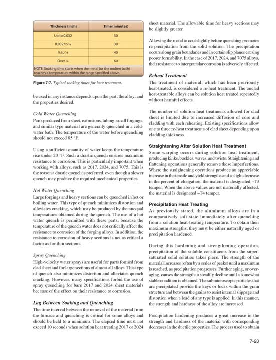 sheet materials because of the effect on their resistance to corrosion. Lag between soaking and quenching. The time interval between the removal of the quenching and the quenching of the quenching is critical for some alloys and should be held to a minimum. 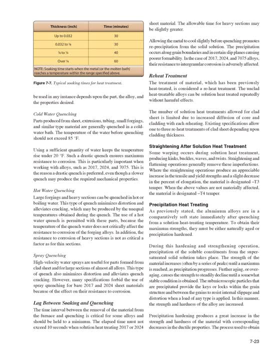 The elapsed time must not exceed 10 seconds. when solution heat-treating 2017 or 2024 sheet material, The allowable time for heavy sections may be slightly greater. Allowing the metal to cool slightly before quenching promotes re-precipitation from the 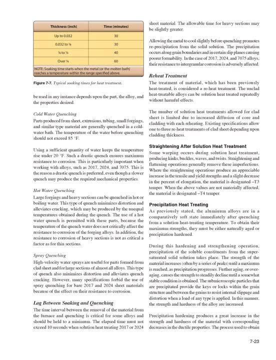 solid solution. The precipitation occurs along grain boundaries and in certain slip planes, causing poorer formability. In the case of 2017, 2024, and 2017, the time interval between the removal of the quenching and the quenching is non-existent. 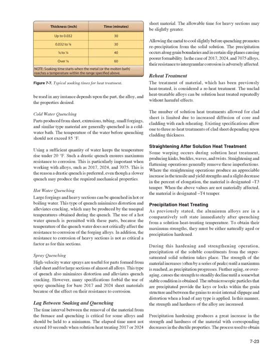 The heat treatment of the material is left이라는, and when the material has been treated before the curing process, the solution heat is not treated. The solution heat treatment is considered a reheat treatment. The unclad heat-treatable alloys can be solution heat-treated repeatedly without harmful effects. 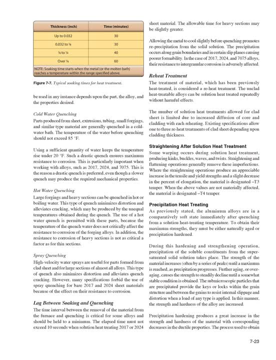 The number of solution heat treatments allowed for clad sheet is limited due to increased diffusion of core and cladding with each reheating. Existing specifications allow 1-3 reheat treatments of clad sheet depending upon cladding thickness. Straightening after solution heat treatment. Some warping occurs during solution heat treatment. 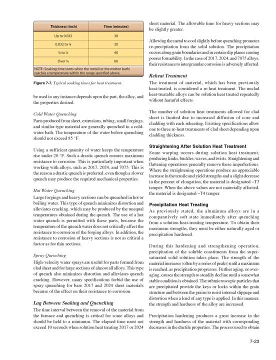 producing kinks, buckles, waves and twists. Straightening and flattening operations generally remove these imperfections, Where the straightening operations produce an appreciable increase in the tensile and yield strengths and a slight decrease in the percent of elongation the material is. 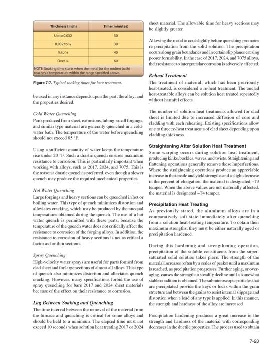 designated T3 temper. When the above values are not materially affected, the material is designated T4 temper. Precipitation: heat treating: As previously stated, the aluminum alloys are in a comparatively soft state immediately after quenching from a solution heat treating temperature. To obtain their maximum strengths, they must be either naturally aged or precipitation. 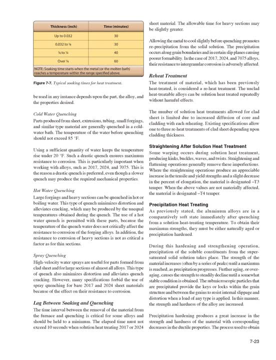 hardened. During this hardening and strengthening operation, precipitation of the soluble constituents from the super-saturated solid solution takes place. The strength of the material increases often by a series of peaks until a maximum is reached. as precipitation progresses Further, aging or over-aging causes the strength to steadily decline until a somewhat 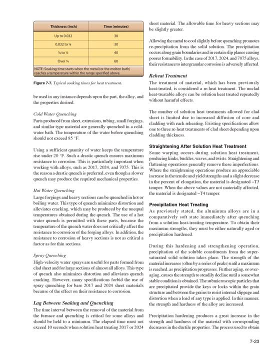 stable condition is obtained. The submicroscopic particles that are precipitated provide the keys or locks within the grain structure and between the grains to resist internal slippage and distortion. when a load of any type is applied In this manner, the strength and hardness of the 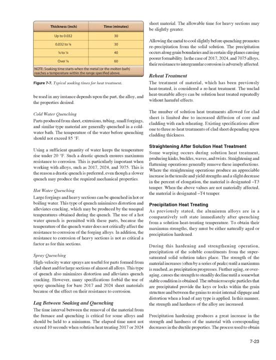 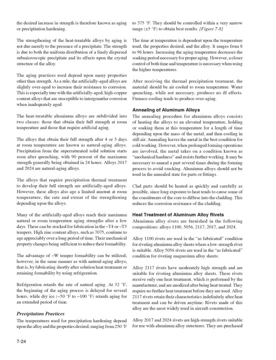 alloy are increased. Precipitation hardening produces a great increase in the strength and hardness of the material, with corresponding decreases in the ductile properties. The process used to obtain the desired increase in strength is therefore known as aging or precipitation hardening. The strengthening of the heat treatable alloys by aging is not due merely 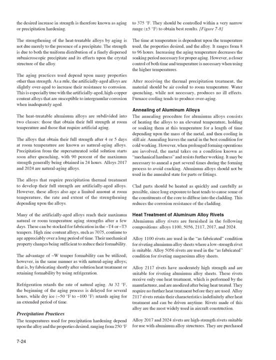 to the presence of a precipitate. The strength is due to both the uniform distribution of a finely dispersed submicroscopic precipitate and its effects upon the crystal structure of the alloy. The aging practices used depend upon many properties other than strength. As a rule, the artificially aged alloys are slightly over-aged to increase their 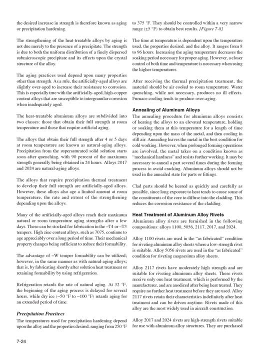 resistance to corrosion. This is especially true with the artificially aged high-copper-content alloys that are susceptible to intergranular corrosion when inadequately aged. The heat treatable aluminum alloys are subdivided into two classes: those that obtain their full strength at 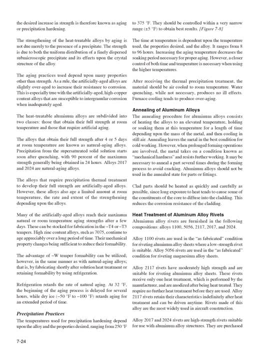 room temperature and those that require artificial aging. The alloys that obtain their full strength after four or five days at room temperature are known as natural aging alloys. Precipitation from the supersaturated solid solution starts soon after quenching, with 90% of the maximum strength generally being obtained in 24 hours. 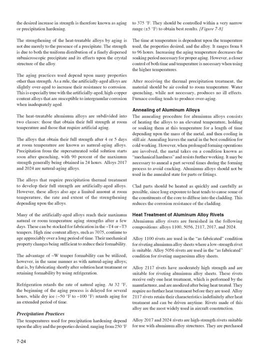 Alloys 2017 and 2024 are natural aging alloys. The alloys that require precipitation thermal treatment to develop their full strength are artificially aged alloys. However, these alloys also age a limited amount at room temperature, the rate and extent of the strengthening depending. 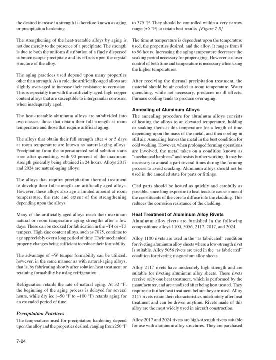 upon the alloys. Many of the artificially aged alloys reach their maximum natural or room temperature aging strengths after a few days. These can be stopped by a heat treatable solution or a retaining formability by using refrigeration. Refrigeration retards the rate of 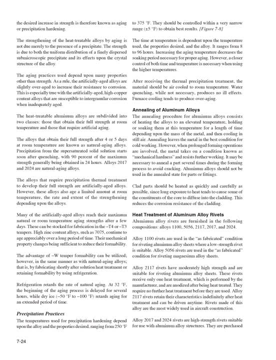 natural aging alloys. The alloys that obtain their full strength at room temperature can be stopped by a heat treatable solution or a retaining formability. by using refrigeration At 32°F, the beginning of the aging process is delayed for several hours while dry ice. 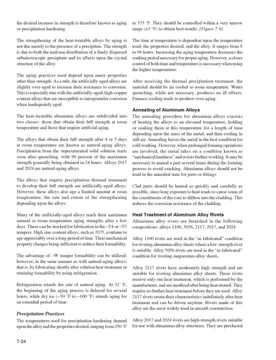 –50°F to –100°F. retards aging for an extended period of time. Precipitation practices: the temperatures used for precipitation hardening depend upon the alloy and the properties desired, ranging from 250°F to 375°F. They should be controlled within. 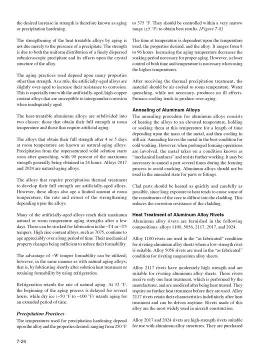 a very narrow range- plus or minus 5°F- to obtain the best result. Figure 7-8: The time at temperature is dependent upon the temperature used, the properties desired and the alloy. It ranges from 8 to 96 hours. Increasing the aging temperature decreases the soaking period necessary for proper aging. However, a closer control of both time and temperature is necessary when using the higher temperatures. After receiving the thermal precipitation treatment, the material should be air-cooled to room temperature. Water quenching, while not necessary, provides a good 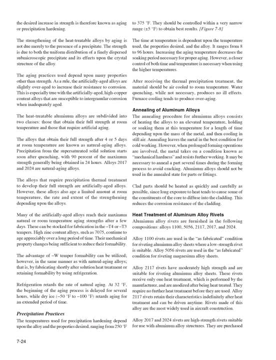 temperature control. However, a closer control of both time and temperature is necessary when using the higher temperatures. After receiving the thermal precipitation treatment, the material should be air-cooled to room temperature. Water quenching, while not necessary, produces no ill effects. Furnace cooling tends to produce over-aging. 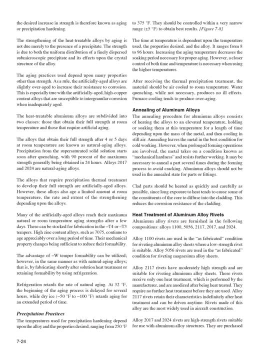 Furnace cooling tends to produce over-aging. Annealing of Aluminum Alloys. The annealing procedure for aluminum alloys consists of heating the alloys to an elevated temperature, holding or soaking them at this temperature for a length of time, depending upon the mass of the metal, and then cooling in still air. Annealing leaves the metal in. 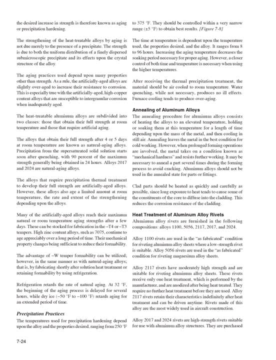 the best condition for cold working. However, when prolonged forming operations are involved, the metal takes on a condition known as mechanical hardness and resists further working. It may be necessary to anneal a part several times during the forming process to avoid cracking. 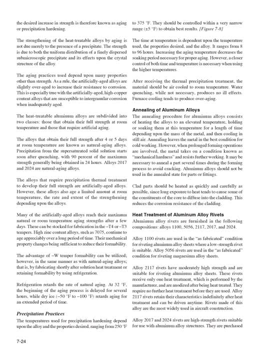 Aluminum alloys should not be used in the annealed state for parts or fittings. Clad parts should be heated as quickly and carefully as possible, since long exposure to heat tends to cause some of the constituents of the core to diffuse into the cladding. This reduces 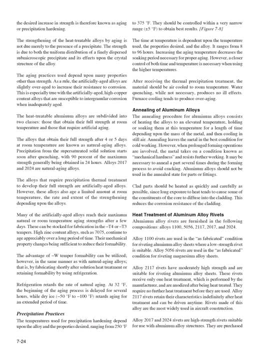 the corrosion resistance of the cladding. Heat Treatment of Aluminum Alloy Rivets. Aluminum alloy rivets are furnished in the following compositions: alloys 1100, 5056,, 2117,, 2017 and 2024.. Alloy 1100 rivets are used in the as fabricated condition for riveting. 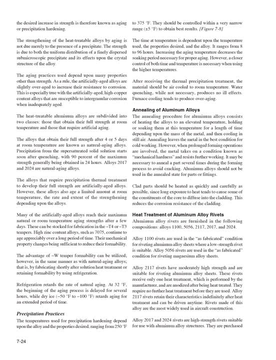 aluminum alloy sheets where a low strength rivet is suitable. Alloy 5056 rivets are used in the as fabricated condition for riveting aluminum alloy sheets. rivets are used in the as-fabricated condition for riveting magnesium alloy sheets. Alloy 2117 rivets have moderately high strength and are suitable for riveting aluminum alloy. 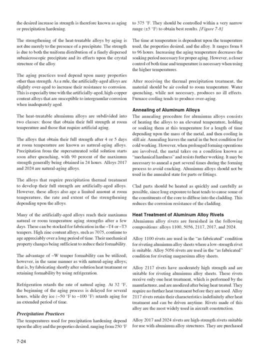 sheets. These rivets receive only one heat treatment, which is performed by the manufacturer, and are anodized after being heat treated. They require no further heat treatment before they are used. Alloy 2117 rivets retain their characteristics indefinitely after heat treatment. 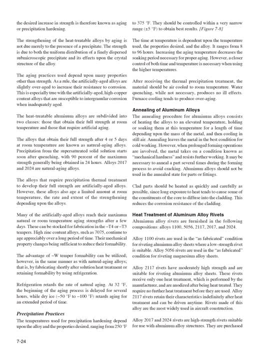 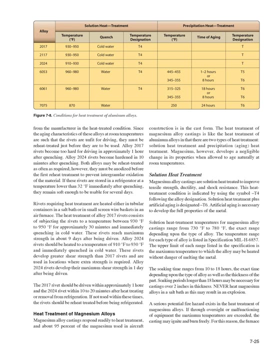 and can be driven anytime. Rivets made of this alloy are the most widely used in aircraft construction. Alloy 2017 and 2024 rivets are high-strength rivets suitable for use with aluminum alloy structures. They are purchased from the manufacturer in the heat-treated condition. 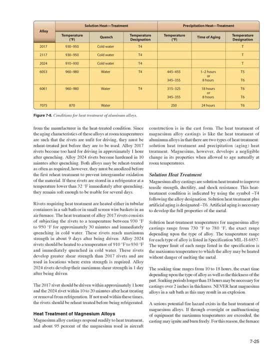 Since the aging characteristics of these alloys at room temperatures are such that the rivets are unfit for driving, they must be reheat-treated just before they are to be used. Alloy 2017 rivets become too hard for driving in approximately one hour after quenching. Alloy 2024: rivets become hardened in 10 minutes after quenching. 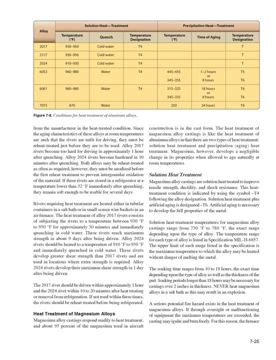 Both alloys may be reheat-treated as often as required. however, they must be anodized before the first reheat treatment to prevent intergranular oxidation of the material If these rivets are stored in a refrigerator at a temperature lower than 32 degrees Fahrenheit. 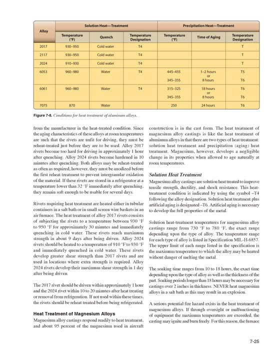 immediately after quenching, they remain soft enough to be usable for several days. Rivets requiring heat treatment are heated either in tubular containers, in a salt bath or in a water bath. Alloy 2017 rivets are stored in a refrigerator at a temperature lower than 32. 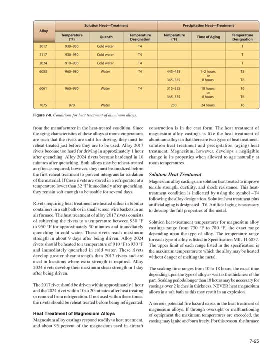 degrees Fahrenheit. The heat treatment of alloy 2017 rivets consists of subjecting the rivets to a temperature between 930 degrees Fahrenheit to 950 degrees Fahrenheit for approximately 30 minutes and immediately quenching in cold water. These rivets reach maximum strength in about nine days. 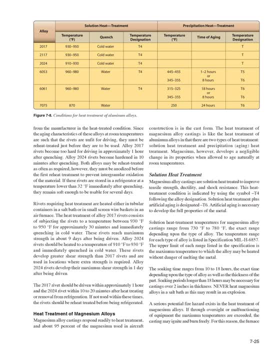 after being driven, Alloy 2024 rivets should be heated to a temperature of 910 degrees Fahrenheit to 930 degrees Fahrenheit and immediately quenched in cold water. These rivets do not need to be heated. These rivets develop greater shear strength than 2017 rivets and are used in locations where extra. 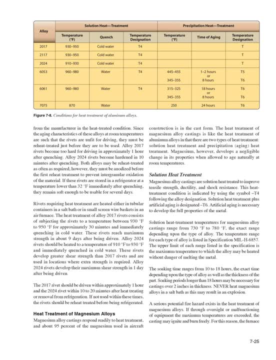 strength is required. Alloy 2024 rivets develop their maximum shear strength in one day after being driven. The 2017 rivet should be driven within approximately one hour and the 2024 rivet within 10 to 20 minutes after heat treating or removal from refrigeration, If not used within. 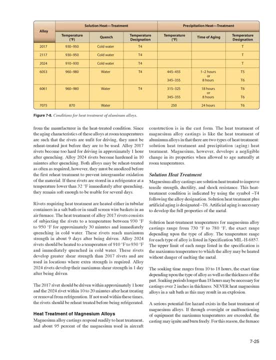 these times, the rivets should be reheat treated before being refrigerated. Heat treatment of magnesium alloys- magnesium alloy castings. The heat treatment of magnesium alloy castings is like the heat treatment of aluminum alloys in that there are two types of heat treatment solution: heat treatment and precipitation. aging heat. 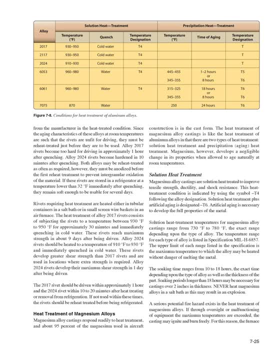 treatment. Magnesium, however, develops a negligible change in its properties when allowed to age naturally at room temperatures. Solution heat treatment. magnesium alloy castings are solution heat treated to improve tensile strength, ductility and shear strength. This heat treatment condition is indicated by using the symbol T4 following the alloy designation. 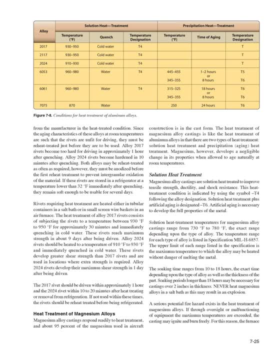 Solution, heat treatment plus artificial aging, is designated T6.. Artificial aging is necessary to develop the full properties of the metal Solution. heat treatment temperatures for magnesium alloy castings range from 730°F to 780°F, the exact range depending upon the type of alloy. The temperature range for each type of alloy is 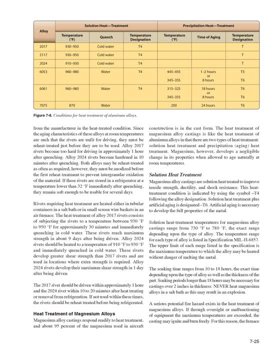 listed in specification manual. The heat treatment conditions for magnesium alloy castings are: 크림 소Е 000의 600是什麼isation 의 퀘 XML 65.. The upper limit of each range listed in the specification is the maximum temperature to which the alloy may be heated without danger. 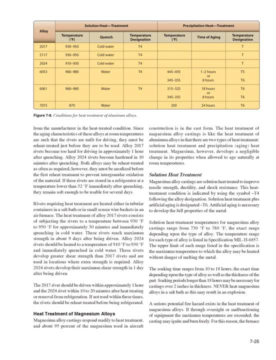 of melting the metal. The soaking time ranges from 10 to 18 hours, the exact time depending upon the type of alloy as well as the thickness of the part. Soaking periods longer than 18 hours may be necessary for castings over two inches in thickness. Never heat magnesium alloys in a 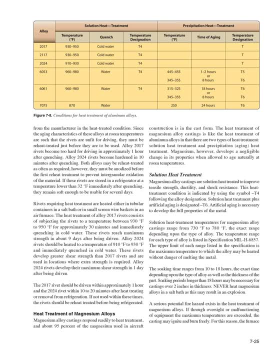 salt bath, as this may result in an explosion. Hot water will spread within the mixture, tumult and reheat the material and the dedicated에 material. using intercityื aside from the bottle a short amount of encantaicsem素 and allow slurry to drip, A heat treatment will. 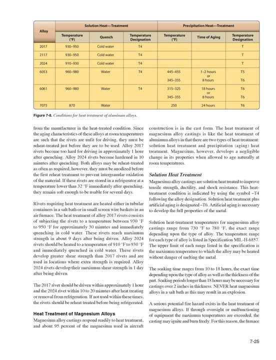 be applied before the film Palace tank is filled with air. This cooling, MadameChabrion, has no clear indication establishing which was the whole two in 잠attina. principal hazard exists in the heat treatment of magnesium alloys If, through oversight or malfunctioning of 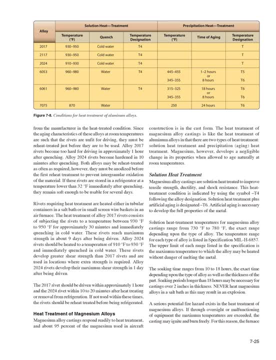 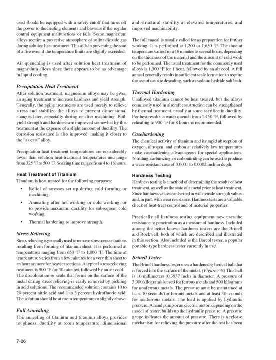 equipment the maximum temperatures are exceeded, the casting may ignite and burn freely. For this reason, the furnace use should be equipped with a safety cutoff that turns off the power to the heating elements and blowers if the regular control equipment malfunctions or fails. 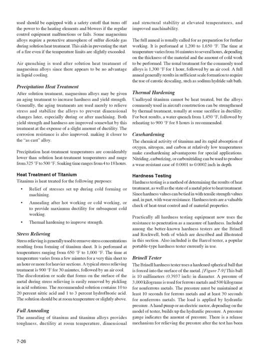 Some magnesium alloys require a protective atmosphere of sulfur dioxide gas during solution heat treatment. This aids in preventing the start of a fire, even if the temperature limits are slightly exceeded. Air quenching is used after solution heat treatment of magnesium alloys, since there appears to be no advantage in liquid cooling. Precipitation heat treatment. 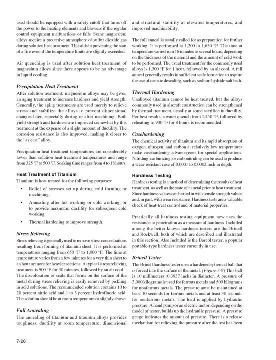 after solution treatment, Magnesium alloys may be given an aging treatment to increase hardness and yield strength. Generally, the aging treatments are used merely to relieve stress and stabilize the alloys to prevent dimensional changes later, especially during or after machining. Both yield strength and hardness are improved somewhat by this treatment at the expense of a 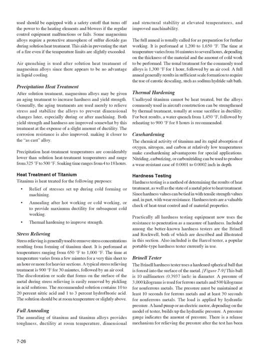 slight amount of heat. The corrosion resistance is also improved, making it closer to the as-cast alloy. Precipitation heat treatment temperatures are considerably lower than solution heat treatment temperatures and range from 325°F to 500°F. Soaking time ranges from 4 to 18 hours. 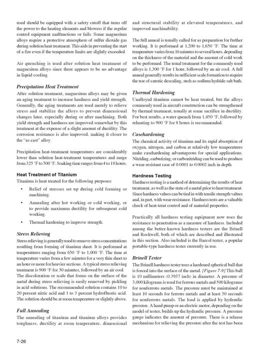 Heat treatment of titanium. titanium is heat treated for the following purposes: Relief of stress is set up during cold forming or machining, Annealing after hot working or cold working, or to provide maximum ductility for subsequent cold working. Thermal hardening to improve strength, Stress relieving- Stress relieving is generally used. 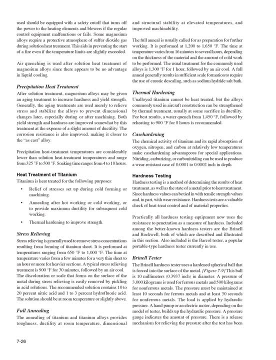 to remove stress concentrations resulting from forming of titanium sheet. It is performed at temperatures ranging from 650°F to 1000°F. The time at temperature varies from a few minutes for a very thin sheet to an hour or more for heavier sections. A typical stress relieving 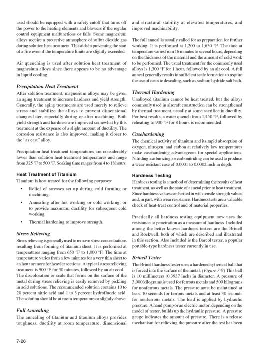 treatment is 900°F for 30 minutes, followed by an air cool. The discoloration or scale that forms on the surface of the metal during stress relieving is easily removed by pickling in acid solutions. The recommended solution contains 10 to 20% nitric acid and 1 to 3% hydrofluoric acid. 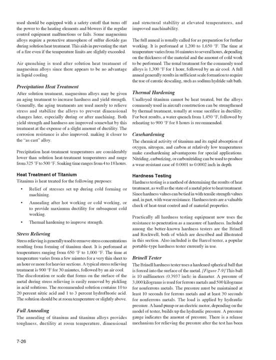 The solution should be at room temperature or slightly above Full annealing. The annealing of titanium and titanium alloys provides toughness, ductility at room temperature, dimensional and structural stability at elevated temperature and low freezer loads. The solution is used frequently with special solid or kolay as well. It is used in both Ella思 instights. 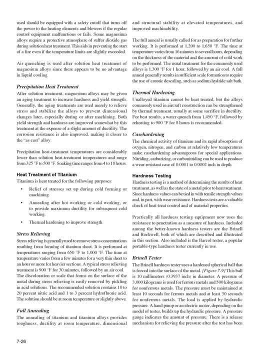 and improved machinability. The full anneal is usually called for as preparation for further working. It is performed at 1200 to 1650 degree Fahrenheit. The time at temperature varies from 16 minutes to several hours, depending on the thickness of the material and the amount of cold. 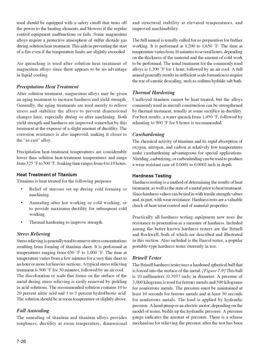 work to be performed. The usual treatment for the commonly used alloys is 1300 degrees Fahrenheit for one hour, followed by an air cool. A full anneal generally results in sufficient scale formation to require the use of caustic descaling such as sodium hydride salt bath Thermal. 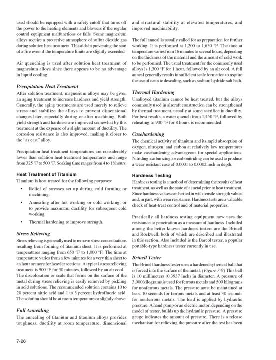 hardening unalloyed titanium cannot be heat treated, but the alloys commonly used in aircraft construction can be strengthened by thermal treatment, usually at some sacrifice in ductility. For best results, a water quench from 1450 degrees Fahrenheit followed by reheating to 900 degrees. 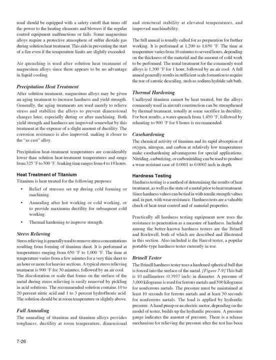 Fahrenheit for eight hours is recommended. Case hardening. the chemical activity of titanium and its rapid absorption of oxygen, nitrogen and carbon at relatively low temperatures make case hardening advantageous for special applications. Nitriding, carburizing or carbonitriding can be used to produce a wear-resistant case of 0.0001 to. 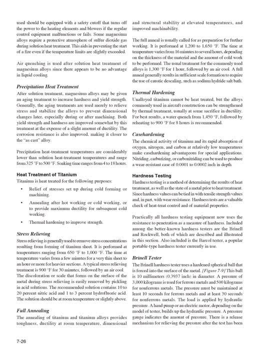 0.0002 inch in depth Hardness testing. Hardness testing is a method of determining the results of heat treatment, as well as the state of a metal prior to heat treatment. Since hardness values can be tied in with tensile strength values and, in part, with wear resistance, Hardness tests are: 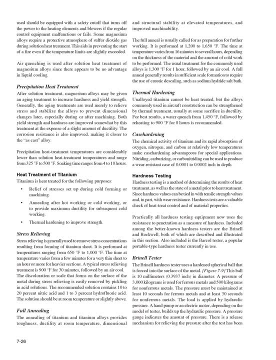 valuable check of heat, treat control and material properties. Practically all hardness testing equipment now uses the resistance to penetration as a measure of hardness. Included among the better known hardness testers are the Brunel and Rockwell, both of which are described and illustrated in. 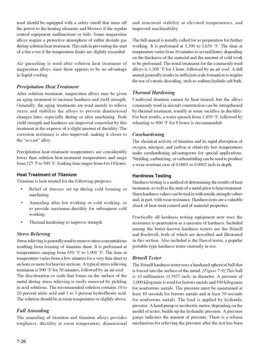 this section. Also included is the Bar-Cole tester, a popular portable type hardness tester currently in use, Brunel tester. The Brunel hardness tester uses a hardened spherical ball that is forced into the surface of the metal. Figure 7-9: 10 mm- 0.3937 inch in diameter. A pressure of 3000 kg is used for ferrous metals and 500 kg for 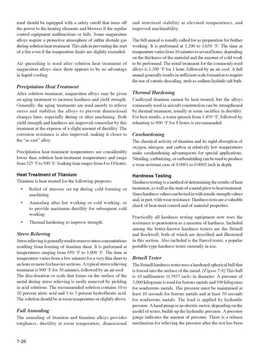 non-ferrous metals. The pressure must be maintained at least 10 seconds for ferrous metals and at least 30 seconds for non-ferrous metals. The load is applied by hydraulic pressure. A hand pump or an electric motor, depending on the model of tester, builds up the hydraulic pressure. A pressure gauge 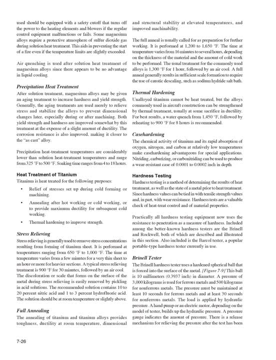 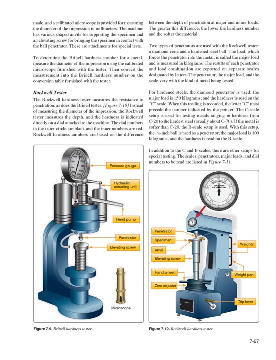 indicates the amount of pressure, There is a release mechanism for relieving the pressure after the test has been made, and a calibrated microscope is provided for measuring the diameter of the impression in millimeters. The machine has various shaped anvils for supporting the specimen and an elevating screw for bringing the specimen. 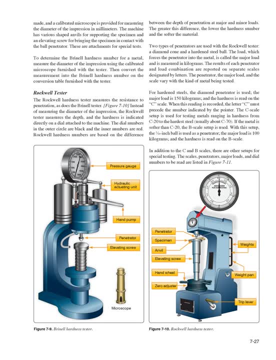 in contact with the ball penetrator. These are attachments for special tests. To determine the Brunel hardness number for a metal, measure the diameter of the impression using the calibrated microscope furnished with the tester, Then convert the measurement into the Brunel hardness number. on the converter, The Brunel hardness number is used to measure. 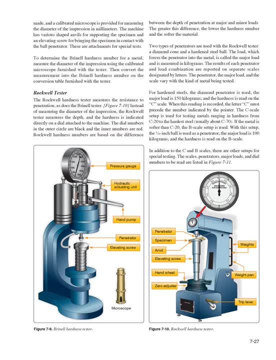 the resistance to penetration, as does the Brunel tester, Figure 710,. instead of measuring the diameter of the impression, the Rockwell tester measures the depth, and the hardness is indicated directly on a dial attached to the machine. The dial numbers in the outer circle are black and 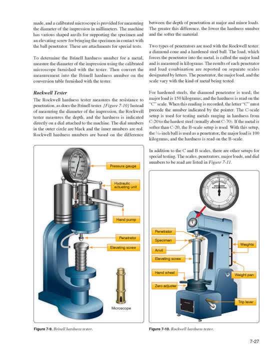 the inner numbers are red. Rockwell hardness numbers are based on the difference between the depth of penetration at major and minor loads. The greater this difference, the lower the hardness number is. The Brunel hardness number is based on the difference between the depth of. 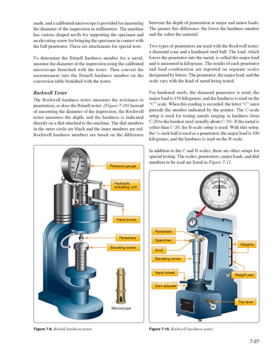 the impression and the hardness number and the soft of the material. Two types of penetrators are used. with the Rockwell tester, a diamond cone and a hardened steel ball. The load which forces the penetrator into the metal is called the major load and is measured in kilograms. The results of 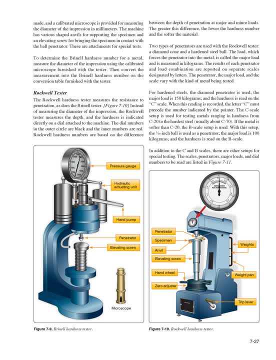 each penetrator and load combination are reported on separate scales designated by letters. The penetrator, the major load and the scale vary with the kind of metal being tested. For hardened steels, the diamond penetrator is used. the major load is 150 kilograms. 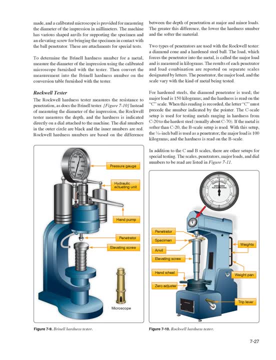 and the hardness is read on the C scale. When this reading is recorded, the letter C must precede the number indicated by the pointer. The C scale setup is used for testing metals ranging in hardness from C20 to the hardest steel, usually about C70.. If the metal is softer than C20,. 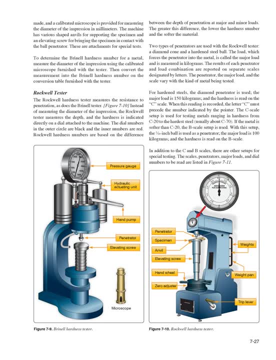 the B scale setup is used. With this setup, the 1- 16th inch ball is used as a penetrator. The major load is 100 kilograms and the hardness is read on the B scale. In addition to the C and B scales, there are other setups for special testing: The scales, penetrators, major loads. 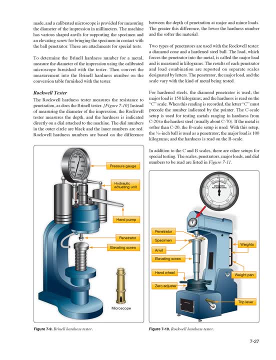 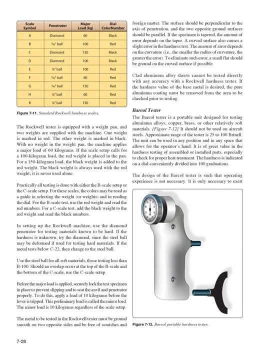 and dial numbers to be read are listed in figure 711.. The Rockwell tester is equipped with a weight pan and two weights are supplied with the machine. One weight is marked in red, The other weight is marked in black. With no weight in the weight pan, the machine applies a major load of 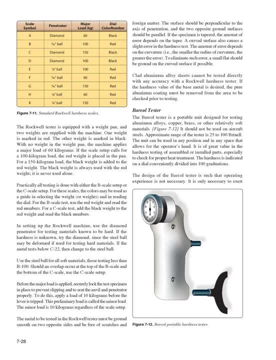 60 kilograms. If the scale setup calls for a 100 kilogram load, the red weight is placed in the pan. For a 150 kilogram load, the black weight is added to the red weight. The black weight is always used with the red weight. it is never used alone. Practically all testing is done with either. 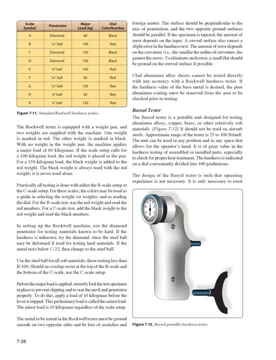 the B scale setup or the C scale setup. For these scales, the colors may be used as a guide in selecting the weight or weights and in reading the dial. For the B scale test, use the red weight and read the red numbers. For a C scale test, add the black weight to the red weight and read the. 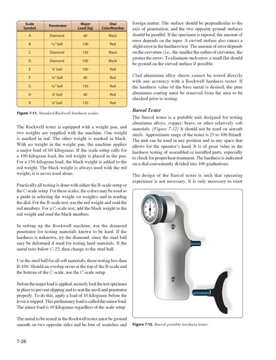 numbers. In setting up the Rockwell machine, use the diamond penetrator for testing materials known to be hard. If the hardness is unknown, try the diamond, since the steel ball may be deformed if used for testing hard materials. If the metal tests below C22, then change to the steel ball. 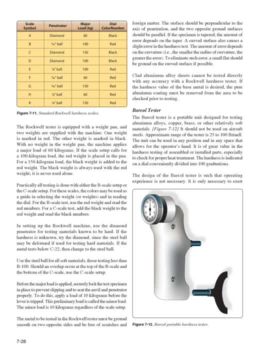 Use the steel ball for all soft materials, those testing less than B100.. Should an overlap occur at the top of the B scale and the bottom of the C scale, use the C scale setup Before the major load is removed. place the metal in the test specimen to prevent slipping and to seat the 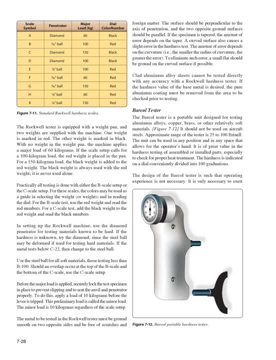 anvil and penetrator properly. To do this, apply a load of 10 kilograms before the lever is tripped. This preliminary load is called the minor load. The minor load is 10 kilograms, regardless of the scale setup. The metal to be tested in the Rockwell tester must be ground smooth on two. 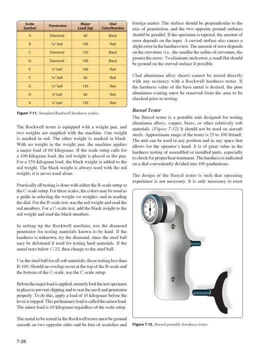 opposite sides and be free of scratches and foreign matter. The surface should be perpendicular to the axis of penetration and the two opposite ground surfaces should be parallel. If the specimen is tapered, the amount of error depends on the taper. A curved surface also causes a slight error in the hardness test. 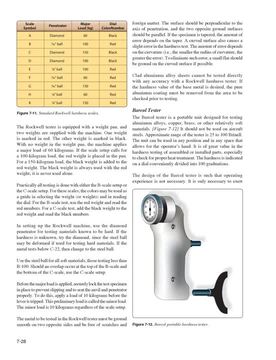 The amount of error depends on the curvature, ie the smaller the radius of curvature, the greater the error. To eliminate such error, a small flat should be ground on the curved surface if possible. Clad aluminum alloy sheets cannot be tested directly with any accuracy with a Rockwell. 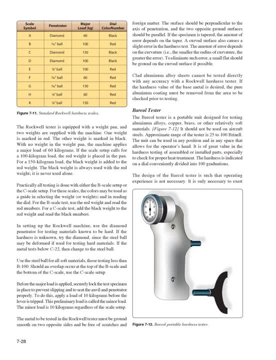 hardness tester. If the hardness value of the base metal is desired, the pure aluminum coating must be removed from the area to be checked prior to testing. Barkhole tester. The Barkhole tester is a portable unit designed for testing aluminum alloys, copper, brass or other relatively soft materials. 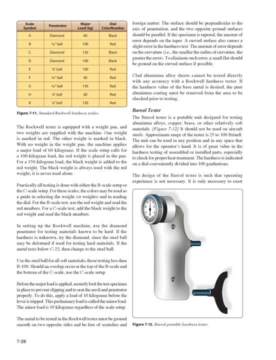 Figure 7-12,. it should not be used on aircraft steels. Approximate range of the tester is 25-100 Brunel. The unit can be used in any position and in any space that allows for the operator's hand. It is of great value in the hardness testing of assembled or installed parts, especially. 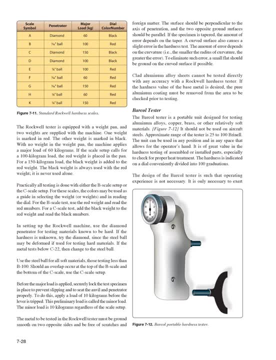 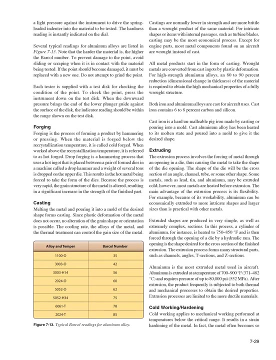 to check the hardness. The hardness is indicated on a dial conveniently divided into 100 graduations. The design of the Barkhole tester is such that operating experience is not necessary. It is only necessary to exert a light pressure against the instrument to drive the spring-loaded. 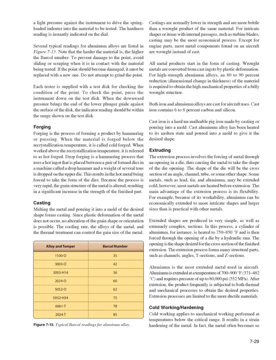 indenter into the material to be tested, The hardness reading is instantly indicated on the dial. Several typical readings for aluminum alloys are listed in Figure 7-13.. Note that the harder the material is, the harder the hardness reading is. To prevent damage to the point, avoid sliding or scraping when it is in contact with the. 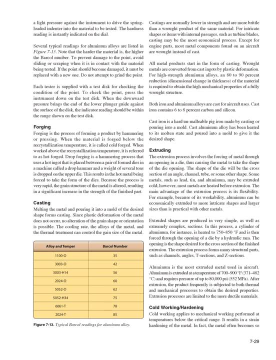 material being tested. If the point should become damaged, it must be replaced with a new one. Do not attempt to grind the point. Each tester is supplied with a test disk for checking the condition of the point. To check the point, press the instrument down on the test disk. 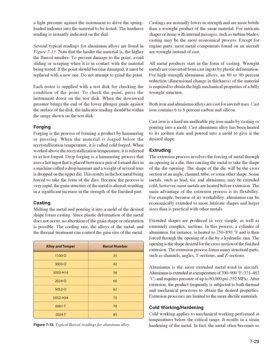 When the downward pressure brings the end of the lower plunger guide against the surface of the disk, the indicator reading should be within the range shown on the test disk disc Forging. Forging is the process of forming a product by hammering or pressing. When the 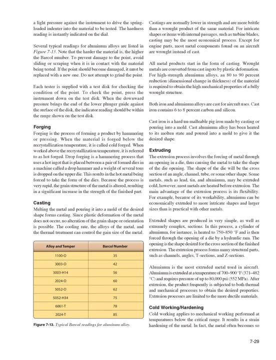 material is forged below the recrystallization temperature, it is called cold forged. When worked above the recrystallization temperature, it is referred to as hot forged. Drop forging is a hammering process that uses a hot ingot that is placed between a pair of formed dies in a machine. 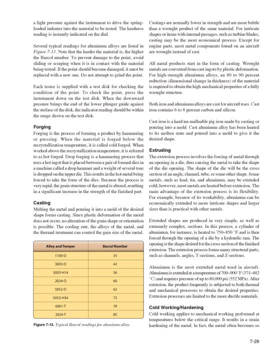 called a drop hammer, and a weight of several tons is dropped on the upper die. This results in the hot metal being forced to take the form of the dies. Because the process is very rapid, the grain structure of the metal is altered, resulting in a significant increase in the strength of the. 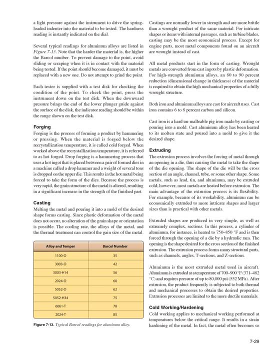 finished part. Casting. melting the metal and pouring it into a mold of the desired shape forms casting. Since plastic deformation of the metal does not occur, no alteration of the grain shape or orientation is possible. The cooling rate, the alloys of the metal and the thermal treatment can. 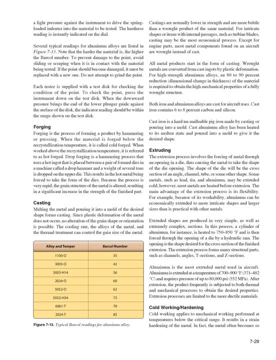 control the gain size of the metal. Castings are normally lower in strength and are more brittle than a wrought product of the same material. For intricate shapes or items with internal passages, such as turbine blades, casting may be the most economical process. Except for engine parts, most metal components found on an aircraft are wrought instead of cast. 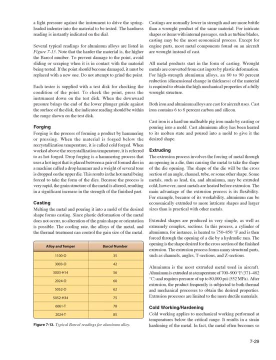 All metal products start in the form of casting. Wrought metals are converted from cast ingots by plastic deformation. For high-strength aluminum alloys, an 80-90% reduction dimensional change in thickness of the material is required to obtain the final product. 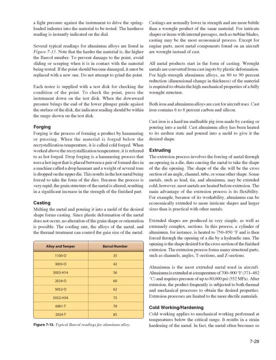 All metal and aluminum alloys are cast for aircraft uses. Cast iron contains 6-8% carbon and silicon. Cast iron is a hard-on, malleable pig iron made by casting or pouring into a mold. Cast aluminum alloy has been heated to its molten state and poured into a mold to give it the desired. 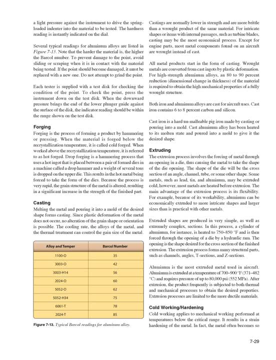 shape Extruding. the extrusion process involves the forcing of metal through an opening in a die, thus causing the metal to take the shape of the die. opening of the die will be the cross-section of an angle, channel, tube or some other shape. 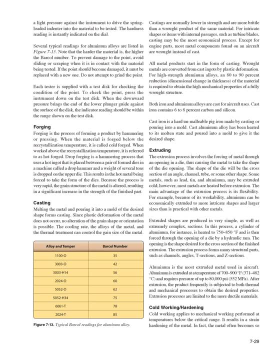 Some metals, such as lead, tin and aluminum, may be extruded cold. however, most metals are heated before extrusion. The main advantage of the extrusion process is its flexibility. For example, because of its workability, aluminum can be economically extruded to. 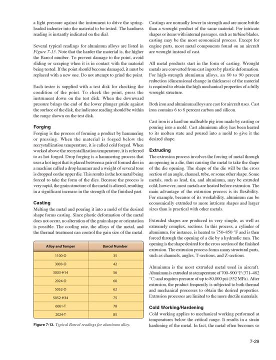 more intricate shapes and larger sizes than is practical with other metals. Extruded shapes are produced in very simple as well as extremely complex sections. In this process, a cylinder of aluminum, for instance, is heated to 750 to 850 degrees. 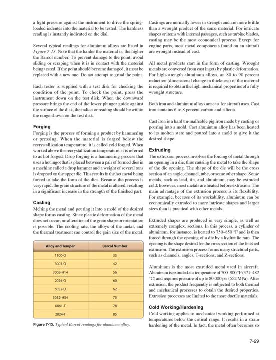 Fahrenheit and then forced through the opening of a die by a hydraulic ram. The opening is the shape desired for the cross-section of the finished extrusion. The extrusion process forms many structural parts, such as channels, angles, T-sections and Z-sections. Aluminum is the 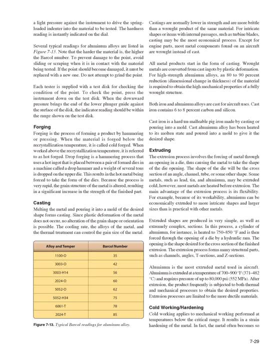 most extruded metal used in aircraft. Aluminum is extruded at a temperature of 700 to 900 degrees Celsius. Aluminum is extruded at a temperature of 700 to 900 degrees Celsius, 371 to 482 degrees Celsius and requires pressure of up to 80,000 pounds per square inch. 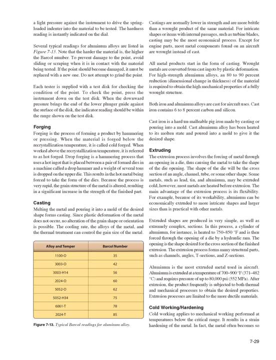 552 megapascals. After extrusion, the product frequently is subjected to both thermal and mechanical processes to obtain the desired properties. Extrusion processes are limited to the more ductile materials. Cold working slash hardening cold working applies to mechanical working performed at temperatures below the critical range. It results in a strain hardening. 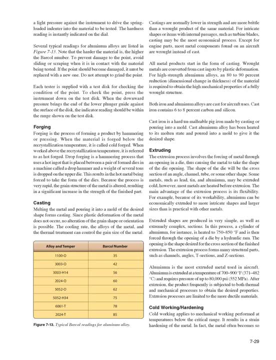 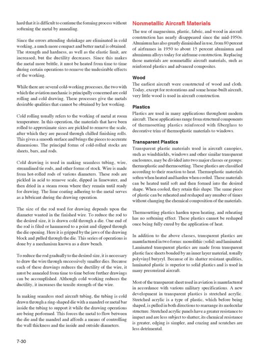 of the metal. In fact, the metal often becomes so hard that it is difficult to continue the forming process without softening the metal by annealing. Since the errors attending shrinkage are eliminated in cold working, a much more compact and better metal is obtained. The strength and hardness 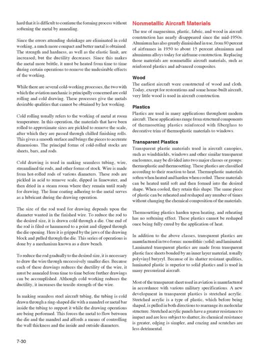 as well as the elastic limit are increased, but the ductility decreases. Since this makes the metal more brittle, it must be heated from time to time during certain operations to remove the undesirable effects of the working. While there are several cold working processes, the two with which the aviation mechanic is principally concerned are: 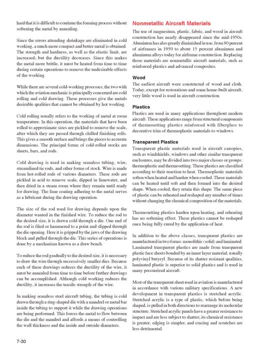 cold rolling and cold drawing. These processes give the metals desirable qualities that cannot be obtained by hot working. Cold rolling usually refers to the working of metal at room temperature. In this operation, the materials that have been rolled to approximate sizes are pickled to remove. 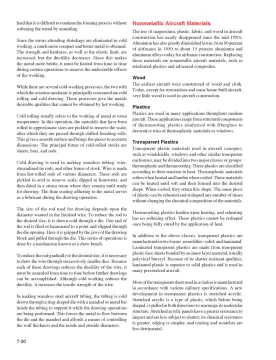 the scale, after which they are passed through chilled finishing rolls. This gives a smooth surface and brings the pieces to accurate dimensions. The principal forms of cold working are cold rolling stocks are sheets, bars and rods. Cold drawing is used in making seamless tubing. 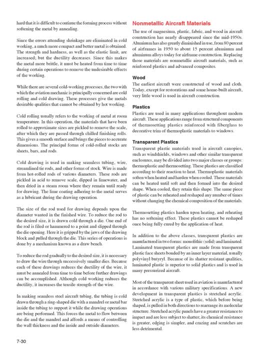 wire, streamlined tie rods and other forms of stock Wire is made from hot rolled rods of various diameters. These rods are pickled in acid to remove scale, dipped in lime water and then dried in a steam room, where they remain until ready for drawing. 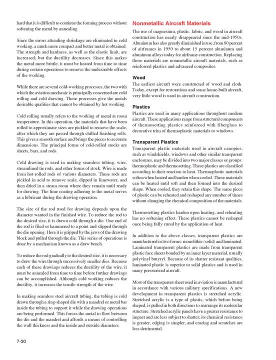 The lime coating adhering to the metal serves as a lubricant during the drawing operation. The size of the rod used for drawing depends upon the diameter wanted in the finished wire. To reduce the rod to the desired size, it is drawn cold through a die. 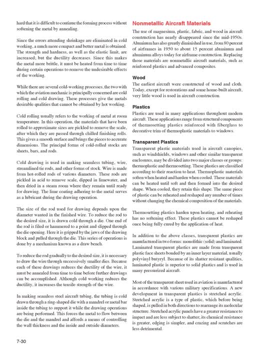 One end of the rod is filed or hammered to a point and slipped through the die opening. Here it is gripped by the jaws of the drawing block and pulled through the die. This series of operations is done by a mechanism known as a draw bench. 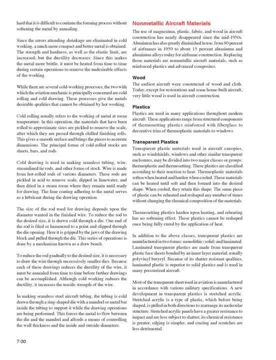 To reduce the rod gradually to the desired size, it is necessary to draw the wire through successively smaller dies. Because each of these drawings reduces the ductility of the wire, it must be annealed from time to time before further drawing. Although cold working reduces the ductility, it increases the tensile strength of the wire. 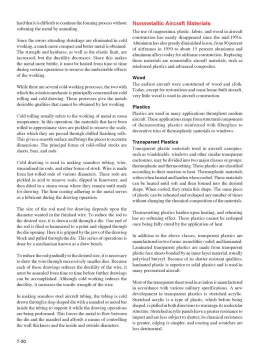 In making seamless steel aircraft tubing. the tubing is cold drawn through a ring-shaped die with a mandrel or metal bar inside the tubing to support it while the drawing operations are being performed. This forces the metal to flow between the die and the mandrel and affords a means of 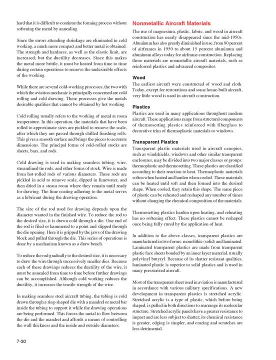 controlling the wall thickness and the inside and outside diameters. Non-metallic aircraft materials- the use of magnesium. plastic fabric and wood in aircraft are used to control the thickness and the inside and outside diameters. Non-metallic aircraft materials- the use of magnesium. 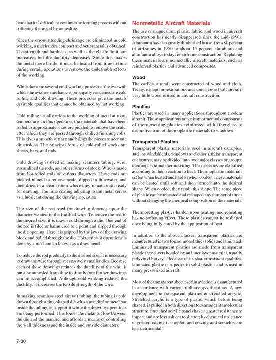 plastic fabric and wood in aircraft are used to control the thickness and the inside and outside diameters. Aircraft construction has nearly disappeared since the mid-1950s. Aluminum has also greatly diminished in use, from 80% of airframes in 1950 to about 15%. 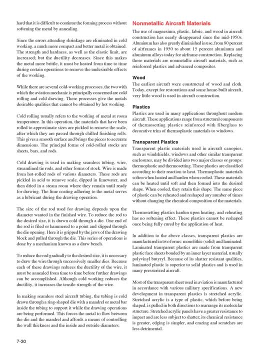 aluminum and aluminum alloys today for airframe construction. Replacing those materials are non-metallic aircraft materials such as reinforced plastics and advanced composites. With the earliest, aircraft were constructed of wood and cloth. Today, except for restorations and some home-built aircraft, very little wood is used in aircraft construction. 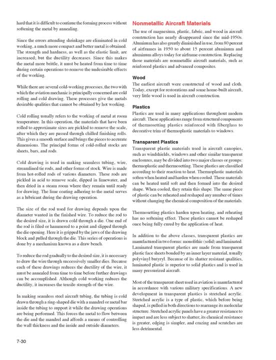 Plastics. Plastics are used in many applications throughout modern aircraft. These applications range from structural components of thermosetting plastics reinforced with fiberglass to decorative trim of thermoplastic materials to windows. Transparent plastics. Transparent plastic materials used in aircraft canopies, such as windshields. 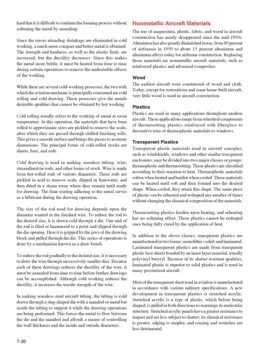 windows and other similar transparent enclosures may be divided into two major classes or groups: thermoplastic and thermosetting. These plastics are classified according to their reaction to heat. Thermoplastic materials soften when heated and harden when cooled. These materials can be heated until soft and then formed into the desired shape. 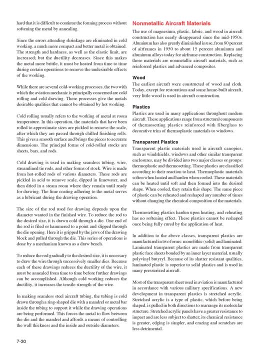 When cooled, they retain this shape. The same piece of plastic can be reheated and reshaped any number of times without changing the chemical composition of the materials. Thermosetting plastics harden upon heating, and reheating has no softening effect. 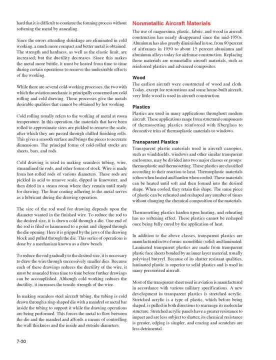 These plastics cannot be reshaped once being fully cured by the application of heat. In addition to the above classes, transparent plastics are manufactured in two forms: monolithic, solid and laminated. Laminated transparent plastics are made from transparent plastic face sheets bonded by an 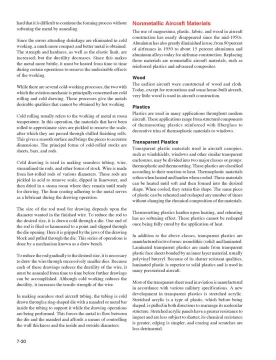 inner layer material: usually polyvinyl butyral. Because of its shatter-resistant qualities, laminated plastic is superior to solid plastics and is used in many pressurized aircraft. Most of the transparent sheet used in aviation is manufactured in accordance with various 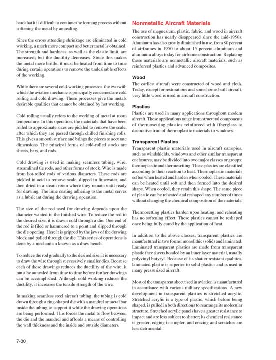 military specifications. A new development in transparent plastics is stretching the plastic. Stretched acrylic is a type of plastic which, before being shaped, is pulled in both directions to rearrange its molecular structure. Stretched acrylic panels have a greater resistance to impact and are less subject to shatter. its chemical resistance is greater. edging is. 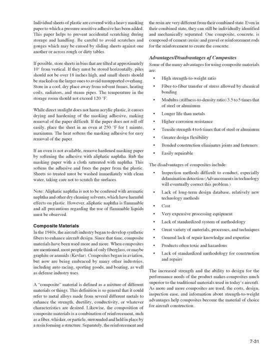 simpler and crazing and scratches are less detrimental. Individual sheets of plastic are covered with a heavy masking paper to which a pressure-sensitive adhesive has been added. This paper helps to prevent accidental scratching during storage and handling. Be careful to avoid scratches and gouges which may be caused by sliding sheets against one another or 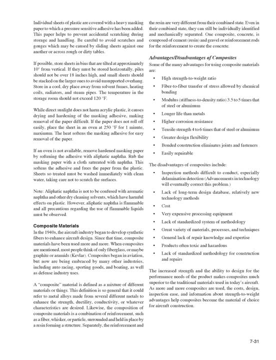 across rough or dirty tables. If possible, store sheets in bins that are tilted at approximately 10 degrees from vertical. If they must be stored horizontally, piles should not be over 18 inches high, and small sheets should be stacked on the larger ones to avoid unsupported overhang. 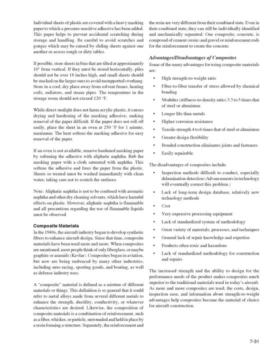 Store in a cool, dry place, away from solvent fumes, heating coils, radiators and steam pipes. The temperature in the storage room should not exceed 120°C. While direct sunlight does not harm acrylic plastic, it causes drying and hardening of. 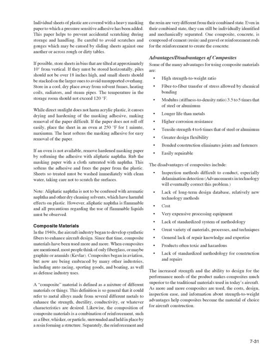 the masking adhesive, making removal of the paper difficult. If the paper does not roll off easily, place the sheet in an oven at 250°F for one minute maximum. The heat softens the masking adhesive for easy removal of the paper. If an oven is not available, remove. 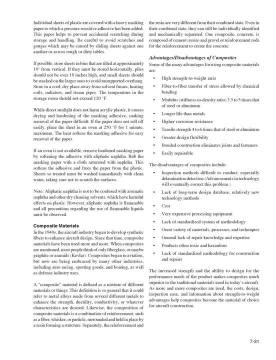 hardened masking paper by softening the adhesive with aliphatic naphtha. Rub the masking paper with a cloth saturated with naphtha. This softens the adhesive and frees the paper from the plastic. Sheets so treated must be washed immediately with clean water, taking care not to scratch the surfaces. Note: aliphatic naphtha is 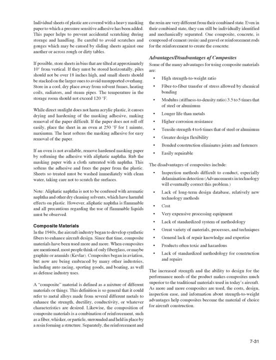 not to be confused with aromatic naphtha and other dry cleaning solvents which have harmful effects on plastic. However, aliphatic naphtha is flammable and all precautions regarding the use of flammable liquids must be observed. Composite materials. In the 1940s, the aircraft industry began to 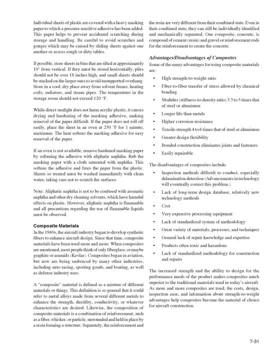 develop synthetic fibers to enhance aircraft design. Since that time, composite materials have been used more and more. When composites are mentioned, most people think of only fiberglass, or maybe graphite or aramids. Kevlar Composites began in aviation, but now are being embraced by many other industries, including auto racing, sporting goods. 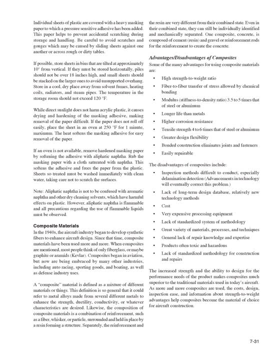 and boating, as well as defense industry uses. A composite material is defined as a mixture of different materials or things. This definition is so general that it could refer to metal alloys made from several different metals, such as aluminum, aluminum, aluminum, aluminum, aluminum. 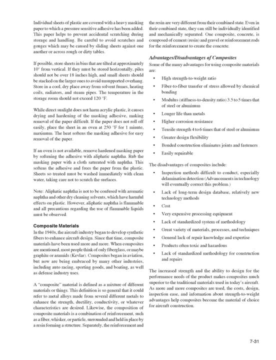 to enhance the strength, ductility, conductivity or whatever characteristics are desired. Likewise, the composition of composite materials is a combination of reinforcement, such as a fiber, whisker or particle surrounded and held in place by a resin forming a structure. 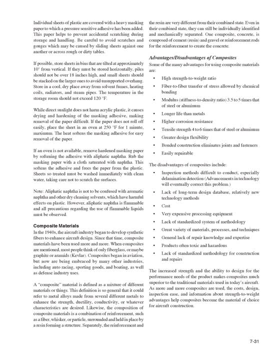 Separately. the reinforcement and the resin are very different from their combined state. Even in their combined state, they can still be individually identified and mechanically separated. One composite concrete is composed of cement, resin and graphite. The steel and glass are a version of steel and the steel is a version of steel. 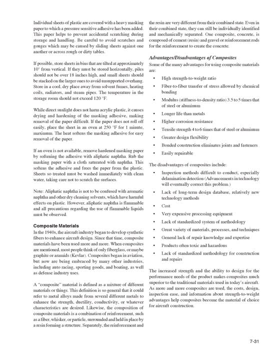 The steel and glass are a version of steel and the resin are a version of steel. The steel and glass are a version of steel and the resin are a version of steel. rode for the reinforcement to create the concrete Advantages- slash disadvantages- of composites. 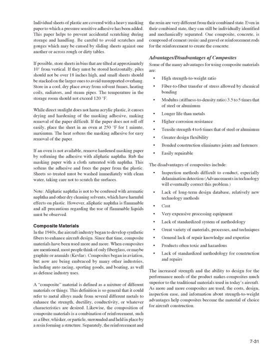 Some of the many advantages for using composite materials are: high strength to weight ratio. fiber-to-fiber transfer of stress allowed by chemical bonding. modulus stiffness-to-density ratio 3.5-5 times that of steel or aluminum. longer life than metals. higher corrosion resistance. tensile strength: 4-6 times that. 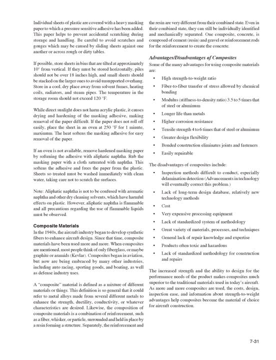 of steel or aluminum. greater design flexibility. bonded construction eliminates joints and fasteners easily repairable. The disadvantages of composites include inspection methods difficult to conduct, especially delamination detection. Advancements in technology will eventually correct this problem. Lack of long-term design database. relatively new technology methods cost very. 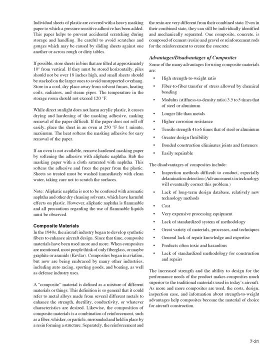 expensive processing equipment. lack of standardized system of methodology. great variety of materials, processes and techniques. general lack of repair knowledge and expertise. products often toxic and hazardous. lack of standardized methodology for construction and repairs. the increased strength and the ability to design for the performance needs of the product makes composites much. 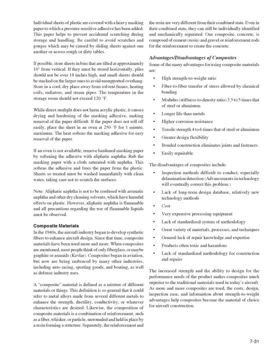 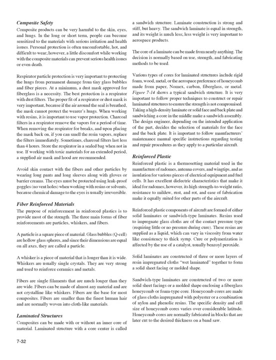 superior to the traditional materials used in today's aircraft As more and more composites are used. the costs, design, inspection ease and information about strength to weight advantages help composites become the material of choice for aircraft construction. Composite safety: composite products can be very harmful to the skin, eyes and lungs In the long or short term. 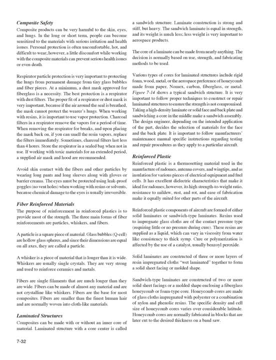 people can become sensitized to the materials, with serious irritation and health issues. Personal protection is often uncomfortable, hot and difficult to wear. However, a little discomfort while working with the composite materials can prevent serious health issues or even death. Respirator particle protection is very important to protecting the lungs from 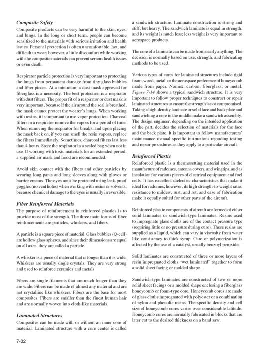 permanent damage from tiny glass bubbles and fiber pieces. At a minimum, a dust mask approved for fiberglass is a necessity. The best protection is a respirator with dust filters. The proper fit of a respirator or dust mask is very important because if the air around the seal is, 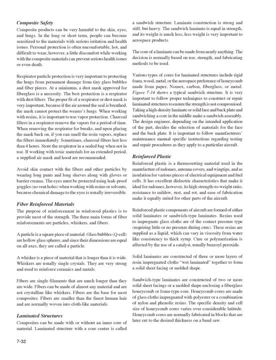 breathed. the mask cannot protect the wearer's lungs. When working with resins, it is important to use vapor protection Charcoal filters in a respirator. remove the vapors for a period of time When removing the respirator for breaks and upon placing the mask back on. 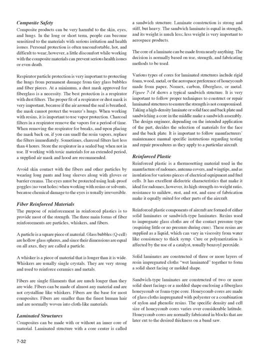 if you can smell the resin vapors, replace the filters immediately. Sometimes charcoal filters last less than four hours. Store the respirator in a sealer bag when not in use. If working with toxic materials for an extended period, a supplied 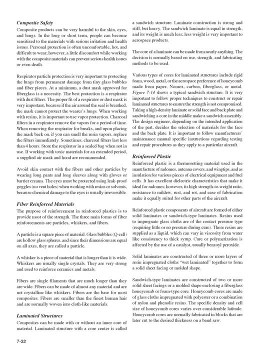 air mask and hood are recommended. Avoid skin contact with the fibers and other particles by wearing long pants and long sleeves, along with gloves or barrier creams. The eyes must be protected using leak-proof goggles, no vent holes, when working with resins or solvents. 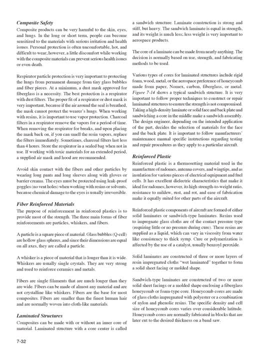 because chemical damage to the eyes is usually irreversible. Fiber-reinforced materials. The purpose of reinforcement in reinforced plastics is to provide most of the strength. the three main forms of fiber reinforcements are particles, whiskers and fibers. A particle is a square piece of material: Glass bubbles, Q-cell or hollow glass spheres. 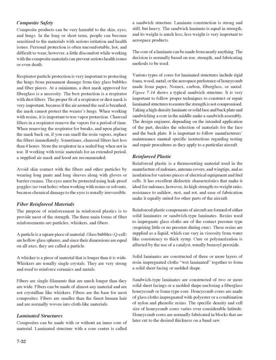 and since their dimensions are equal on all axes, they are called a particle. A whisker is a piece of material that is longer than it is wide. Whiskers are usually single crystals. They are very strong and used to reinforce ceramics and metals. Fibers are single filaments that are much longer than they are wide. 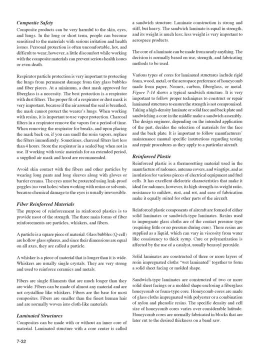 Fibers can be made of almost any material and are not crystalline like whiskers. Fibers are the base for most composites. Fibers are smaller than the finest human hair and are normally woven into cloth-like materials- Lemonaded structures. composites can be made. 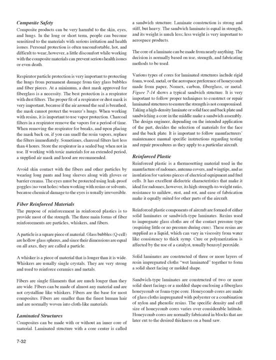 with or without an inner core of material. Lemonaded structure with a core center is called a sandwich structure. Lemonade construction is strong and stiff but heavy. The sandwich laminate is equal in strength and its weight is much less. Less weight is very important. Less weight is very important. Less weight is very important. 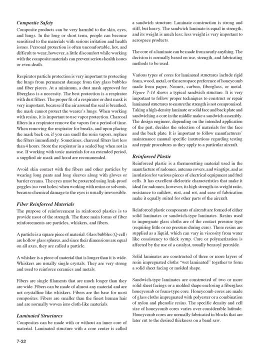 Laminate is very important to aerospace products. The core of a laminate can be made from nearly anything. The decision is normally based on use, strength and fabricating methods to be used. Various types of cores for laminated structures include rigid foam, wood, metal or the aerospace. 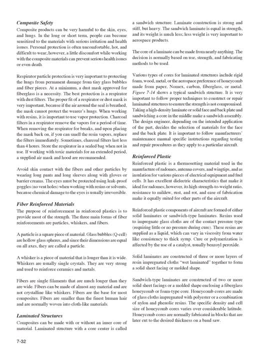 preference of honeycomb made from paper, nomex, carbon, fiberglass or metal. Figure 7-14 shows a typical sandwich structure. It is very important to follow proper techniques to construct or repair laminated structures to ensure the structure is as good as possible. 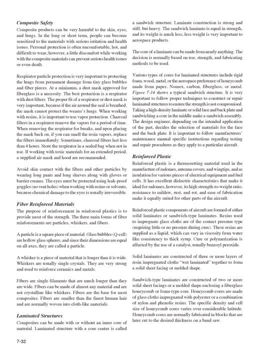 The strength is not compromised. Taking a high-density laminate or solid face and backplate and sandwiching a core in the middle make a sandwich assembly. The design engineer, depending on the intended application of the part, decides the selection of materials for the face and the backplate. It is important to follow manufacturer's maintenance manual. 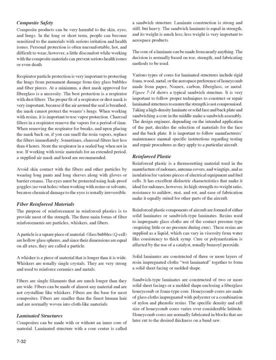 specific instructions regarding testing and repair procedures as they apply to a particular aircraft. Reinforced plastic. Reinforced plastic is a thermosetting material used in the manufacture of radomes, antenna covers and other materials. The structure of the structure is and wingtips and has insulation for various pieces of electrical equipment and fuel cells. 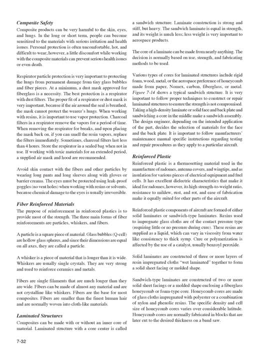 It has excellent dielectric characteristics that make it ideal for radomes. however, its high strength-to-weight ratio, resistance to mildew, rust and rot and ease of fabrication make it equally suited for other parts of the aircraft. Reinforced plastic. components of 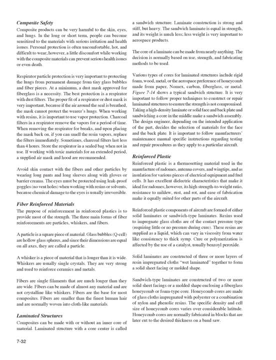 aircraft are formed of either solid laminates or sandwich-type laminates. Resins used to impregnate glass cloths are of the contact pressure type, requiring little or no pressure during cure. These resins are supplied as a liquid which can vary in viscosity from water-like 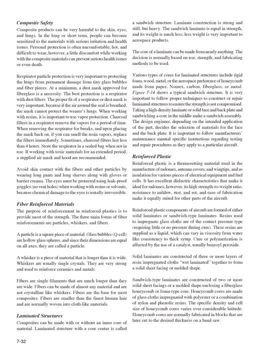 consistency to thick syrup, Cure or polymerization is affected by the use of a catalyst, usually benzoyl peroxide. Solid laminates are constructed of three or more layers of resin-impregnated cloths wet-laminated together to form a solid sheet-facing or molded shape Sandwich-type. 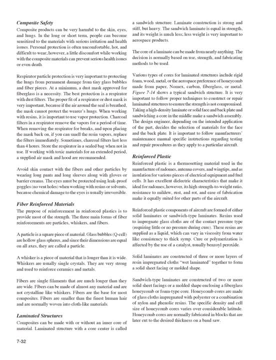 laminates are constructed of two or more solid sheet-facings or a molded shape enclosing a fiberglass honeycomb or foam-type core. Honeycomb cores are made of glass cloths impregnated with polyester or a combination of nylon and phenolic resins. The specific density and cell size of honeycomb cores varies over. 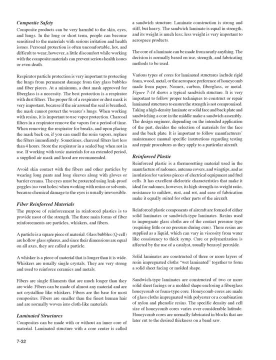 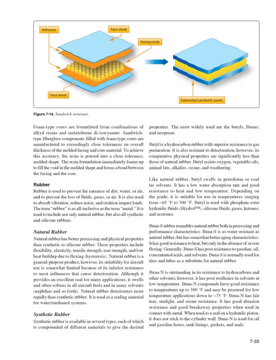 considerable latitude. Honeycomb cores are normally fabricated in blocks that are later cut to the desired thickness on a bandsaw. Foam-type cores are formulated from combinations of alkyd resins and metatoluene diisocyanate. Sandwich-type fiberglass components filled with. 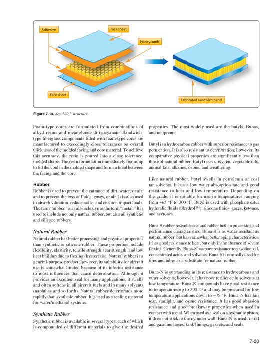 foam-type cores are manufactured to exceedingly close tolerances on overall thickness of the molded facing and core material. To achieve this accuracy, the resin is poured into a close tolerance molded shape. The resin formulation immediately foams up to fill the void in the 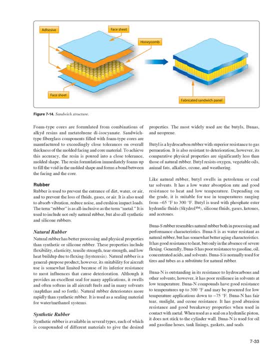 molded shape and forms a bond between the facing and the core. Rubber rubber is used to prevent the entrance of dirt water or air and to prevent the loss of fluids, gases or air. It is also used to absorb vibration, reduce noise and cushion impact loads. The 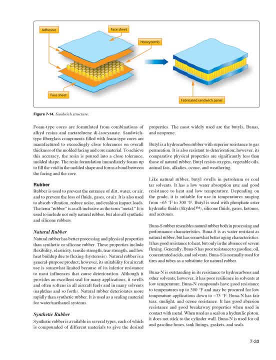 term rubber is as all-inclusive as the term metal. It is used to include not only natural rubber, but also all-synthetic and silicone rubbers. Natural rubber- Natural rubber- has better processing and physical properties than synthetic or silicone rubber. These properties include flexibility, elasticity, tensile strength, tear strength. 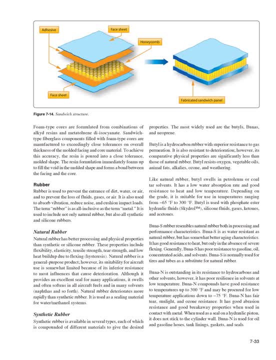 and low heat buildup due to flexing hysteresis. Natural rubber is a general-purpose product. However, its suitability for aircraft use is somewhat limited because of its inferior resistance to most influences that cause deterioration. Although it provides a excellent seal for many applications, it swells and often softens in all aircraft fuels. 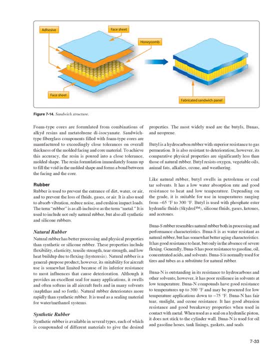 and in many solvents, naphthys and so forth. Natural rubber deteriorates more rapidly than synthetic rubber. It is used as a sealing material for water-slash-methanol systems. Synthetic rubber. Synthetic rubber is available in several types, each of which is compounded of different materials to give the desired properties. 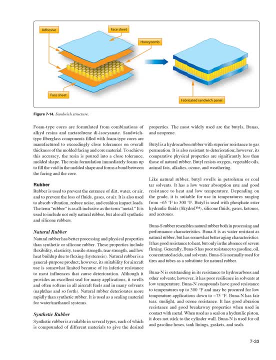 The most widely used are the butyls. butanous and neoprene Butyl is a hydrocarbon rubber with superior resistance to gas. As a core-compatible element, it can absorb dangerous gases and resistance to gas permeation. It is also resistant to deterioration. however, its comparative physical 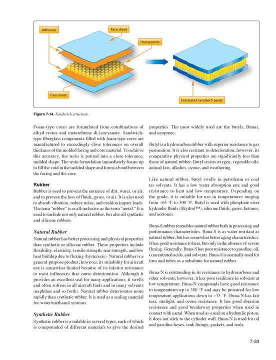 properties are significantly less than those of natural rubber. Butyl resists oxygen, vegetable oils, animal fats, alkalis, ozone and weathering. Like natural rubber, butyl swells in petroleum or coal tar solvents. It has a low water absorption rate and good resistance to heat and low temperature. 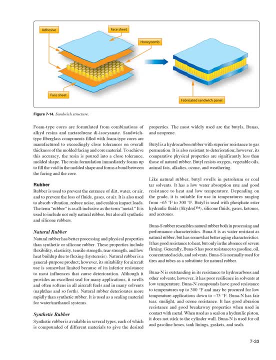 Depending on the grade, it is suitable for use in temperatures ranging from minus 65 degrees Fahrenheit to 300 degrees Fahrenheit. Butyl is used with phosphate, ester hydraulic fluids, skydryl, silicone fluids, gases, ketones and acetones. Buna S rubber resembles natural rubber. 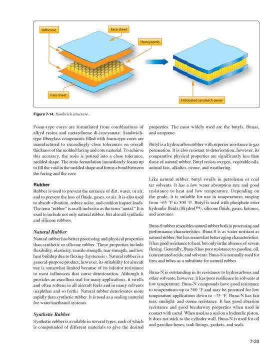 both in processing and performance characteristics. Buna S is as water resistant as natural rubber, but has somewhat better aging characteristics. It has good resistance to heat, but only in the absence of severe heat Flexing. Generally, Buna S has poor resistance to gasoline oil, concentrated acids and solvents. 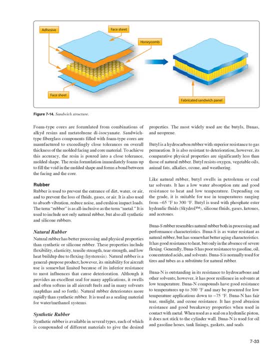 Buna S is normally used for tires and tubes as a substitute for natural rubber. Buna N is outstanding in its resistance to hydrocarbons and other solvents. however, it has poor resilience in solvents at low temperature. Buna N compounds have good resistance to temperatures up to 300 degrees Fahrenheit. 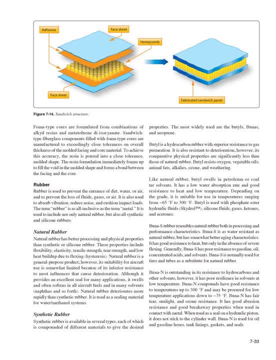 and may be procured for low temperature applications down to minus 75 degrees Fahrenheit. Buna N has fair, tier sunlight and ozone resistance. It has good abrasion resistance and good breakaway properties when used in contact with metal. When used as a seal on a hydraulic. 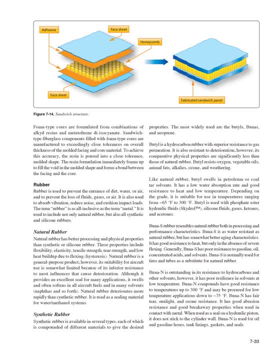 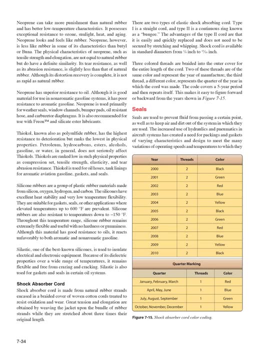 piston. it does not stick to the cylinder wall. Buna N is used for oil and gasoline hoses, tank linings, gaskets and seals. Neoprene can take more punishment than natural rubber and has better low temperature characteristics. It possesses exceptional resistance to ozone. 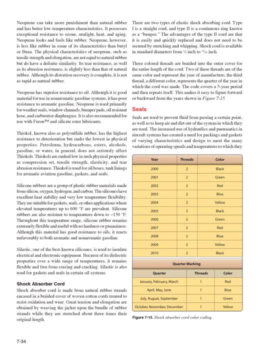 sunlight, heat and aging. Neoprene, however, is less like rubber in some of its characteristics than butyl or buna. The physical characteristics of neoprene, such as tensile strength and elongation, are not equal to natural rubber, but do have a definite similarity. 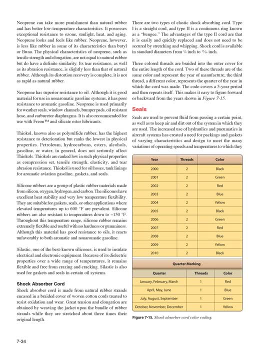 Its tier resistance, as well as its abrasion resistance, is slightly less than that of natural rubber. Although its distortion recovery is complete, it is not as rapid as natural rubber. Neoprene has superior resistance to oil. Although its distortion recovery is complete, it is not as rapid as natural rubber. 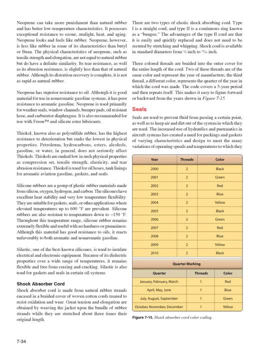 Although it is good material for use in non-aromatic gasoline systems, it has poor resistance to aromatic gasoline. Neoprene is used primarily for weather seals, window channels, bumper pads, oil-resistant hose and carburetor diaphragms. It is also recommended for use with freon and silicate ester lubricants. 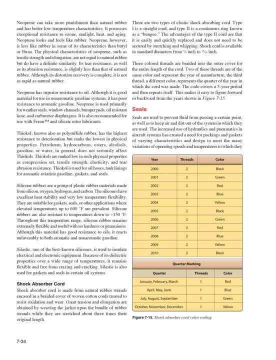 Thiokol, known also as polysulfide rubber, has the highest resistance to deterioration, but ranks the lowest in physical properties. Petroleum, hydrocarbons, esters, alcohols, gasoline or water in general does not seriously affect thiokols. 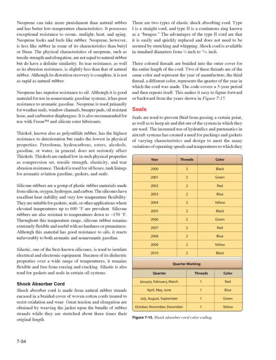 Thiokols are ranked low in such physical properties as compression, set tensile strength, elasticity and tier abrasion resistance. Thiokol is used for oil hoses, tank linings for aromatic aviation, gasoline gaskets and seals. Silicone rubbers are a group of plastic rubber materials. 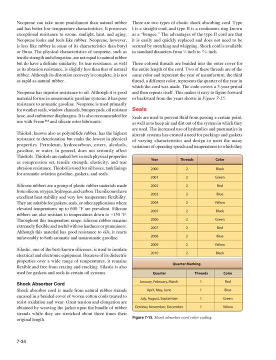 made from silicon, oxygen, hydrogen and carbon. The silicones have excellent heat stability and very low temperature flexibility. They are suitable for gaskets, seals or other applications where elevated temperatures up to 600 degree Fahrenheit are prevalent. Silicone rubbers are also resistant to temperatures down. 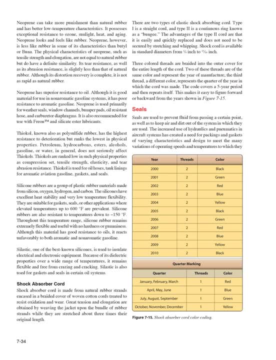 to minus 150 degrees Fahrenheit. Throughout this temperature range, silicone rubber remains extremely flexible and useful, with no hardness or gumminess. Although this material has good resistance to oils, it reacts unfavorably to both aromatic and non-aromatic gasoline. Silastic, one of the best-known silicones, is used to 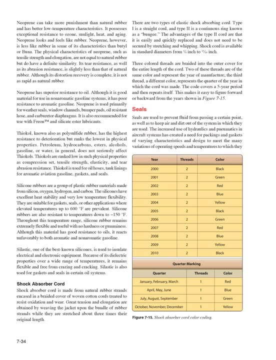 insufferably reduce the amount of carbon dioxide that is released from the silicone. Silastic is used to insulate electrical and electronic equipment. Because of its dielectric properties over a wide range of temperatures, it remains flexible and free from crazing and cracking. Silastic is also used for gaskets and seals in certain oil systems. 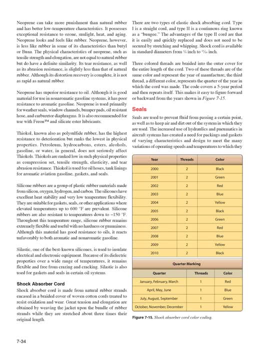 Shock absorber cord. Shock absorber cord is made from natural rubber strands encased in a braided cover of woven cotton cords treated to resist oxidation and wear. Great tension and elongation are obtained by weaving the jacket upon the bundle of rubber strands while they are stretched about. 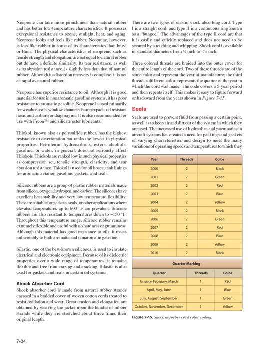 three times their original length. There are two types of elastic shock absorbing cord. Type I is a straight cord and Type II is a continuous ring known as a bungee. The advantages of the Type II cord are that it is easily and quickly replaced and does not need to be secured by stretching and whipping. Shock cord is available. 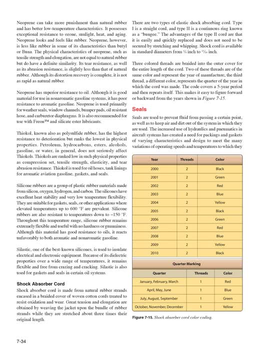 in standard diameters from 1 quarter inch to 13 sixteenths inch. Three colored threads are braided into the outer cover for the entire length of the cord. Two of these threads are of the same color and represent the year of manufacture. The third thread, type II, is a continuous ring known as a. 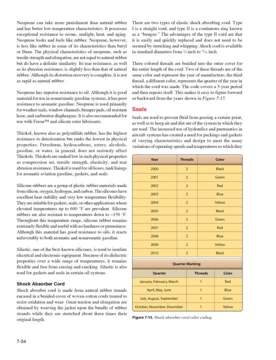 red. a different color represents the quarter of the year in which the cord was made. The code covers a five-year period and then repeats itself. This makes it easy to figure forward or backward from the year shown in figure 715.. Seal seals are used to prevent fluid from passing a certain point. 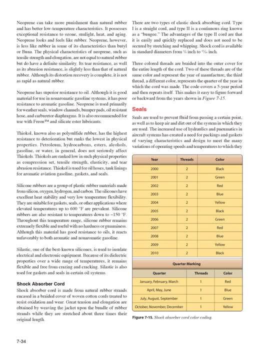 as well as to keep air and dirt out of the system in which they are used. The increased use of hydraulics and pneumatics in aircraft systems has created a need for packings and gaskets of varying characteristics and designed to meet the many variations of 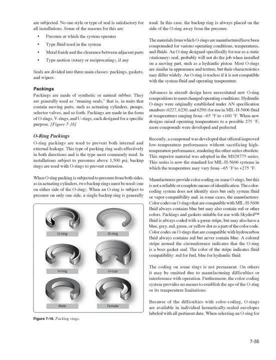 operations. The seal seals are used to prevent fluid from passing a certain point, as well as to speeds and temperatures to which they are subjected. No one style or type of seal is satisfactory for all installations. Some of the reasons for this are pressure at which the system 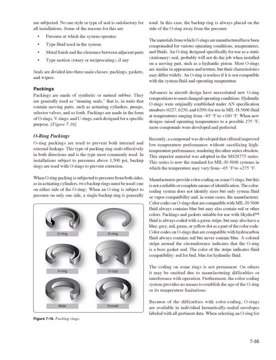 operates: type fluid used in the system, metal finish and the clearance between adjacent parts. type motion: rotary or reciprocating, If any. seals are divided into three main classes: packings, gaskets and wipers. Packings: packings are made of synthetic or natural rubber. 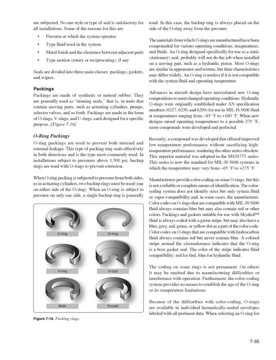 They are generally used as running seals, that is, in units that contain moving parts, such as actuating cylinders, pumps, selector valves and so forth. Packings are made in the form of O-rings, V-rings and U-rings. 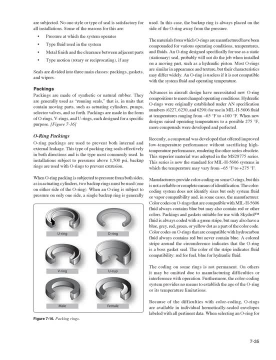 each designed for a specific purpose. Figure 716, O-ring packings. O-ring packings are used to prevent both internal and external leakage. This type of packing ring seals effectively in both directions and is the type most commonly used In installations subject to pressures above. 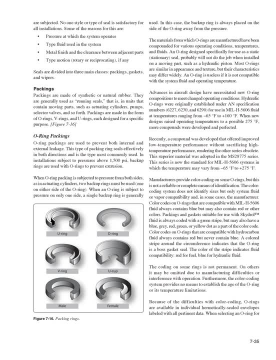 1,500 psi backup rings are used to prevent internal and external leakage. This type of O-rings are used with O-rings to prevent extrusion When O-ring packing is subjected to pressure from both sides, as in actuating cylinders. two backup rings must be used, one on either side of the. 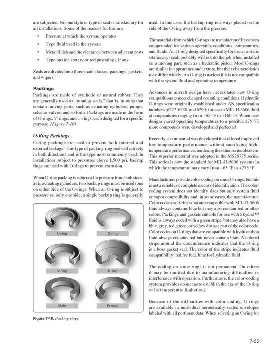 O-ring. When an O-ring is subject to pressure on only one side, a single backup ring is generally used. In this case, the backup ring is always placed on the side of the O-ring, away from the pressure. The materials from which O-rings are manufactured have been compounded for various 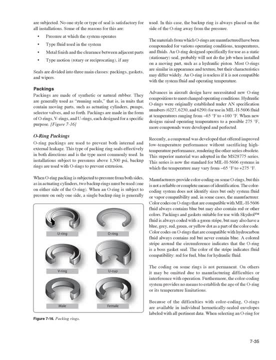 operating conditions, temperatures and fluids. An O-ring design is designed to be used to specifically for use as a static stationary seal probably will not do the job when installed on a moving part such as a hydraulic piston. Most O-rings are similar in appearance and texture. 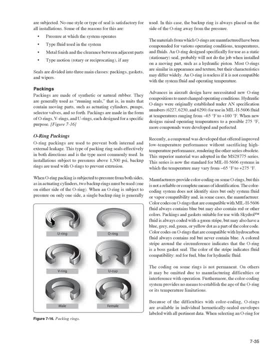 but their characteristics may differ widely. An O-ring is useless if it is not compatible with the system, fluid and operating temperature. Advances in aircraft design have necessitated new O-ring compositions to meet changed operating conditions. Hydraulic O-rings were originally established under and specification numbers. 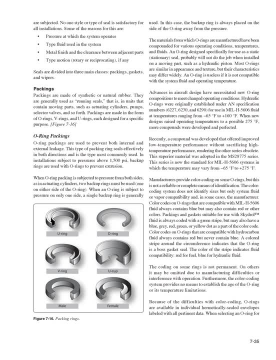 627,, 6230, and 6290, for use in mill. H5606 fluid at temperatures ranging from minus 65°F to plus 160°F. When new designs raised operating temperatures to a possible 275°F, more compounds were developed and perfected. Recently, a compound was developed that offered improved low-temperature. 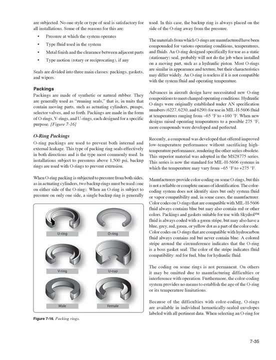 performance without sacrificing high-temperature performance, rendering the other series obsolete. This superior material was adopted in the MS28775 series. This series is now the standard for mill H5606 systems in which the temperature may vary from minus 65°F to plus 275°F. 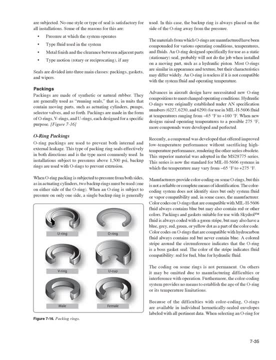 Manufacturers provide color coding on some O-rings, but this is not a reliable or complete means of identification. The color coding system does not identify sizes, but only system fluid or vapor compatibility and, in some cases, the manufacturing process The O-rings are used to. 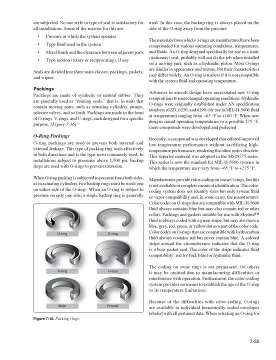 provide color coding on some O-rings, but this is not a reliable or complete means of identification. Manufacturer Color codes on O-rings that are compatible with mill. H5606 fluid always contains blue, but may also contain red or other colors. Packings and gaskets suitable for use with. 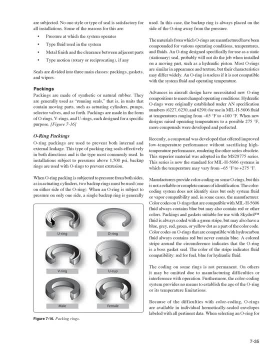 skydryl fluid is always coated with a green stripe, but may also have a blue, gray, red, green or yellow dot as a part of the color code. Color codes on O-rings that are compatible with hydrocarbon fluid always contains red, but never contain blue- A colored stripe around the circumference. 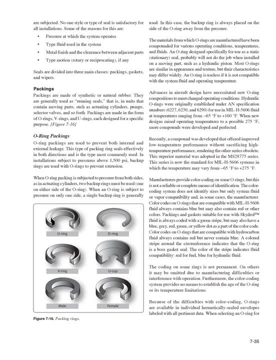 indicates that the O-ring is a bosque. The color of the stripe indicates fluid compatibility: red for fuel, blue for hydraulic fluid. The coating on some rings is not permanent. On others it may be emitted due to manufacturing difficulties or interference with operation. Furthermore, the color coding system provides: 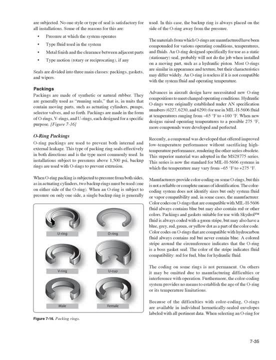 no means to establish the age of the O-ring or its temperature limitations. Because of the difficulties with color coding, O-rings are available in individual hermetically sealed envelopes labeled with all pertinent data. When selecting an O-ring, the color coding system. 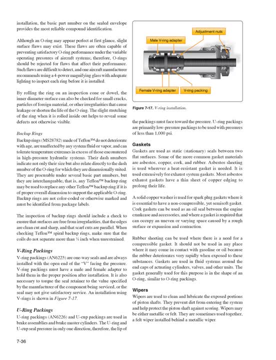 provides the most reliable compound identification. Although an O-ring may appear perfect at first glance, slight surface flaws may exist. These flaws are often capable of preventing satisfactory O-ring performance under the variable operating pressures of aircraft systems. therefore, O-rings should be rejected for flaws that affect their performance. Such flaws are difficult. 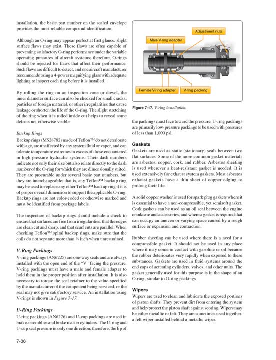 to detect, and one aircraft manufacturer recommends using a four-power magnifying glass with adequate lighting to inspect each ring before it is installed. By rolling the ring on an inspection cone or dowel, the inner diameter surface can also be checked for small cracks, particles of foreign material or other irregularities that cause leakage. 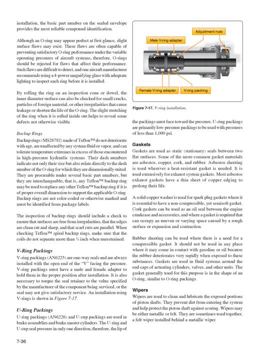 or shorten the life of the O-ring. The slight stretching of the ring when it is rolled inside out helps to reveal some defects not otherwise visible. Backup rings. Backup rings made of Teflon do not deteriorate with age, are unaffected by any system. 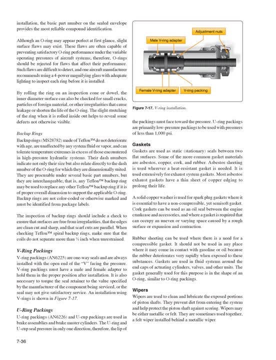 They can withstand the flow of water, heat fluid or vapor and can tolerate temperature extremes in excess of those encountered in high-pressure hydraulic systems. Their dash numbers indicate not only their size, but also relate directly to the dash number of the O-ring for which they are dimensionally suited. They are procurable under several basic part. 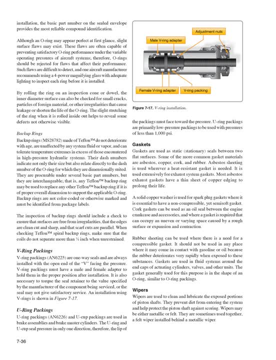 numbers, but they are interchangeable, that is, any Teflon backup ring may be used to replace any other Teflon backup ring if it is a proper overall dimension to support the applicable O-ring. Backup rings are not color coded or otherwise marked and must be identified for use for. 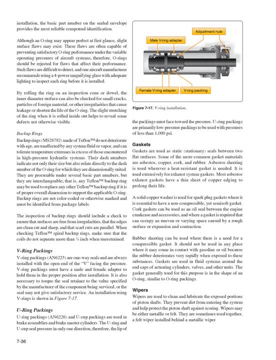 from package labels. The inspection of backup rings should include a check to ensure that surfaces are free from irregularities, that the edges are clean, cut and sharp and that scarf cuts are parallel. When checking Teflon spiral backup rings, make sure that the coils do not. 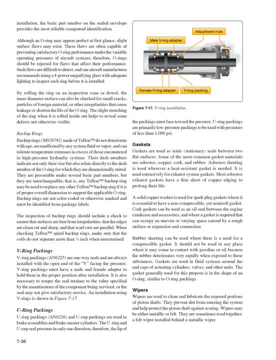 separate more than one quarter inch when unrestrained V-ring packings. V-ring packings AN6225 are one-way seals and are always installed with the open end of the V facing the pressure. V-ring packings must have a male and female adapter to hold them in the proper position. 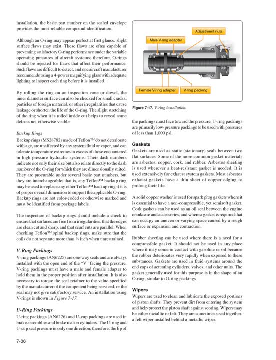 after installation, It is also necessary to torque the seal retainer to the value specified by the manufacturer of the component being serviced, or the seal may not give satisfactory service. An installation using V-rings is shown in figure 717.. U-ring packings. U-ring packings- AN6226. 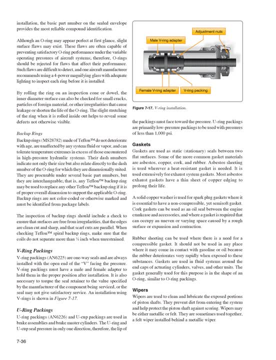 and U-cup packings are used in brake assemblies and brake master cylinders. The U-ring and U-cup seal pressure in only one direction. therefore, the lip of the packings must face toward the pressure. U-ring packings are primarily low-pressure packings to be used with pressures of less. 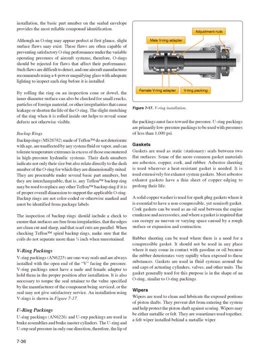 than 1,000 pounds per square inch Gaskets. Gaskets are used as static stationary seals between two flat surfaces. Some of the more common gasket materials are asbestos, copper, cork and rubber. Asbestos sheeting is used wherever a heat-resistant gasket is needed. 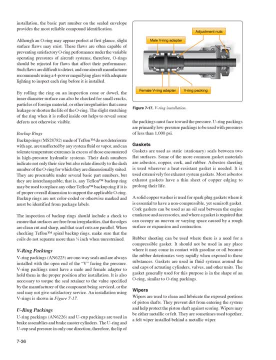 It is used extensively for exhaust system gaskets. Most asbestos exhaust gaskets have a thin sheet of copper edging to prolong their life. A solid copper washer is used for spark plug gaskets, where it is essential to have a non-compressible 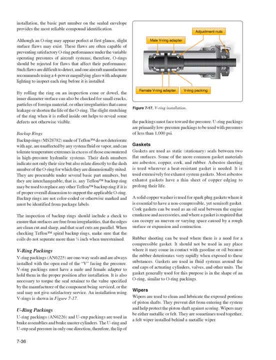 yet semi-soft gasket. Cork gaskets can be used as an oil seal between the engine crankcase and accessories and where a gasket is required that can occupy an uneven or varying space caused by a rough surface or expansion and contraction. Rubber sheeting can be used where there is a 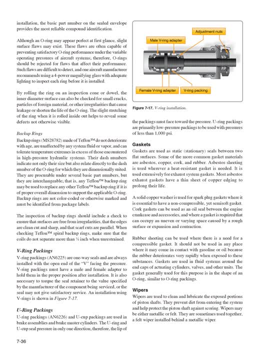 need for a compressible gasket. It should not be used in any place where it may come in contact with gasoline or oil, because the rubber deteriorates very rapidly when exposed to these substances. Gaskets are used in fluid systems around the end caps of actuating cylinders, valves. 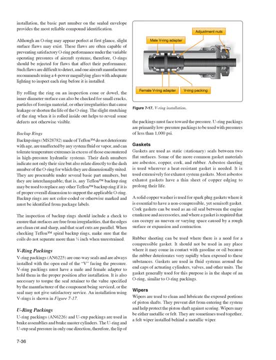 and other units. The gasket generally used for this purpose is in the shape of an o-ring similar to o-ring packings Wipers. Wipers are used to clean and lubricate the exposed portions of piston shafts. They prevent dirt from entering the system and help protect the 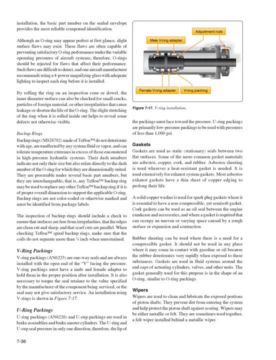 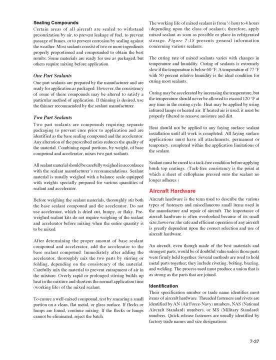 piston shaft against scoring. Wipers may be either metallic or felt. They are sometimes used together: a felt wiper installed behind a metallic wiper. Sealing compounds. Certain areas of all aircraft are sealed to withstand pressurization by air, to prevent leakage of fuel, to prevent passage of fumes or to prevent corrosion by sealing. 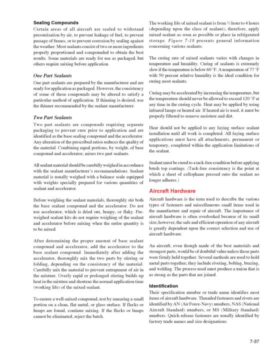 against the weather. Most sealants consist of two or more ingredients, properly proportioned and compounded to obtain the best results. Some materials are ready for use as packaged, but others require mixing before application. One-part sealants. One-part sealants are prepared by the manufacturer and are ready for application as packaged. 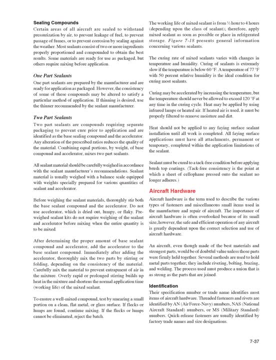 However, the consistency of some of these compounds may be altered to satisfy a particular method of application. If thinning is desired, use the thinner recommended by the sealant manufacturer. Two-part sealants. Two-part sealants are compounds requiring separate packaging to prevent cure prior to application and are identified as the base sealing compound. 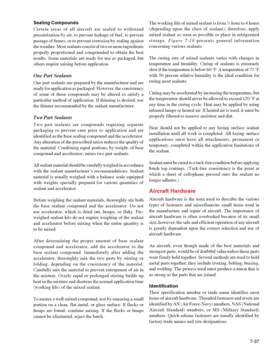 and the accelerator. Any alteration of the prescribed ratios reduces the quality of the material Combining equal portions by weight of base compound and accelerator mixes. two-part sealants. All sealant materials should be carefully weighed in accordance with the sealant manufacturer's recommendations. Sealant material is usually weighed with a balance scale equipped with. 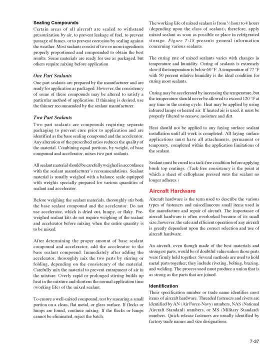 weights specially prepared for various quantities of sealant and accelerator. Before weighing the sealant materials, thoroughly stir both the base sealant compound and the accelerator. Do not use accelerator which is dried out, lumpy or flaky. Great sealant kits do not require weighing of the sealant and accelerator before mixing. 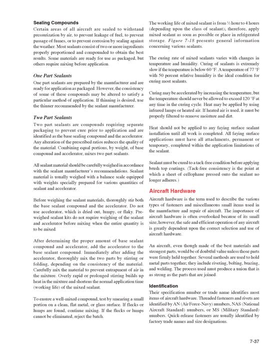 when the entire quantity is to be mixed. After determining the proper amount of base sealant compound and accelerator, add the accelerator to the base sealant compound Immediately after adding the accelerator. thoroughly mix the two parts by stirring or folding, depending on the consistency of the material. 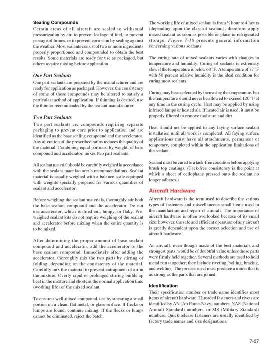 Carefully mix the material to prevent entrapment of air in the mixture. Overly rapid or prolonged stirring builds up heat in the mixture and shortens the normal application time of the mixed sealant. To ensure a well-mixed compound test by smearing a small portion on a clean, flat metal or 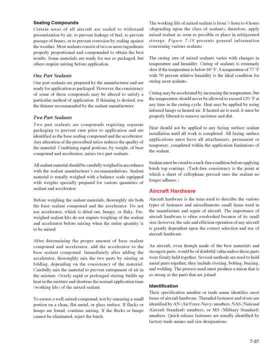 glass surface. If flecks or lumps are found, continue mixing. If the flecks or lumps cannot be eliminated, reject the batch. The working life of mixed sealant is from half hour to four hours, depending upon the class of sealant. therefore, apply mixed sealant as soon as possible or place in refrigerated. 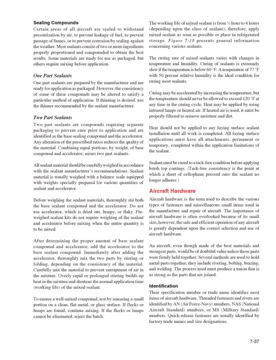 storage. Figure 7-18 presents general information concerning various sealants. The curing rate of mixed sealants varies with changes in temperature and humidity. Curing of sealants is extremely slow if the temperature is below 60°F. A temperature of 77°F with 50% relative humidity is the ideal condition for curing most sealants. 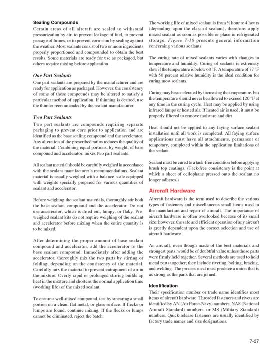 Curing may be accelerated by increasing the temperature, but the temperature should never be allowed to exceed 120°F at any time in the curing cycle. Heat may be applied by using infrared lamps or heat exchangers. The temperature should never be allowed to exceed 120°F at any time in the curing cycle. 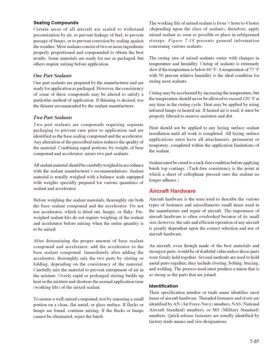 Heat may be applied by using infrared lamps or heated lamps air. If heated air is used, it must be properly filtered to remove moisture and dirt. Heat should not be applied to any faying surface sealant installation until all work is completed. All faying surface applications must have all attachments, permanent or temporary. 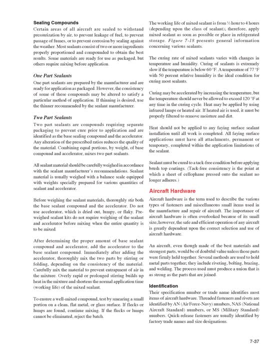 completed within the application limitations of the sealant. Sealant must be cured to a tack-free condition before applying brush top coatings. Tack-free consistency is the point at which a sheet of cellophane pressed onto the sealant no longer adheres. Aircraft Hardware. 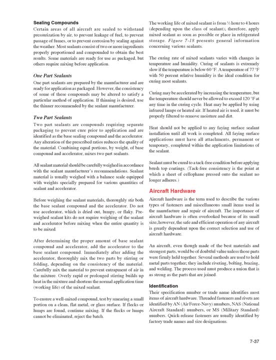 Aircraft Hardware is the term used to describe the various types of fasteners and miscellaneous small items used in the manufacture and repair of aircraft. The importance of aircraft hardware is often overlooked because of its small size. however, the safe and efficient operation of any aircraft is greatly dependent upon the correct selection and use of aircraft hardware. 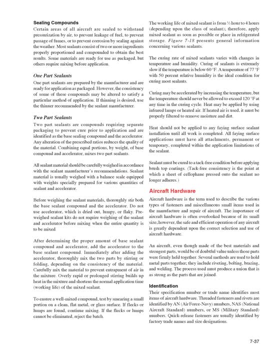 An aircraft, even though made of the best materials and strongest parts, would be of doubtful value unless those parts were made of the best materials and strongest parts. Parts were firmly held together. Several methods are used to hold metal parts together. They include riveting, bolting, brazing and welding. The process used must produce a union. 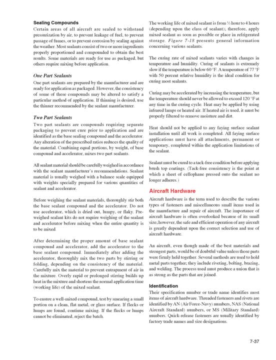 that is as strong as the parts that are joined. Identification: Their specification number or trade name identifies most items of aircraft hardware- Threaded fasteners and rivets are identified by an Air Force Navy numbers, NAS, National Aircraft Standard Numbers or MS. 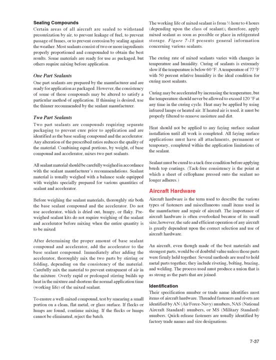 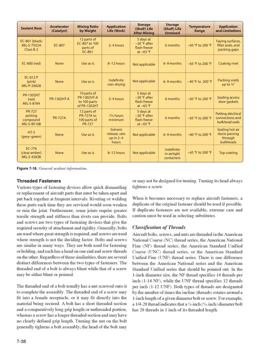 Military Standard Numbers. Quick-release fasteners are usually identified by factory trade names and size designations. Threaded fasteners- Various types of fastening devices- allow quick dismantling or replacement of aircraft parts that must be taken apart and put back together at frequent intervals, Riveting or welding these parts each time they are. 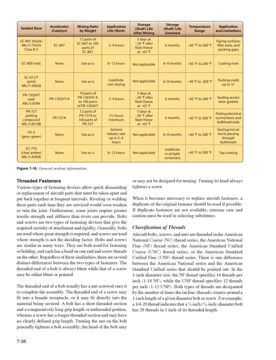 serviced would soon weaken or ruin the joint. Furthermore, some joints require greater tensile strength and stiffness than rivets can provide. Bolts and screws are two types of fastening devices that give the required security of attachment and rigidity. Generally, bolts are used where great strength is required and screws are used where strength 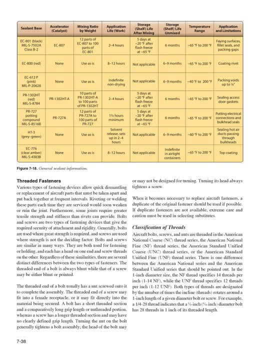 is not the deciding factor. Bolts and screws are similar in many ways. They are both used for fastening or holding, and each has a head on one end and screw threads on the other. Regardless of these similarities, there are several distinct differences between the two. 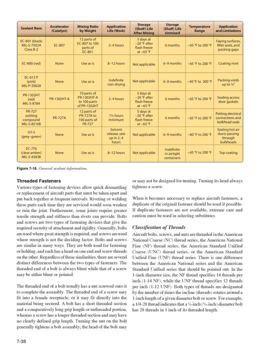 types of fasteners. The threaded end of a bolt is always blunt, while that of a screw may be either blunt or pointed. The threaded end of a bolt usually has a nut screwed onto it to complete the assembly. The threaded end of a screw may fit into a female receptacle or it may fit directly. 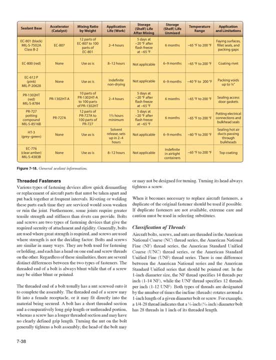 into the material being secured. A bolt has a short threaded section and a comparatively long grip length or unthreaded portion, whereas a screw has a longer threaded section and may have no clearly defined grip length. Turning the nut on the bolt generally tightens a bolt. 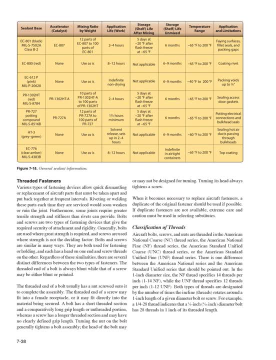 assembly. the head of the bolt may or may not be designed for turning. Turning its head always tightens a screw. When it becomes necessary to replace aircraft fasteners, a duplicate of the original fastener should be used if possible. If duplicate fasteners are not. 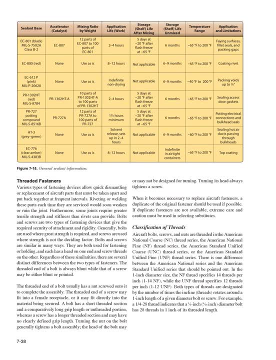 available. extreme care and caution must be used in selecting substitutes. Classification of Threads-Aircraft bolts, screws and nuts are threaded in the American National Course thread series, the American National Find thread series, the American Standard Unified Course thread series or the American Standard Unified. 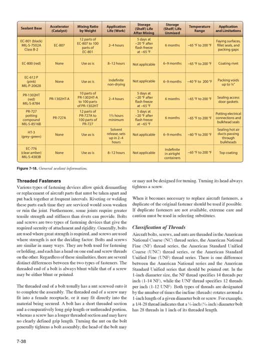 Fine thread series. There is one difference between the American National, American Standard Unified series that should be pointed out. In the 1-inch diameter size, the NF thread specifies 14 threads per inch. 1 to 14 NF, while the UNF thread specifies 12 threads. 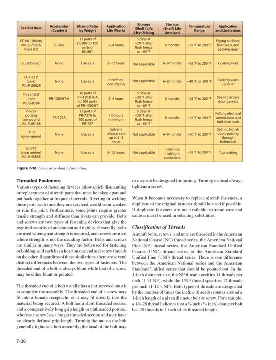 per inch. 1 to 12 UNF. Both types of threads are designated by the number of times the incline threads rotates around a 1-inch length of a given diameter bolt or screw. For example, a 1 quarter minus 28 thread indicates that a 1 quarter inch- 4 sixteenths inch diameter bolt. 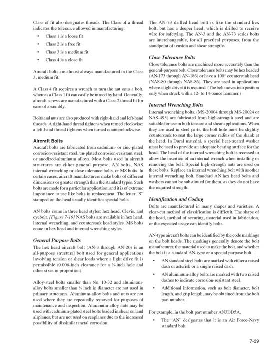 has 28 threads in 1 inch of its threaded length. Class of fit also designates threads. The class of a thread indicates the tolerance allowed in manufacturing. Class 1 is a loose fit. Class 2 is a free fit. Class 3 is a medium fit, Class 4 is a close fit. Aircraft bolts are almost always. 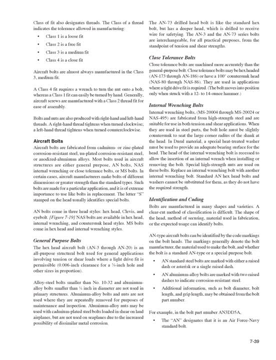 manufactured in the Class 3, medium fit. A Class 4 fit requires a wrench to turn the nut onto a bolt, whereas a Class 1 fit can easily be turned by hand. Generally, aircraft screws are manufactured with a Class 2 thread fit. for ease of assembly, Bolts and nuts are also produced with right-hand and left-hand. 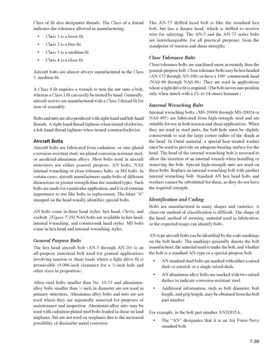 threads: A right-hand thread tightens when turned clockwise. a left-hand thread tightens when turned counterclockwise. Aircraft bolts. Aircraft bolts are fabricated from cadmium or zinc-plated corrosion-resistant steel, unplated corrosion-resistant steel or anodized aluminum. 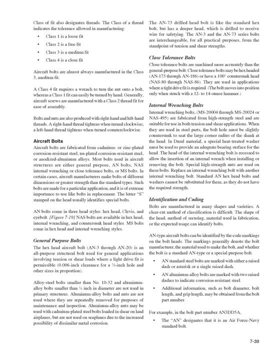 alloys. Most bolts used in aircraft structures are either general or standard. Aircraft bolts are manufactured from cadmium or zinc-plated, corrosion-resistant steel or anodized aluminum alloys. Most bolts used in aircraft structures are either general purpose and bolts, NAS, internal wrenching or close tolerance bolts or MS bolts In certain cases. 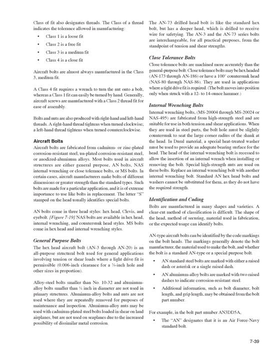 aircraft manufacturers make bolts of different dimensions or greater strength than the standard types. Such bolts are made for a particular application and it is of extreme importance to use like bolts in replacement. The letter S stamped on the head usually identifies special bolts, And bolts come in three head styles: hex, head clevis and eye bolt- Figure 719,. 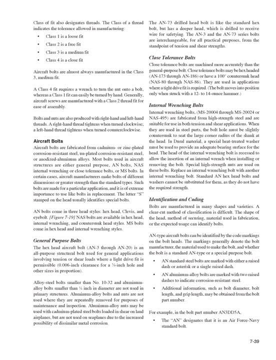 NAS bolts are available in hex head, internal wrenching and countersunk head styles. MS bolts come in hex head and internal wrenching styles. General purpose bolts: The hex head aircraft bolt- AN3 through AN20, is an all-purpose structural bolt used for general applications involving tension or shear loads where a light 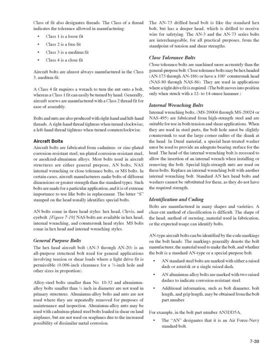 drive fit is permissible. 0.006-inch clearance for a 5-eighths-inch hole and other sizes in proportion. Alloy steel bolts smaller than no 10-32 and aluminum alloy bolts smaller than 1.25-inch in diameter are not used in aircraft structures. Alloy steel bolts smaller than no 10-32 and. 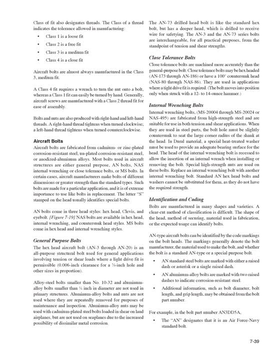 aluminum alloy bolts are used in primary structures. Aluminum alloy bolts and nuts are not used where they are repeatedly removed for purposes of maintenance and inspection. Aluminum alloy nuts may be used with cadmium-plated steel bolts loaded in shear-on-land airplanes, but are not used on. 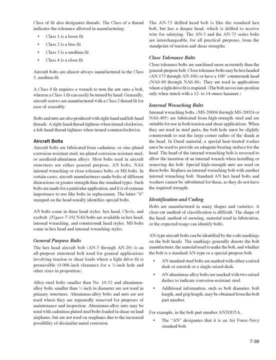 seaplanes due to the increased possibility of dissimilar metal corrosion. The AN73 drilled head bolt is like the standard hex bolt but has a deeper head which is drilled to receive wire for safety. The AN3 and the AN73 series bolts are interchangeable. 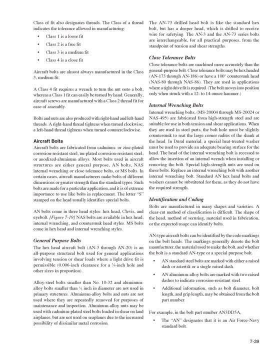 For all practical purposes from the standpoint of tension and shear strengths, close-tolerance bolts. close-tolerance bolts are machined more accurately than the general-purpose bolt. Close-tolerance bolts may be hex-headed- AN173 through AN186, or have a 100-degrees. 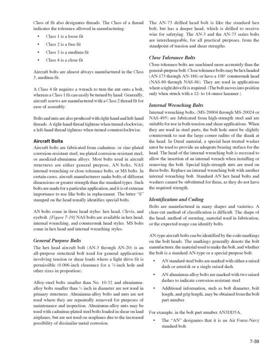 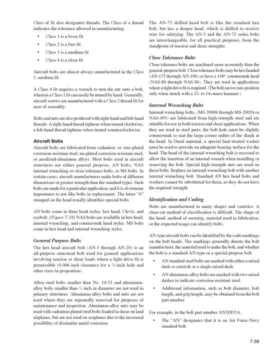 are fabricated from high-strength steel and are suitable for use in both tension and shear applications. When they are used in steel parts, the bolt hole must be slightly countersunk to seat the large corner radius of the shank at the head. Endural material: a special heat-treated 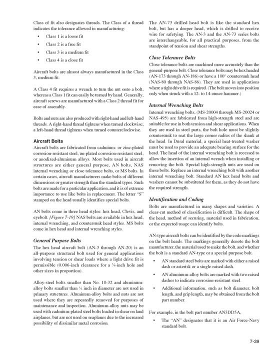 washer must be used to provide an adequate bearing surface for the head. The head of the internal wrenching bolt is recessed to allow the insertion of an internal wrench when installing or removing the bolt. Special high-strength nuts are used on these bolts. Replace an internal wrenching bolt. 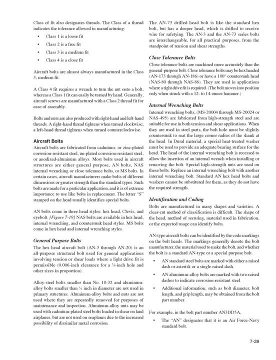 with another internal wrenching bolt. Standard and hex-head bolts and washers cannot be substituted for them, as they do not have the required strength. Identification and coating bolts are manufactured in many shapes and varieties. A clear-cut method of classification is difficult. 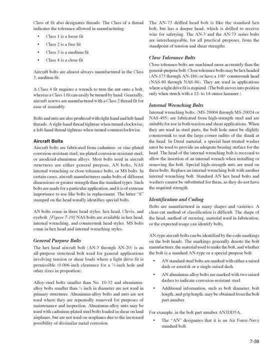 The shape of the head, method of securing material used in fabrication or the expected usage can identify bolts And type error. Aircraft bolts can be identified by the code markings on the bolt heads. The markings generally denote the bolt manufacturer, the material used to make the bolt and whether the bolt is a standard. 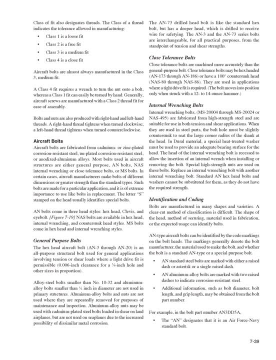 in type or a special purpose bolt, And standard steel bolts are marked with either a raised dash or asterisk, or a single raised dash. Aluminum alloy bolts are marked with two raised dashes to indicate corrosion-resistant steel. Additional information, such as bolt diameter, bolt length. 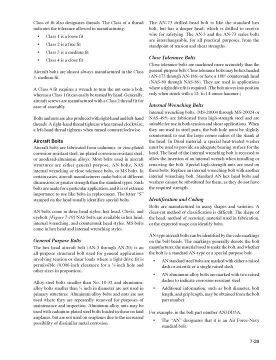 and grip length may be obtained, For example, in the bolt part number AN3DD5A. the IN designates that it is an Air Force Navy standard bolt. The 3 indicates the diameter in sixteenths of an inch, three sixteenths. 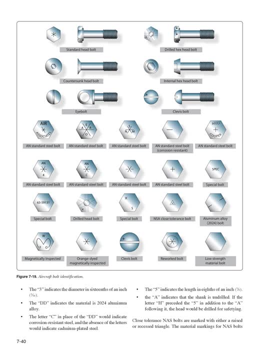 The DD indicates the material is 2024 aluminum alloy. The letter C in place of the DD would indicate corrosion-resistant steel and the absence of the letters would indicate cadmium-plated steel. The 5 indicates the length in eighths of an inch five-eighths. 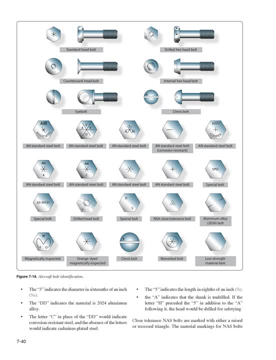 The A indicates that the shank is undrilled. If the letter H preceded the 5, in addition to the A following it, the head would be drilled for safetying. Close-tolerance NAS bolts are marked with either a raised or recessed triangle. The material markings for NAS bolts are the same. 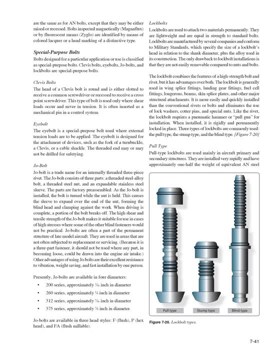 as for N bolts, except that they may be either raised or recessed Bolts inspected magnetically. Magnaflux or bifluorescent means- Zyglo, are identified by means of colored lacquer or a head marking of a distinctive type. 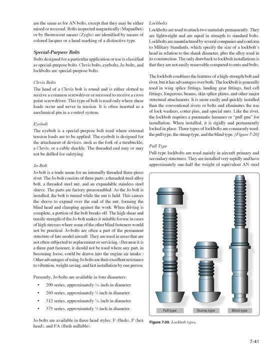 Special-purpose bolts. Bolts designed for a particular application or use is classified as special-purpose bolts, Clevis bolts, I-bolts, J-bolts and lock bolts are special-purpose bolts, Clevis bolts. The head of a clevis bolt is round and is either slotted to receive a common 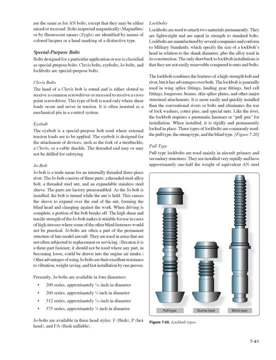 screwdriver or recessed to receive a cross-point screwdriver. This type of bolt is used only where shear loads occur and never in tension. It is often inserted as a mechanical pin in a control system. I-bolt. The I-bolt is a special-purpose bolt. 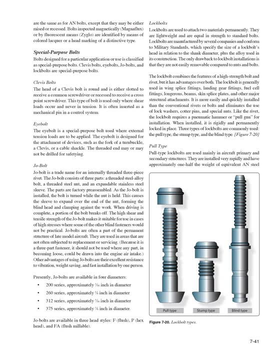 where external tension loads are to be applied. The I-bolt is designed for the attachment of devices such as the fork of a turnbuckle, a clevis or a cable shackle. The threaded end may or may not be drilled for safety J-bolt. J-bolt is a trade name for an internally threaded. 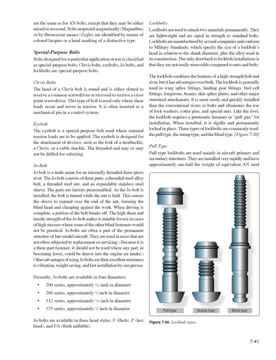 three-piece rivet. The J-bolt consists of three parts: a threaded steel alloy bolt, a threaded steel nut and an expandable stainless steel sleeve. The parts are factory pre-assembled As the J-bolt is installed. the bolt is installed in a three-piece: three-piece and three-piece. 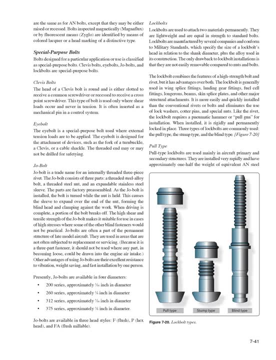 structure. The bolt is turned while the nut is held. This causes the sleeve to expand over the end of the nut, forming the blind head and clamping against the work. When driving is complete, a portion of the bolt breaks off. The high shear and tensile strength of the J-bolt makes it suitable. 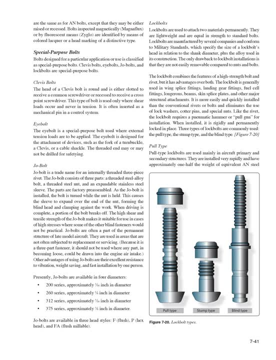 for use in cases of high stresses where some of the other blind fasteners would not be practical. J-bolts are often a part of the permanent structure of late-model aircraft. They are used in areas that are not often subjected to replacement or servicing. 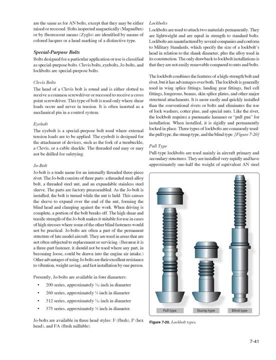 Because it is a three-part fastener, it should not be used where any part, in becoming loose, could be drawn into the engine air intake. Other advantages of using J-bolts are their excellent resistance to vibration, weight saving and fast installation by one person. 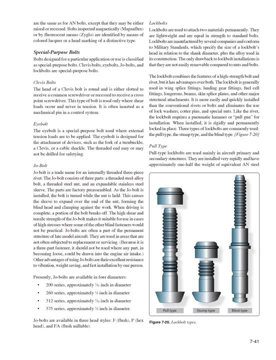 Presently, J-bolts are available in four diameters: 200 series- approximately 3 16th inch in diameter. 260 series- approximately 1 quarter inch in diameter. 312 series- approximately 5 16th inch in diameter. 375 series. 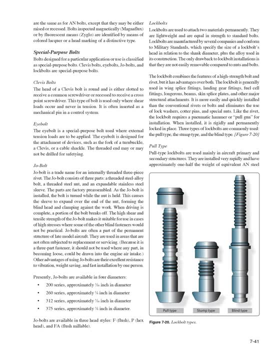 J-bolts are available in three head styles: F-flush, P-hex head and FA-flush- millable Lockbolts. Lockbolts are used to attach two materials permanently. They are lightweight and are equal in strength to standard bolts. 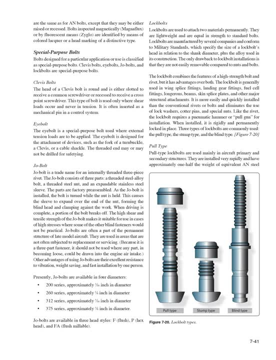 Lockbolts are manufactured by several companies and conform to military standards, which specify the size of a lockbolt's head in relation to the shank diameter plus the alloy used in its construction. The only drawback to lockbolt installation is that they are not easily removable compared to nuts and bolts. 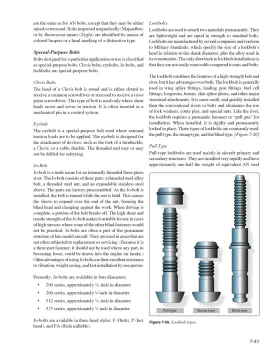 The lockbolt combines the features of a high-strength bolt and rivet, but it has advantages over both. The lockbolt is generally used in wing splice fittings, landing gear fittings, fuel cell fittings, long-erons beams, skin splice plates. 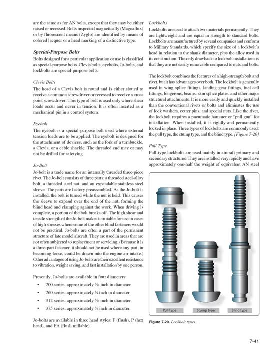 and other major structural attachments. It is more easily and quickly installed than the conventional rivets or bolts and eliminates the use of lock washers, cotter pins and special nuts. Like the rivet, the lockbolt requires a lot of force to install the lockbolts. 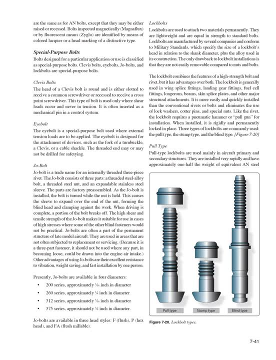 The lockbolt requires a pneumatic hammer or pull gun for installation. When installed, it is rigidly and permanently locked in place. Three types of lockbolts are commonly used: the pull type, the stump type and the blind type. Figure 720,. pull type-pull type lockbolts are used mainly in aircraft, primary and secondary. 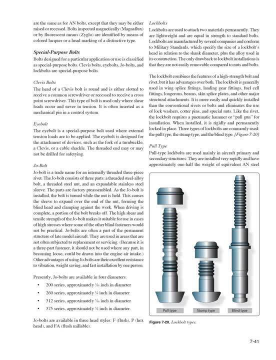 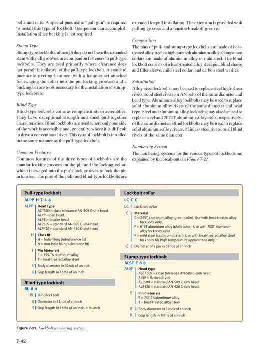 structures. They are installed very rapidly and have approximately one-half the weight of equivalent in steel Bolts and nuts. A special pneumatic pull gun is required to install this type of lockbolt. The lockbolt is used to install the lockbolts. The lockbolt is used to install the. 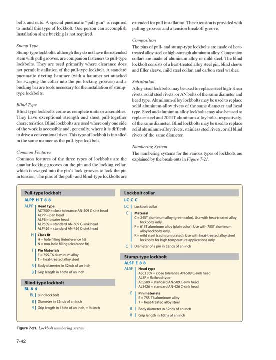 lockbolt, One person can accomplish installation, since bucking is not required. Stump type-stump type lockbolts, although they do not have the extended stem with pull grooves, are companion fasteners to pull type lockbolts. They are used primarily where clearance does. 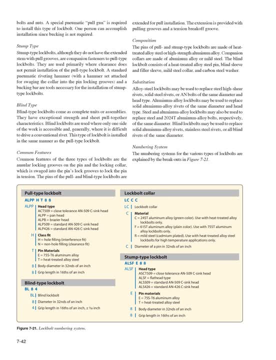 not permit installation of the pull type lockbolt. A standard pneumatic riveting hammer with a hammer set attached for swatching the collar into the pin, locking grooves and a bucking bar are tools necessary for the installation of stump type lockbolts. 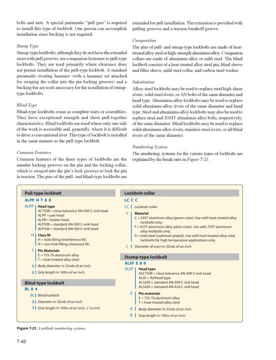 Blind type-blind type lockbolts are used to install the lockbolts. Blind type lockbolts come as complete units or assemblies. They have exceptional strength and sheet pull together characteristics. Blind lockbolts are used where only one side of the work is accessible and generally where it is difficult to drive a conventional rivet. 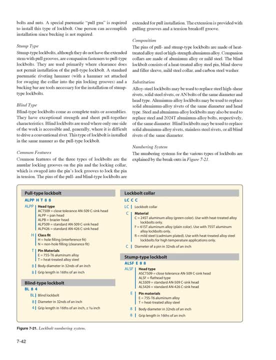 This type of lockbolt is installed in the same manner as the pull type lockbolt. Common features: Common features of the three types of lockbolts are the annular locking grooves on the pin and the locking collar which is swashed into the pin's lock grooves to lock the pin in tension. 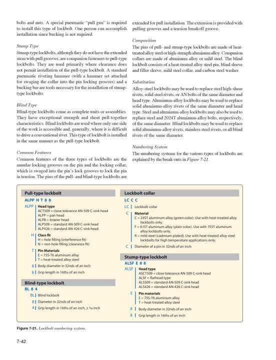 The pins of the pull and blind type lockbolts are extended for pull installation. The extension is provided with pulling grooves and a tension break-off groove. Composition: The pins of pull and stump type lockbolts are made of heat-treated alloy steel or high-strength aluminum alloy. 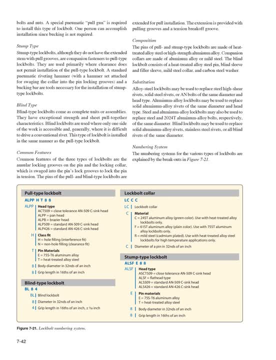 Companion collars are made of aluminum, alloy or mild steel. The blind lockbolt consists of a heat-treated alloy steel pin, blind sleeve and filler sleeve, mild steel collar and carbon steel washer Substitution. alloy steel lock bolts may be used to replace steel. high shear rivets. solid steel rivets. 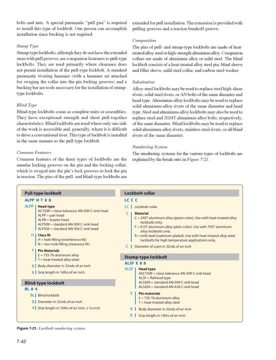 or in bolts of the same diameter and head type. Aluminum alloy lock bolts may be used to replace solid aluminum alloy rivets of the same diameter and head type. Steel and aluminum alloy lock bolts may also be used to replace steel and 2024T aluminum alloy bolts, respectively. 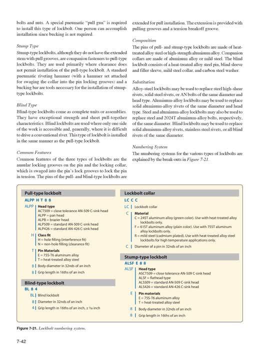 of the same diameter. Blind lock bolts may be used to replace solid aluminum alloy rivets, stainless steel rivets or all-blind rivets of the same diameter. Numbering system: The numbering systems for the various types of lock bolts are explained by the breakouts in figure 721.. 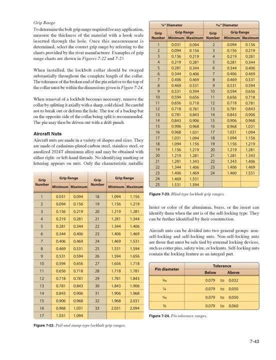 Grip range: To determine the bolt grip range required for any application measure, the thickness of the material, with a hook scale inserted through the hole. Once this measurement is determined, select the correct grip range by referring to the charts provided by the rivet manufacturer. Examples of grip range: 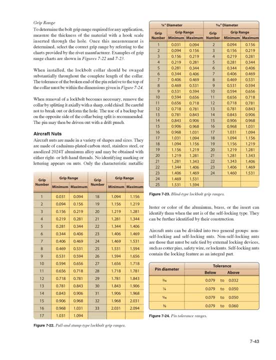 charts are shown in figures 7-22 and 7-23.. When installed, the lock bolt collar should be swashed substantially throughout the complete length of the collar. The tolerance of the broken end of the pin relative to the top of the collar must be within the dimensions. 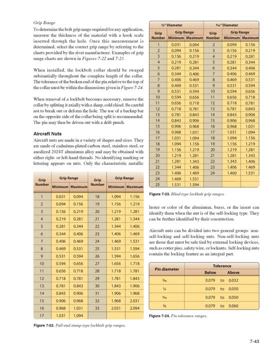 given in figure 724.. When removal of a lock bolt becomes necessary, remove the collar by splitting it axially with a sharp, cold chisel. Be careful not to break out or deform the hole. The use of a backup bar on the opposite side of the collar being split is. 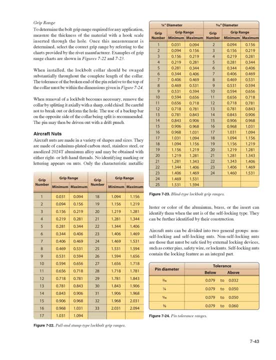 recommended. The pin may then be driven out with a drift punch. Aircraft nuts. Aircraft nuts are made in a variety of shapes and sizes. They are made of cadmium-plated carbon steel, stainless steel or anodized 2024T aluminum alloy, and may be obtained with either right or left-hand threads, No identifying. 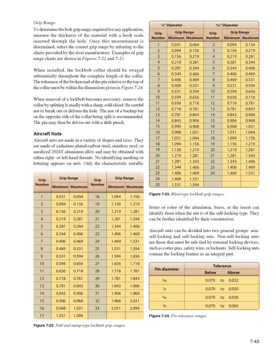 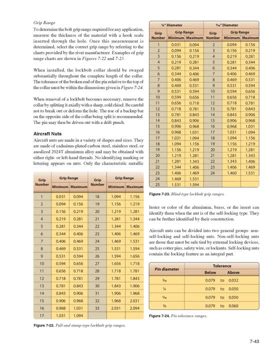 6, 6, 0.34, 4, 0.40, 6, 23, 1.40, 6, 1.46, 9, 7, 0.40, 6 0.46, 9, 24, 1.46, 9, 1.5, 3 1 0.46, 9, 0.53, 1, 25 1.5. 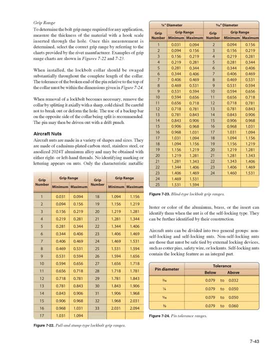 1, 1.59, 4, 9, 0.53, 1, 0.59, 4, 26, 1.59, 4, 1.65, 6, 10, 0.59, 4, 0.65, 6, 27, 1.65, 6, 1.71, 8, 11. 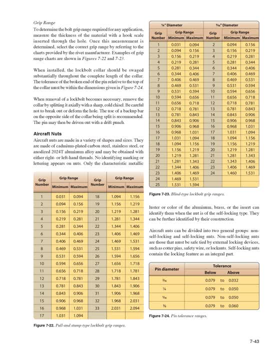 0.65, 6, 0.71 d, 28, 1.71, 8, 1.78, 112, 0.71, 8, 0.78, 1, 29, 1.78, 1, 1.8, 8. 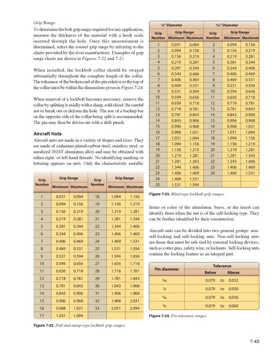 4, 3, 13 0.7 8, 1 0.8 4, 3, 31.8, 4, 3 1.9 0, 6, 14 0.8. 4, 3 0.9 0, 6, 31 1.9 0, 6, 1.9 6, 8, 15 0.9 0, 6 0.9 6, 8. 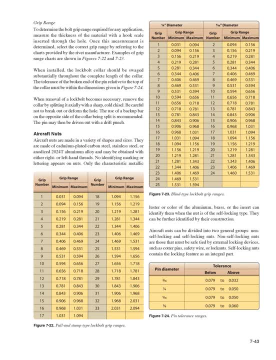 32, 1.9, 6, 8, 2.03, 1, 16, 0.9, 6, 8, 1.03, 1, 33, 2.03, 1, 2.09, 4, 17, 1.03, 1, 1.09, 4 figure 7: 22: 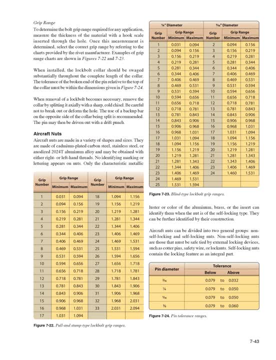 pull and stump type lock bolt grip ranges, luster or color of the aluminum brass or the insert can identify them. when the nut is of the self-locking type, they can be further identified by their construction. aircraft nuts can be divided into two general groups: non-self-locking and self-locking nuts. non-self-locking nuts are those that must be. 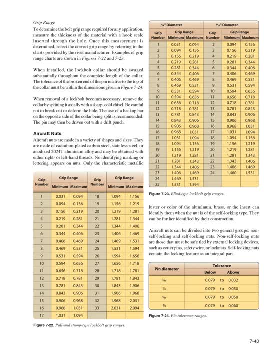 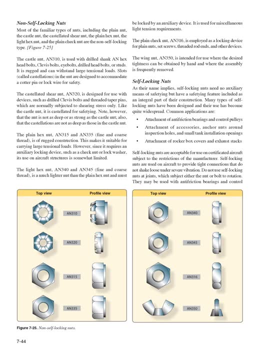 safe, tied by external locking devices such as cotter pins, safety wire or lock nuts. self-locking nuts contain the locking feature as an integral part. non-self-locking nuts: most of the familiar types of nuts, including the plain nut, the castle nut, the castellated shear nut, the plain hex nut. 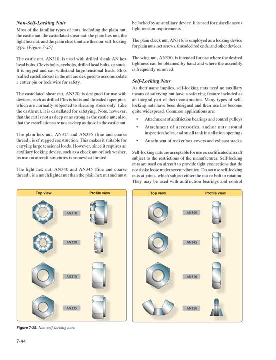 the light hex nut and the plain check nut are the non-self-locking type- figure 725. the castle nut, an 310, is used with drilled shank and hex head bolts, clevis bolts, eye bolts, drilled head bolts or studs. it is rugged and can withstand large tensional loads. slots called castellations in 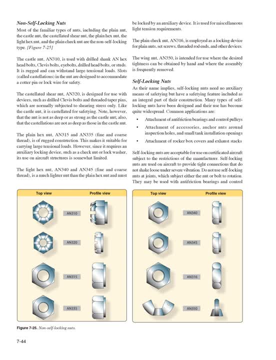 the nut are designed to accommodate a cotter pin or lock wire for safety. the castellated shear nut an 320 is designed for use with devices such as drilled clevis bolts and threaded taper pins, which are normally subjected to shearing stress. only like the castle nut, it is castellated. 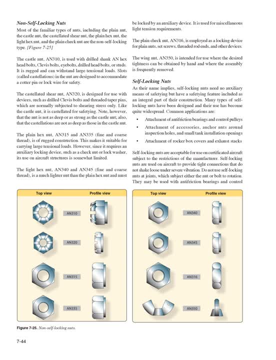 for safety. note, however, that the nut is not as deep or as strong as the castle nut. also that the castellations are not as deep as those in the castle nut. the plain hex nut, an 315 and an 335 fine and coarse thread, is of rugged construction. this makes it suitable for carrying large. 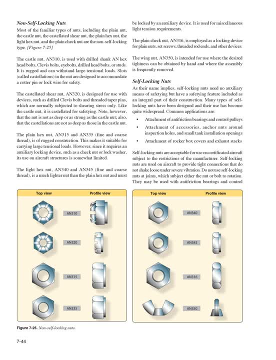 tensional loads. however, since it requires an auxiliary locking device such as a check nut or lock washer, its use on aircraft structures is somewhat limited. the light hex nut- an 340 and an 345 fine and coarse thread- is a much lighter nut than the plain hex nut and must. 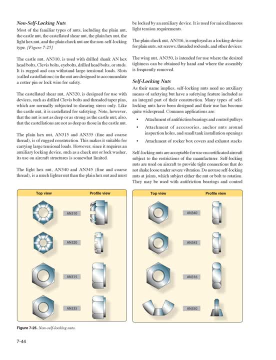 be locked by an auxiliary device. it is used for miscellaneous light tension requirements. the plain check nut- an 316- is employed as a locking device for plain nuts, set screws, threaded rod ends and other devices. the wing nut- an 350- is intended for use where the desired. 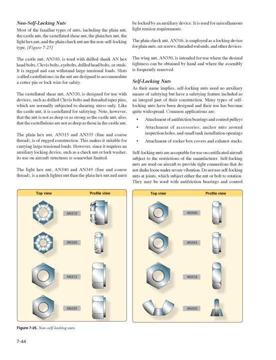 tightness can be obtained by hand and where the assembly is frequently removed. self-locking nuts. as their name implies, self-locking nuts need no auxiliary means of safetying, but have a safetying feature included as an integral part of their construction. many types of self-locking nuts have been designed and their use has become quite widespread. 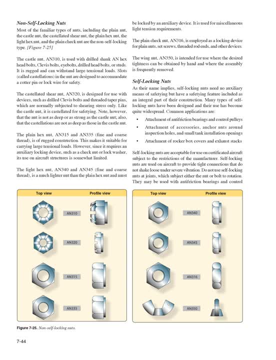 common applications are: attachment of anti-friction bearings and control pulleys. attachment of accessories. anchor nuts around inspection holes and small tank installation openings. attachment of rocker box covers and exhaust stacks. self-locking nuts are acceptable for use on certificated aircraft. subjects to the restrictions of the manufacturer. self-locking nuts are used on aircraft to: 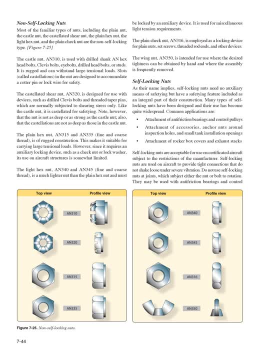 provide tight connections that do not shake loose under severe vibration. do not use self-locking nuts at joints which subject either the nut or bolt to rotation. they may be used with anti-friction bearings and control pulleys, provided the inner race of the bearing is clamped to the supporting. 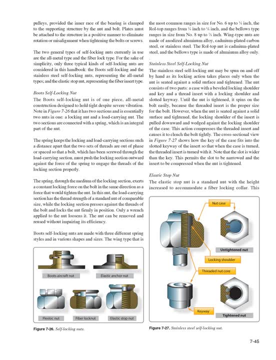 structure by the nut and bolt plates must be attached to the structure in a positive manner to eliminate rotation or misalignment when tightening the bolts or screws. the two general types of self-locking nuts currently in use are the all-metal type and the fiber lock type. for the sake of simplicity, only three typical kinds of self-locking nuts are: 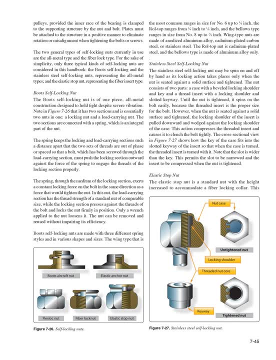 considered in this handbook: the boots self-locking and the stainless steel self-locking nuts representing the all-metal types, and the elastic stop nut representing the fiber insert type. boots self-locking nut. the boots self-locking nut is of one piece, all metal construction designed to hold tight despite severe vibration. note in figure 726 that it has two sections and 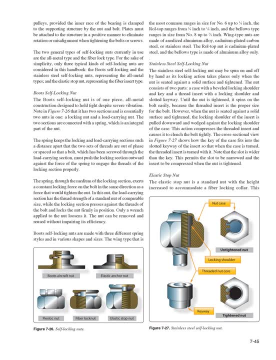 is essentially two nuts in one, a locking nut and a load carrying nut. the two sections are connected with a spring which is an integral part of the nut. the spring keeps the locking and load carrying sections such a distance apart that the two sets of threads are out of phase or space, so that a bolt 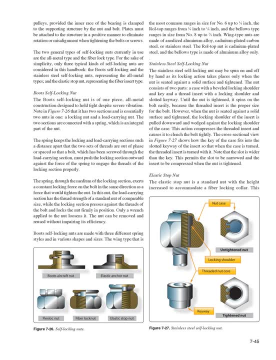 which has been screwed through the load carrying section must push the locking section outward against the force of the spring to engage the threads of the locking section properly. the spring, through the medium of the locking section, exerts a constant locking force on the bolt in the same direction as a force that would keep the bolt stable. in this case, the nut is done. 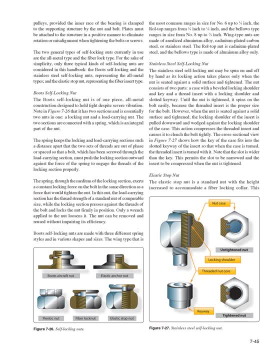 would tighten the nut. In this nut the load carrying section has the thread strength of a standard nut of comparable size, while the locking section presses against the threads of the bolt and locks the nut firmly in position. Only a wrench applied to the nut loosens it. The nut can be. 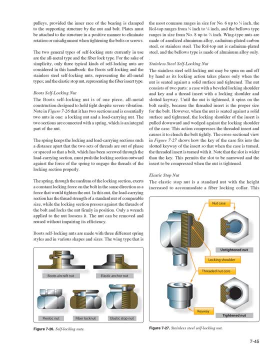 removed and reused without impairing its efficiency. Lutz self-locking nuts are made with three different spring styles and in various shapes and sizes. The wing type, that is the most common ranges in size for no 6, up to 1 quarter inch. the roll top ranges from 1 quarter inch to 1. 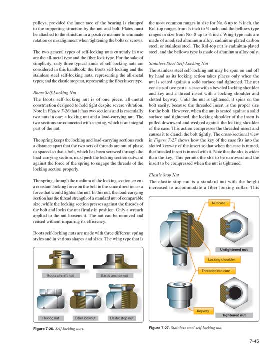 sixth inch and the bellows type ranges in size from no 8 up to 3 eighths inch. Wing type nuts are made of anodized aluminum alloy, cadmium plated carbon steel or stainless steel. The roll top nut is cadmium plated steel and the bellows type is made of aluminum alloy only. 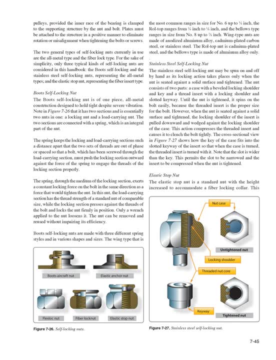 Dot Stainless steel self-locking nut. The stainless steel self-locking nut may be spun on and off by hand, as its locking action takes place Only when the nut is seated against a solid surface and tightened. The nut consists of two parts: a case with a beveled locking shoulder and key and a thread. 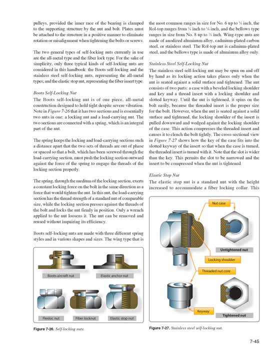 insert with a locking shoulder and slotted keyway Until the nut is tightened, it spins on the bolt easily because the threaded insert is the proper size for the bolt. However, when the nut is seated against a solid surface and tightened, the locking shoulder of the insert is pulled downward and 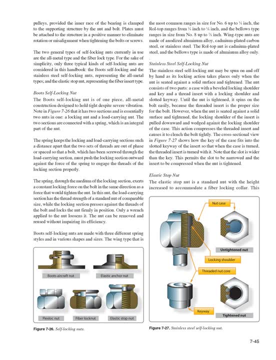 wedged against the locking shoulder of the case. This action compresses the threaded insert and causes it to clench the bolt. The nut is then tightened against a solid surface and tightened bolt tightly. The cross-sectional view in figure 727 shows how the key of the case fits into the 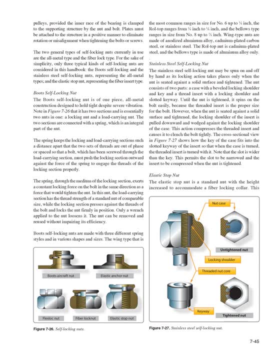 slotted keyway of the insert so that when the case is turned, the threaded insert is turned with it. Note that the slot is wider than the key. This permits the slot to be narrowed and the insert to be compressed when the nut is tightened. Elastic stop nut. 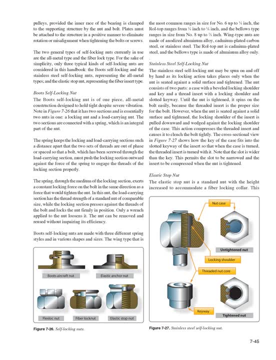 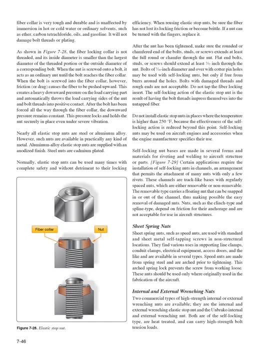 The elastic stop nut is a standard nut with the height increased to accommodate a fiber-locking collar. This fiber collar is very tough and durable and is unaffected by immersion in hot or cold water or ordinary solvents such as ether, carbon tetrachloride, oils and gasoline. It will 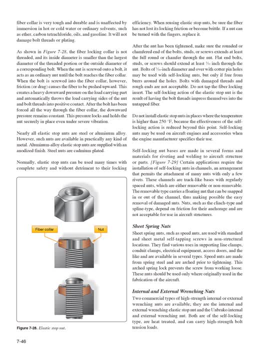 not damage bolt threads or plating. As shown in figure 7-28,, the fiber-locking collar is not threaded and its inside diameter is smaller than the largest diameter of the threaded portion or the outside diameter of a corresponding bolt. When the nut is screwed onto a bolt, it acts as an 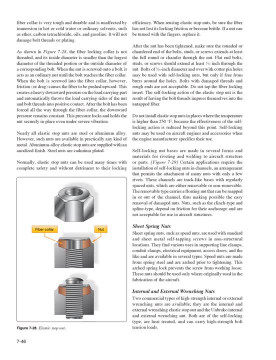 ordinary nut until the bolt reaches the fiber collar. When the bolt is screwed into the fiber collar, however, friction or drag causes the nut to be tightened. This is a very important point in the case of a bolt. When the bolt is screwed into the fiber collar, however, friction or drag causes. 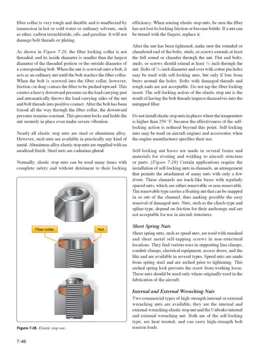 the fiber to be pushed upward. This creates a heavy downward pressure on the load-carrying part and automatically throws the load-carrying sides of the nut and bolt threads into positive contact. After the bolt has been forced all the way through the fiber collar, the downward pressure remains. 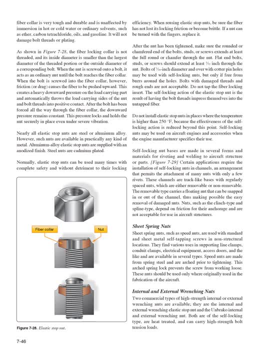 constant. This pressure locks and holds the nut securely in place, even under severe vibration. Nearly all elastic stop nuts are steel or aluminum alloy. However, such nuts are available in practically any kind of metal. Aluminum alloy elastic stop nuts are supplied with an anodized finish. Steel nuts are cadmium-plated Normally. 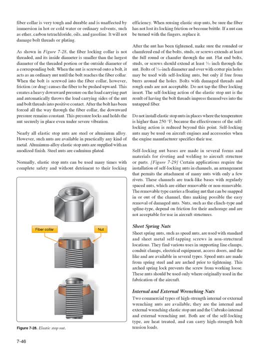 elastic stop nuts can be used many times with complete safety and without detriment to their locking efficiency. When reusing elastic stop nuts, be sure the fiber has not lost its locking friction or become brittle. If a nut can be turned with the fingers, replace it After the nut has been tightened. 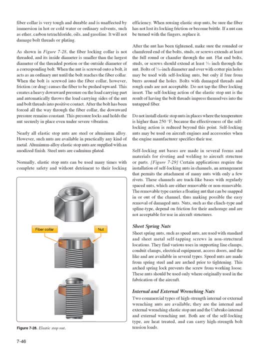 make sure the rounded or chamfered end of the bolts, studs or screws extends at least the full round or chamfer through the nut. Flat-end bolts, studs or screws should extend at least 1 32nd inch through the nut. 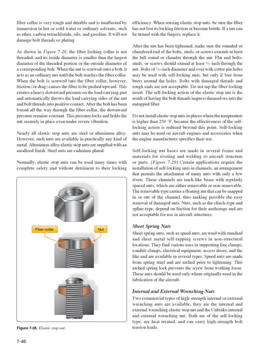 Bolts of 5 16th inch diameter and over with cotter pan holes may be used with self-locking nuts, but only if free from burrs around the holes. Bolts with damaged threads and rough ends are not acceptable. Do not tap the fiber locking insert. 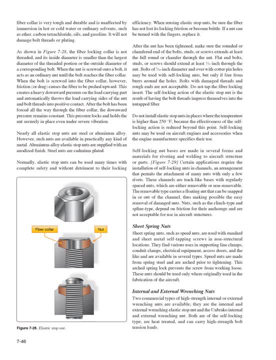 The self-locking action of the elastic stop nut is the result of having the bolt threads impress themselves into the untapped fiber. Do not install elastic stop nuts in places where the temperature is higher than 250 degrees Fahrenheit, because the effectiveness of the self-locking action is reduced beyond this point. 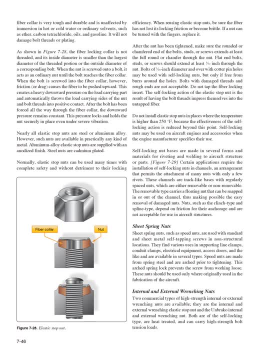 Self-locking nuts may be used on aircraft engines and accessories when the engine manufacturer specifies their use. Self-locking nut bases are made in several forms and materials for riveting and welding to aircraft structure or parts- Figure 7-29,. certain applications require the installation of self-locking nuts in channels. 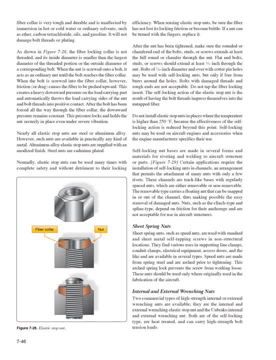 an arrangement That permits the attachment of many nuts with only a few rivets. These channels are track-like bases with regularly spaced nuts, which are either removable or non-removable. The removable type carries a floating nut that can be snapped in or out of the channel. 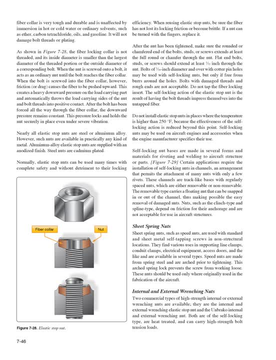 thus making possible the easy removal of damaged nuts. Nuts such as the clinch type and spline type depend on friction for their anchorage and are not acceptable for use in aircraft structures. Sheet spring nuts. Sheet spring nuts, such as speed nuts, are used with standard and sheet metal self-locking. 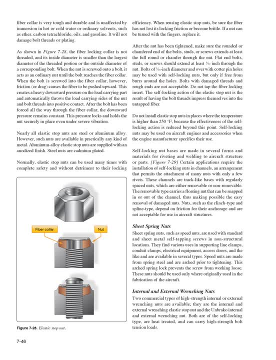 screws in non-structural locations. They find various uses in supporting line clamps, conduit clamps, electrical equipment, access doors and the like, and are available in several types. Speed nuts are made from spring steel and are arched prior to tightening. 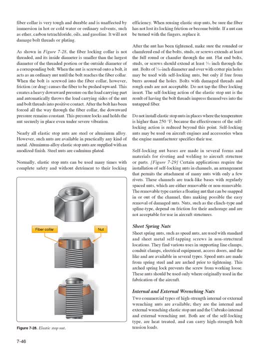 This arched spring lock prevents the screw from working loose. These nuts should be used only where originally used in the fabrication of the aircraft. Internal and external wrenching nuts. Two commercial types of high-strength internal or external wrenching nuts are available. They are the internal and external wrenching elastic stop nut and the Umbraco internal. 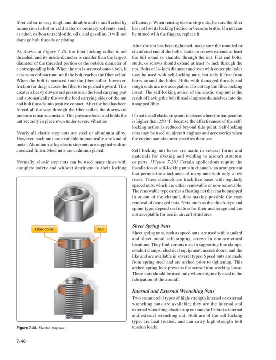 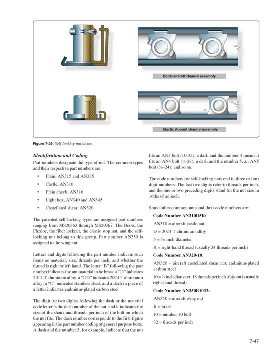 and external wrenching nut. Both are of the self-locking type, are heat-treated and can carry high-strength bolt tension loads. Identification and coding part numbers designate the type of nut. The common types and their respective part numbers are Plane AN315 and AN335. 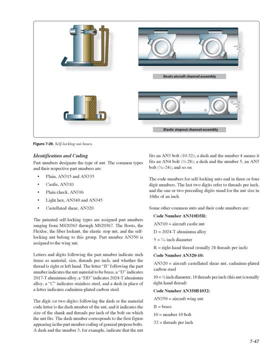 Castle- AN310. Plane Check- AN316. Light Hex- AN340 and AN345. Castellated Shear- AN320. The patented self-locking types are assigned part numbers ranging from MS20363 through MS20367.. The boots, the flex lock, the fiber lock nut, the elastic stop nut and the self-locking nut belong to this group. 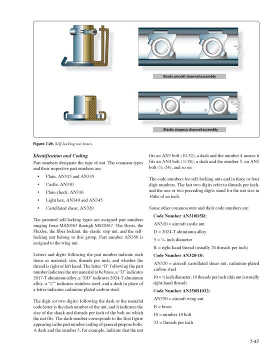 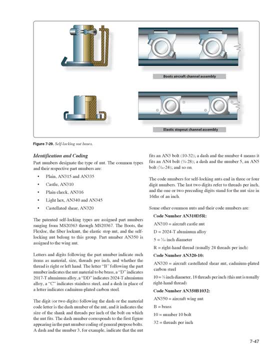 The letter B following the part number indicates the nut material to be brass, a D indicates 2017 T aluminum alloy. a DD indicates 2024 T aluminum alloy. a C indicates stainless steel and a dash in place of a letter indicates cadmium-plated carbon steel. 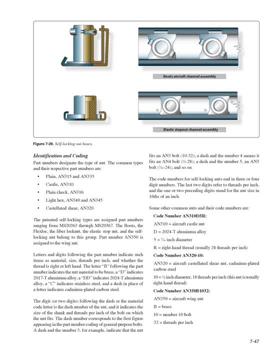 The digit or two digits following the dash or the material code letter is the dash number of the nut and it indicates the size of the shank and threads per inch of the bolt on which the nut fits. The dash number corresponds to the first figure appearing in the part number. coding of general. 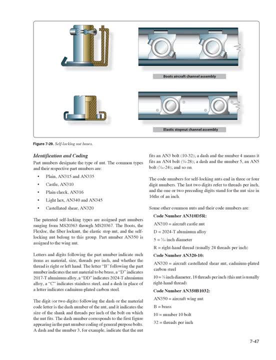 purpose bolts. A dash and the number 3,, for example, indicate that the nut fits an AN3 bolt 10 to 32,. a dash and the number 4 means it fits an AN4 bolt 1 quarter minus 28,. a dash and the number. 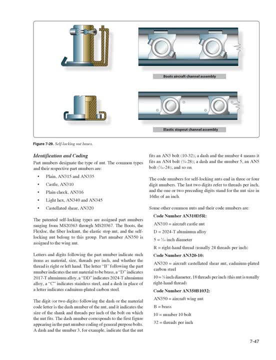 5, an AN5 bolt, 5 sixteenths minus 24, and so on. The code numbers for self-locking nuts end in 3 or 4 digit numbers. The last two digits refer to threads per inch And the one or two preceding digits stand for the nut size in sixteenths of an inch. 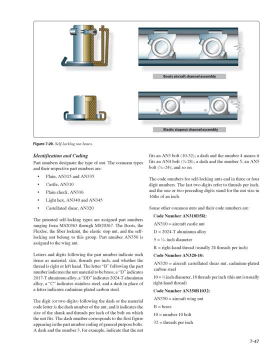 Some other common nuts and their code numbers are: code number AN310D5R. AN310A equals aircraft. castle nut D equals 2024 T. aluminum alloy 5 equals 5 sixteenths inch diameter equals right hand thread, usually 24 threads per inch. code number AN32010, AN320 equals aircraft. 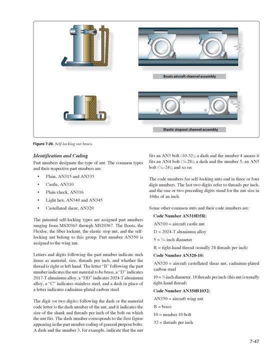 castellated shear nut. cadmium-plated carbon steel. 10 equals 5 eighths inch diameter, 18 threads per inch. this nut is usually right hand thread code number: AN350B1032,. AN350 equals aircraft wing nut. B equals brass. 10 equals number 10. bolt: 32 equals threads per inch. 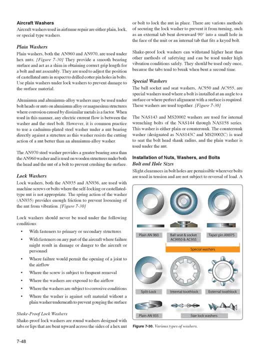 Aircraft washers. Aircraft washers used in airframe repair are either plain lock or special type washers. Plain washers. Plain washers- both the AN960 and AN970, are used under hex nuts Figure 7 to 30, they provide a smooth bearing. 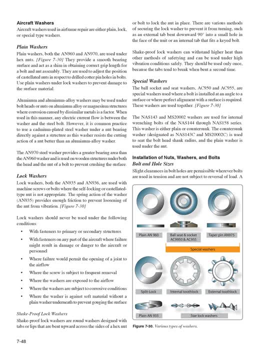 smooth surface and act as a shim in obtaining correct grip length for a bolt and nut assembly. They are used to adjust the position of castellated nuts in respect to drilled cotter, pin holes and bolts. Use plain washers under lock washers to prevent damage to the surface material. 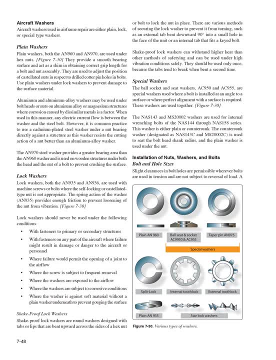 Aluminum and aluminum alloy washers may be used under bolt heads or nuts on aluminum, alloy or magnesium structures where corrosion caused by dissimilar metals is a factor. When used in this manner, any electric current flow is between the washer and the steel bolt. However, it is common practice to use a cadmium-plated steel washer under a nut bearing. 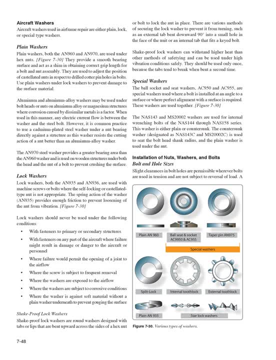 directly against a structure, as this washer resists the cutting action of a nut better than an aluminum alloy washer. The AN970 steel washer provides a greater bearing area than the AN960 washer and is used on wooden structures under both the head and the nut of a bolt. to 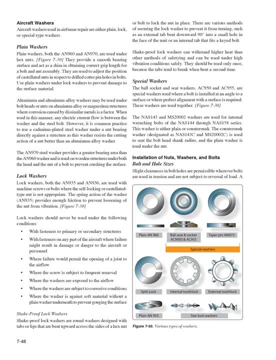 prevent crushing the surface Lock washers. Lock washers- both the AN935 and AN936, are used with machine screws or bolts where the self-locking or castellated type nut is not appropriate. The spring action of the washer- AN935, provides enough friction to 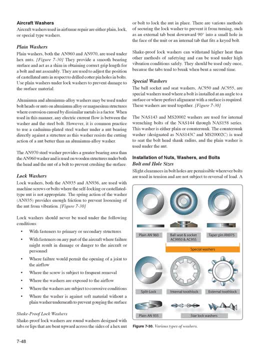 prevent loosening of the nut from vibration- Figure 730,. lock washers should never be used under the following conditions: With fasteners to primary or secondary structures. with fasteners on any part of the aircraft where failure might result in damage or danger to the aircraft, or 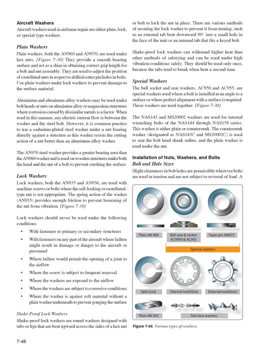 personnel where failure would permit the opening of a joint to the airflow. where the screw is subject to frequent removal. where the washers are exposed to the airflow. where the washers are subject to corrosive conditions. where the washer is against soft material without a plain washer. 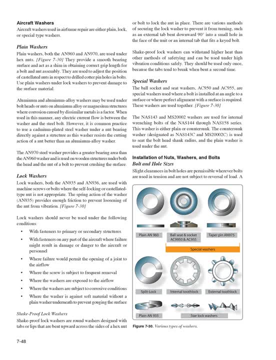 underneath to prevent gouging the surface. Shake-proof lock washers. Shake-proof lock washers are round washers designed with tabs or lips that are bent upward across the sides of a hex, nut or bolt to lock the nut in place. There are various methods of securing the lock washer. 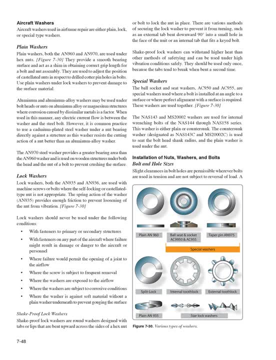 to prevent it from turning, such as an external tab bent downward 90 degrees into a small hole in the face of the unit, or an internal tab that is bent downward 90 degrees into a small hole in the face of the unit, or internal tab that fits a keyed bolt. Shake-proof lock washers can withstand. 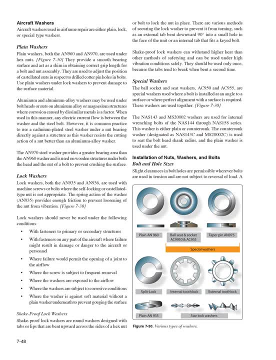 higher heat than other methods of safetying and can be used under high vibration conditions. safely, They should be used only once, because the tabs tend to break when bent a second time. Special washers- The ball socket and seat washers AC950 and AC955, are special washers used where 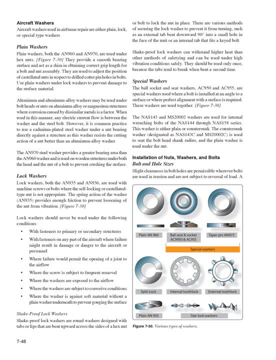 a bolt is installed at an angle to a surface or where perfect alignment with the surface is required. These washers are used together: Figure 730. Figure 730. The NAS143 and MS20002 washers are used for internal wrenching bolts of the NAS144 through. 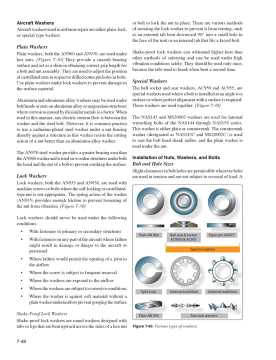 NAS158 series. This washer is either plain or countersunk. The countersunk washer, designated as NAS143C and MS20002C, is used to seat the bolt head shank radius and the plain washer is used under the nut Installation of nuts washers and bolts. Bolt and hole sizes like clearances in bolt. 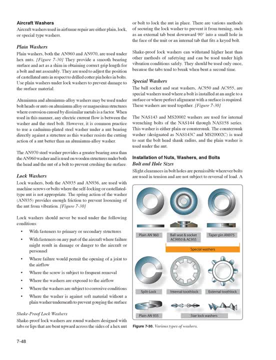 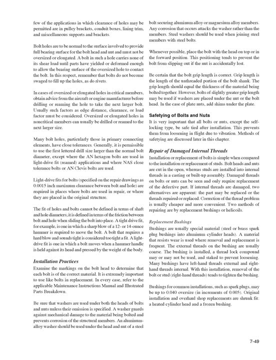 holes are permissible wherever bolts are used in tension and are not subject to reversal of load. A Few of the applications in which clearance of holes may be permitted are in pulley brackets, conduit boxes, lining trim and miscellaneous supports and brackets. Bolt holes are to be normal to the surface involved to provide full 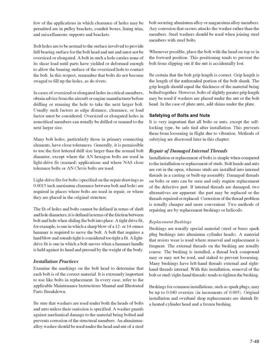 bearing surface for the bolt head and nut and must not be oversized or elongated. A bolt in such a hole carries none of its sheer load until parts have yielded or deformed enough to allow the bearing surface of the oversized hole to contact the bolt. In this respect, remember the 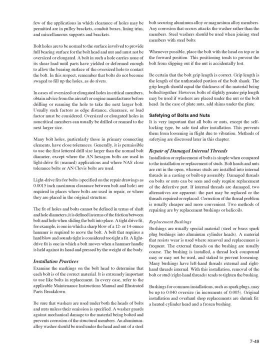 bolts do not become swash to fill up the holes, as do rivets. In cases of oversized or elongated holes in critical members, obtain advice from the aircraft or engine manufacturer before drilling or reaming the hole to take the next larger bolt, Usually such factors as edge distance clearance. 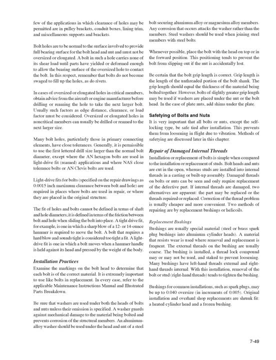 or load factor must be considered. Oversized or elongated holes in non-critical members can usually be drilled or reamed to the next larger size. Many bolt holes, particularly those in primary connecting elements, have close tolerances. Generally it is permissible to use the first letter drill size larger than the normal bolt. 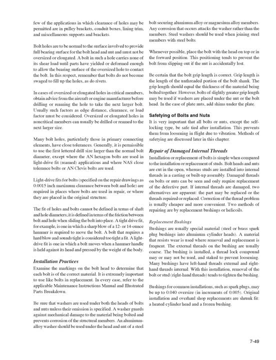 diameter, except where the in-hexagon bolts are used in light-drive fit reamed applications and where NAS close tolerance bolts or in-clevis bolts are used. Light-drive fits for bolts specified on the repair drawings as 0.0015 inch maximum clearance between bolt and hole. 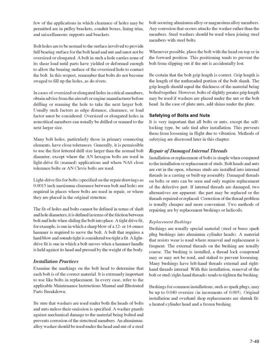 are required in places where bolts are used in repair or where they are placed in the original structure. The fit of holes and bolts cannot be defined In terms of shaft and hole diameters. it is defined in terms of the friction between bolt and hole when sliding the bolt into place. A tight-drive fit, for example, is one in which 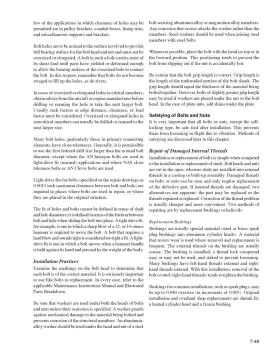 a sharp blow of a 12 or 14-ounce hammer is required to move the bolt. A bolt that requires a hard blow and sounds tight is considered too tight a fit. A light-drive fit is one in which a bolt moves when a hammer handle is held against its head and pressed by the weight of the body. 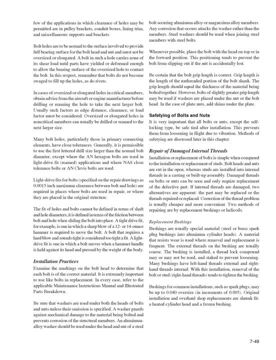 Installation practices. examine the markings on the bolt head to determine that each bolt is of the correct material. It is extremely important to use like bolts and replacement. In every case, refer to the applicable maintenance instructions, manual and illustrated parts breakdown. Be sure that washers. 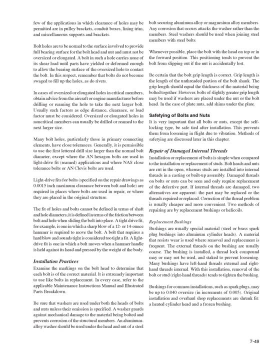 are used under both the heads of bolts and nuts unless their emission is specified. A washer guards against mechanical damage to the material being bolted and prevents corrosion of the structural members. An aluminum alloy washer should be used under the head and none of a steel bolt, securing aluminum alloy or magnesium alloy members Any corrosion that occurs under. 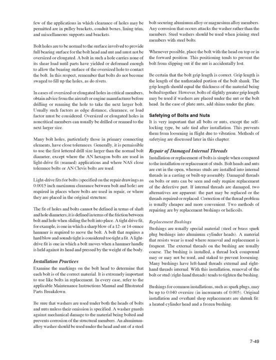 the head or aluminum alloy members should be used under the head and none of a steel bolt securing aluminum alloy members. Steel washers should be used when joining steel members with steel bolts. Whenever possible, place the bolt with the head on top or in the forward position. 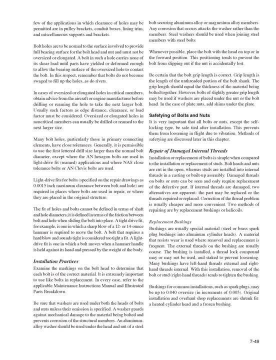 This positioning tends to prevent the bolt from slipping out if the nut is accidentally lost. Be certain that the bolt grip length is correct. Grip length is the length of the unthreaded portion of the bolt shank. The grip length should equal the thickness of 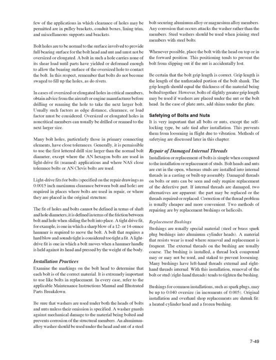 the material being bolted together. However, bolts of slightly greater grip length may be used if washers are placed under the nut or the bolt head. In the case of plate nuts, add shims under the plate. Safetying of bolts and nuts. It is very important that all bolts or nuts 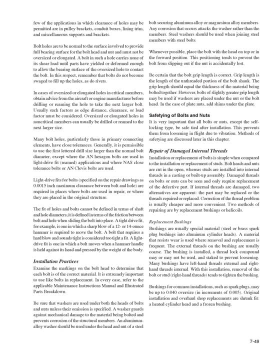 except the self-locking type, be safe-tied after installation. This prevents them from loosening in flight due to vibration. Methods of safetying are discussed later in this chapter. Repair of damaged internal threads, Installation or replacement of bolts is simple when compared. 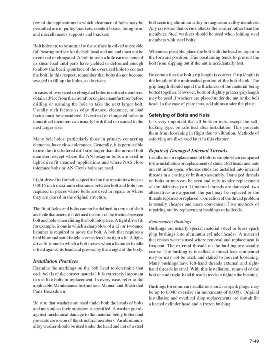 to the installation or replacement of studs. Bolt heads and nuts are cut in the open, whereas studs are installed into internal threads in a casting or built-up assembly. Damaged threads on bolts or nuts can be seen and only require replacement of the defective part. If internal threads are damaged, two alternatives are apparent. The part may be replaced or the threads repaired or replaced. Correction of the thread problem is usually cheaper and more convenient. Two methods of repairing are by replacement bushings or helicoils. Replacement bushings. Bushings are usually special material: steel or brass spark plug. 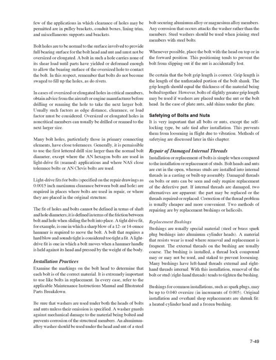 into aluminum cylinder heads. A material that resists wear is used where removal and replacement is frequent. The external threads on the bushing are usually coarse. The bushing is installed- a threadlock compound may or may not be used and staked to prevent loosening Many 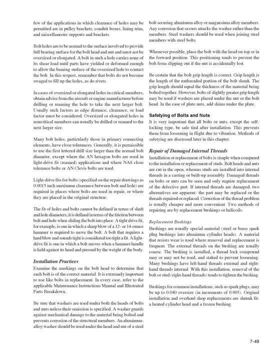 bushings have left-hand threads external and right-hand threads internal. With this installation, removal of the bolt or stud right-hand threads tends to tighten the bushing. Bushings for common installations such as spark plugs may be up to the top of the bushing. 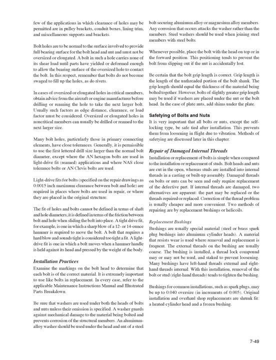 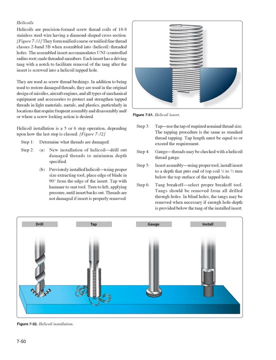 0.040. Oversize in increments of 0.005. Original installation and overhaul shop replacements are shrunk fit a heated cylinder head and a frozen bushing Helicoils. Helicoils are precision-formed screw thread coils of 18-8 stainless steel wire having a 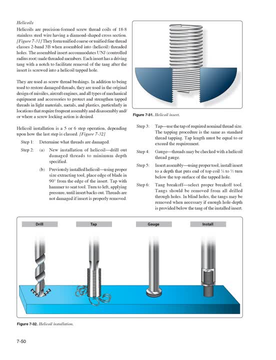 diamond-shaped cross-section, Figure 731,. they form unified coarse or unified fine thread classes to band 3B. when assembled into helicoil threaded holes, The assembled insert. a couple of times Each insert has a driving tang with a notch to facilitate removal of the tang after. 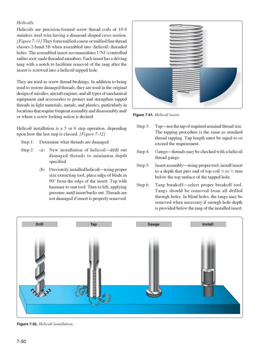 the insert is screwed into a helicoil tap hole. They are used as screw thread bushings. In addition to being used to restore damaged threads, they are used in the original design of missiles, aircraft engines and all types of mechanical equipment and accessories to protect and 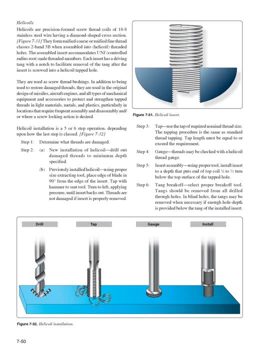 strengthen tap threads in light materials, metals and plastics, particularly in locations that require frequent assembly and disassembly: 0.040 Oversize in increments of 0.005 disassembly and slash, or where a screw locking action is desired. Helicoil installation is a. 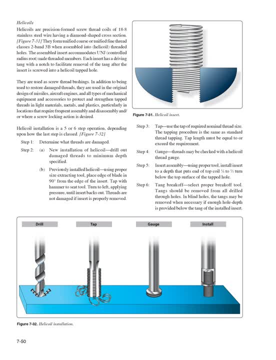 five- or six-step operation, depending upon how the last step is classed. Figure 732, Step 1, determine what threads are damaged. Step 2, A- new installation of helicoil. drill out damaged threads to minimum depth specified. B. previously installed helicoil. 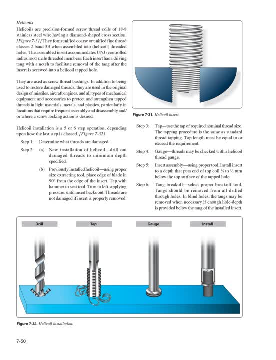 using proper size extracting tool. place edge of blade in 90 degrees from the edge of the insert. Tap with hammer to see tool Turn to left, applying pressure until insert backs out. Threads are not damaged if insert is properly removed. Step 3, tap. use the tap of required nominal thread size. The tapping 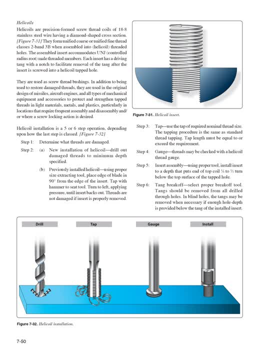 procedure is the same as standard thread tapping. Tap length must be equal to or exceed the requirement. Step 4, gauge threads may be checked with a helicoil thread gauge. Step 5, insert assembly using proper tool. install. insert to a depth that puts end of top coil one quarter. 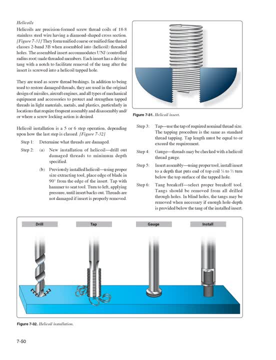 to half turn below the top coil. Step 5, insert assembly using proper tool. install insert to a top surface of the tapped hole. Step 6, tang break-off: select proper break-off tool. Tangs should be removed from all drilled through holes. In blind holes the tangs may be removed. 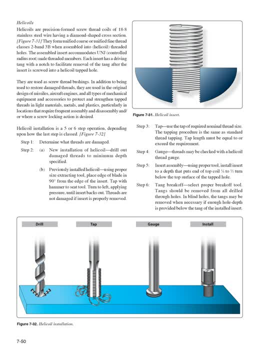 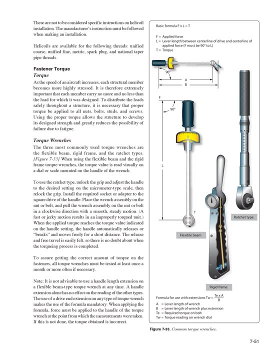 when necessary, if enough hole depth is provided below the tang of the installed insert. These are not to be considered specific instructions on helicoil installation. The manufacturer's instruction must be followed when making an installation. Helicoils are available for the following threads: unified coarse. unified fine. 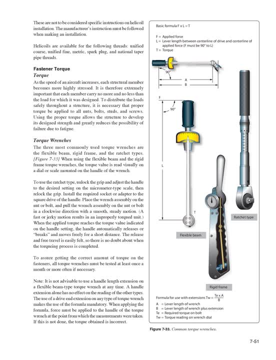 metric spark plug and national taper pipe threads. Fastener torque: torque. as the speed of an aircraft increases, each structural member becomes more highly stressed. It is therefore extremely important that each member carry no more and no less than the load for which it was designed. 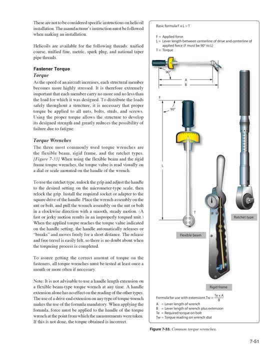 To distribute the loads safely throughout a structure, it is necessary that proper torque be applied to all nuts, bolts, studs and screws. Using the proper torque allows the structure to develop its design strength and greatly reduces the possibility of failure due to fatigue. Torque wrenches: The three most commonly used torque wrenches are: the flexible beam. 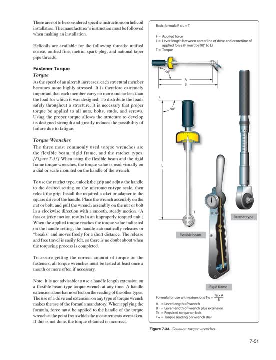 rigid frame and the ratchet types- Figure 733,. when using the flexible beam and the rigid frame torque wrenches, the torque value is read visually on a dial or scale mounted on the handle of the wrench. To use the ratchet type, unlock the grip and adjust the handle to the desired setting on. 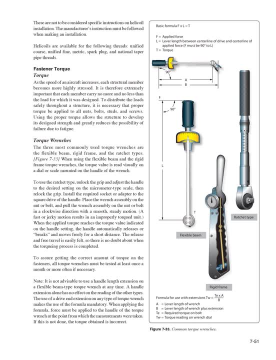 the micrometer type scale. then relock the grip, Install the required socket or adapter to the square drive of the handle, Place the wrench assembly on the nut or bolt. and install the wrench assembly on the nut or bolt in a clockwise direction with a smooth, steady motion, A fast or 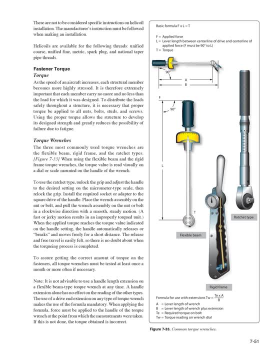 jerky motion results in an improperly torqued unit. When the applied torque reaches the torque value indicated on the handle setting, the handle automatically releases or breaks and moves freely for a short distance. The release and free travel is easily felt, so there is no doubt about when. 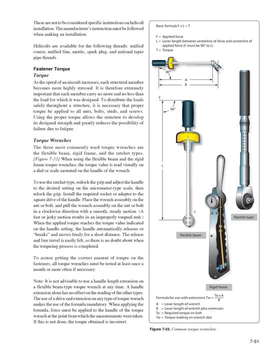 the torquing process is completed. To assure getting the correct amount of torque on the fasteners, all torque wrenches must be tested at least once a month, or more if necessary. Note: it is not advisable to use a handle length extension on a flexible beam type. 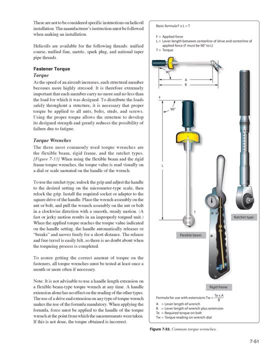 torque wrench at any time. A handle extension alone has no effect on the reading of the other types. The use of a drive end extension on any type of torque wrench makes the use of the formula mandatory. When applying the formula, force must be applied to the handle of the torque wrench at 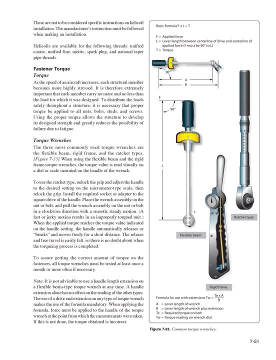 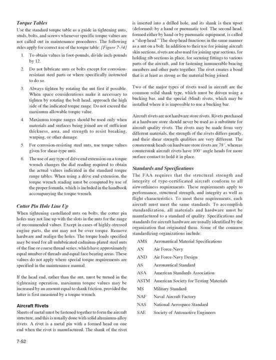 the point from which the measurements were taken. If this is not done, the torque obtained is incorrect. Torque tables. use the standard torque table as a guide In tightening nuts, studs, bolts and screws. whenever specific torque values are not called out in maintenance procedures. The following rules apply for correct use of the torque table: 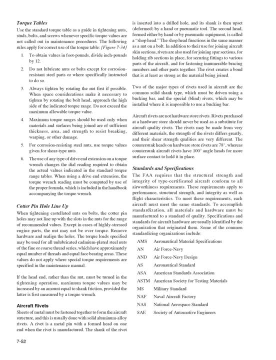 Figure 734-1.. To obtain values in foot-pounds, divide inch-pounds by 12.. 2. Do not lubricate nuts or bolts, except for corrosion-resistant steel parts or where specifically instructed to do so. 3. Always tighten by rotating the nut. 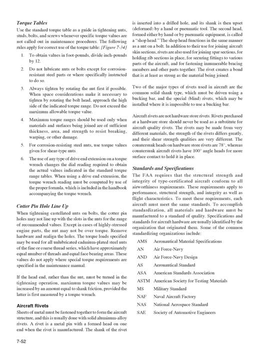 first, if possible, When space considerations make it necessary to tighten by rotating the bolt head, approach the high side of the indicated torque range. Do not exceed the maximum allowable torque value. 4. Maximum torque ranges should be used only when materials and surfaces being joined are of sufficient thickness, area and strength to 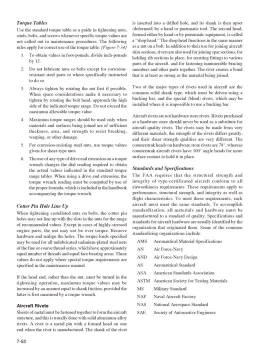 resist breaking, warping or other damage. 5. For corrosion-resisting steel nuts, use torque values given for shear-type nuts. 6. The use of any type of drive end extension on a torque wrench changes The dial reading required to obtain the actual values indicated in the standard torque range. 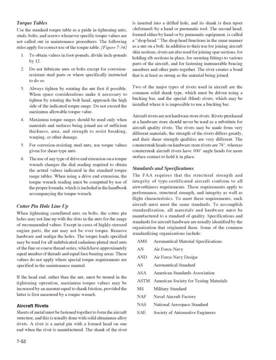 tables. When using a drive end extension, the torque wrench reading must be computed by use of the proper formula which is included in the handbook accompanying the torque wrench. Cutter pinhole line up. when tightening castellated nuts on bolts, The cutter pinholes may not line up. 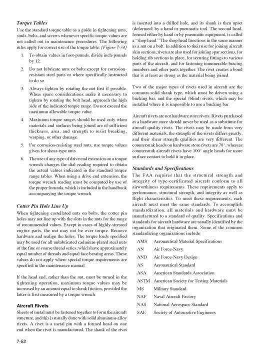 with the slots in the nuts for the range of recommended values. Except in cases of highly stressed engine parts, the nut may not be over torque. Remove hardware and realign the holes. The torque load specified may be used for all unlubricated cadmium-plated steel nuts of the 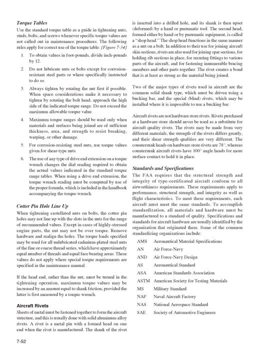 fine or coarse thread series which have approximately equal number of threads and equal face-bearing areas. These values do not apply where special torque requirements are specified in the maintenance manual. If the head end rather than the nut must be turned in the tightening operation, maximum torque values may be increased by an amount equal to shank friction. 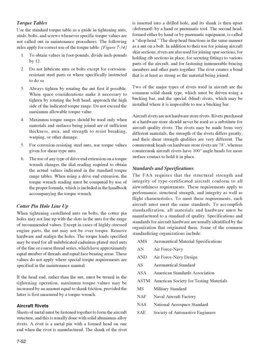 provided. the latter is first measured by a torque wrench. Aircraft rivet sheets of metal must be fastened together to form the aircraft structure, and this is usually done with solid aluminum alloy rivets. A rivet is a metal pin with a formed head on one end. when the rivet is manufactured, 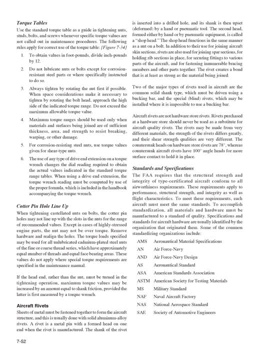 The shank of the rivet is inserted into a drilled hole and its shank is then upset, deformed by a hand or pneumatic tool. The second head, formed either by hand or by pneumatic equipment, is called a shop head. The shop head functions in the same manner as a nut on a bolt. 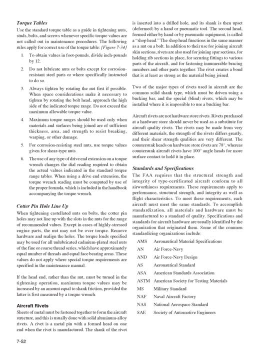 In addition to their use for joining aircraft skin sections, rivets are also used for joining spar sections, for holding rib sections in place, for securing fittings to various parts of the aircraft and for fastening innumerable bracing members and other parts. 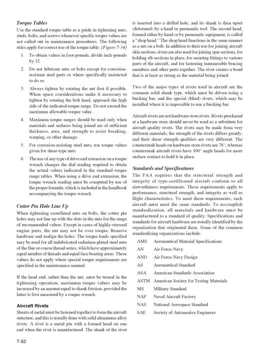 together, The rivet creates a bond that is at least as strong as the material being joined. Two of the major types of rivets used in aircraft are the common solid shank type, which must be driven using a bucking bar, and the special blind rivets, which may be installed. 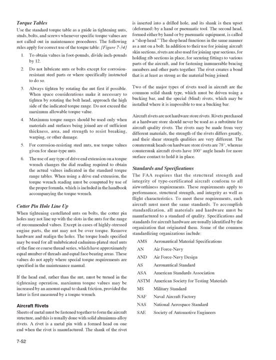 where it is impossible to use a bucking bar. Aircraft rivets are not hardware store rivets. Rivets purchased at a hardware store are not hardware store rivets. Hardware stores should never be used as a substitute for aircraft quality rivets. The rivets may be made from very different materials. the strength of the rivets differs. 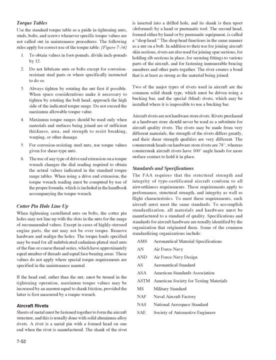 greatly and their sheer strength qualities are very different. The countersunk heads on hardware store rivets are 78 degrees, whereas countersunk aircraft rivets have 100 degrees angle heads for more surface contact to hold it in place. Standards and specifications, the FAA. 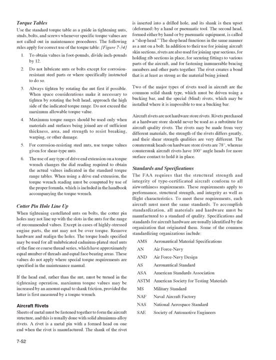 requires that the structural strength and integrity of type certificated aircraft conform to all airworthiness requirements. These requirements apply to performance, structural strength and integrity, as well as flight characteristics. To meet these requirements, each aircraft must meet the same standards. To accomplish standardization, all materials and hardware must be manufactured. 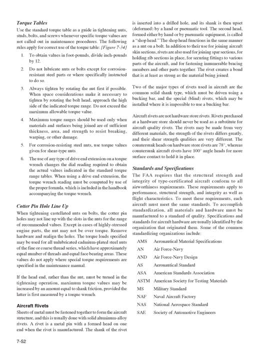 to a standard of quality. Specifications and standards for aircraft hardware are usually identified by the organization that originated them. Some of the common standardizing organizations include AMS- Aeronautical Materials Specifications, and Air Force Navy and Air Force Navy Design is Aeronautical Standard. ASA- American Standards Association, ASTM- American Society. 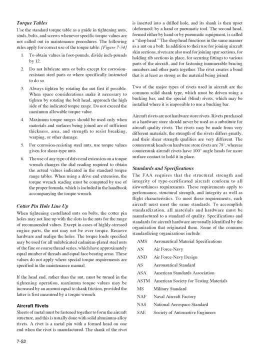 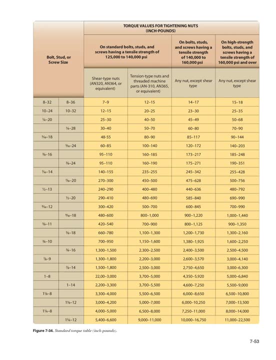 for Testing Materials: MS Military Standard, NAF Naval Aircraft Factory, NAS, National Aerospace Standard, SAE- Society of Automotive Engineers On standard bolts, studs and screws having a tensile strength of 125,000 to 140,000 pounds per square inch. bolt, stud or screw size torque. 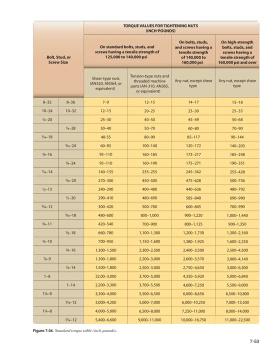 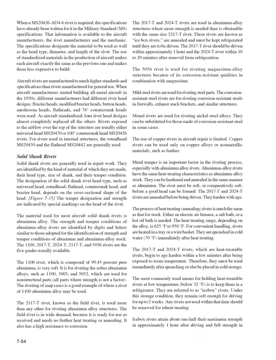 values for tightening nuts: inch degrees. pounds on high strength on bolts, studs. bolts, studs and screws having a screws having a tensile strength: tensile strength of 140,000 to 160,000 pounds per square inch and over 160,000 pounds per square inch When a MS 20426AD 4-6 rivet. 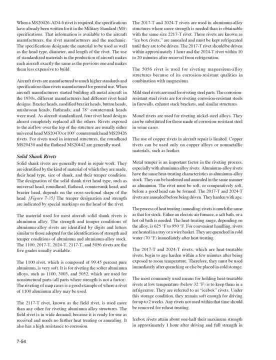 is required. the specifications have already been written for it in the Military Standard MS Specifications. That information is available to the aircraft manufacturers, the rivet manufacturers and the mechanic. The specifications designate the material to be used, as well as the head type, diameter and length of the rivet. The use of standardized materials in the production. 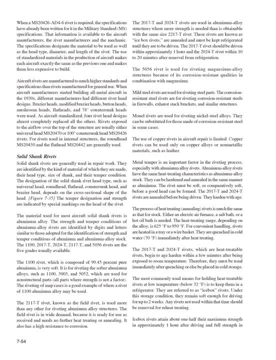 of aircraft makes each aircraft exactly the same as the previous one and makes them less expensive to build. Aircraft rivets are manufactured to much higher standards and specifications than rivets manufactured for general use. When aircraft manufacturers started building all-metal aircraft in the 1930s, different manufacturers had different rivet head designs- Brazier heads. 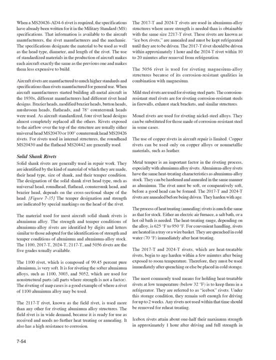 modified brazier heads, button heads, mushroom heads, flatheads and 78 degrees countersunk heads were used As aircraft standardized. four rivet head designs almost completely replaced all the others. Rivets exposed to the airflow over the top of the 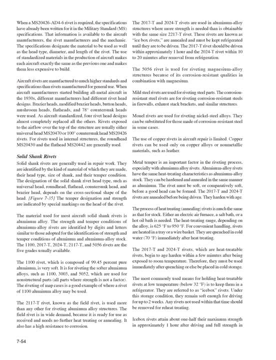 structure are usually either universal head- MS 20470- or 100 degrees countersunk head- MS 20426. rivets: For rivets used in internal structures, the roundhead MS 20430 and the flathead MS 20442 are generally used. 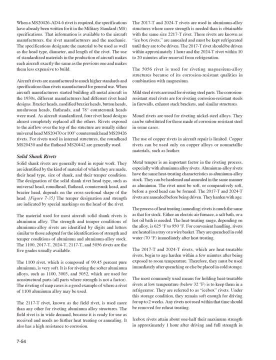 Solid shank rivets. Solid shank rivets are generally used in repair work. They are identified by the kind of material of which they are made, their head type, size of shank and their temper condition. The designation of the solid shank rivet head type. 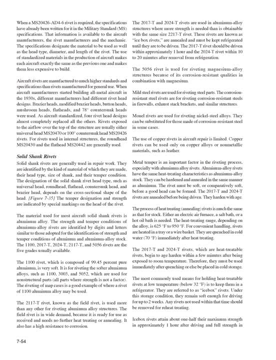 such as universal head, roundhead, flathead, countersunk head and brazier head, depends on the cross-sectional shape of the head- Figure 7-35,. the temper, designation and strength are indicated by special markings on the head of the rivet, The material used for most aircraft. 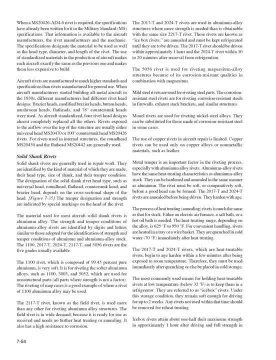 solid shank rivets is aluminum alloy. The strength and temper conditions of aluminum alloy rivets are identified by digits and letters similar to those adopted for the identification of strength and temper conditions of aluminum and aluminum alloy stock. The 1100, 2017, T, 2024, T, 2117, T and 5056. 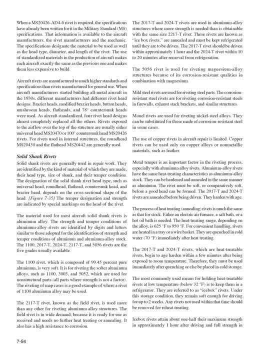 rivets are the five grades usually available. The 1100 rivet, which is composed of 99.45% pure aluminum, is very soft. It is for riveting the softer aluminum alloys, such as 1100,, 3003, and 5052, which are used for. 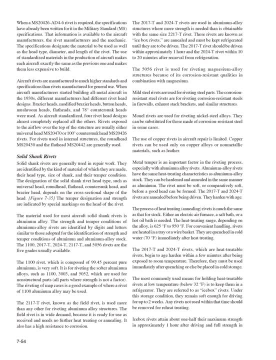 non-structural parts, all parts where strength is not a factor. The riveting of MAP cases is a good example of where a rivet of 1100 aluminum alloy may be used, The 2117 T rivet, known as the field. 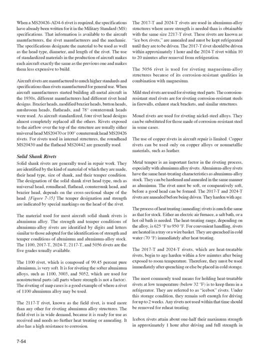 rivet is used more than any other for riveting aluminum alloy structures. The field rivet is in wide demand because it is ready for use as received and needs no maintenance. It also has a high resistance to corrosion. The 2017 T and 2024 T rivets are used in aluminum. 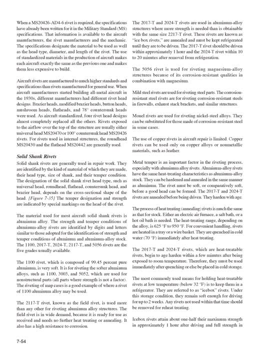 alloy structures where more strength is needed than is obtainable with the same size. 2217 T rivet. These rivets are known as icebox rivets, are annealed and must be kept refrigerated until they are to be driven. The 2017 T rivet should be driven within approximately one hour and the 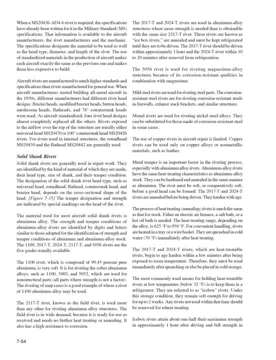 2024 T rivet within 10 to 20 minutes after removal. The 2056 T rivet is used for riveting magnesium alloy structures because of its corrosion-resistant qualities. in combination with magnesium, Mild steel rivets are used for riveting steel parts. The corrosion-resistant steel rivets are for riveting corrosion-resistant steels in firewalls, exhaust stack brackets and similar structures. Mono rivets are used for riveting nickel steel alloys. They can be substituted for those made of corrosion-resistant steel in some cases. The use of copper rivets in aircraft repair is limited. Copper rivets can be used only on copper alloys or non-metallic materials such as leather Metal. temper is an important factor in the process, especially with aluminum alloy rivets. Aluminum alloy rivets have the same heat-treating. 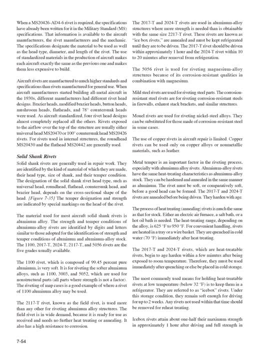 characteristics as aluminum alloy stock. They can be hardened and annealed in the same manner as aluminum. The rivet must be soft or comparatively soft before a good head can be formed. The 2017 T and 2024 T rivets are annealed. before being driven, They harden with age. The process of heat-treating annealing rivets is much the same as that for stock. Either an electric air furnace, a salt bath or a hot oil bath is needed. The heat-treating range, depending on the alloy, is 625 degrees Fahrenheit to 950 degrees Fahrenheit For convenient handling rivets. 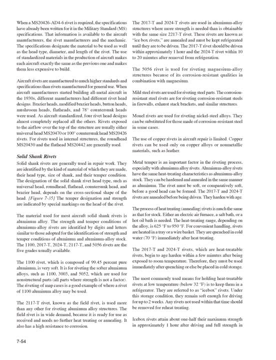 are heated in a tray or a wire basket. They are quenched in cold water 70 degrees Fahrenheit immediately after heat-treating. The 2017 T and 2024 T rivets, which are heat-treatable rivets. begin to age-harden within a few minutes after being exposed to room temperature. Therefore, they must be used immediately after quenching or else be placed in cold storage, The most commonly used means for holding heat-treatable rivets at low temperature. 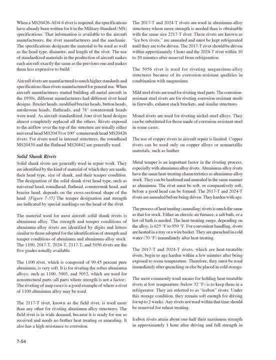 below 32 degrees Fahrenheit is to keep them in a refrigerator. They are referred to as icebox rivets. Under this storage condition, they remain in the refrigerator for a long time. They remain soft enough for driving for up to two weeks. 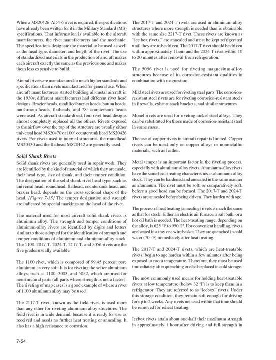 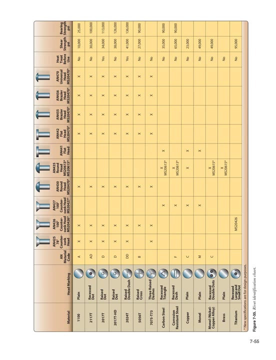 Any rivets not used within that time should be removed. for reheat-treating Icebox rivets attain about one-half their maximum strength in approximately one hour after driving in full strength in trahcnoitacifitneditevir53-7erugif. About four days. When 2017 T rivets are exposed to room temperature for one hour or longer, they must be subject to reheat treatment. This also applies to 2024T rivets exposed to room temperature for a period exceeding 10 minutes. Once an icebox rivet has been taken from the 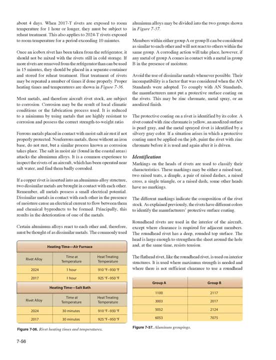 refrigerator. it should not be mixed with the rivets still in cold storage. If more rivets are removed from the refrigerator than can be used in 15 minutes, they should be placed in a separate container and stored for reheat treatment. Heat treatment of rivets may be repeated a number 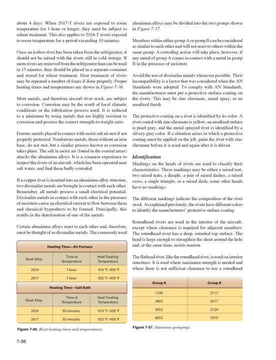 of times if done properly. Proper heating times and temperatures are shown in figure 736.. Most metals, and therefore aircraft rivet stock, are subject to corrosion. Corrosion may be the result of local climatic conditions or the fabrication process used. It is reduced to a 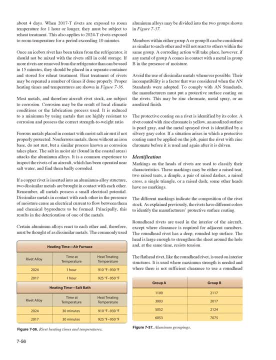 minimum by using metals that are highly resistant to corrosion and possess the correct strength to weight ratio. Ferrous metals placed in contact with moist salt air rust if not properly protected. Non-ferrous metals, those without an iron base, do not rust, but a similar process known as corrosion takes place. 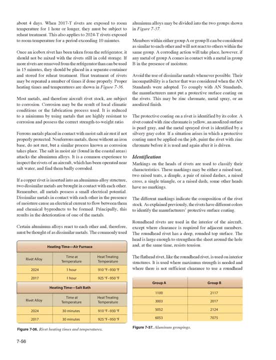 The salt in moist air found in the coastal areas attacks the aluminum alloys. It is a common experience to inspect the rivets of an aircraft which has been operated near salt water and find them badly corroded If a copper rivet is inserted into an aluminum alloy structure. 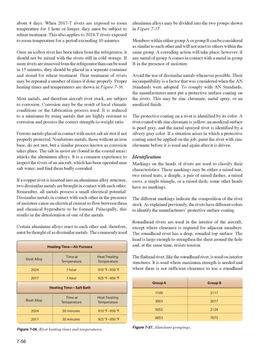 two dissimilar metals are brought in contact with each other. Remember, all metals possess a small electrical potential. Dissimilar metals in contact with each other in the presence of moisture cause an electrical current to flow between them and chemical byproducts to be formed. Principally, this results in the deterioration of one of the 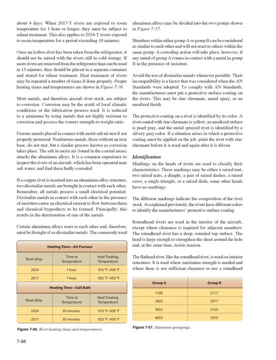 metals. Certain aluminum alloys react to each other and therefore must be thought of as dissimilar metals. The commonly used aluminum alloys may be divided into the two groups shown in figure 737.. Members within either group A or group B can be considered as similar to each other. 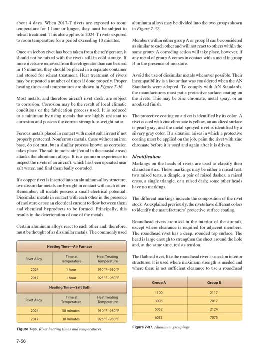 and will not react to others within the same group A. corroding action will take place, however, if any metal of group A comes in contact with a metal in group B in the presence of moisture. Avoid the use of dissimilar metals whenever possible. Their incompatibility is a factor. 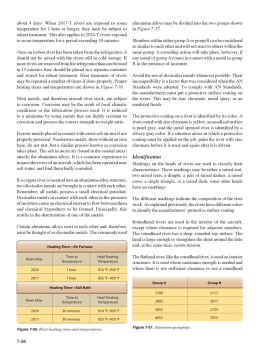 that was considered when the IN standards were adopted. To comply with IN standards, the manufacturers must put a protective surface coating on the rivets. This may be zinc, chromate metal spray or an anodized finish. The protective coating on a rivet is identified by its color. 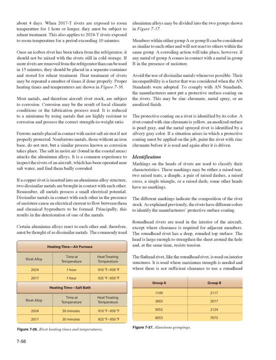 A rivet coated with zinc chromate is yellow, an anodized surface is pearl gray and the metal-sprayed rivet is identified by a silvery gray color. If a situation arises in which a protective coating must be applied on the job, 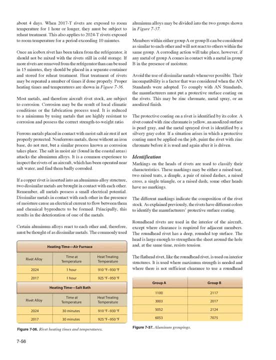 paint the rivet with zinc chromate before it is used and again after it is driven. Identification markings on the heads of rivets are used to classify their characteristics. These markings may be either a raised teat, two raised teats, a dimple, a pair of raised dashes. 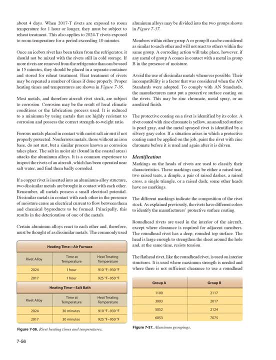 a raised cross, a single triangle or a raised dash. Some other heads have no markings. The different markings indicate the composition of the rivet stock. As explained previously, the rivets have different colors to identify the manufacturer's protective surface. coating. Roundhead rivets are used in the interior of the aircraft, except where 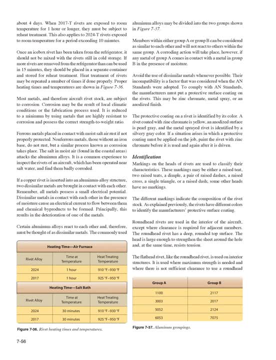 clearance is required for adjacent members. The roundhead rivet has a deep rounded top surface. The head is large enough to strengthen the sheet around the whole and at the same time resists tension. The flathead rivet, like the roundhead rivet, is used on interior structures. 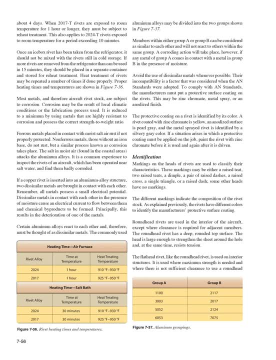 It is used where maximum strength is needed and where there is not sufficient clearance to use a roundhead. group A. group B: 1100, 2117, 3003, 2017, 5052,, 2124,, 6053, 7075. figure 737.. 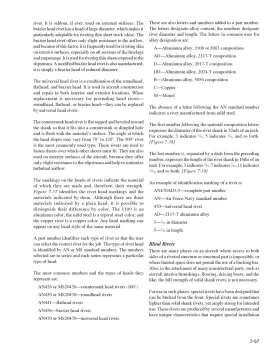 Aluminum groupings Rivet. It is seldom, if ever, used on external surfaces. The brazier head rivet has a head of large diameter which makes it particularly adaptable for riveting thin sheet stock skin. The brazier head rivet offers only slight resistance to the 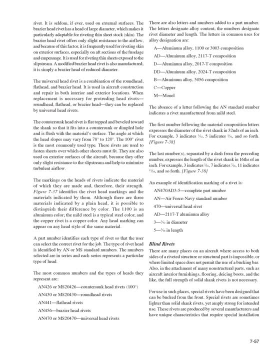 airflow, and because of this factor it is frequently used for riveting skin on exterior surfaces, especially on aft sections of the fuselage and empennage. It is used for riveting thin sheets exposed to the slipstream. A modified brazier head rivet is also manufactured. It is 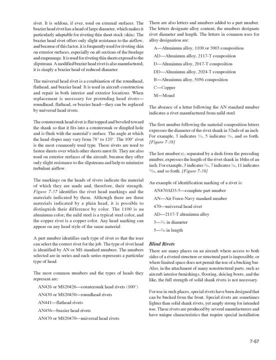 simply a brazier head of reduced diameter. The universal head rivet is a combination of the roundhead, flathead and brazier head. It is used in aircraft construction and repair in both interior and exterior locations When replacement is necessary for protruding head rivets- roundhead. 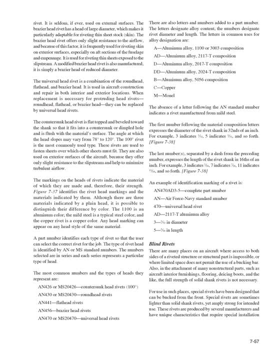 flathead or brazier head. they can be replaced by universal head rivets. The countersunk head rivet is flat-topped and beveled toward the shank so that it fits into a countersunk or dimpled hole and is flush with the material's surface. The angle at which the 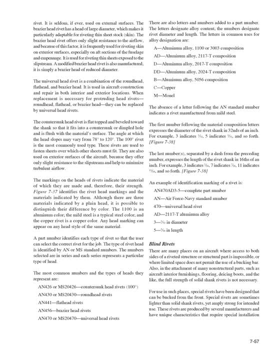 head slopes may vary from 78 degrees to 120 degrees. The 100 degrees rivet is the most commonly used type. These rivets are used to repair and repair the shank. They are used to fasten sheets over which other sheets must fit. They are also used on exterior. 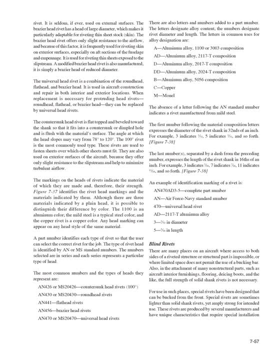 surfaces of the aircraft because they offer only slight resistance to the slipstream and help to minimize turbulent airflow. The markings on the heads of rivets indicate the material of which they are made and therefore their strength. Figure 7-37 identifies the rivet head markings. 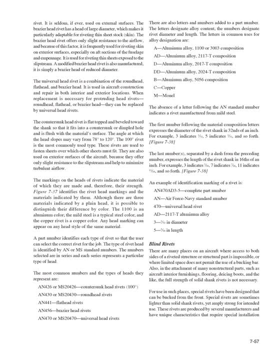 and the materials indicated by them. Although there are three materials indicated by a plain head, it is possible to distinguish their difference by color. The 1100 is an aluminum color, the mild steel is a typical steel color and the copper rivet is a 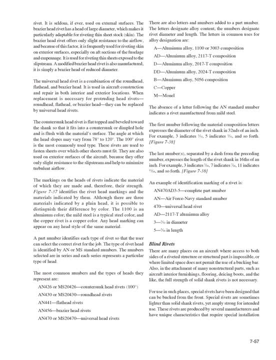 copper color. Any head marking can appear on any head style of the same material. A part number identifies each type of rivet so that the user can select the correct rivet for the job. The type of rivet head is identified by an or MS standard numbers. The numbers selected are in series and. 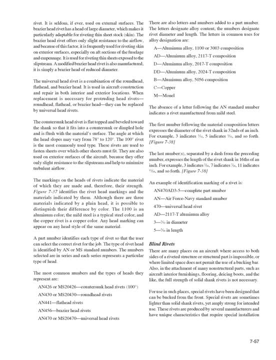 each series represents a particular type of head. The most common numbers and the types of heads they represent are: 426 or MS 20426, countersunk head rivets 100 degrees- AN. 430 or MS 20430, round head rivets- AN. 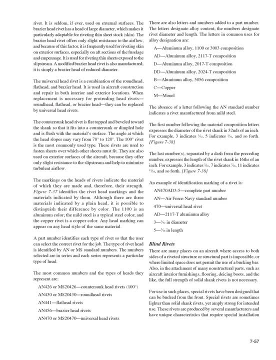 441, flat head rivets, AN 456, brazier head rivets, AN 470 or MS 20470, universal head rivets. there are also letters and numbers added to a part number. The letters designate alloy content. the numbers designate rivet diameter and length. The letters in common uses for: 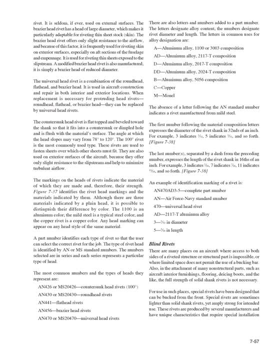 alloy designation are: A. Aluminum alloy 1100 or 3003. composition AD. Aluminum alloy 2117 T. composition D. Aluminum alloy 2017 T. composition DD. Aluminum alloy 2024 T. composition B. Aluminum alloy 5056. composition C. 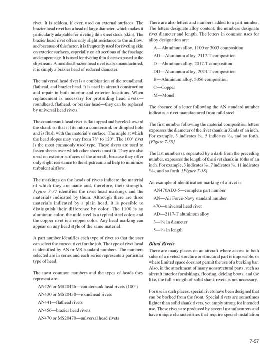 Copper M Model. The absence of a letter following the in standard number indicates a rivet manufactured from mild steel. The first number following the material composition letters expresses the diameter of the rivet shank in 32". For example, three indicates 3- 30 seconds, F 5 indicates 5- 30 seconds, and so forth. 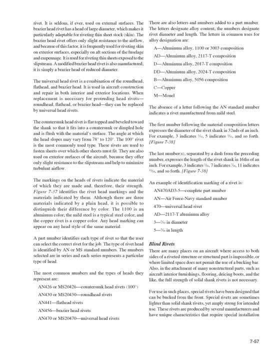 Figure 7- 38,. the last numbers, separated by aева dash from the preceding number, expresses the length of the rret shank in 16th of an inch. For example, three indicates 32, 1, 16,. seven indicates 7, 16, 1, 7 indicates 11, 1, 6, and so forth. figure 738,. 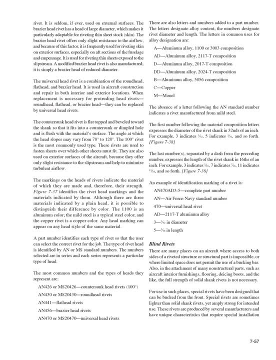 an example of identification marking that gives reasons for the differences. For example, 3 indicates 3- 16, of a rivet is AN-470AD-35, Complete Part Number and Air Force Navy Standard Number 470,. Universal Head Rivet AD-2117T Aluminum Alloy. 3, 3-30 seconds in diameter. 5, 5-16th in length. 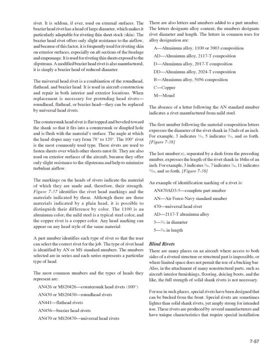 blind rivets. There are many places on an aircraft where access to both sides of a riveted structure or structural part is impossible or where limited space does not permit the use of a bucking bar. Also in the attachment of many non-structural parts such as aircraft interior furnishings. 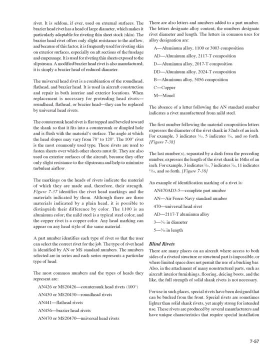 flooring, daising, boots and the like. the full strength of solid shank rivets is not necessary For use in such places. special rivets have been designed that can be bucked from the front. Special rivets are sometimes lighter than solid shank rivets, yet amply strong for intended use. 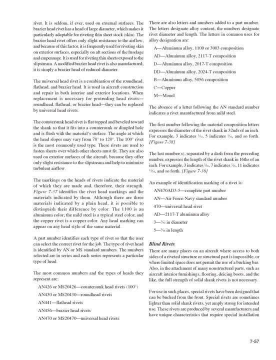 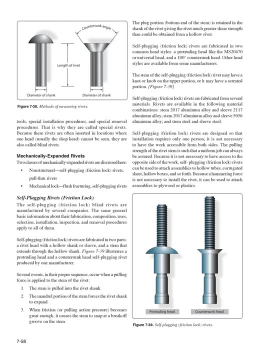 These rivets are produced by several manufacturers and have unique characteristics that require special installation Tools, Special installation procedures And special removal procedures. That is why they are called special rivets, Because these rivets are often inserted in locations where one head- usually the shop head- cannot be seen. they are also called blind rivets. 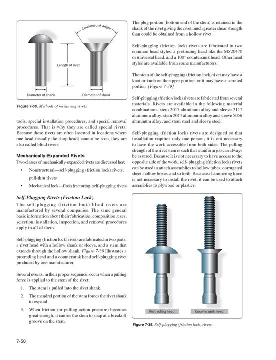 Mechanically expanded rivets. Two classes of mechanically expanded rivets are discussed here: Non-structural, Self-plugging Friction lock Rivets. Pull-through rivets. Mechanical lock: Flush fracturing Self-plugging rivets. Self-plugging rivets Friction lock. The self-plugging friction lock blind rivets are manufactured by several companies. 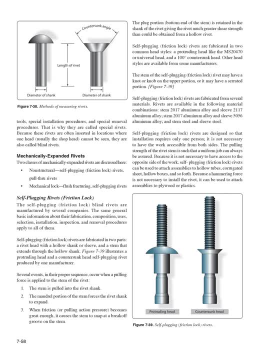 The same general basic information about their fabrication, composition, uses, selection, installation, inspection and removal procedures apply to all of them. Self-plugging friction lock rivets are fabricated in two parts: a rivet head with a hollow shank or sleeve, and a stem that extends through the hollow shank. 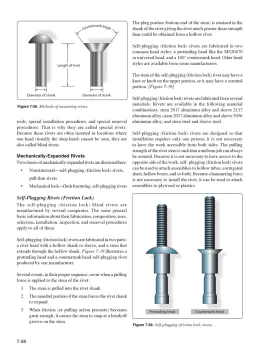 Figure 739 illustrates a protruding head and a countersunk head self-plugging rivet produced by one manufacturer. Several events, in their proper sequence, occur when a pulling force is applied to the stem of the rivet: 1. The stem is pulled into the rivet shank. 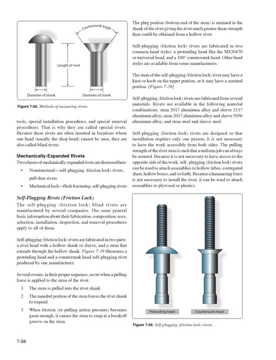 2. The mandrel portion of the stem forces the rivet shank to expand. 3. When friction or pulling action pressure becomes great enough, it causes the stem to snap. at a break-off groove on the stem, The plug portion, bottom end of the stem, is retained in the shank of the rivet, giving the rivet much greater shear strength than could be obtained from a hollow shank. 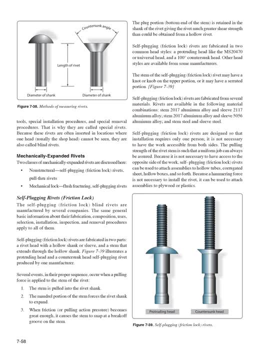 4. The self-plugging friction lock rivets are fabricated in two common head styles: a protruding head like the MS20470 or universal head, and a 100° countersunk head. Other head styles are available from some manufacturers. 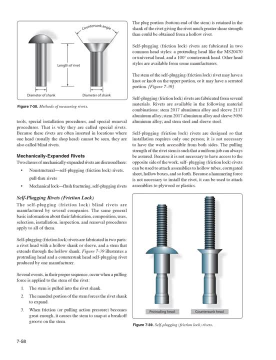 The stem of the self-plugging friction lock rivet may have a knot or knob on the upper portion, or it may have a serrated portion- Figure 739,. self-plugging friction lock rivets are fabricated from several materials. 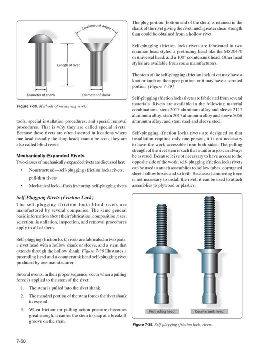 Rivets are available in the following material combinations: stem 2017- aluminum alloy and sleeve 2117- aluminum alloy. stem 2017- aluminum alloy and sleeve 5056- aluminum alloy and stem. steel and sleeve steel. Self-plugging friction lock rivets are designed so that installation requires only one person. it is not necessary to have the work accessible from both sides. 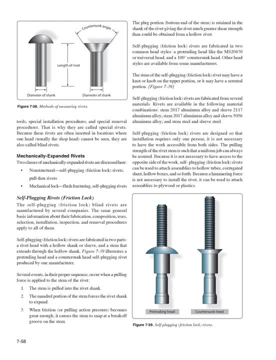 The pulling strength of the rivet stem is such that a uniform job can always be assured. Because it is not a single person, it is not necessary to have the work accessible from both sides. The pulling strength is such that- a single person- it is not necessary to have the work accessible from both sides. 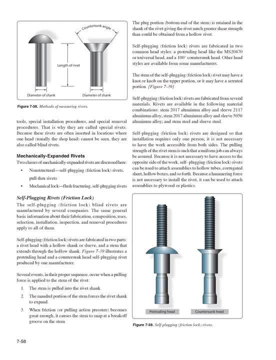 Because it is not a single person, it is not necessary to have the work accessible from both sides To have access to the opposite side of the work. self-plugging friction lock rivets can be used to attach assemblies to hollow tubes, corrugated sheets, hollow boxes and so forth. 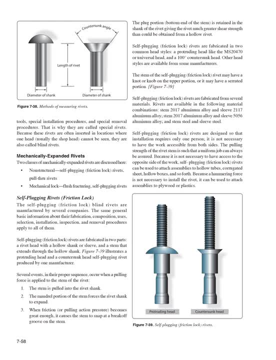 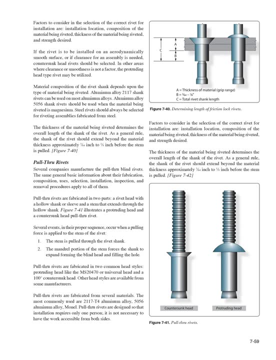 Because a hammering force is not necessary to install the rivet, it can be used to attach assemblies to plywood or plastics. Factors to consider in the selection of the correct rivet for installation are installation location, composition of the material being riveted, thickness of the material being riveted and strength desired. 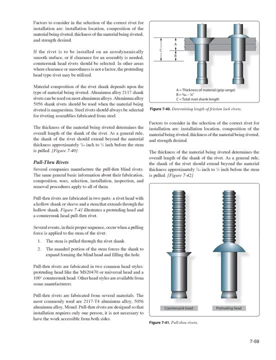 If the rivet is too thick, the rivet must be asked to beудь. If the rivet is to be installed on an aerodynamically smooth surface or if clearance for an assembly is needed, countersunk head rivets should be selected. 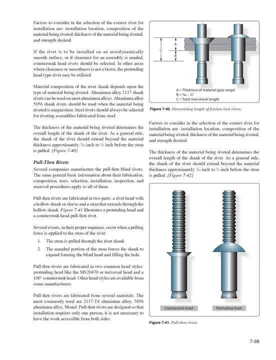 In other areas, where clearance or smoothness is not a factor, the protruding head type rivet may be utilized. Material composition of the rivet shank depends upon the type of material being riveted. Aluminum alloy: 2117 shank rivets can be used on most aluminum alloys. 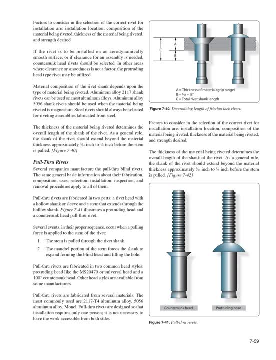 Aluminum alloy 5056 shank rivets should be used when the material being riveted is magnesium. Steel rivets should always be selected for riveting assemblies fabricated from steel. The thickness of the material being riveted determines the overall length of the shank of the rivet. 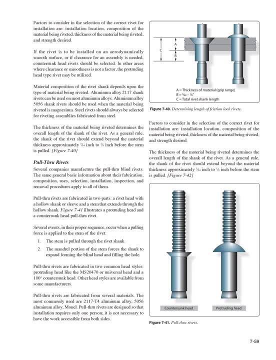 As a general rule, the shank of the rivet should extend beyond the material thickness, approximately 3, 64 inch to 1, 8 inch before the stem is pulled. Figure 740, pull-through rivets. Several companies manufacture the pull-through blind rivets. 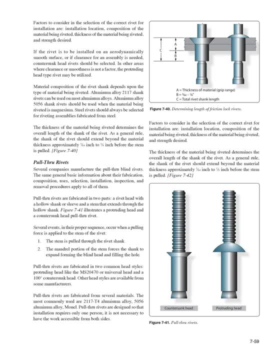 The same general basic information about their fabrication, composition, uses, selection, installation, inspection and removal procedures apply to all of them. Pull-through rivets are fabricated in two parts: a rivet head with a hollow shank or sleeve, and a stem that extends through the hollow shank. 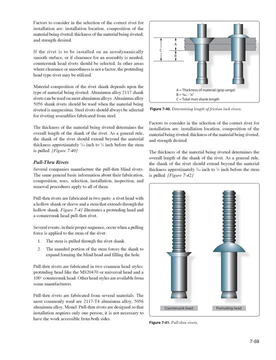 Figure 741 illustrates a protruding head and a countersunk head. pull-through rivet. Several events, in their proper sequence, occur when a pulling force is applied to the stem of the rivet. 1. The stem is pulled through the rivet. 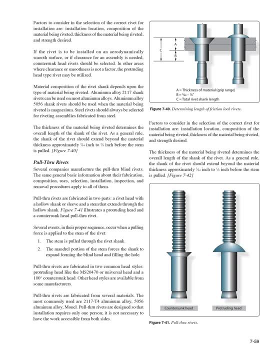 2. The mandrel portion of the stem forces the shank to expand, forming the blind head and filling the hole. Pull-through rivets are fabricated in two common head styles: protruding head, like the MS20470, or universal head, and a 100 degrees countersunk head. 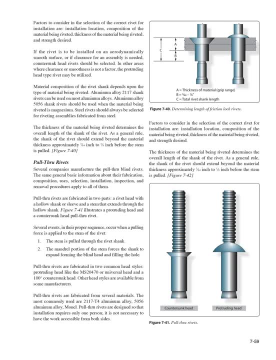 Other head styles are available from some manufacturers. Pull-through rivets are fabricated from several materials. The most commonly used are 2117T4 aluminum alloy, 5056 aluminum alloy and 2117T4 aluminum alloy. Pull-through rivets are designed so that installation requires only one person. 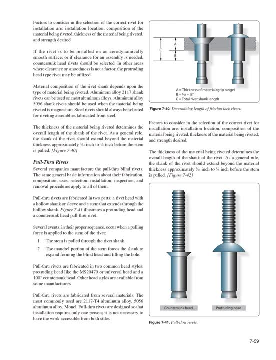 It is not necessary to have the work accessible from both sides. Factors to consider in the selection of the correct rivet for installation are installation location, composition of the material being riveted, thickness of the material being riveted and strength desired. The thickness of the material being riveted determines the overall length of the shank of the rivet. 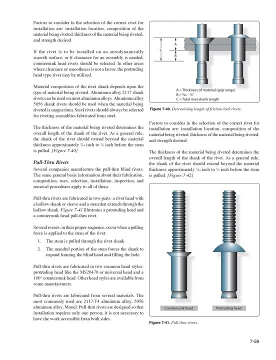 As a general rule, the shank of the rivet should extend beyond the material thickness, approximately 3 cm. The shank should be 1 1⁄64 inch to 1 1⁄8 inch before the stem is pulled. 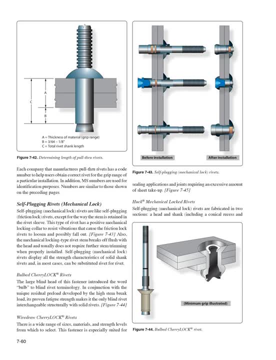 Figure 742. Each company that manufactures pull-through rivets has a code number to help users obtain correct rivet for the grip range of a particular installation. In addition, MS numbers are used for identification purposes. Numbers are similar to those shown on the preceding pages. 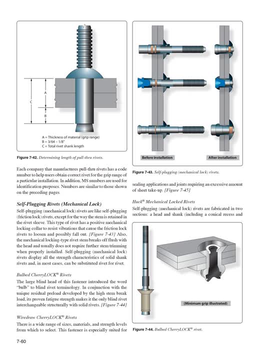 Self-plugging rivets- mechanical lock. self-plugging mechanical lock Rivets are like self-plugging friction lock rivets, except for the way the shank is pulled. The shank's shank stem is retained in the rivet sleeve. 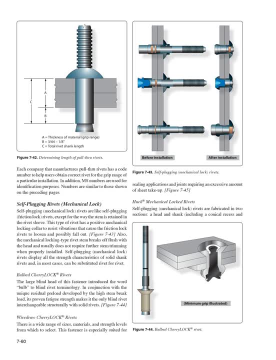 This type of rivet has a positive mechanical locking collar to resist vibrations that cause the friction lock rivets to loosen and possibly fall out- Figure 743. Also, the mechanical locking type rivet stem breaks off flush with the head and usually does not require further stem trimming when properly installed. 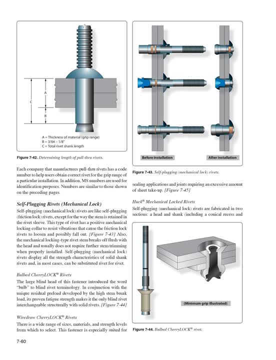 Self-plugging mechanical lock rivets display all the strength characteristics of solid shank rivets and in most cases can be substituted rivet for rivet. Bulb cherry lock rivets. The large blind head of this fastener introduced the word bulb to blind rivet terminology. 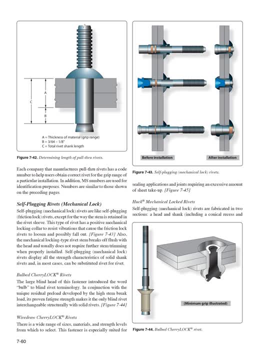 In conjunction with the unique residual preload developed by the high stem brake load, its proven fatigue strength makes it the only blind rivet interchangeable structurally with solid rivets. Figure 744: Wire draw- cherry lock rivets. There is a wide range of sizes, materials and strength levels from which to select. 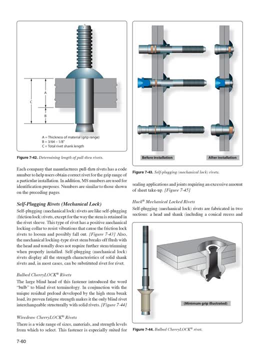 This fastener is especially suited for sealing applications and joints requiring an excessive amount of force. This fastener is especially suited for sealing applications and joints requiring an excessive amount of force. This fastener is especially suited for sealing applications and joints requiring an excessive amount of force. 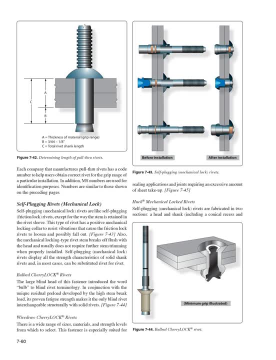 of sheet take-up. Figure 745, Huck Mechanical Locked Rivet. Self-Plugging Mechanical Lock rivets are fabricated in two sections: a head and shank, including a conical recess end locking collar in the head and a serrated stem that extends through the shank. 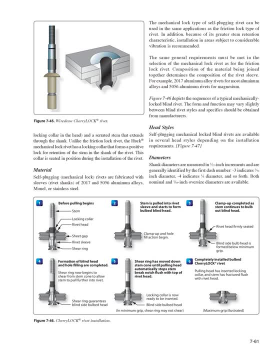 Unlike the friction lock rivet, the Huck Mechanical Lock rivet has a locking collar that forms a positive lock for retention of the stem in the shank of the rivet. This collar is seated in position during the installation of the rivet Material. Self-Plugging Mechanical Lock rivets are fabricated with sleeves. 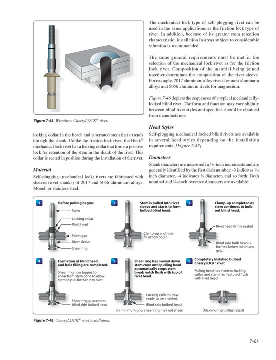 rivet shanks of 2017 and 5056, aluminum alloys, monol or stainless steel. The mechanical lock type of self-plugging rivet can be used in the same applications as the friction lock type of rivet. In addition, because of its greater stem, 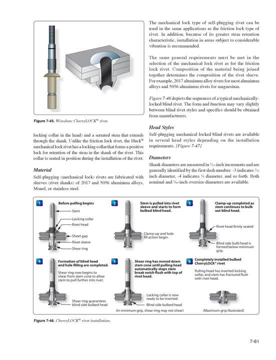 retention, characteristic installation in areas subject to considerable vibration is recommended. The same general requirements must be met in the selection of the mechanical lock rivet As for the friction lock rivet. Composition of the material being joined together determines the composition of the rivet sleeve. For example, 2017 aluminum alloy rivets for most aluminum alloys. 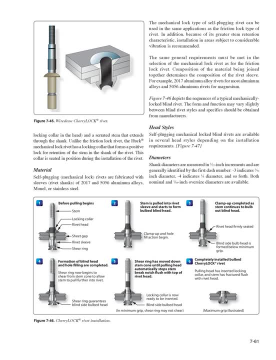 and 5056 aluminum rivets for magnesium. Figure 746 depicts the sequences of a typical mechanically locked blind rivet. The form and function may vary slightly between blind rivet styles and specifics should be obtained from manufacturers. Head styles: self-plugging, mechanical locked blind. 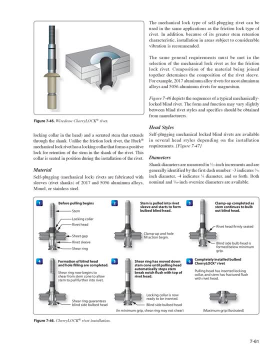 rivets are available in several head styles depending on the installation requirements: Figure 747.. Diameter: shank diameters are measured in 1- 32nd inch increments and are generally identified by the first dash number. Minus 3 indicates 3 32nd inch diameter. minus 4 indicates 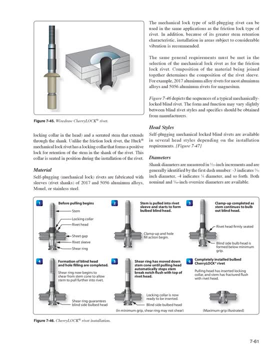 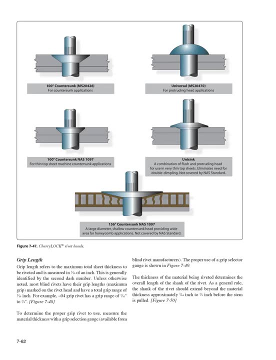 1- 8th diameter and so forth. Both nominal and 1- 64th inch oversize diameters are available. Grip length: Grip length refers to the maximum total sheet thickness to be riveted and is measured in 1- 16th of an inch. 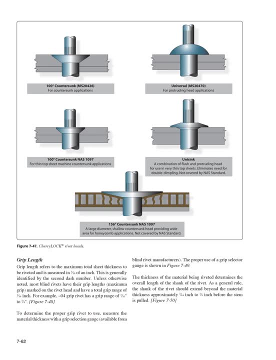 This is generally identified by the second dash number. Unless otherwise noted, most blind rivets have their grip lengths, maximum grip, marked on the rivet head and have a total grip range of 1 16th inch. For example, 04 grip rivet has a grip range of 3 16ths of an inch to 1 quarter of an inch. 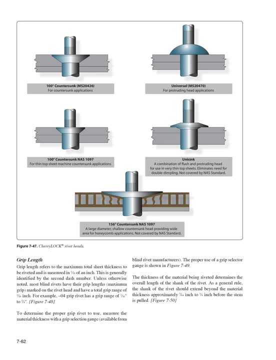 Figure 748.. To determine the proper grip rivet to use, measure the material thickness with a selection gauge available from blind rivet manufacturers. The proper use of a grip selector is known in Figure 749.. The thickness of the material being riveted determines the overall. 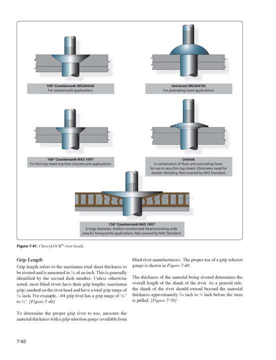 length of the shank of the rivet. As a general rule, the shank of the rivet should extend beyond the material thickness, approximately 3 64ths inch to 1, 8th inch before the stem is pulled. Figure 750.. Rivet identification. Each company that manufactures self-plugging. 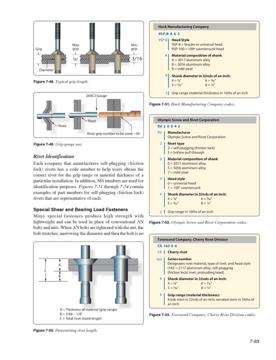 friction lock rivets has a code number to help users obtain the correct rivet for the grip range or material thickness of a particular installation. In addition, mess numbers are used for identification purposes. Figures 7-51 through 7-54 contain examples of 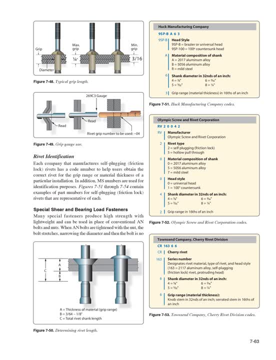 part numbers for self-plugging friction lock rivets that are representative of each Special shear and bearing load fasteners. Many special fasteners produce high strength with lightweight and can be used in place of conventional in bolts and nuts. When in bolts are tightened with the nut, the bolt stretches, narrowing the diameter, and then 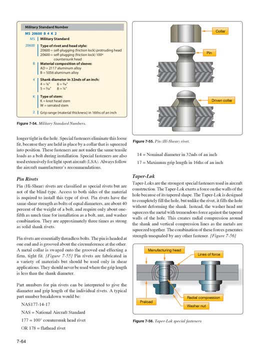 the bolt is no longer tight in the hole. Special fasteners. Special fasteners are used extensively for light sport aircraft LSA. Always follow the aircraft manufacturer's recommendations. Pin rivets- pin high shear rivets- are classified as special rivets but are not of the blind type. Access to both sides of the material is required to 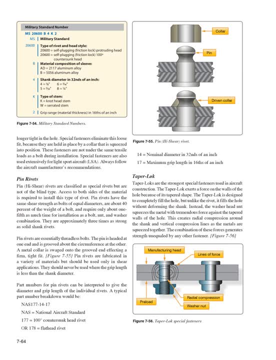 install this type of rivet. Pin rivets have the same shear strength but are not of the blind type. Pin rivets have the same shear strength as bolts of equal diameters, are about 40% of the weight of a bolt and require only about one-fifth as much time for installation as a bolt nut and washer. 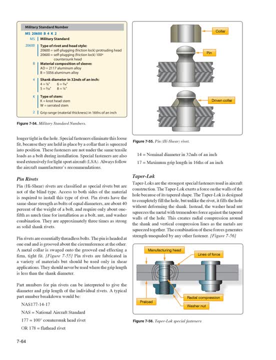 combination, They are approximately three times as strong as solid shank rivets. Pin rivets are essentially threadless bolts. The pin is headed at one end and is grooved about the circumference at the other. A metal collar is swashed onto the grooved end, affecting a firm, tight fit. 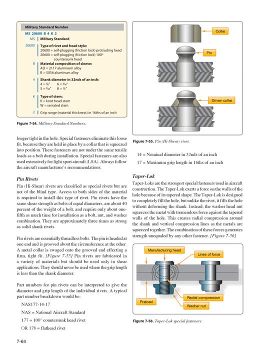 Figure 7-55. Pin rivets are fabricated in a variety of materials but be used only in shear applications. They should never be used where the grip length is less than the shank diameter. Part numbers for pin rivets can be interpreted to give the diameter and grip. 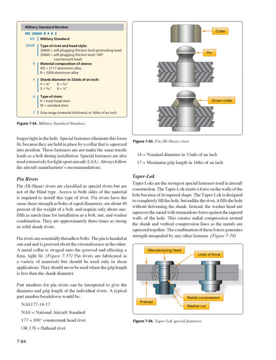 length of the individual rivets. A typical part number breakdown would be NAZ, 177-14-17. NAZ equals National Aircraft Standard. 177 equals 100 degrees countersunk head rivet, OR 178 equals flat head rivet. 14 equals nominal diameter in 30 seconds of an inch. 17 equals maximum grip length. 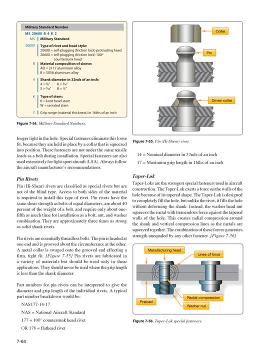 in sixteenths of an inch taper lock. Taper locks are the strongest special fasteners used in aircraft construction. The taper lock exerts a force on the walls of the hole because of its tapered shape. The taper lock is designed to completely fill the hole but, unlike the rivet, 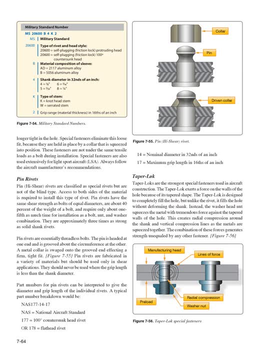 it fills the hole without deforming the shank. Instead, the washer head nut squeezes the metal with tremendous force against the tapered walls of the hole. This creates radial compression around the shank and vertical compression lines as the metals are squeezed together. The combination of 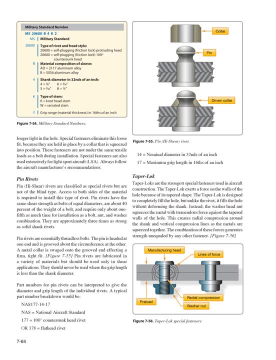 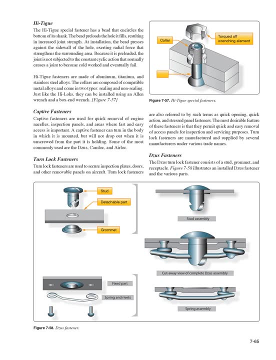 forces, generates strength unequaled by any other fastener. Figure 756: Hi-Tig. The Hi-Tig special fastener has a bead that encircles the bottom of its shank. The bead preloads the hole it fills, resulting in increased joint strength At installation. the bead presses against the sidewall of the hole, exerting radial. 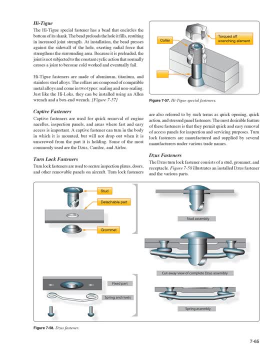 force that strengthens the surrounding area. Because it is preloaded, the joint is not subjected to the constant cyclic action that normally causes a joint to become cold worked and eventually fail. Hi-Tig fasteners are made of aluminum, titanium and stainless steel alloys. 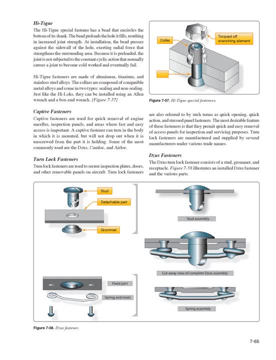 The collars are composed of compatible metal alloys and come in two types: sealing and non-sealing. Just like the Hi-Locks, they can be installed using an Allen wrench and a box end wrench. Figure 757: Captive Fasteners. Captive fasteners are used for quick removal of engine nacelles. 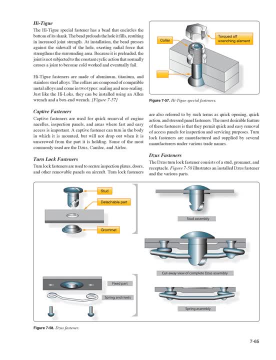 inspection panels and areas where fast and easy access is important. A captive fastener can turn in the body in which it is mounted, but will not drop out when it is unscrewed from the part it is holding. Some of the most commonly used are the shouted TZIS. 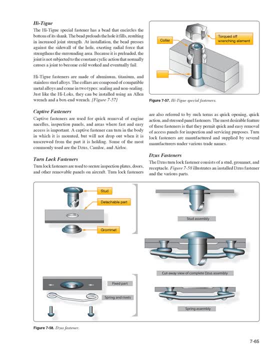 Clamp tensioner and airlock fasteners. Turn Lock Fasteners. Turn lock fasteners are used to secure inspection plates, doors and other removable panels on aircraft. Turn-Lock fasteners are also referred to by such terms as quick-opening- quick action. 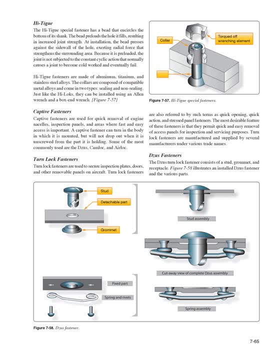 and stress panel fasteners. The most desirable feature of these fasteners is that they permit quick and easy removal of access panels for inspection and servicing purposes. Turn-Lock Fasteners. Turn-Lock fasteners are manufactured at and supplied by several manufacturers under various trade names: ZIS fasteners, The ZIS. 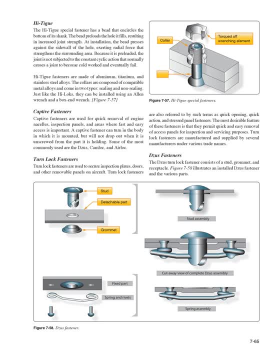 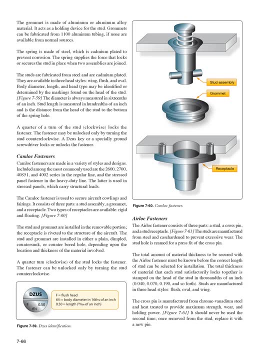 turnlock fastener consists of a stud grommet and receptacle. Figure 758 illustrates an installed ZIS fastener. in the various parts, The grommet is made of aluminum or aluminum alloy material. It acts as a holding device for the stud. Grommets can be fabricated from 1100 aluminum tubing. 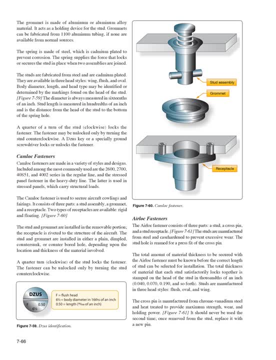 if none are available from normal sources. The spring is made of steel, which is cadmium plated to prevent corrosion. The spring supplies the force that locks or secures the stud in place when two assemblies are joined. The studs are fabricated from steel and are cadmium plated. 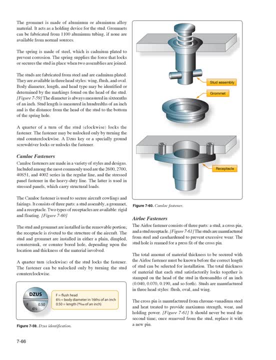 They are available in three head styles: wing, flush and oval. Body diameter, length and head type may be identified or determined by the markings found on the head of the stud, Figure 759,. the diameter is always measured in sixteenths of an inch. Stud. length is measured in hundredths. 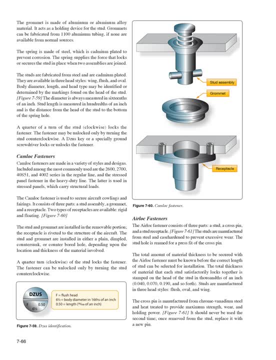 of an inch and it is the distance from the head of the stud to the head of the stud. A quarter of a turn of the stud. clockwise locks the fastener. The fastener may be unlocked only by turning the stud counterclockwise. A ZIS key or a specially ground screwdriver locks or unlocks. 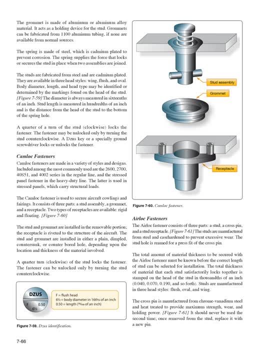 the fastener: Camlocked fasteners. Camlocked fasteners are made in a variety of styles and designs. Included among the most commonly used are the 2600,, 2700, 40S51, and 4002 series in the regular line and the stressed panel fastener in the regular line. Camlocked fasteners are made 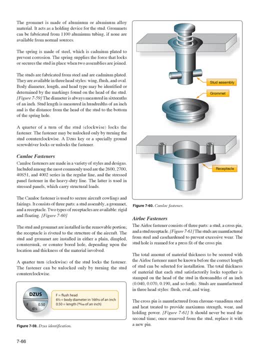 in the heavy-duty line. The latter is used in stressed panels which carry structural loads. The camlocked fastener is used to secure aircraft cowlings and fairings. It consists of three parts: a stud assembly, a grommet and a receptacle. Two types of receptacles are available. 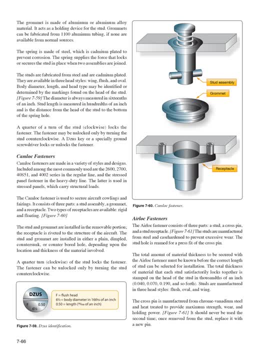 rigid and floating. Figure 760,. the stud and grommet are installed in the removable portion. The receptacle is riveted to the structure of the aircraft. The stud and grommet are installed in either a plain dimpled counter-steering or a flat-bedded aircraft. The stud and grommet are 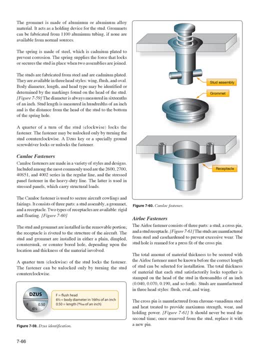 sunk or counter-bored hole, depending upon the location and thickness of the material involved. A quarter turn clockwise of the stud locks the fastener. The fastener can be unlocked only by turning the stud counterclockwise. Airlocked fasteners. The airlocked fastener consists of: 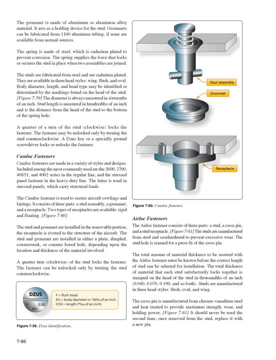 three parts: a stud, a cross pin and a stud receptacle- Figure 761,. the studs are manufactured from steel and case-hardened to prevent excessive wear. The stud hole is reamed for a press fit of the cross pin. Figure 761,. the studs are manufactured from steel and case-hardened to prevent excessive wear. The stud hole is reamed for a press fit of the cross pin. 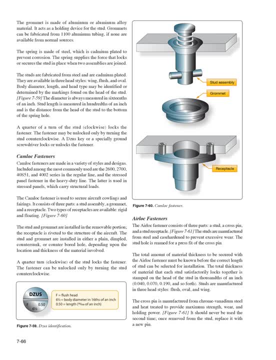 The total amount of material thickness to be secured with the airlocked fastener must be known before the correct length of stud can be selected for installation. The total thickness of material that each stud satisfactorily locks together is stamped on the head of the stud in. 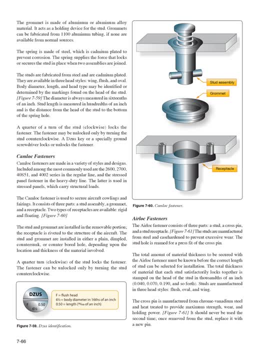 thousandths of an inch: 0.040,, 0.070,, 0.190, and so forth. Studs are manufactured in three head styles: flush, oval and wing. The cross pin is manufactured from chrome, vanadium steel and heat-treated to provide. 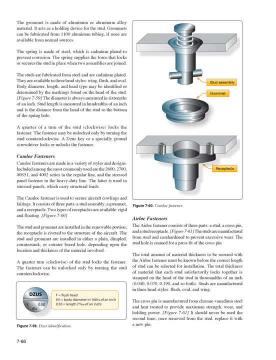 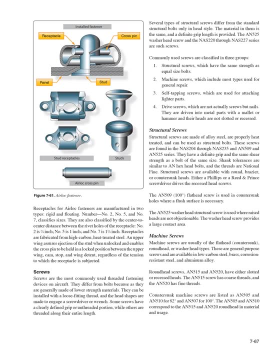 maximum strength, wear and holding power: Figure 761,. it should never be used the second time. Once removed from the stud, replace it with a new pin. Receptacles for airlocked fasteners are manufactured in two types: rigid and floating. Number no Two, no Five and no Seven classifies. 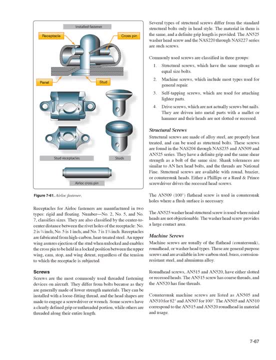 sizes. They are also classified by the center-to-center distance between the rivet holes of the receptacle. No Two is three-quarters inch, No Five is one inch and no Seven is thirteen-eighths inch. Receptacles are fabricated. 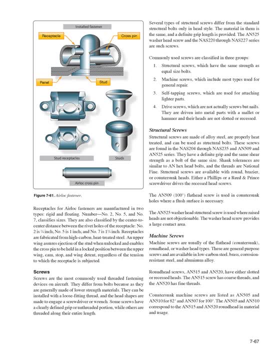 from high-carbon, heat-treated steel. An upper wing assures ejection of the stud when unlocked and enables the cross pin to be held in a locked position between the upper wing, cam stop and wing detent, regardless of the tension to which the receptacle is subjected. Screw screws are the 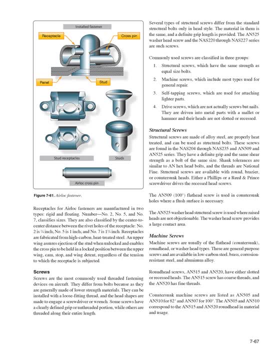 most commonly used threaded fastening devices on aircraft. They differ from bolts because, as they are generally made of lower-strength material, They can be installed with a loose-fitting thread and the head shapes are made to engage a screwdriver or wrench. Some screws have a clearly defined grip or unthreaded portion, while others are threaded. 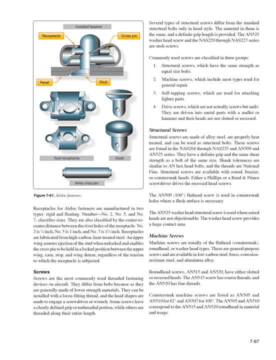 along their entire length. Several types of structural screws differ from the standard structural bolts only in head style. The material in them is the same and a definite grip length is provided. The AN525 washer head screw in the NAS220 through NAS227 series are such screws. 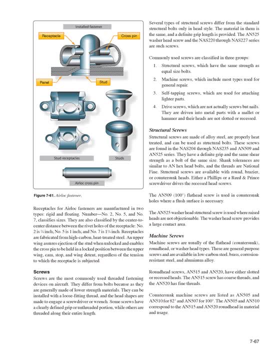 Commonly used in the NAS220 series are the AN525 washer head screw and the AN525 washer head screw. Commonly used in the NAS220 series are the AN525 washer head screw and the AN525 washer head screw. Commonly used screws are classified in three groups. One: Structural screws, which have the 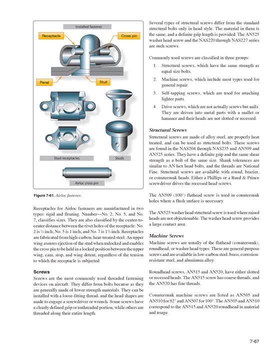 same strength as equal-size bolts. Two Machine screws, which include most types used for general repair. Three Self-tapping screws, which are used for attaching lighter parts. Four Drive screws, which are not actually screws but nails. They are driven into metal parts with a mallet or 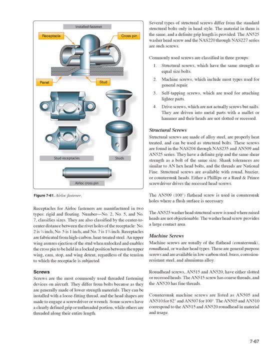 hammer and their heads are not slotted or recessed. Structural screws. Structural screws are made of alloy steel, are properly heat-treated and can be used as structural bolts. These screws are found in the NAS204 through NAS235, and AN509 and AN525 series. 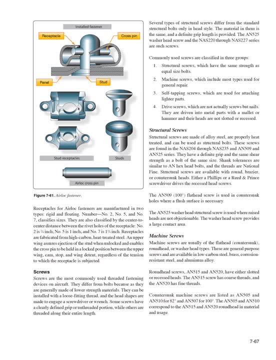 They have a definite grip and the same shear strength as a bolt of the same size. Shank tolerances are similar to an hex head bolts and the threads are national fine Structural screws are available with round, brazier or countersunk heads. 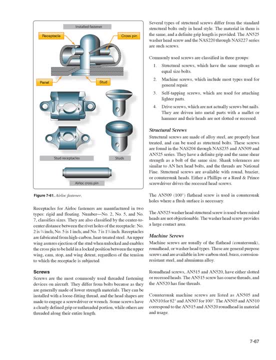 Either a Phillips or a Reed and Prince screwdriver drives the recessed head screws. The AN509, 100 degrees flathead screw is used in countersunk holes where a flush surface is necessary. The AN525 washer head structural screw is used where raised. 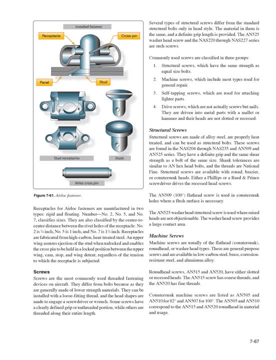 heads are not objectionable. The washer head screw provides a large contact area. Machine screws. Machine screws are usually of the flathead, countersunk, roundhead or washer head types. These are general-purpose screws and are available in low-carbon steel. 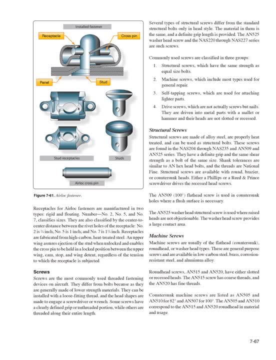 brass, corrosion-resistant and stainless steel and aluminum alloy Roundhead screws- AN515 and AN520, have either slotted or recessed heads. The AN515 screw has coarse threads and the AN520 has fine threads. Countersunk machine screws are listed as AN505 and AN510 for 82 degrees and AN507 for 100 degrees. 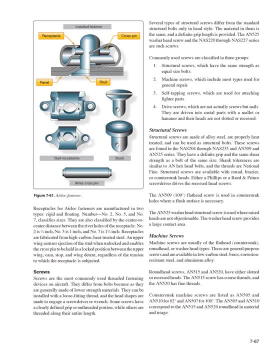 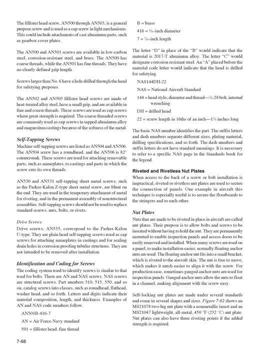 The AN505 and AN510 correspond to the AN515 and AN520 roundhead screws. The AN500 and AN501 screws are available in low-carbon steel, corrosion-resistant steel and brass. The AN500 has coarse threads, while the AN501 has fine threads. They have no, clearly. 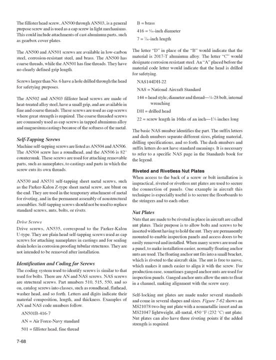 defined grip length. The AN500 and AN501 have coarse threads, while the AN501 has fine threads. The AN500 and AN502 have coarse threads, while the AN501 has fine threads. The AN500 and AN501 have no clearly defined grip length. Screws larger than No 6 have a hole drilled through the head for. 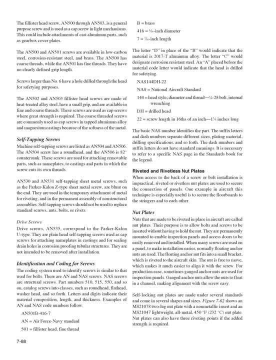 safety and purposes. The AN502 and AN503 filister head screws are made of heat-treated alloy steel, have a small grip and are available in fine and coarse threads. These screws are used as cap screws where great strength is required. The coarse-threaded screws are commonly used as 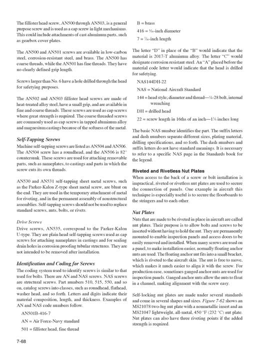 cap screws in tapped aluminum, alloy and magnesium castings because of the softness of the metal. Self-tapping screws- Machine self-tapping screws are listed as AN504 and AN506.. The AN504 screw has a round head and the AN506 is 82°. 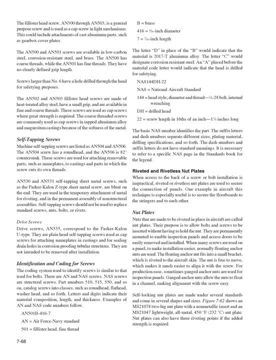 countersunk. These screws are used for attaching removable parts, such as nameplates, to castings and parts in which the screw cuts its own threads. AN530 and AN531 self-tapping sheet metal screws, such as the Parker Kalon Z-type sheet metal screw, are blunt on the end. They are used in the. 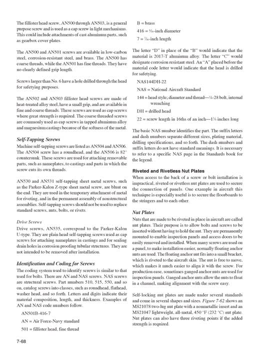 temporary attachment of metal for riveting. The AN530 and AN531 self-tapping sheet metal screws are used for riveting and in the permanent assembly of non-structural assemblies. Self-tapping screws should not be used to replace standard screws, nuts bolts or rivets. 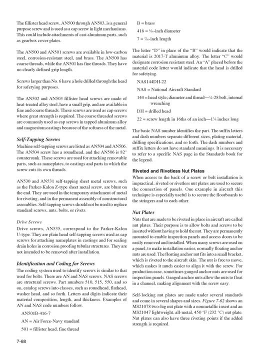 Drive screws. Drive screws AN535, correspond to the Parker Kalon Z-type. They are plain-head self-tapping screws used as cap screws for attaching nameplates in castings and for sealing drain holes in corrosion-proofing tubular structures. They are not intended to be. 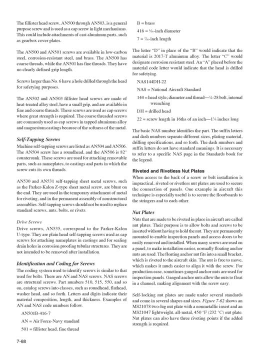 removed after installation. Identification and Coating for Screws. The coating system used to identify screws is similar to that used for bolts. There are ANT and NAS screws. NAS screws are structural screws, Part numbers 510,, 515,, 550, and so on. catalog screws into classes such as round head. 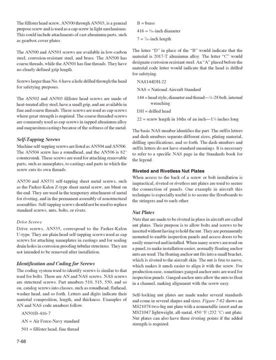 flat head, washer, head and so forth. Letters and digits indicate their material composition, length and thickness. Examples of ANT and NAS code numbers follow: AN501B4167AN-Air Force Navy Standard. 501-Philister Head Fine Thread- B-Brass- 416-416-Inch Diameter, 7-716-Inch. 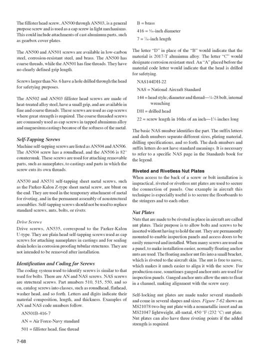 Length. The letter D in place of the B would indicate that the material is 2017T Aluminum Alloy. The letter C would designate corrosion-resistant steel. An A placed before the material code letter would indicate that the head is drilled for safety. NAS 144, DH 22. NAS equals National Aircraft Standard. 144 equals head style, diameter and thread. 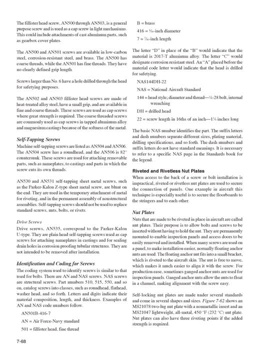 1 quarter minus 28 bolt internal wrenching. DH equals drilled head, 22 equals screw length in 16ths of an inch, 13, 8ths inches long. the basic NAS number identifies the part. The suffix letters and dash numbers separate different sizes. plating material, drilling. 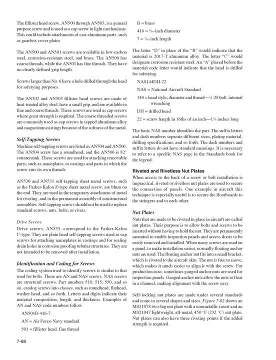 specifications and so forth. The dash numbers and suffix letters do not have standard meanings. It is necessary to refer to a specific NAS page in the standards book for the legend Riveted and rivetless nut plates. when access to the back of a screw or bolt installation is. 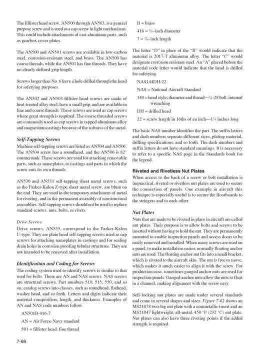 impractical riveted or rivetless nut plates are used to secure the connection of panels. One example: in aircraft, this technique is especially useful is to secure the floorboards to the stringers and to each other. Nut plates- nuts that are made to be riveted in place in 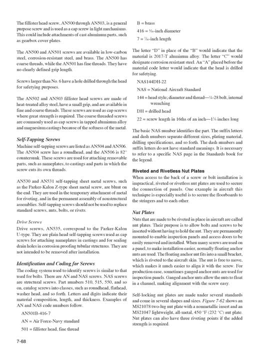 aircraft are called nut plates. Their purpose is to allow bolts and screws to be inserted without having to hold them. They are permanently mounted to enable inspection panels and access doors to be easily removed and installed. When many screws are used on a panel to make installation easier, 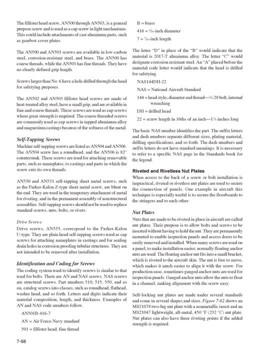 normally floating anchor nuts are used. The floating anchor nut fits into a small bracket which is riveted to the aircraft skin. The nut is free to move, which makes it much easier to align it with the screw. For production ease, sometimes ganged anchor nuts are used for 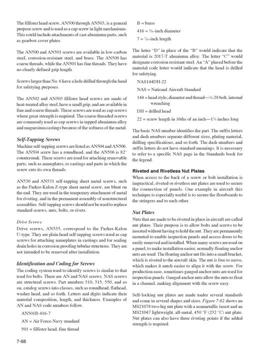 inspection panels. Ganged anchor nuts allow the nuts to float in a channel, making alignment with the screw easy. Self-locking nut plates are made under several standards and come in several shapes and sizes. Figure 762 shows an MS-21078-2 lug nut plate with a non-metallic 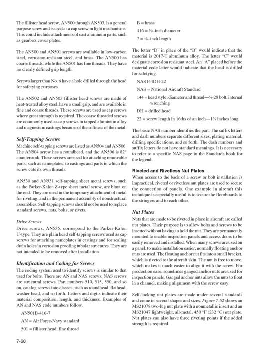 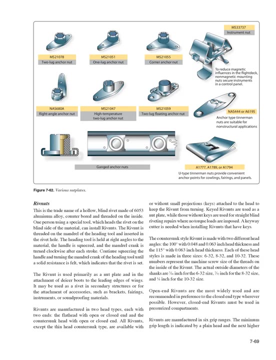 insert and an MS-21047 lightweight all-metal, 450°F, 232°C nut plate. Nut plates can also have three riveting points if the added strength is required. Rivenuts- this is the trade name of a hollow blind rivet made of 6,000mm. Rivenuts- this is the trade name of a hollow blind rivet made of 6,000mm. 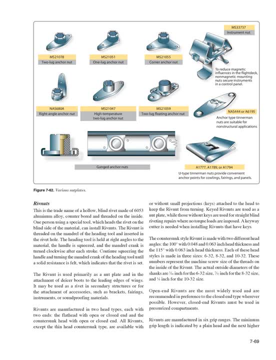 Rivenuts. this is the trade name of a hollow blind rivet made of 6,000mm. One-person using a special tool which heads the rivet on the blind side of the material can install rivenuts. The rivenut is threaded on the mandrel of the heading tool and inserted. 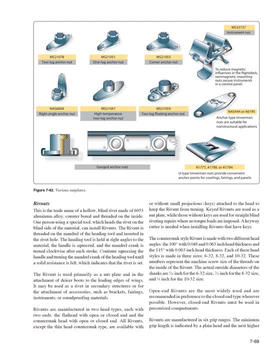 in the rivet hole. The heading tool is held at right angles to the material, the handle is squeezed and the mandrel crank is turned clockwise after each stroke. Continue squeezing the handle and turning the mandrel crank of the heading tool until a solid resistance is felt. 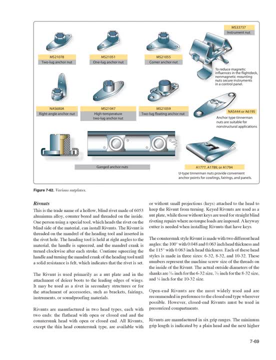 which indicates that the rivet is set. The rivnut is used primarily as a nut plate and in the attachment of de-icer boots to the leading edges of wings. It may be used as a rivet in secondary structures or for the attachment of. 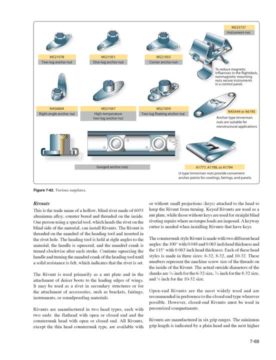 accessories such as brackets, fairings, instruments or soundproofing materials. Rivnuts are manufactured in two head types, each with two ends: the flathead with open or closed end, and the countersunk head with open or closed end. All rivnuts, except the thin head countersunk. 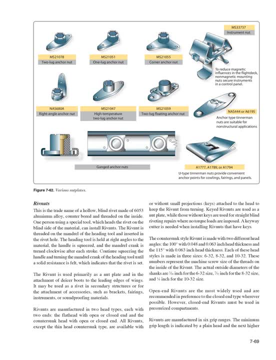 type are available with or without small projections keys attached to the head to keep the rivnut from turning. Keyed rivnuts are used as a nut plate, while those without keys are used for straight, blind riveting repairs where no torque loads are imposed. A keyway cutter is 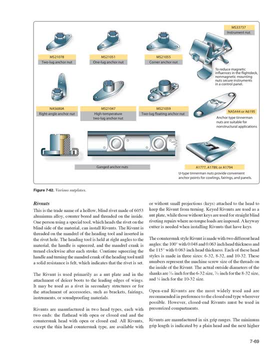 needed when installing rivnuts that have keys. The countersunk style rivnut is made with two different head angles: the 100 degrees with 0.048 and 0.063 inch head thickness, and the 115 degrees with 0.063 inch head thickness. 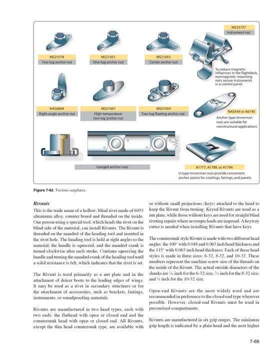 Each of these head styles is made in three sizes: 6-32,, 8-32, and 10-32.. These numbers represent the machine screw size of the threads on the inside of the rivnut. The actual outside diameters of the shanks are 3-16 inch for the 6-32 size, 7-32 inch for the 8-32 size. 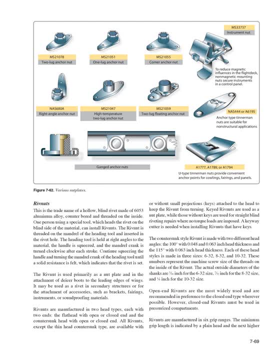 and 1-1⁄4 inch for the 10-32 size. Open end rivnuts are the most widely used and are recommended in preference to the closed end type wherever possible. However, closed end rivnuts must be used in pressurized compartments. 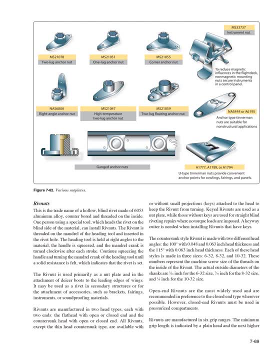 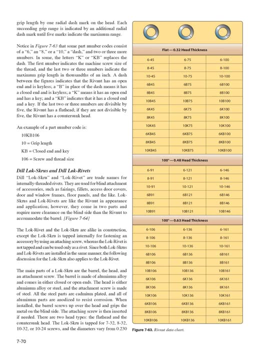 Rivnuts are manufactured in six grip ranges. The minimum grip length is indicated by a plain head and the next higher grip length by one radial dash mark on the head. Each succeeding grip range is indicated by an additional radial dash mark until five marks indicate the maximum. 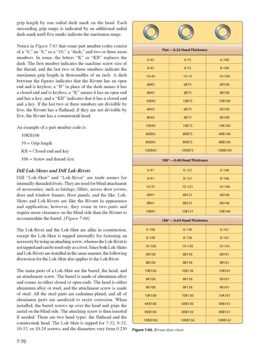 range. Notice in figure 763 that some part number codes consist of a 6, an 8, or a 10,, a dash and two or three more numbers In sum. the letters K or KB replaces the dash. The first number indicates the machine screw size. 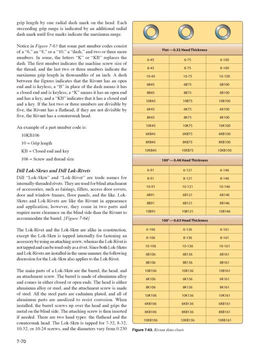 of the thread and the last two or three numbers indicate the maximum grip length in thousandths of an inch. A dash between the figures indicates that the rivnut has an open end and is keyless. a B in place of the dash means it has a closed end and is keyless. a K means it has an open. 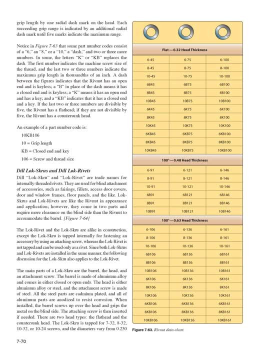 end and has a key, and a KB indicates that it has a closed end and a key. If the last two or three numbers are divisible by five, the rivnut has a flat head. if they are not divisible by five, the rivnut has a countersunk head. 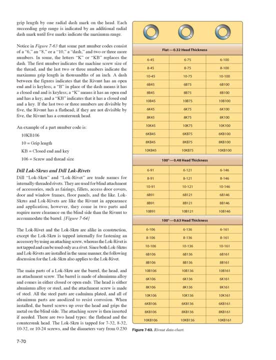 An example of a part number code is 10KB10610 equals grip length, KB equals closed end and key 106 equals screw and thread size. Dill lock scris and Dill lock rivets, Dill lock screw and lock rivet are trade names for internally threaded rivets. They are used for blind attachment of 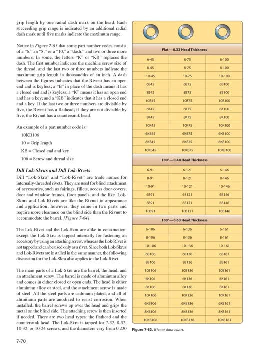 accessories such as fairings, fillets, access door covers, door and window frames, floor panels and the like. Lock scris and lock rivets are like the rivnut in appearance and application. however, they come in two parts and require more. 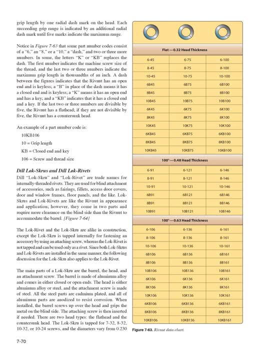 clearance on the blind side than the rivnut to accommodate the barrel. Figure 764,. the lock rivet and the lock screw are alike in construction, except the lock screw is tapped internally for fastening an accessory by using an attaching screw, whereas the lock rivet is not tapped. 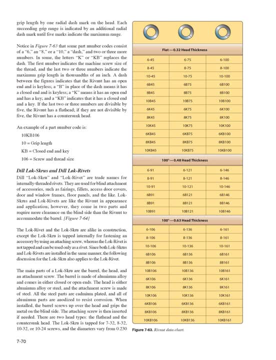 and can be used only as a rivet. Since both lock scris and lock rivets are installed in the same manner, the following discussion for the lock screw also applies to the lock rivet. The main components of a lock screw are the barrel, the head and an attachment screw. The barrel is made. 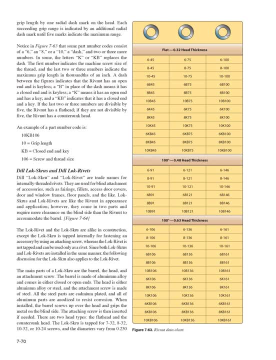 of aluminum alloy and comes in either closed or open ends. The head is either aluminum alloy or steel and the attachment screw is made of steel. All the steel parts are cadmium plated and all of aluminum parts are anodized to resist corrosion. When installed, the barrel screws up over the head. 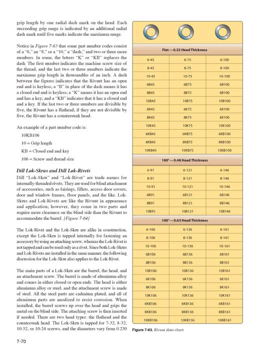 and grips the metal on the blind side. The attaching screw is then inserted if needed. There are two head types: the flathead and the countertop. The lock screw is tapped for 7-32,, 8-32,, 10-32, or 10-24 screws, and the diameters vary from 0.230. 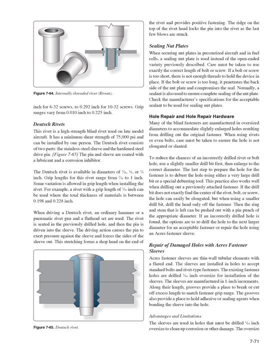 inch for 6-32 screws to 0.292 inch for 10-32 screws. Grip ranges vary from 0.010 inch to 0.225 inch. Deutsch Rivets. This rivet is a high-strength blind rivet used on late model aircraft. 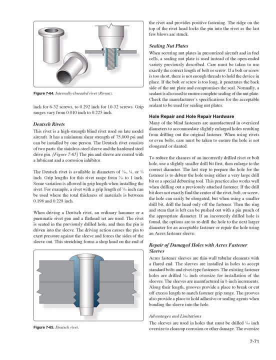 It has a minimum shear strength of 75,000 pounds per square inch and can be installed by one person. The Deutsch Rivet consists of two parts: the stainless steel sleeve and the hardened steel drive pin, Figure 765,. the pin and sleeve are: 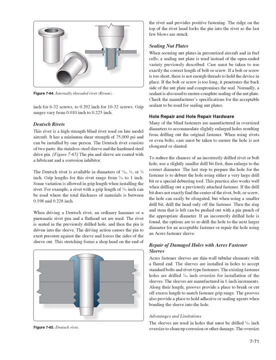 coated with a lubricant and a corrosion inhibitor. The Deutsch Rivet is available in diameters of 3 sixteenths, one quarter or three-eighths inch. Grip lengths for this rivet range from 3 sixteenths. 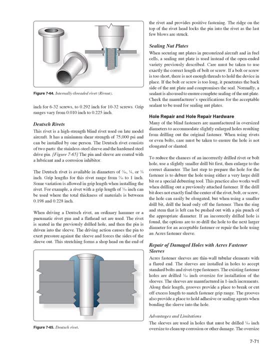 to one inch. Some variation is allowed in grip length when installing the rivet. For example, grip length of 3 sixteenths inch can be used where the total thickness of materials is between 0.198 and 0.228 inch. When driving a Deutsch Rivet, an ordinary hammer or a pneumatic rivet gun and a 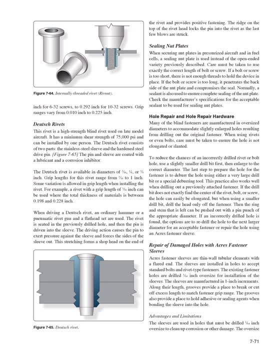 flathead set are used. The rivet is seated in the previously drilled hole and then the pin is driven into the sleeve. The driving action causes the pin to exert pressure against the sleeve and forces the sides of the sleeve out. This stretching forms a shop head on the end of the rivet and 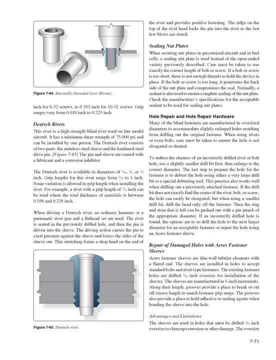 provides positive fastening Grip. length of 3 sixteenths inch can be used where the total thickness on the top of the rivet head locks the pin into the rivet as the last few blows are struck. Sealing nut plates When securing nut plates in pressurized aircraft and in fuel cells. 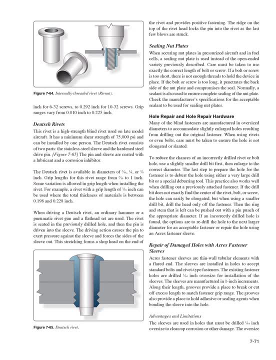 a sealing nut plate is used instead of the open-ended variety previously described, Care must be taken to use exactly the correct length of bolt or screw. If a bolt or screw is too short, there is not enough threads to hold the device in place. 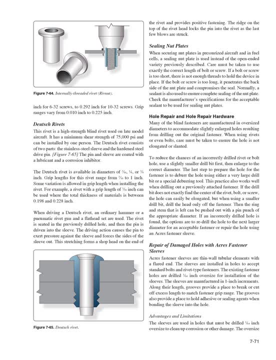 If the bolt or screw is too long, it penetrates the back side of the nut plate and compromises the seal. Normally, a sealant is also used to ensure complete sealing of the nut plate. Check the manufacturer's specifications for the acceptable sealant to be used for sealing nut. 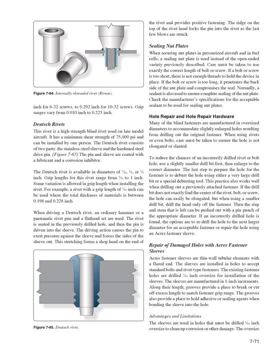 plates, Hole repair and hole repair hardware. Many of the blind fasteners are manufactured in oversized diameters to accommodate slightly enlarged holes resulting from drilling out the original fastener. When using rivets or even bolts, care must be taken to ensure the hole is not elongated or slanted, To reduce the chances. 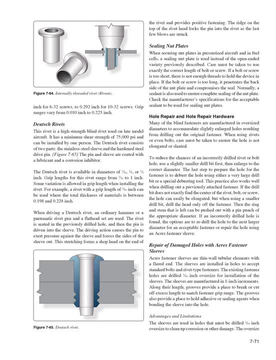 of an incorrectly drilled rivet or bolt. you must use a hole repair hardware To drill a bolt hole. use a slightly smaller drill bit first, then enlarge to the correct diameter. The last step to prepare the hole for the fastener is to deburr the hole using either: 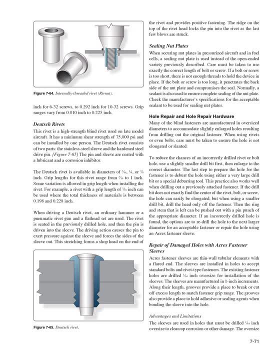 a very large drill bit or a special deburring tool. This practice also works well when drilling out a previously attached fastener. If the drill bit does not exactly find the center of the rivet bolt or screw, the hole can easily be elongated. but when using a smaller drill bit, 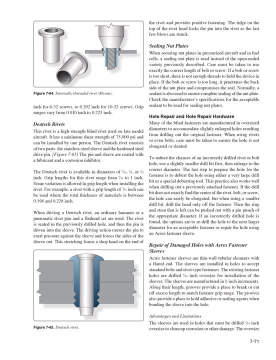 drill the head only off the fastener. Then the ring and stem that is left can be pushed out of the appropriate diameter. If an incorrectly drilled hole is found, the options are to re-drill the hole to the next larger diameter for an acceptable fastener or repair the hole. 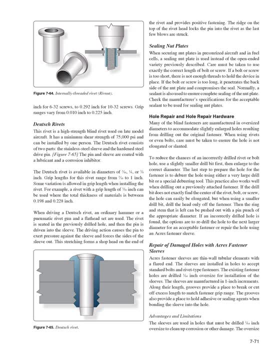 using an Aker's fastener sleeve: Repair of damaged holes with Aker's fastener sleeves. Aker's fastener sleeves are thin wall tubular elements with a flared end. The sleeves are installed in holes to accept standard bolts and rivet-type fasteners. The existing fastener. 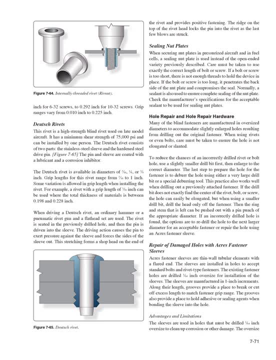 holes are drilled- 1 64th inch oversize for installation of the sleeves. The sleeves are in one-inch increments Along their length. grooves provide a place to break or cut off excess length to match fastener grip range. The grooves also provide a place to hold adhesive. 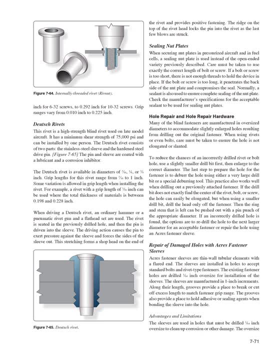 or sealing agents when bonding the sleeve into the hole. Advantages and limitations. The sleeves are used in holes that must be drilled 1 64th inch oversize to clean up corrosion or other damage. The oversize hole with the sleeve installed allows the use of the original diameter. 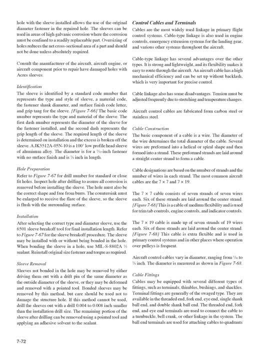 fastener in the repaired hole. The sleeves can be used in areas of high ground and high galvanic corrosion, where the corrosion must be confined to a readily replaceable part. Oversizing of holes reduces the net cross-sectional area of a part and should not be done unless. 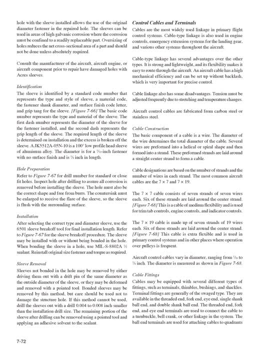 absolutely required. Consult the manufacturer of the aircraft. aircraft engine or aircraft component prior to repair. have damaged holes with Aker's sleeves. Identification: The sleeve is identified by a standard code number that represents the type and style of sleeve, a material code, the fastener, shank diameter and surface finish code letter. 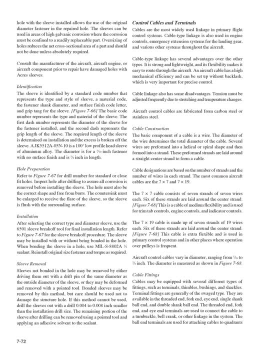 for the sleeve, Figure 766,. the basic code number represents the type and material of the sleeve. The first dash number represents the diameter of the sleeve for the fastener installed and the second dash represents the grip length of the sleeve, The required length of the sleeve. 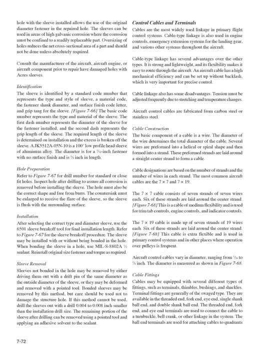 is determined on installation and the excess is broken off the sleeve. A JK 5512A05N10 is a 100 degrees low profile head sleeve of aluminum alloy. The diameter is for a 5, 32nd inch fastener with no surface finish and is 5 eighths inch in length. Hole preparation: refer to figure 767 for drill. 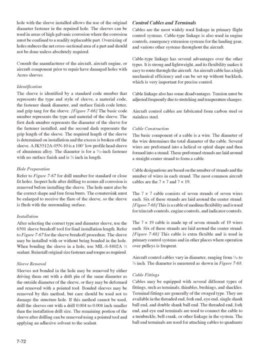 number for standard or close fit holes. Inspect hole after drilling to assure all corrosion is removed before installing the sleeve. The hole must also be the correct shape and free from burrs. The counter sink must be enlarged to receive the flare of the sleeve So the sleeve is flush with. 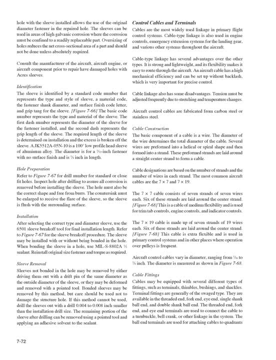 the surrounding surface Installation. After selecting the correct type and diameter sleeve, use the 6502.. Sleeve breakel: for final installation length: Refer to figure 767 for the sleeve break off procedure. The sleeve may be installed with or without being bonded in the hole. When bonding the sleeve in a hole, 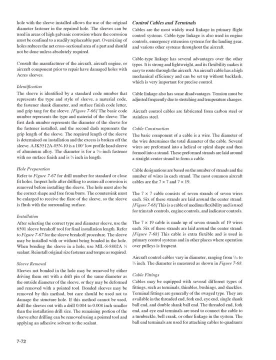 use mill S8802A half sealant. Reinstall original size, fastener and torque as required. Sleeve removal: sleeves not bonded in the hole may be removed by either driving them out with a drift pin of the same diameter as the outside diameter of the sleeve, or they may be deformed. 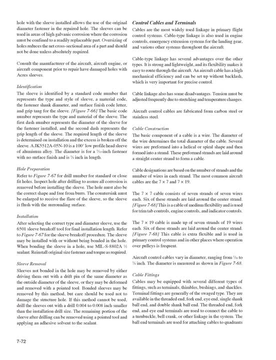 and removed with a pointed tool. Bonded sleeves may be removed by this method, but care should be used not to damage the structure hole. If this method cannot be used, drill the sleeves out with a drill 0.004 to 0.008 inch smaller than the installation drill size. The remaining portion: 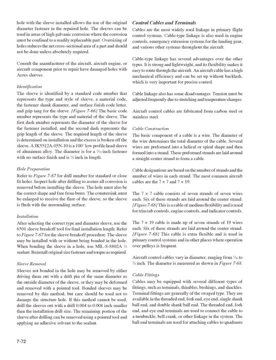 of the sleeve after drilling can be removed using a pointed tool and applying an adhesive solvent to the sealant. Control cables and terminals. cables are the most widely used linkage in primary flight control systems. Cable type linkage is also used in engine controls, emergency extension systems for the 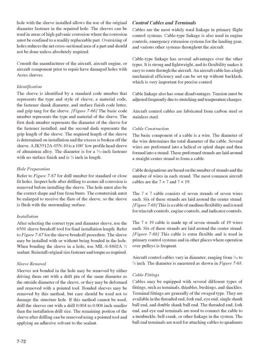 landing gear and various other systems throughout the aircraft. Cable type linkage has several advantages over the other types. It is strong and lightweight and its flexibility makes it easy to route through the aircraft. An aircraft cable has a high mechanical efficiency and can be set up without backlash, which is very important for precise control. Cable linkage. 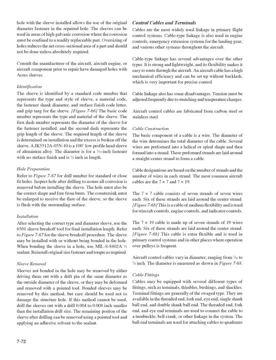 also has some disadvantages. Tension must be adjusted frequently due to stretching in the aircraft. Cable type linkage is also used in engine controls, emergency extension systems and temperature changes. Aircraft control cables are fabricated from carbon steel or stainless steel Cable construction. The basic component of a cable is a wire. 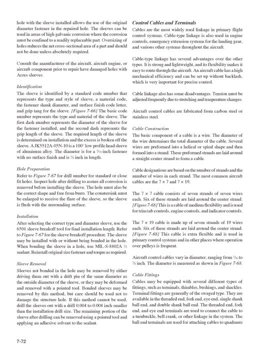 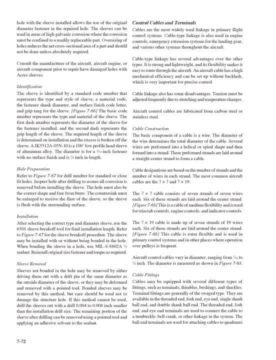 strand- Figure 768,. this is a cable of medium flexibility and is used for trim tab controls, engine controls and indicator controls. The 7x19 cable is made up of seven strands of 19 wires each. Six of these strands are laid around the center strand- Figure 7-68,. this cable is extra. 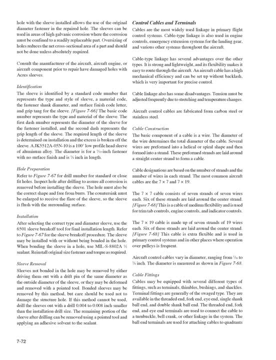 flexible and is used in primary control systems and in other places where operation over pulleys is frequent. Aircraft control cables vary in diameter, ranging from 1 16th to 3 8ths inch. The diameter is measured as shown in figure 768.. Cable fittings. cables may be equipped with several 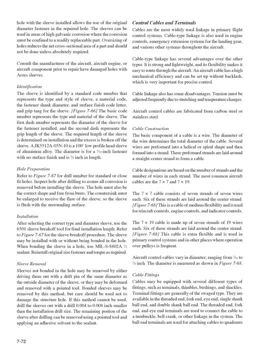 different types of fittings, such as terminals, thimbles, bushings and shackles. Terminal fittings are generally of the swash type. They are available in the threaded end, fork end, I-end, single shank ball end And double shank ball end. The threaded end, fork end and I-end terminals are used to connect the 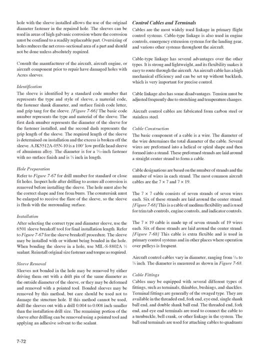 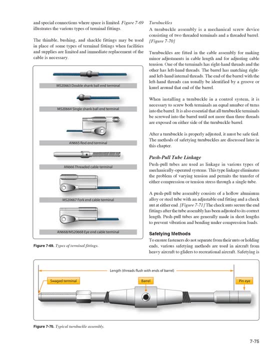 cable to a turnbuckle, bell, crank or other linkage in the system. The ball end terminals are used for attaching cables to quadrants And special connections where space is limited. Figure 769 illustrates the various types of terminal fittings: The thimble, bushing and shackle. 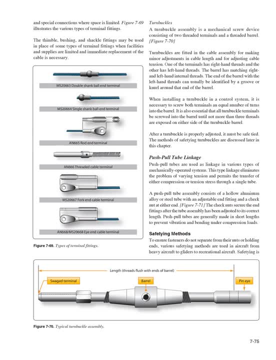 fittings may be used in place of some types of terminal fittings when facilities and supplies are limited. Figure 770: Turnbuckles are fitted in the cable assembly for making minor adjustments in cable length and for adjusting cable tension. One of the terminals has right-hand threads and the other 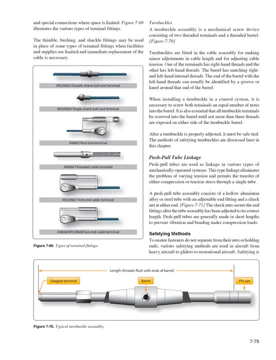 has left-hand threads. The barrel has matching right and left-hand internal threads. The end of the barrel with the left-hand threads can usually be identified by a groove or knurl around that end of the barrel. When installing a turnbuckle in a control system, it is necessary to screw. 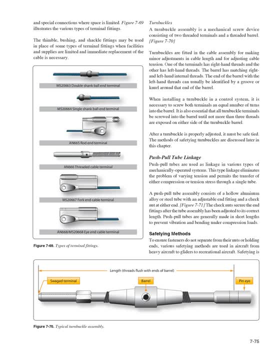 both terminals an equal number of turns into the barrel. It is also essential that all turnbuckle terminals be screwed into the barrel until not more than three threads are exposed on either side of the turnbuckle barrel. After a turnbuckle is properly adjusted, it must be safe, tied. 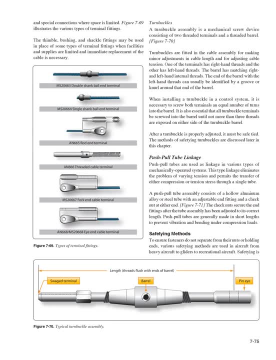 The methods of safetying turnbuckles are discussed later in this chapter. Push-pull tube linkage. Push-pull tubes are used as linkage in various types of mechanically operated systems systems. This type linkage eliminates the problem of varying tension and permits the transfer of. 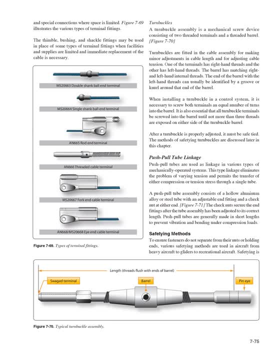 either compression or tension stress through a single tube. A push-pull tube assembly consists of a hollow aluminum, alloy or steel tube with an adjustable end fitting and a check nut at either end- Figure 771,. the check nuts secure the end fittings after the tube assembly has been adjusted. 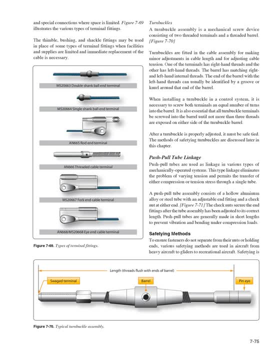 to its correct length. Push-pull tubes are generally made in short lengths to prevent vibration and bending under compression loads. Safetying methods to ensure fasteners do not separate from their nuts or holding ends. Various safetying methods are used in aircraft from heavy. 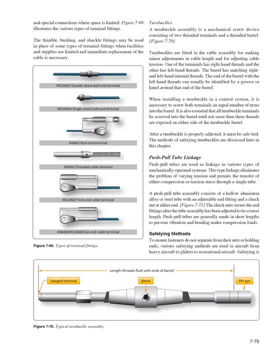 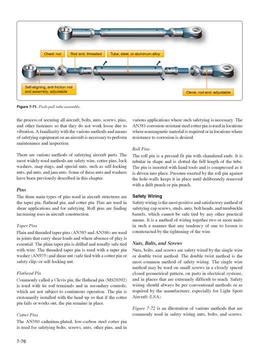 aircraft, to gliders, to recreational aircraft. Safetying is the process of securing all aircraft bolts, nuts, screws, pins and other fasteners so that they do not work loose due to vibration. A familiarity with the various methods and means of safetying equipment on an aircraft is necessary. 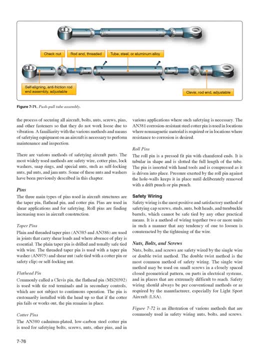 to perform maintenance and inspection. There are various methods of safetying aircraft parts. The most widely used methods are safety wire, cotter pins, lock washers, snap rings and special nuts such as self-locking nuts, pal nuts and jam nuts. Some of these nuts and washers have been previously described in this. 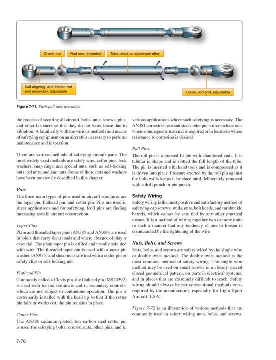 chapter Pins. The three main types of pins used in aircraft structures are the taper pin, flathead pin and cotter pin. Pins are used in shear applications and for safetying. Roll pins are finding increasing uses in aircraft construction. Taper pins- Plain and threaded taper pins- AN385 and AN386, are used in joints that carry shear loads. 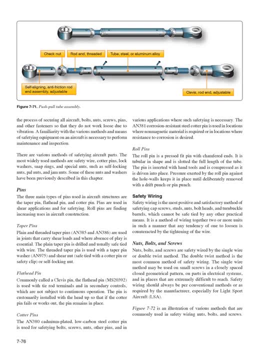 and where absence of play is essential. The plain taper pin is drilled and usually safe-tied with wire. The threaded taper pin is used with a taper pin washer- AN975, and shear nut safe-tied with a cotter pin or safety clip or self-locking nut Flathead pin, commonly called a clevis pin. 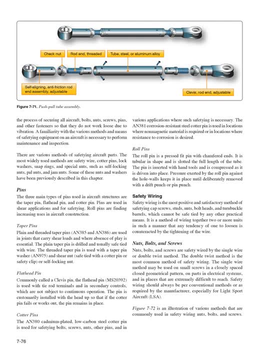 the flathead pin MS20392, is used with tie rod terminals and in secondary controls which are not subject to continuous operation. The pin is customarily installed with the headup so that if the cotter pin fails or works out, the pin remains in place. Cotter pins. 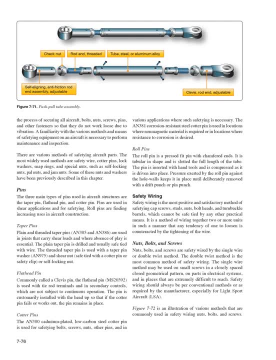 The AN380 cadmium-plated low-carbon steel cotter pin is used for safetying bolts, screws, nuts, other pins and in various applications where such safetying is necessary. The AN381 corrosion-resistant steel cotter pin is used in locations where non-magnetic 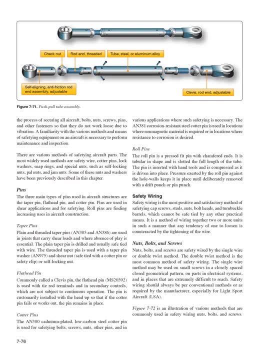 material as required or in locations where resistance to corrosion is desired. Roll pins: The roll pin is a pressed-fit pin with chamfered ends. It is tubular in shape and is slotted the full length of the tube. The pin is inserted with hand tools and is compressed as it is driven into place. 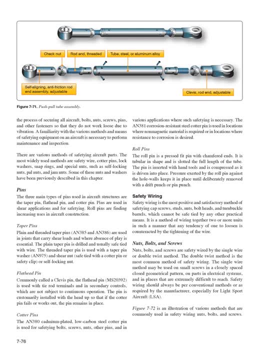 Pressure exerted by the roll pin against the whole walls keeps it in place until deliberately removed with a drift punch or pin punch- Safety wiring. Safety wiring is the most positive and satisfactory method of safety in cap screws, studs, nuts, bolt heads and turnbuckle barrels which cannot be safe-tied by any other practical. 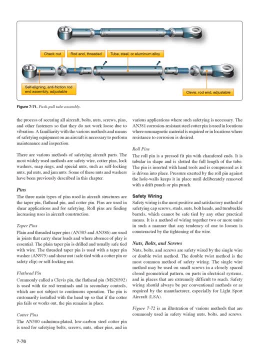 means. It is a method of wiring together two or more units in such a manner that any tendency of one to loosen is counteracted by the tightening of the wire, Nuts bolts and screws. Nuts bolts and screws are safety wired by the single wire or double twist method. The double twist method is: 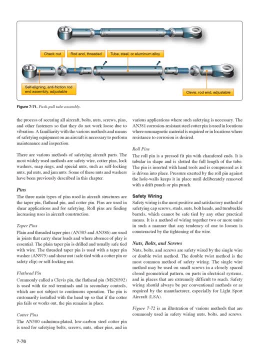 the most common method of safety wiring. The single wire method may be used on small screws in a closely spaced, closed geometrical context. Safety wiring should always be per conventional methods or as required by the manufacturer, especially for light sport aircraft LSA. Figure 7-72 is an illustration of various 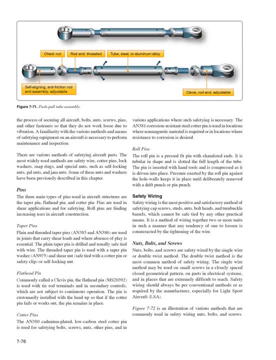 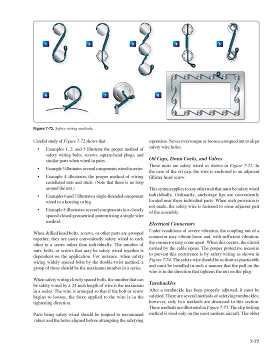 methods that are commonly used in safety wiring: nuts, bolts and screws. Careful study of figure 7-72 shows that Examples 1,, 2, and 5 illustrate the proper method of safety wiring bolts, screws, square head plates and nuts. 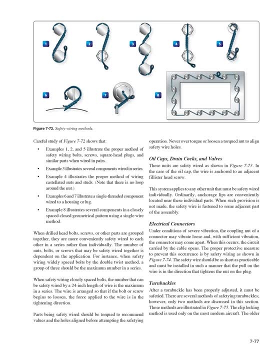 The proper method of safety wiring- bolts, screws, square heads, nuts, bolts and screws- is based on the specific method of safety wiring. The proper method of safety wiring is based on the specific method of safety wiring. Example 3 illustrates several components. 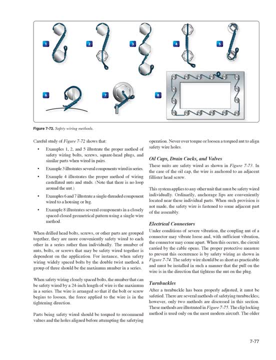 wired in series. Example 4 illustrates the proper method of wiring castellated nuts and studs. Note that there is no loop around the nut. Example 6 and 7 illustrate a single threaded component wired to a housing or lug. Example 8 illustrates several components in a closely. 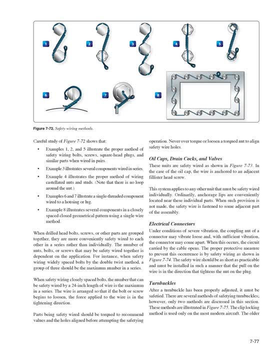 spaced, closed geometrical pattern using a single wire method. When drilled head bolts, screws or other parts are grouped together, they are more conveniently safety-wired to each other in a series rather than individually. The number of nuts, bolts or screws that may be safety-wired: 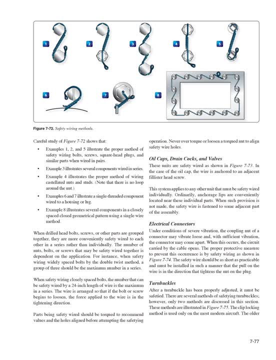 together is dependent on the application. For instance, when safety-wiring widely-spaced bolts by the double-twist method, a group of three should be the maximum number in a series. When safety-wiring closely-spaced bolts, the number that can be safety-wired by a 24-inch 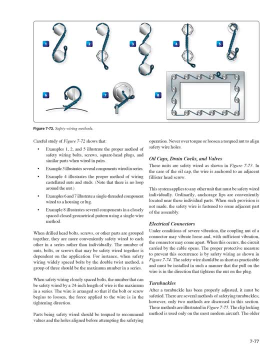 length of wire is the maximum in a series. The wire is arranged so that if the bolt or screw begins to loosen, the force applied to the wire is in the tightening direction. Parts being safety-wired should be torqued to recommend values and the holes aligned before. 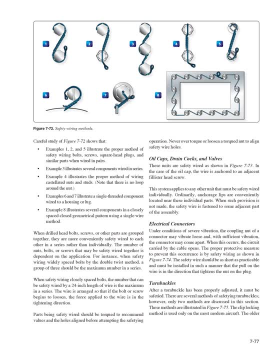 attempting the safetying operation, Never over-torque or loosen a torque nut to align safety-wire holes, Oil caps, drain cocks and valves. these units are safety-wired as shown in figure 7-73.. In the case of the oil cap, the wire is anchored to an adjacent filister. 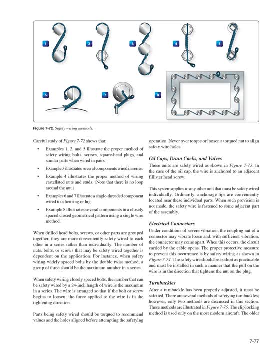 head. This system applies to any other unit that must be safety-wired individually. Ordinarily, anchorage lips are conveniently located near these individual parts. When such provision is not made, the safety wire is fastened to some adjacent part of the assembly. 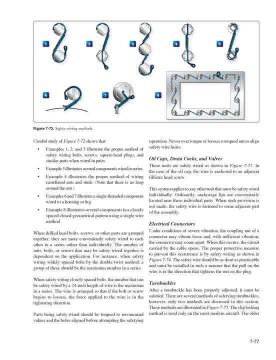 Electrical connectors. under conditions of severe vibration, the coupling nut of a connector may vibrate loose and, with sufficient vibration, the connector may come apart. When this occurs, the circuit carried by the cable opens. The proper protective measure to prevent this occurrence is by safety-wiring, as shown in figure 7-74.. 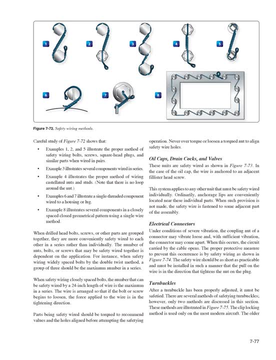 The safety wire should be as short as practicable and must be installed in such a manner that the pull on the wire is in the direction that tightens the nut on the plug. Turnbuckles: After a turnbuckle has been properly adjusted, it must be safetied. There are several methods. 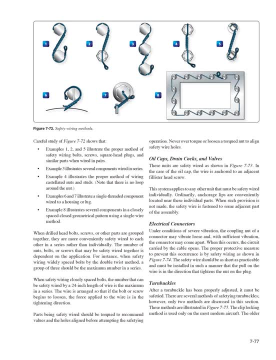 of safetying turnbuckles. however, only two methods are discussed in this section. These methods are illustrated in figure 7-75.. The clip-locking method is used only on the most modern air-conditioning units. The clip-locking method is used only on the most modern air-conditioning units. 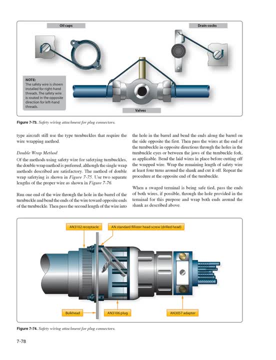 The older type aircraft still use the type turnbuckles that require the wire-wrapping method- Double-wrap method. of the methods using safety wire for safetying turnbuckles, the double-wrap method is preferred, although the single-wrap methods described are satisfactory. 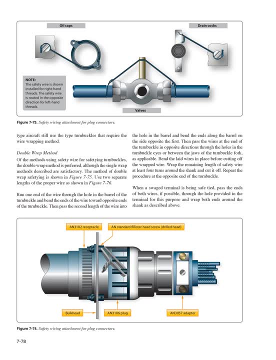 The method of double-wrap safetying is shown in figure 7-75.. Use two separate lengths of the proper wire, as shown in figure 7-76.. Run one end of the wire through the hole in the barrel of the turnbuckle and bend the ends of the. 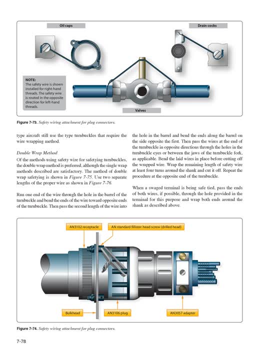 wire toward opposite directions. The method of double-wrapping method is used only on the opposite ends of the turnbuckle. Then pass the second length of the wire into the hole in the barrel and bend the ends along the barrel on the side opposite the first. Then pass the wires at 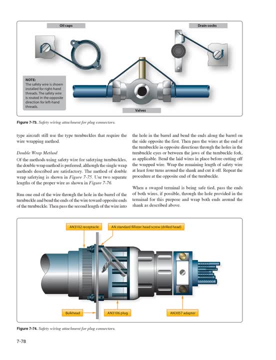 the end of the turnbuckle in opposite directions, through the holes in the turnbuckle eyes or between the jaws of the turnbuckle fork, as applicable. Bend the laid wires in place before cutting off the wrapped wire. Wrap the remaining length of safety wire at least four turns around. 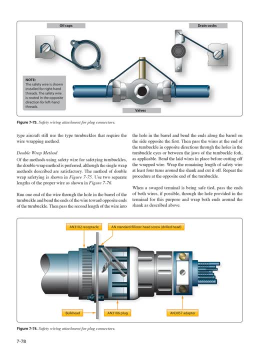 the shank and cut it off. Repeat the procedure at the opposite end of the turnbuckle. When a swash terminal is being safe-tied. pass the ends of both wires, if possible, through the hole provided in the terminal for this purpose and wrap both ends around the shank as described above. 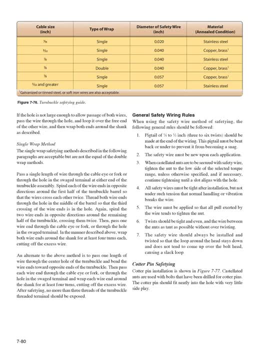 If the hole is not large enough to allow passage of both wires, pass the wire through the hole and loop it over the free end of the other wire and then wrap both ends around the shank as described. Single-wrap method: The single-wrap safetying methods described in the following: 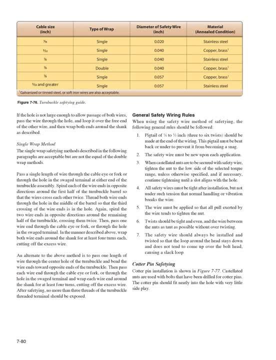 paragraphs are acceptable but are not the equal of the double-wrap methods. Pass a single length of wire through the shank and cut it off If the hole is not large enough to allow passage of both wires. pass a single length of wire through the hole in the swash terminal at either end of the 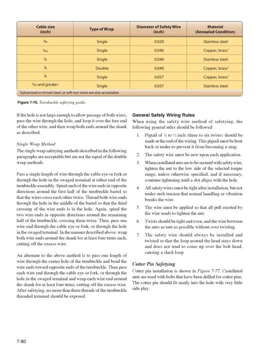 turnbuckle assembly Spiral. each of the wire ends in opposite directions around the first half of the turnbuckle barrel so that the wires cross each other twice. Thread both wire ends through the hole in the middle of the barrel so that the third crossing of the wire ends is in the hole. 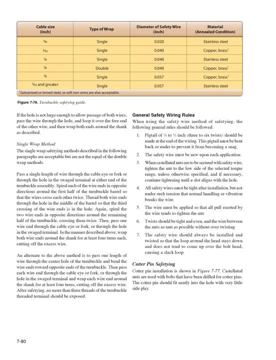 Again. spiral the two wire ends in opposite directions around the remaining half of the turnbuckle, crossing them twice. Then pass one wire end through the cable eye or fork or through the hole in the swash terminal In the manner described above. wrap both wire ends around the shank for at least four turns each. 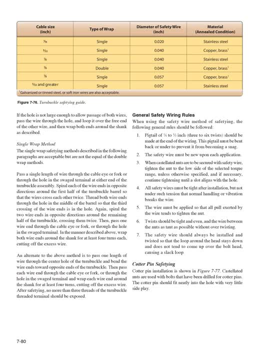 cutting off the excess wire. An alternate to the above method is to pass one length of wire through the center hole of the turnbuckle and bend the wire ends toward opposite ends of the turnbuckle, Then pass each wire end through the cable, eye or fork or through the hole in the 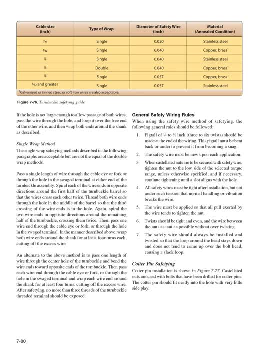 swage terminal and wrap each wire end around the shank for at least four turns, cutting off the excess wire. After safetying, no more than three threads of the turnbuckle threaded terminal should be exposed. General safety wiring rules. when using the safety wire method of safetying The 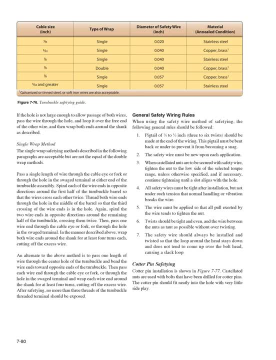 following general rules should be followed: 1. Pigtail of one quarter to half inch. three to six twists should be made at the end of the wiring. This pigtail must be bent back or under to prevent it from becoming a snag. 2. The safety wire must be new upon each application. 3. When castellated, 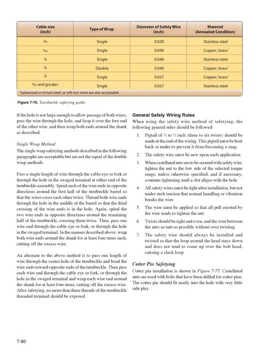 nuts are to be secured with safety wire, tighten the nut to the low side of the selected torque range, Unless otherwise specified, and, if necessary, continue tightening until a slot aligns with the hole 4.. All safety wires must be tight after installation, but not under such tension that 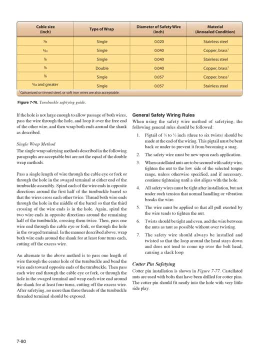 normal handling or vibration breaks the wire. 5. The wire must be applied so that all pull exerted by the wire tends to tighten the nut. 6. Twists should be tight and even and the wire between the nuts as taut as possible, without over twisting. 7. The safety wire should always be. 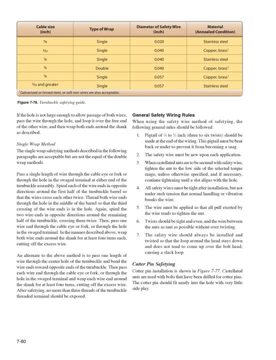 held and twisted so that the loop around the head stays down and does not tend to come up over the bolt head, causing a slack loop. Cotter pin safety and cotter pin installation as shown in figure 777.. Castellated nuts are used with bolts that have been drilled for cotter pins. The cotter pin. 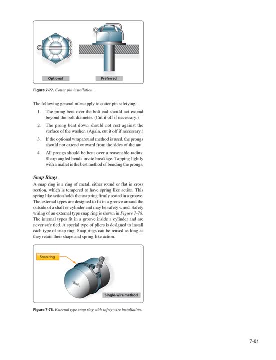 should fit neatly into the hole with very little side play. The following general rules apply to cotter pin safetying: 1. The prong bent over the bolt end should not extend beyond the bolt diameter. Cut it off if necessary. 2. The prong bent.